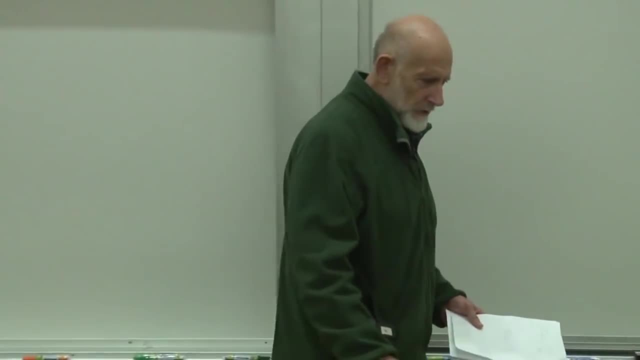 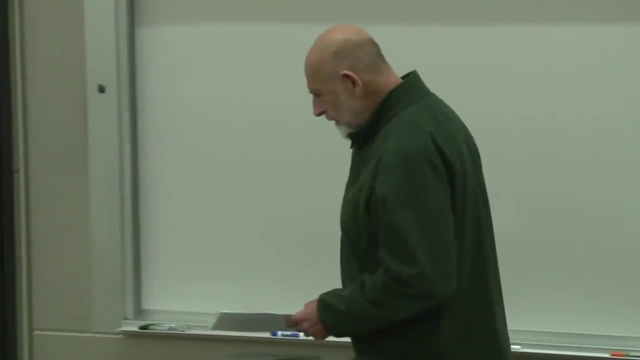 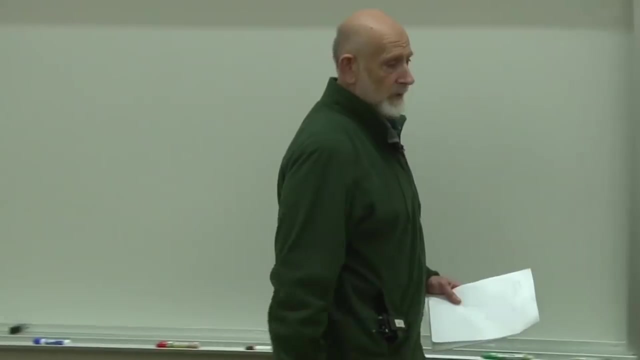 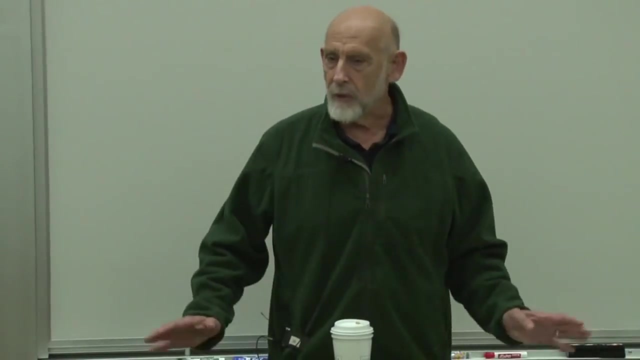 forces, particularly magnetic forces on charged particles. Electric forces: electric forces means electrostatic forces, the forces due to electric fields produced by charged particles standing still. Static electric forces. Those forces are of the type of garden variety of forces that we've already studied. What do I mean garden variety? I mean simply this: that the force 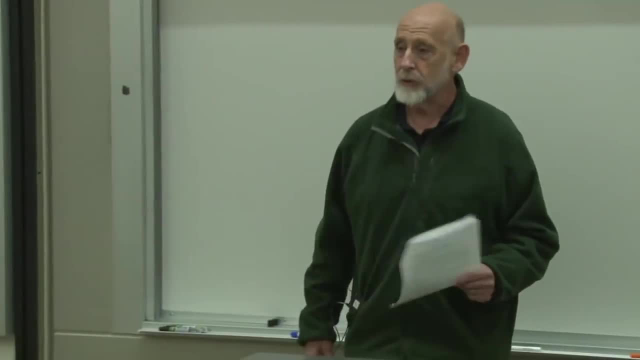 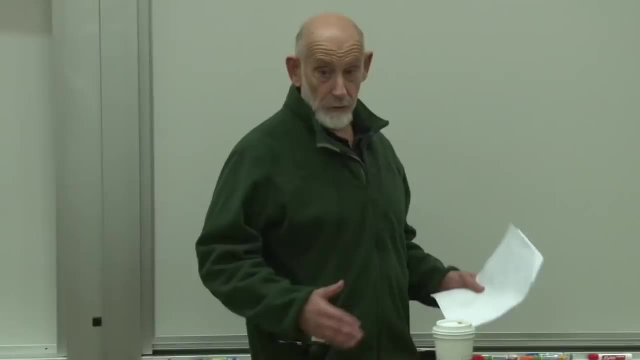 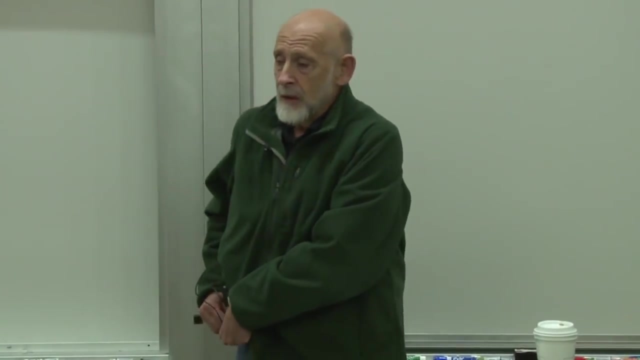 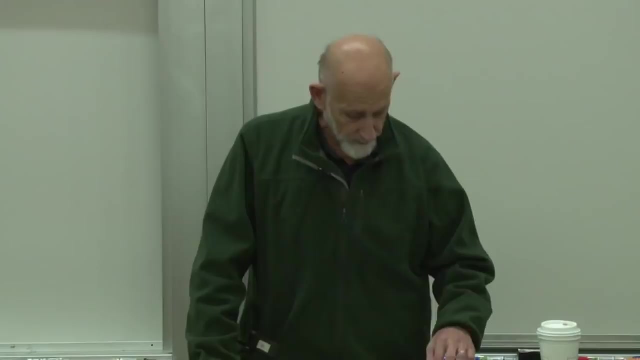 is described by the derivative of a potential energy with respect to position. Remember the formula F is equal to minus the gradient or the derivative of the potential energy. That rule was equivalent to energy conservation. We derived energy conservation from it And 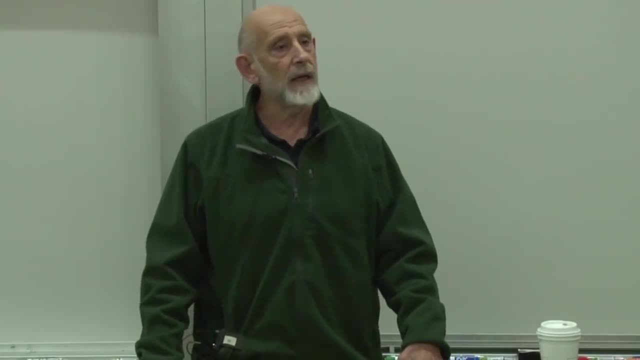 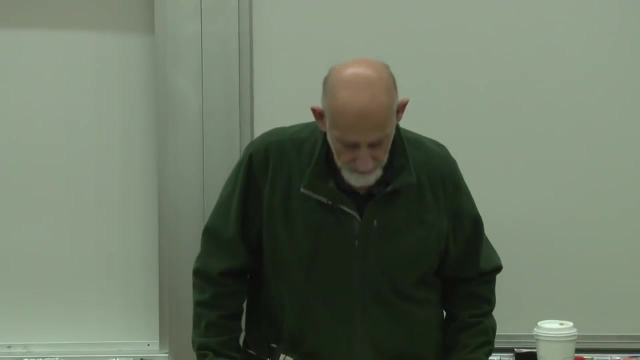 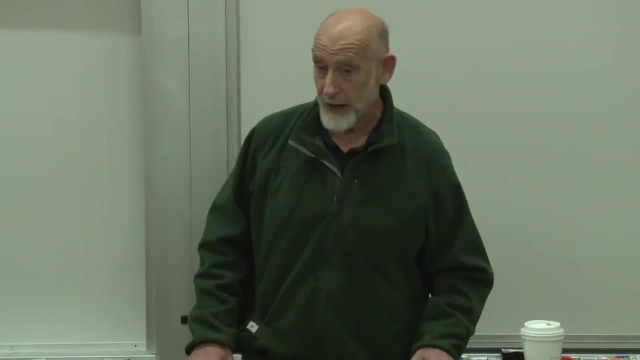 there's nothing new as far in that respect in electrostatic forces on charged particles. What is new is when there are magnetic field present. Magnetic fields have forces which are not described by the kinds of rules that we've set up up till now. They are described. 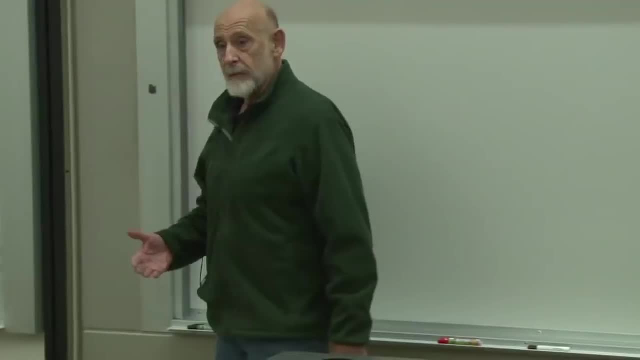 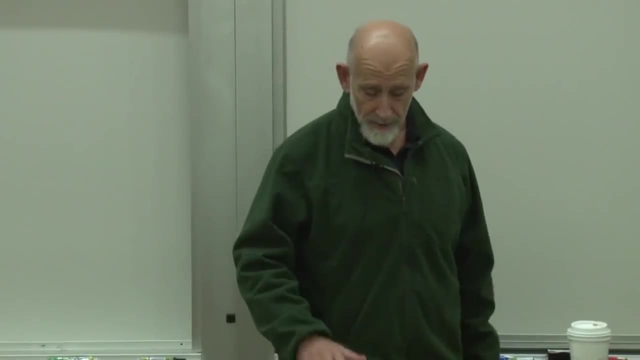 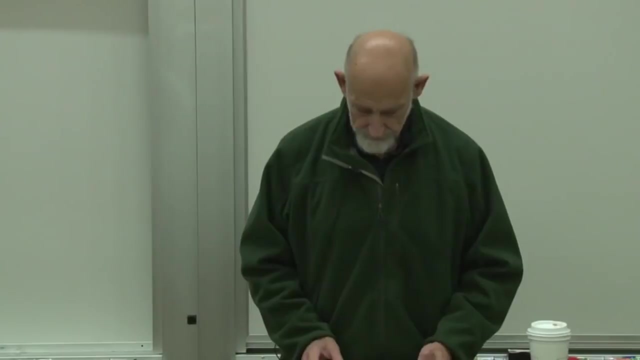 and we will talk about it in a general sense by principle of least action, by Lagrangian, by Hamiltonian, all that kind of stuff is right, but the equations of motion are of a different type than we've studied up till now. So we get to that tonight: Electric and 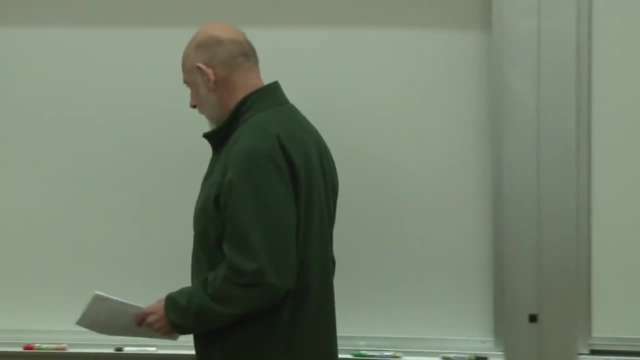 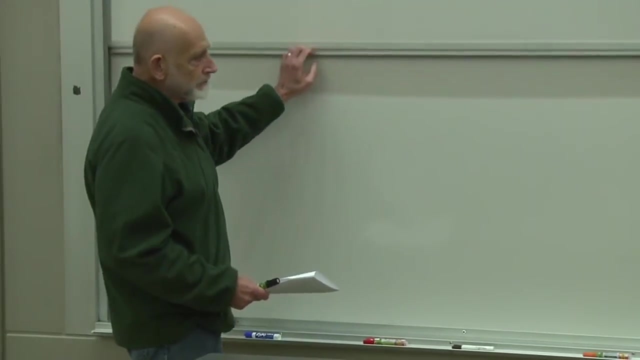 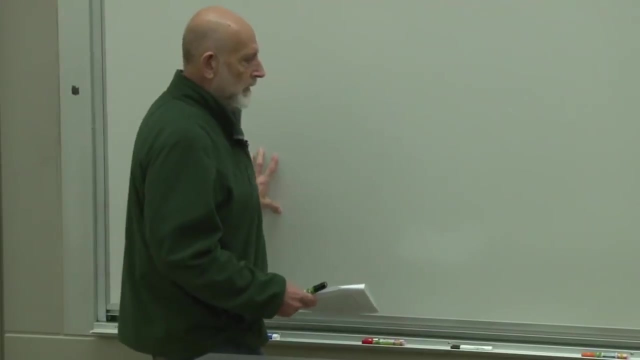 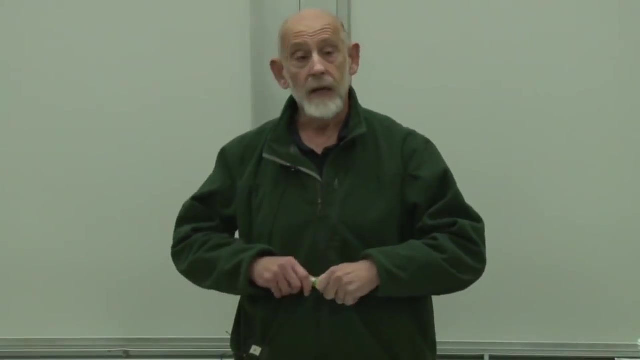 magnetic fields and their influence on charged particles. Before we do that, I think we have to a mathematical interlude. for many of you this will be old stuff, for some of you not, and since the purpose of this course is to start really at the beginning and uh, 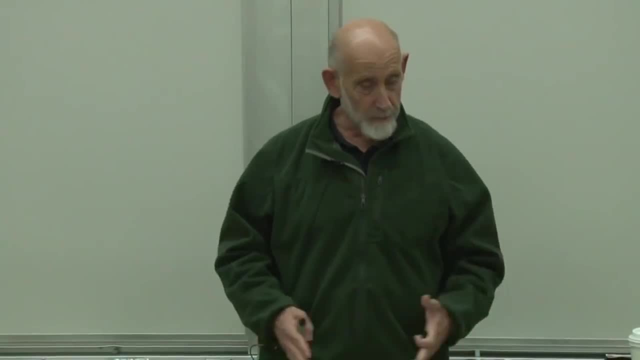 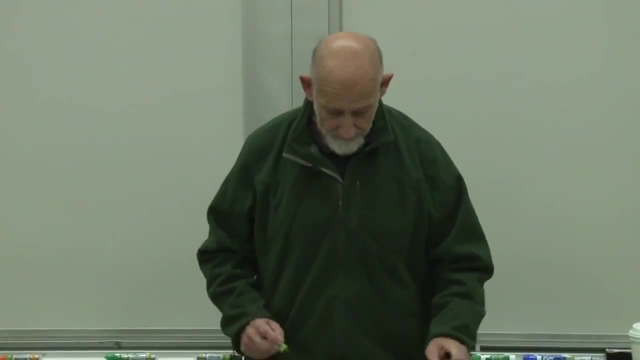 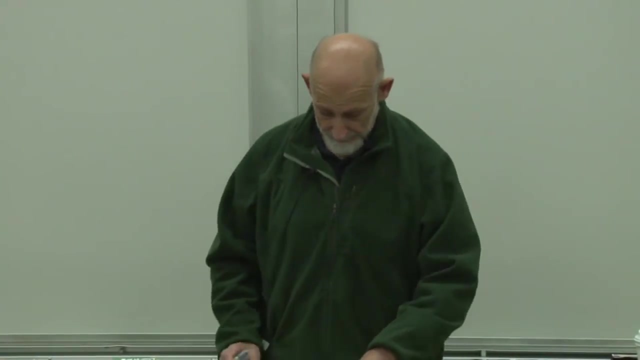 continue through each step being spelled out in detail, both for you and for the people who, uh, who are on the other end of that camera over there. uh, i'm going to spend a little bit of time talking about vector calculus. how many people are really familiar with vector calculus? 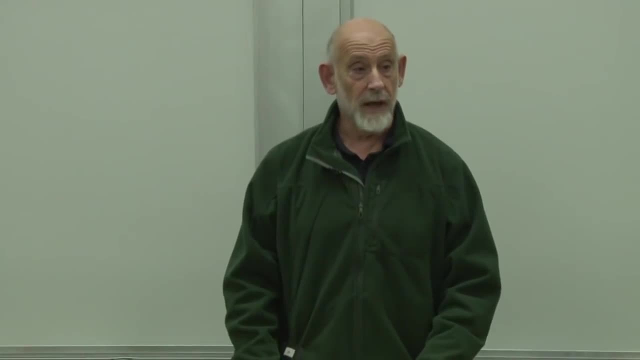 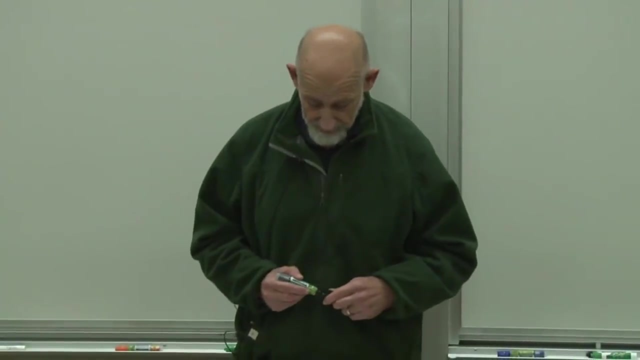 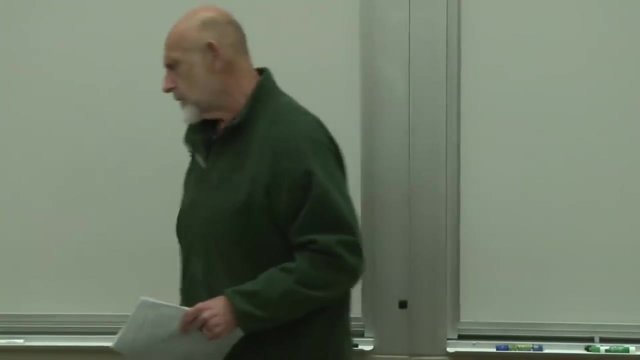 a good fraction of you. how many are not? so we're gonna spend a few minutes, maybe even uh, several minutes, talking about vector calculus and then move on to the uh, to the question at hand. all right fields. what is a field? 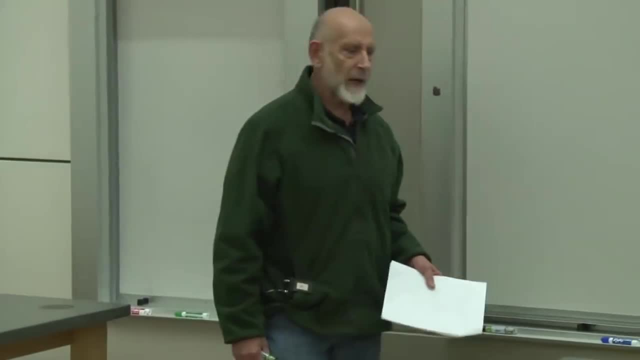 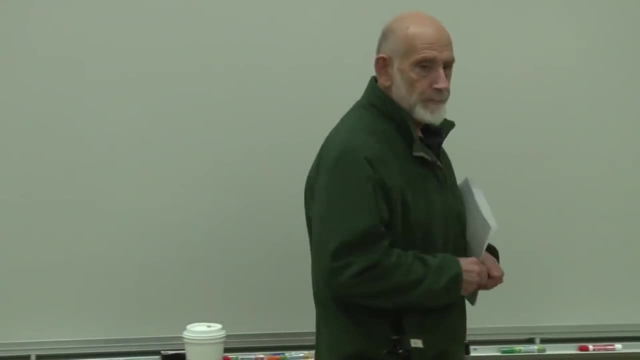 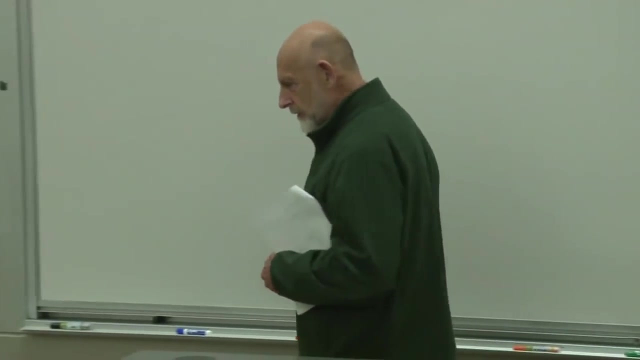 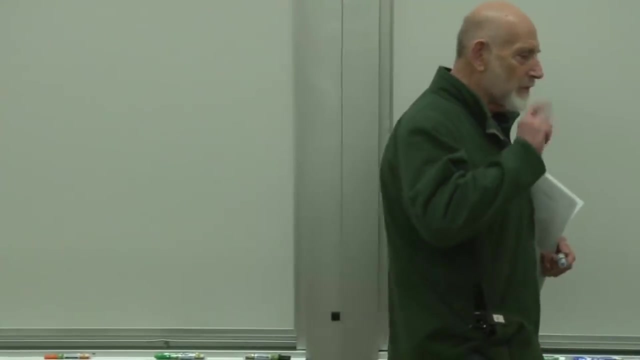 a field is simply a physical quantity which depends on space and time. an example of fields would be the temperature at any position, air pressure at any position. those are both scalar fields. they are not vectors, they don't have a sense of direction, they don't have components. i suppose you could say they have one component. 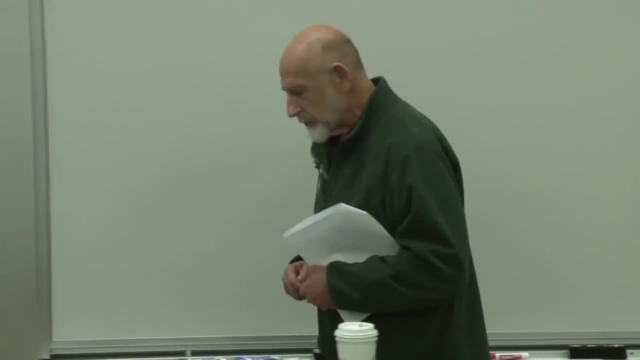 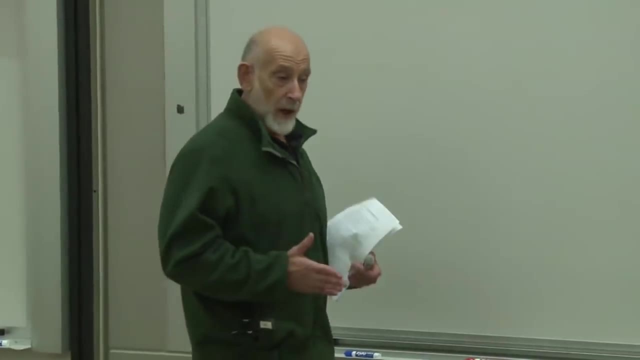 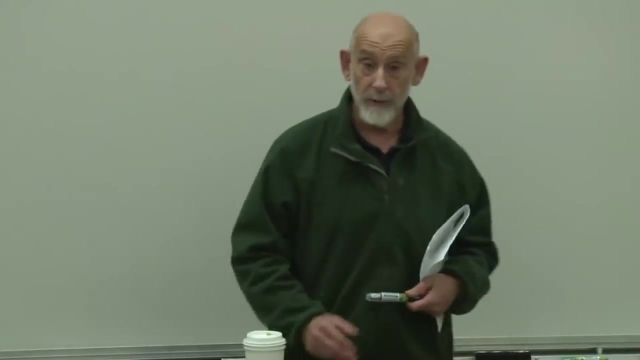 namely the value of the temperature or the pressure or the air pressure. another example taken from meteorology is a vector field, namely the wind velocity. the wind velocity has both a magnitude and a direction. it varies from place to place and it varies over time. fields can vary with respect to position. it can also vary with respect to time. 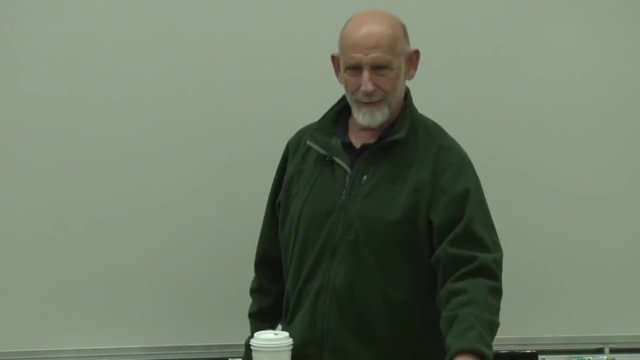 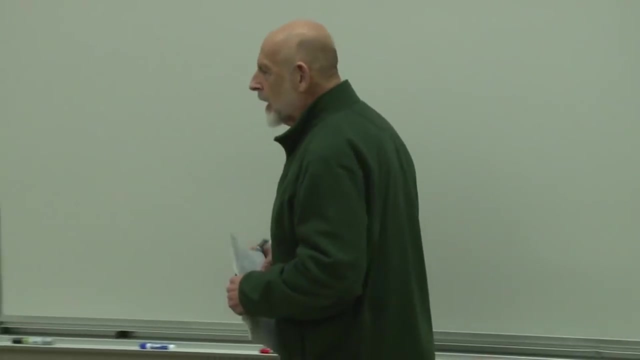 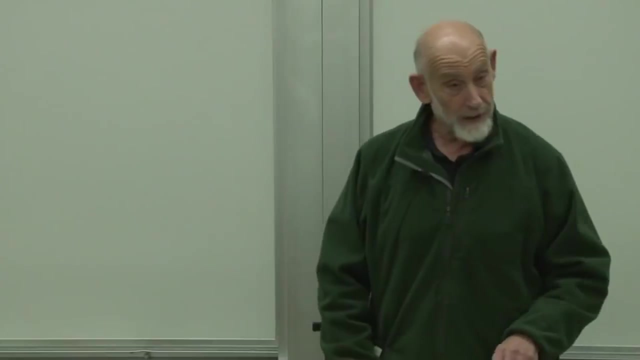 and so the wind velocity is a field, not of a fundamental kind, not of a kind like electric and magnetic fields, but nevertheless they are fields, they vary and the wind velocity is, as i said, a vector field. now we're not being another. this is not a course on meteorology. 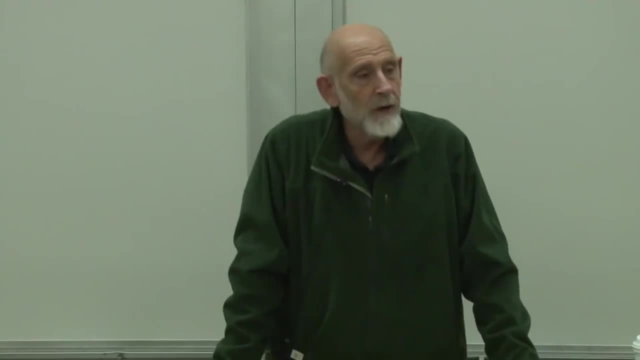 so we're interested in other kinds of fields, more fundamental in some sense, force fields. the electric field is a vector, it points in a direction and has a magnitude, and it's a field because it varies from place to place. likewise with the magnetic field. magnetic field: Are there scalar fields in nature? Yes, there are scalar fields in. 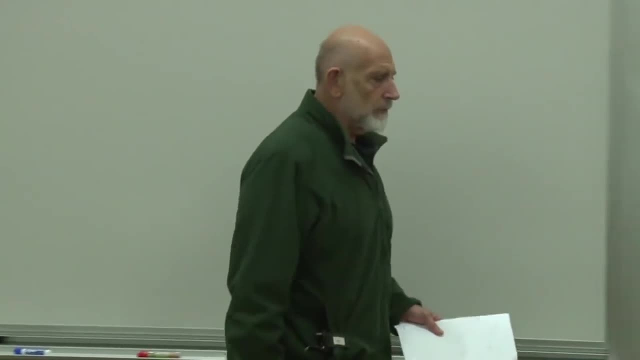 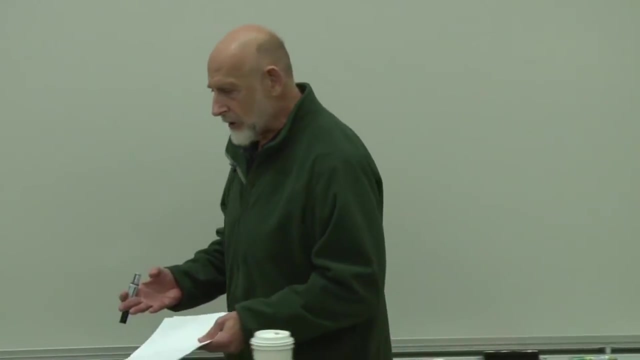 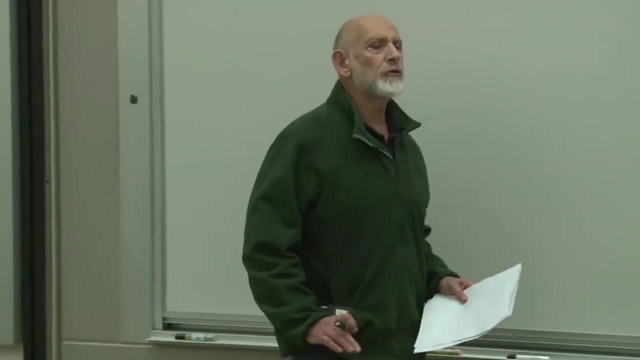 nature, but they happen to be not as apparent because they are very short range fields. They surround particles, they surround sources, sources of the field, but they have a range which is typically extremely small- particle physics scales- and so we don't see them in ordinary nature. The gravitational 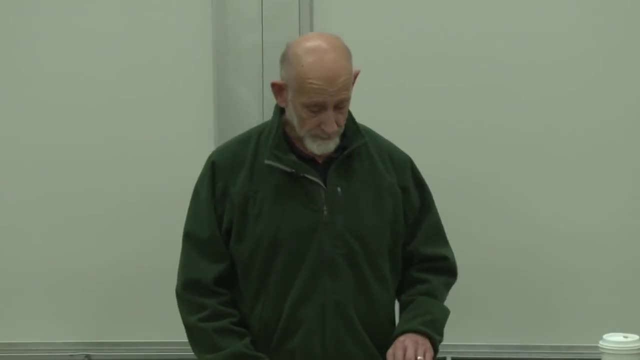 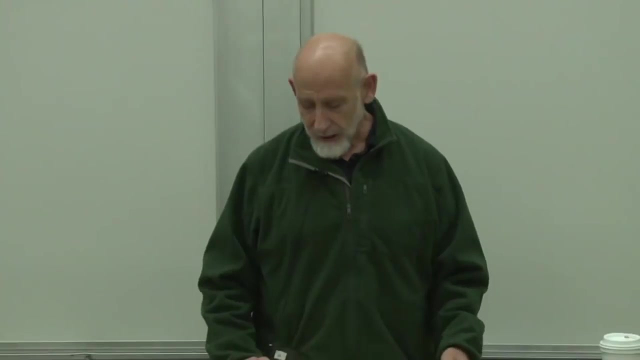 field is neither a vector nor a scalar. It's in fact a tensor. we're not going to get into that tonight. but the main thing which makes fields all fields is that they vary from place to place And, what's more, in most cases, with an exception. 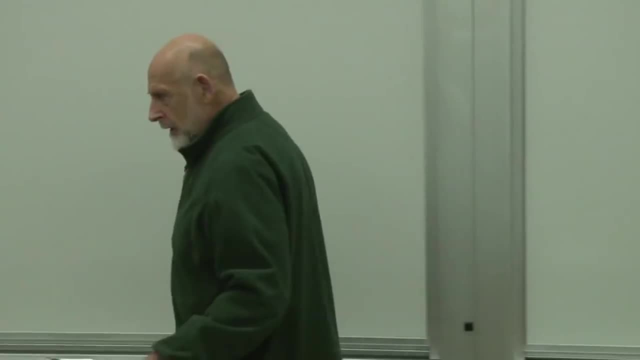 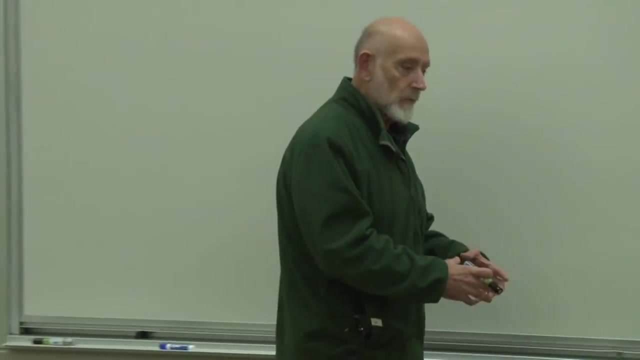 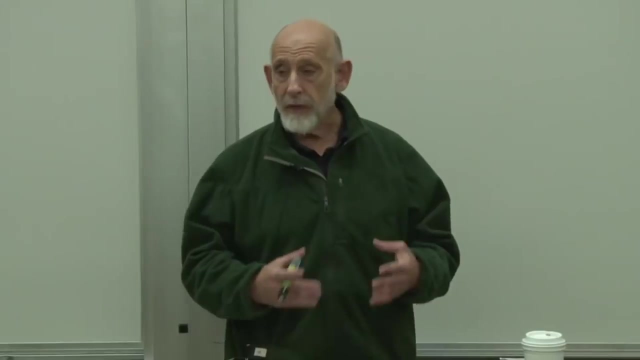 that we'll come to today. they are measurable in the sense that if you want to know the value of a field in a particular region of space and time, you can do an experiment in that region of space which will tell you what the value of the 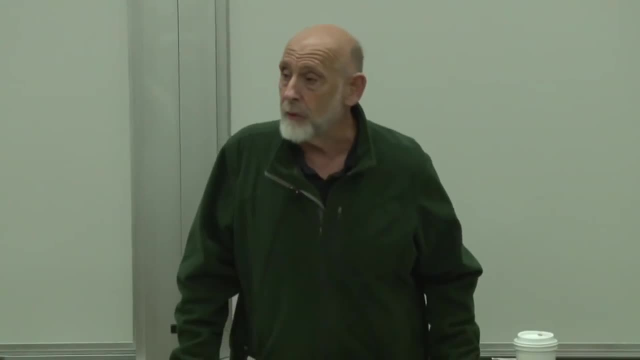 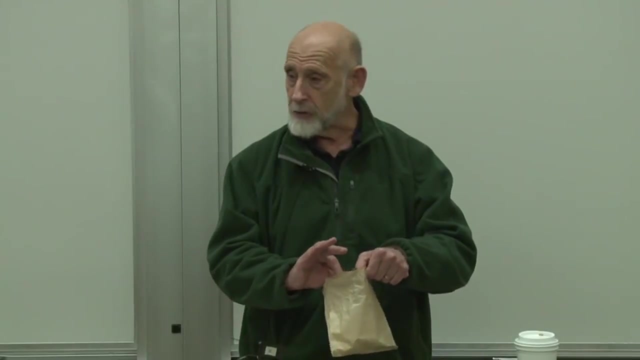 field is. For example, in the case of electric field, you want to do an experiment to find out what the electric field in this bag here. you put a charged particle into it and you see how the charged particle accelerates. You don't. 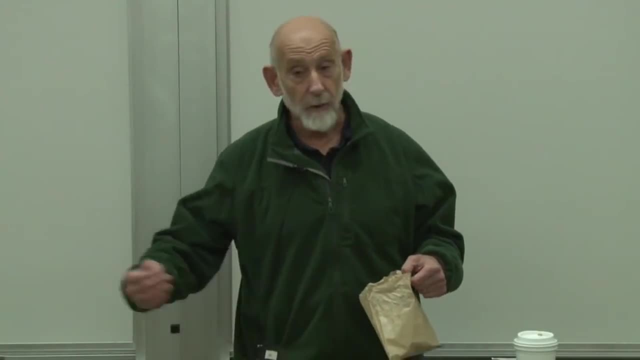 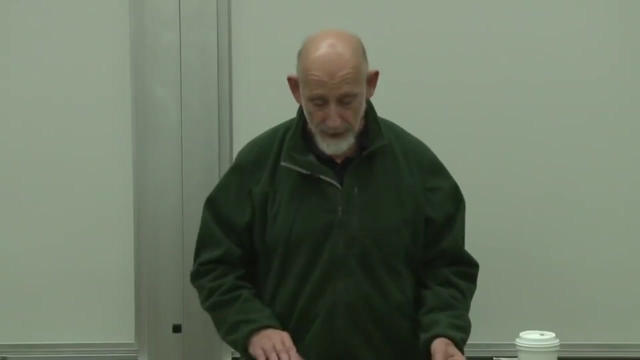 have to look outside the bag, you don't. it doesn't help you to put the particle outside the bag. you want to know the electric field inside the bag. you do the experiment inside the bag and that's called. that goes under the name of locality, The. 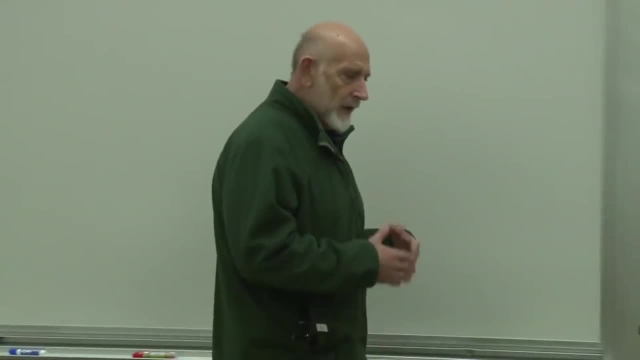 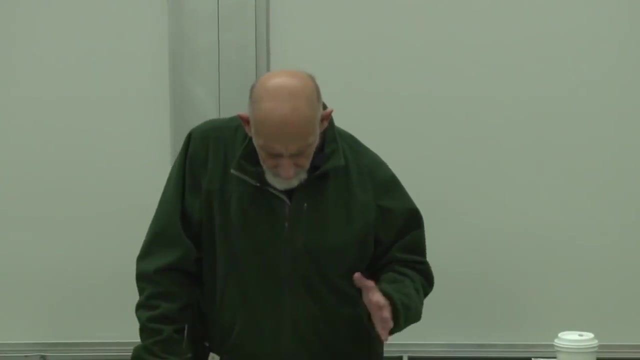 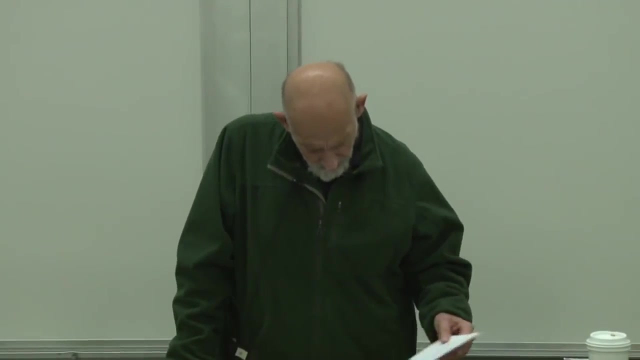 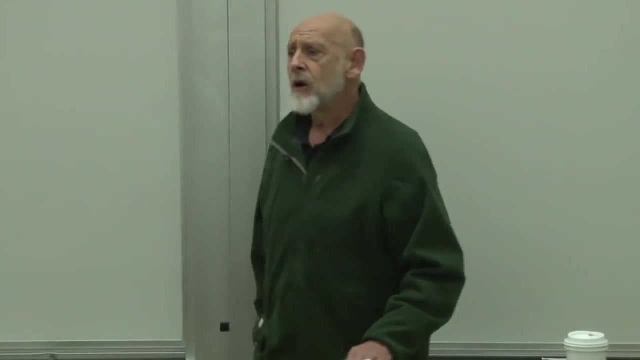 effect of the field is local. it influences things in its immediate neighborhood or it influences things wherever the field happens to be. As we'll see, there are some exceptions- an important exception to this idea, but we'll come to it. Okay, so we have fields which vary in space. We can different. we can do various. 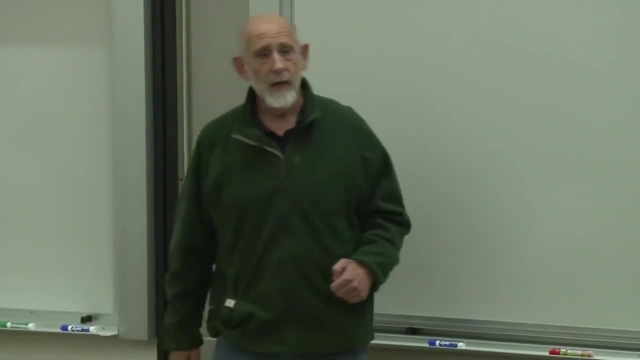 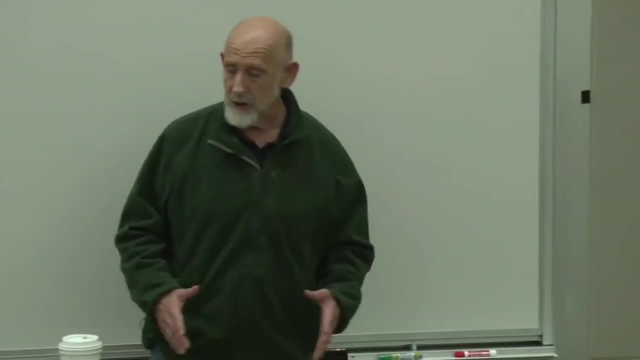 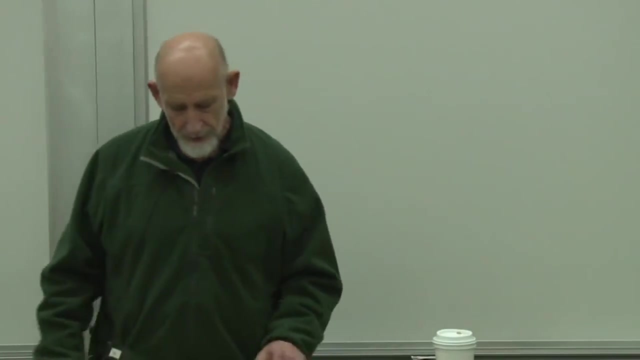 things to those fields to create other fields. but in particular, I'm interested in the things that we can do to the fields to create other fields, which we do by differentiating them. Any function, its derivative, is also a function. so any field, its derivative is also a field, and so there's an 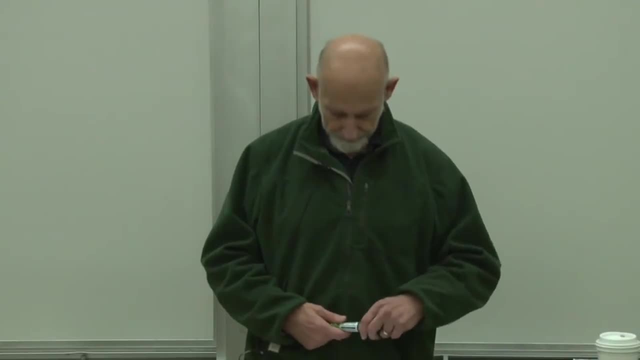 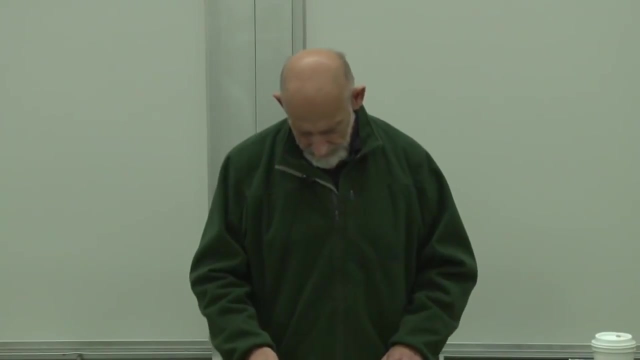 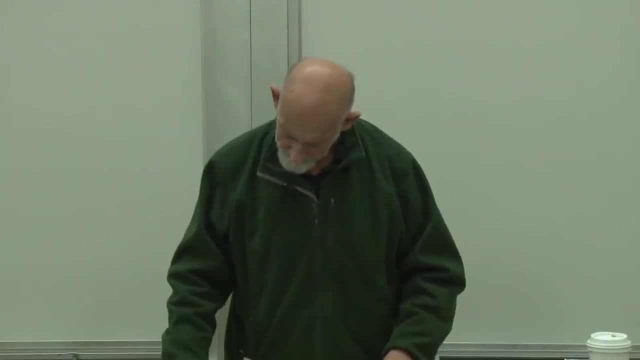 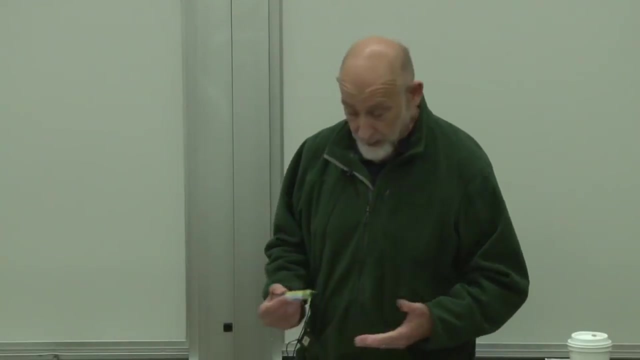 example, There's a calculus of fields that tells us how to create new kinds of fields from old kinds of fields. Okay, where am I To implement the idea of making fields out of fields? by by differentiation, we introduce a kind of fake vector. 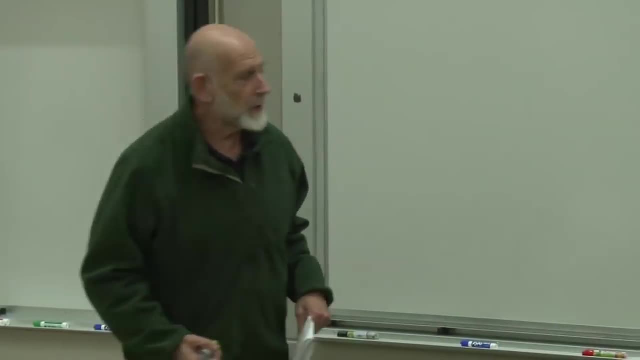 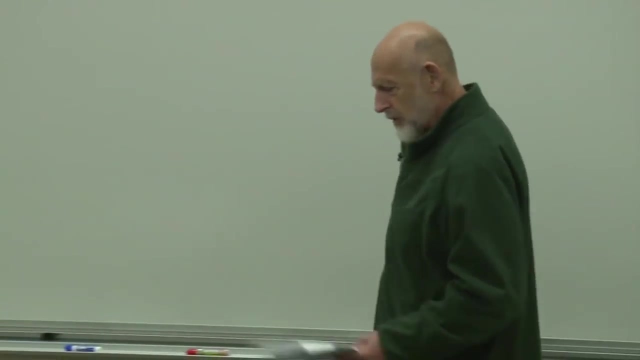 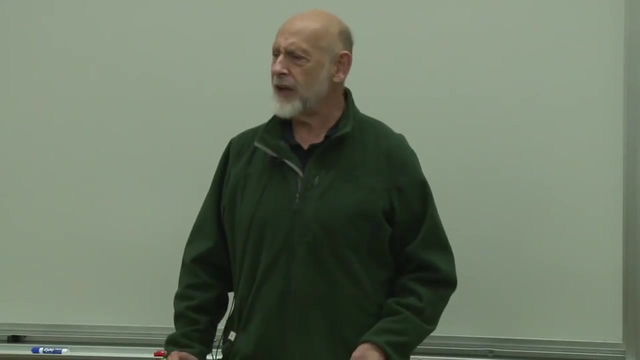 A fake vector. most of you know what it is. it goes by the name of nabla, Sometimes it's called nabla, sometimes it's called del, sometimes it's just written down as an upside down triangle. Can a triangle be upside down? What's a right side up? 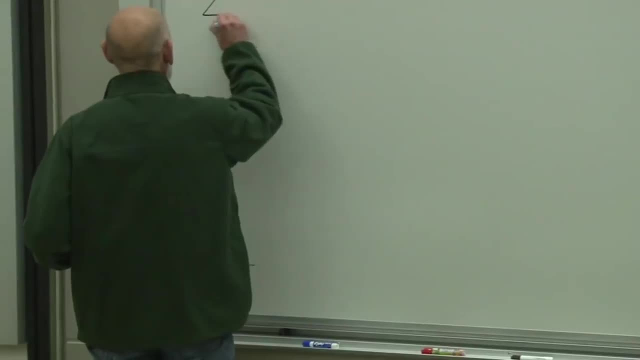 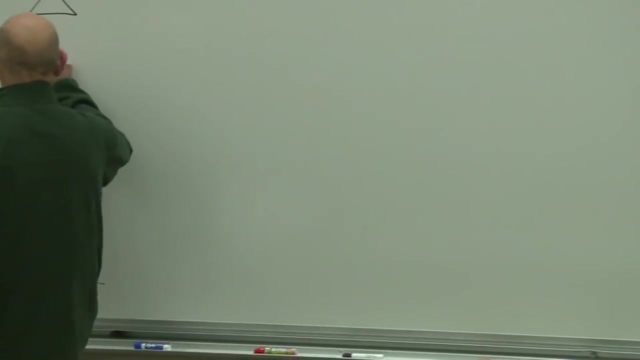 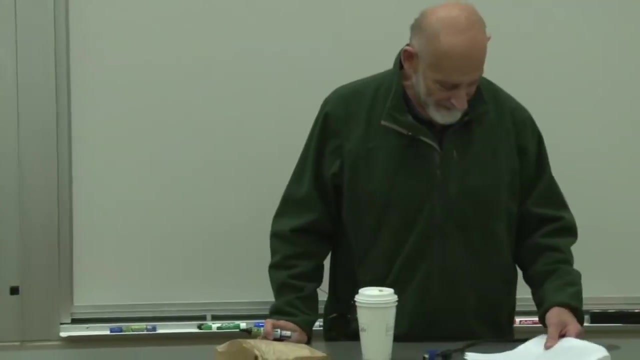 triangle. There's something about triangles that makes you want to draw them this way. right? That's a good, stable triangle, Right? This is an unstable triangle. right? This triangle is unstable. It's not a good triangle at all. Well, it's upside down. The symbol for del is an upside down triangle. 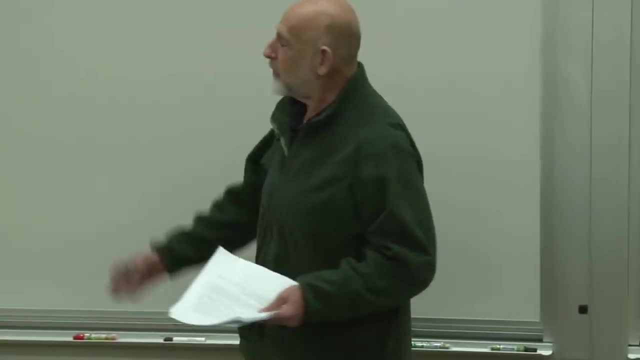 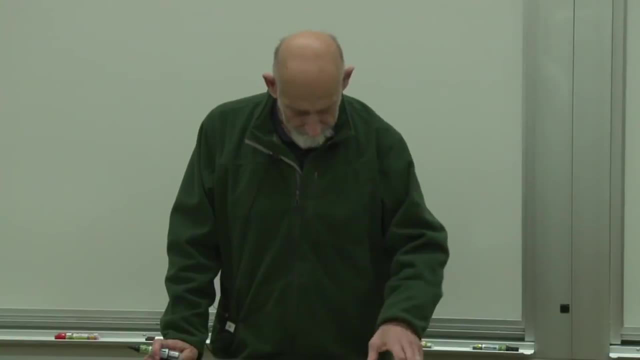 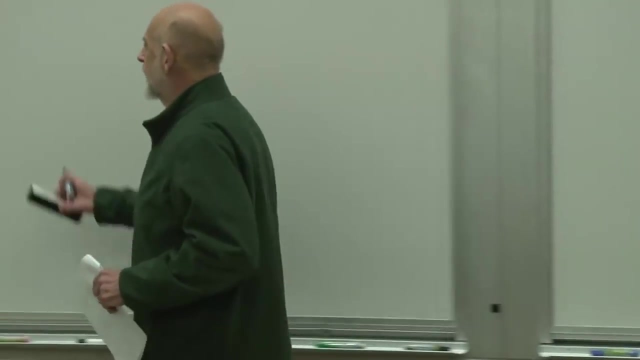 in that sense It's called del. Why is it called del? Because it looks like delta, but it's not delta. It's upside down delta and we think of it as an object which has components. So it's a vector. Well, it is and it isn't a vector. It's a kind of fake vector. And 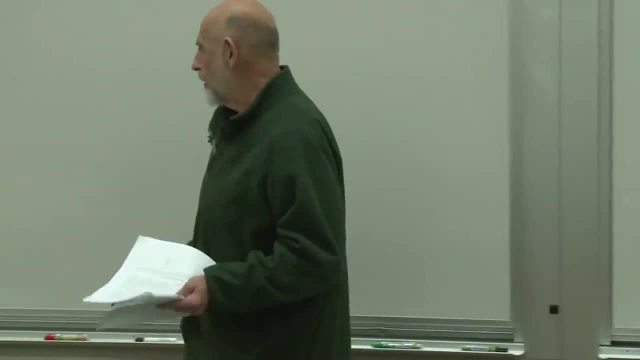 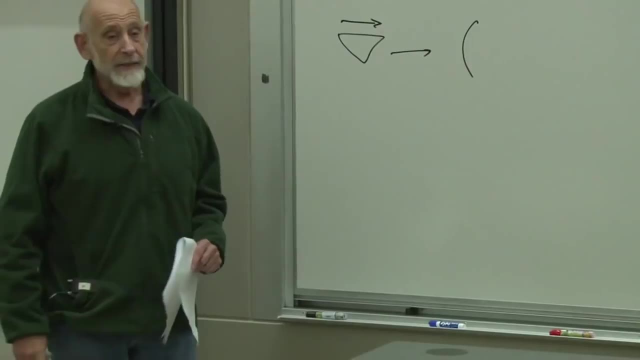 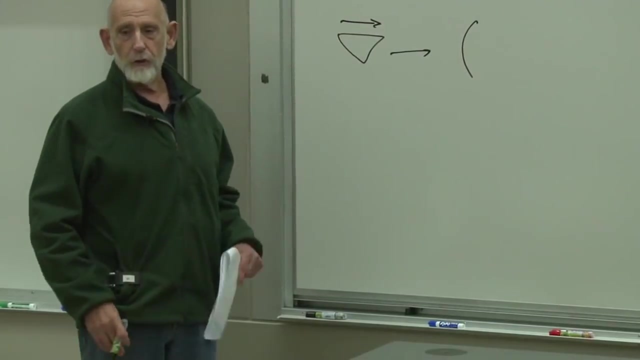 what are its components? Its components are fake components, So its components are. it has an. incidentally, we're talking about three-dimensional space now, not the, not the 26-dimensional space, not the three-dimensional configuration space where n is the number. 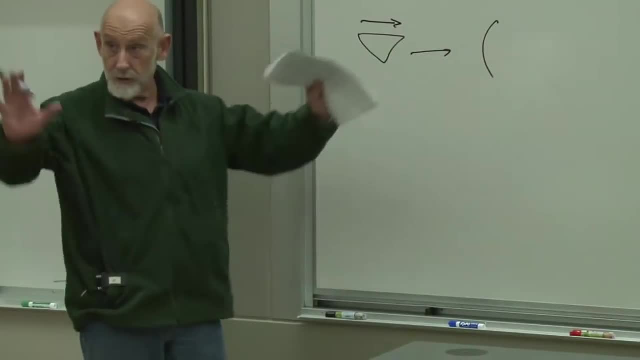 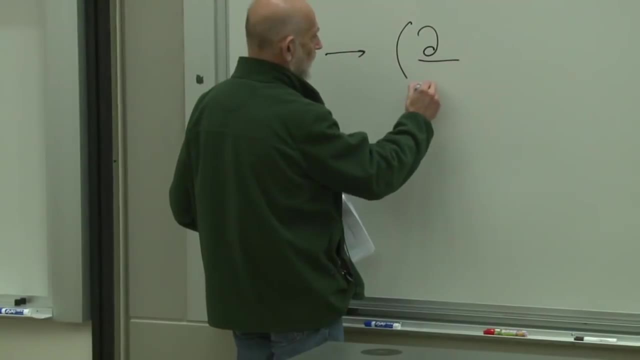 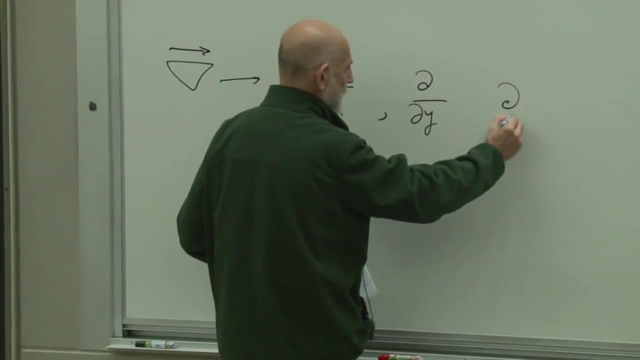 of particles. It's a six-dimensional phase space, Ordinary three-dimensional real space. Its components are derivative symbols: Derivative with respect to x, derivative with respect to y and derivative with respect to z. Now, what kind of vector is that? What direction is it pointing That? 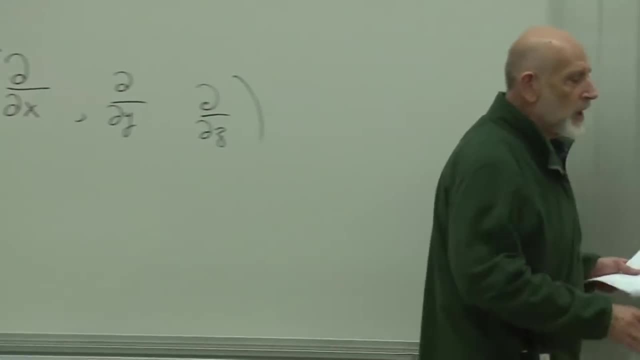 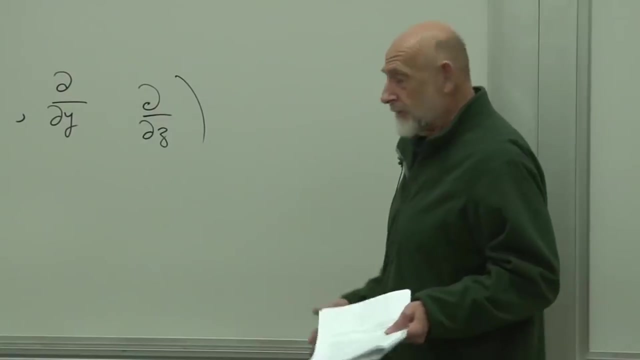 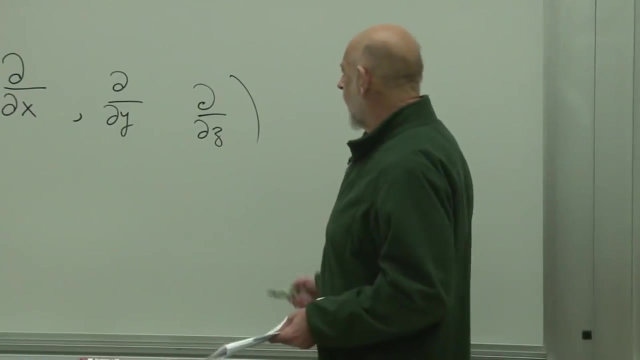 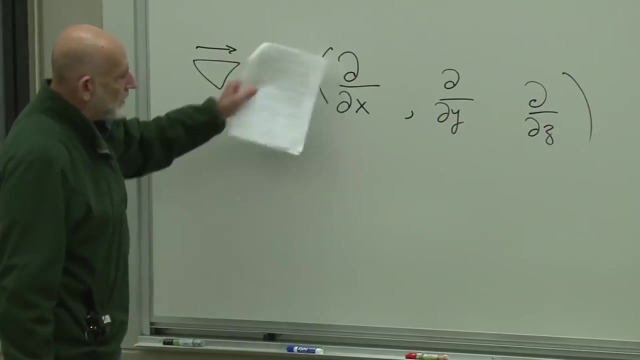 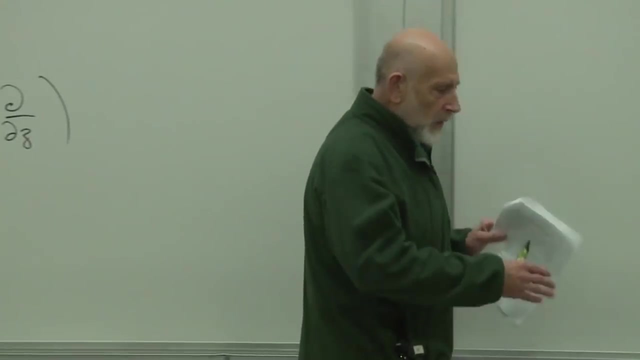 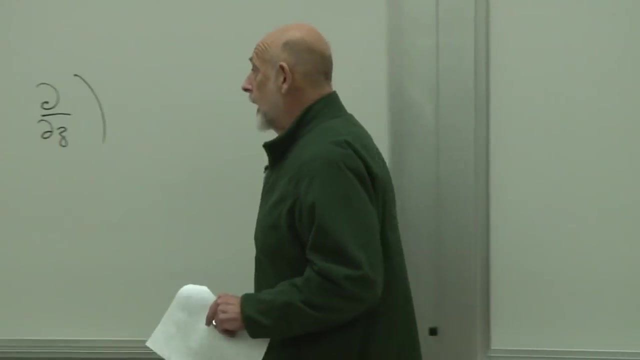 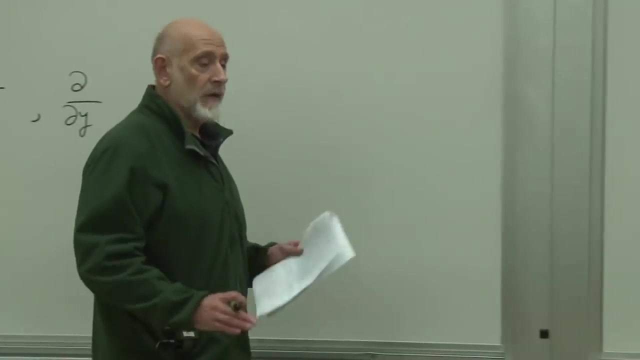 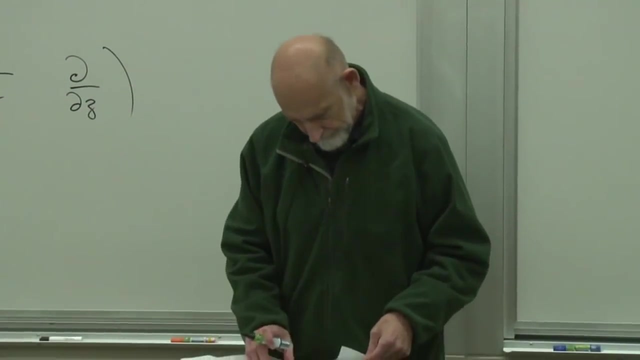 direction? is a point in that direction? How big is it? What's its magnitude? All of these questions are- And in the case of del, it acts on fields- to give other fields Okay, so let's take a few examples. First of all, supposing we have a scalar field, It could be the temperature. 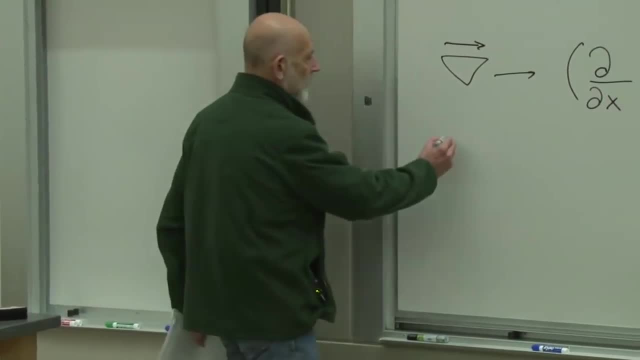 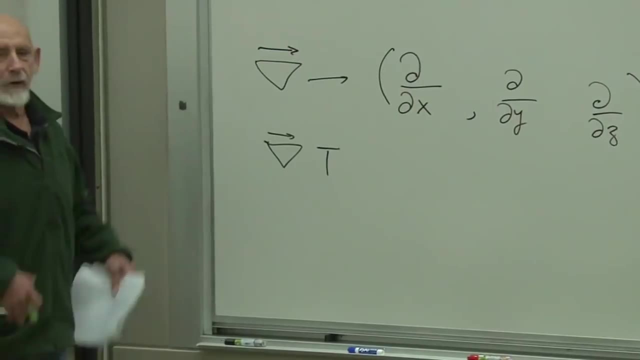 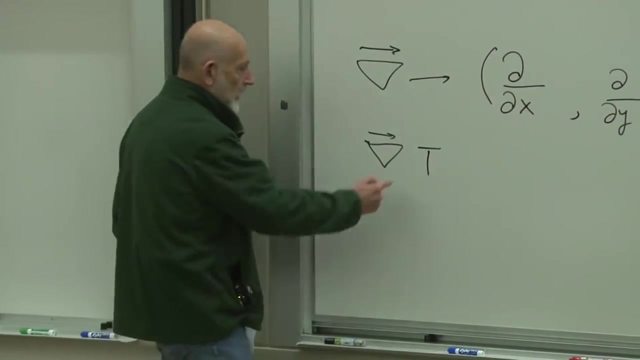 Let it be the temperature. All right Then. del is a symbol which can be fulfilled, let us say, by acting on a scalar function, or it can act on other things too. It acts on a scalar function. The temperature is a function of position and also time. but 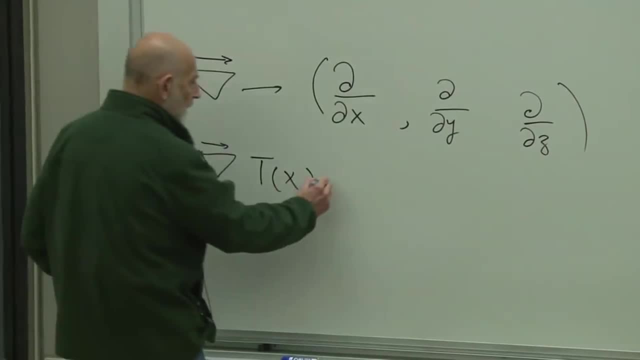 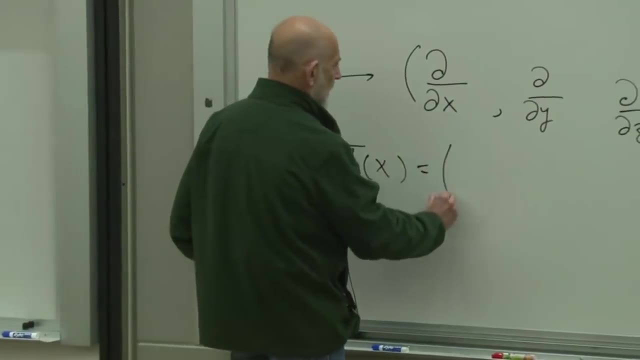 I'm going to suppress the time dependence for the moment. And now. this thing really is a vector. It has three components. The three components are: the derivative of the temperature with respect to x, the derivative of the temperature with respect to z, the 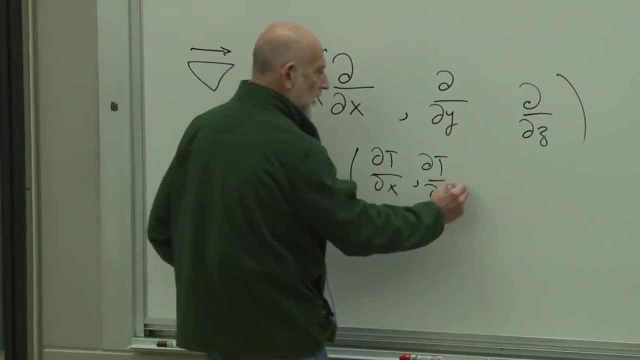 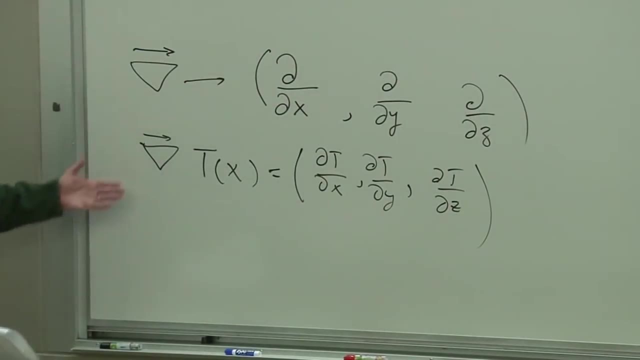 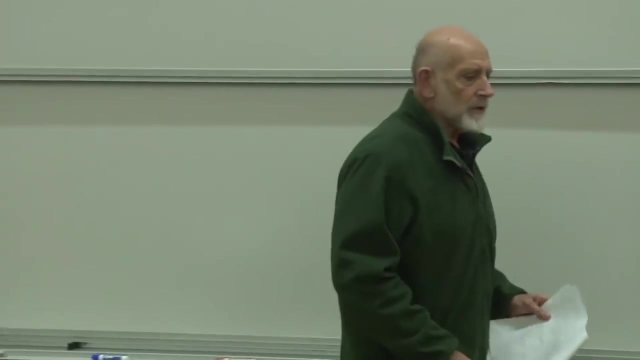 derivative of the temperature with respect to y, the derivative of the temperature with respect to y and the derivative of the temperature with respect to z, And that's the way del is used. Let's think about some more examples. This was the action. 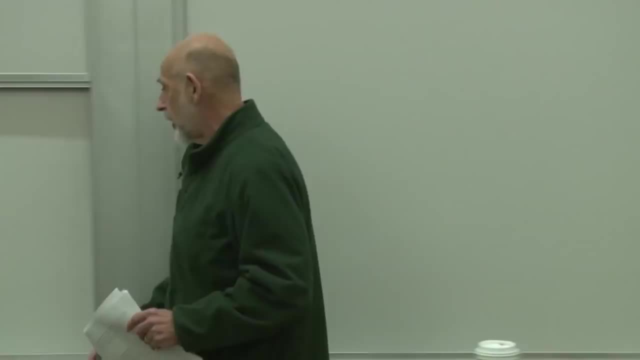 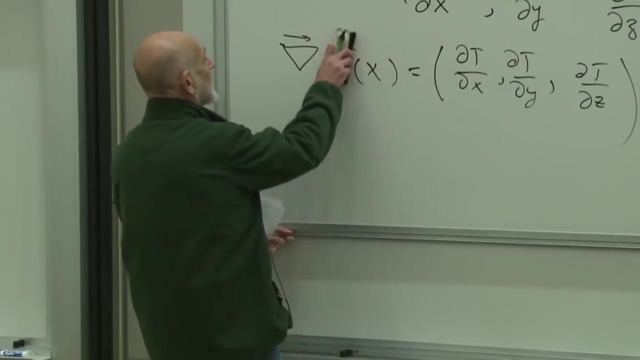 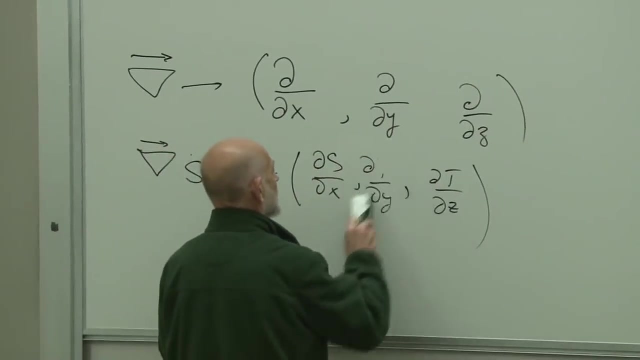 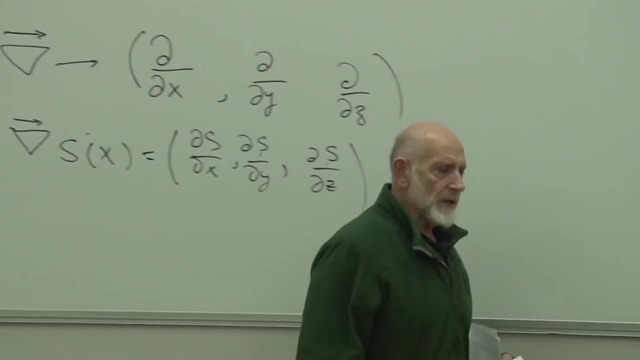 of del on a scalar, And, incidentally, we might generalize it, and so there's no reason why we're talking about temperature. We could be talking about any scalar, and so let's just call it a scalar f, S-s-s-s. Yeah, I said that there are no scalars that are easily observed, That's. 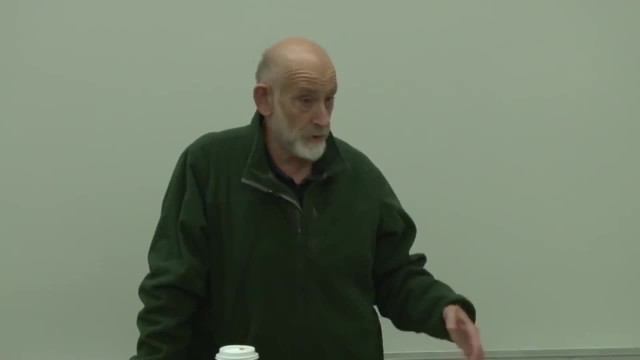 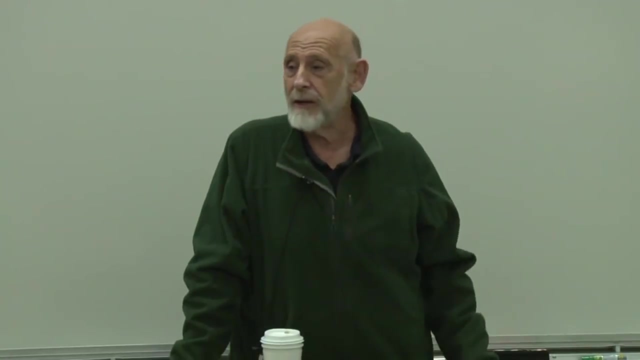 not quite true. I'll give you an example of a scalar which can be observed. It's a scalar which is made out of the electric field. Can you make a scalar out of the electric field? What would you do to the electric field? 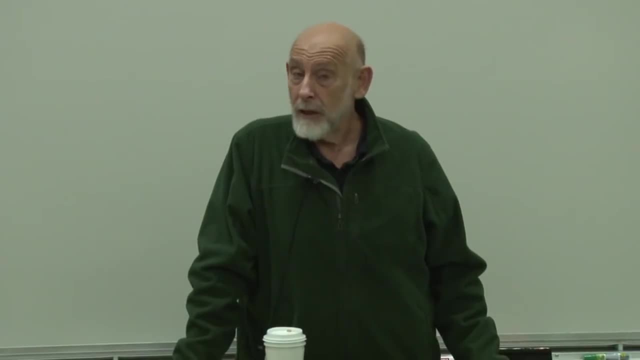 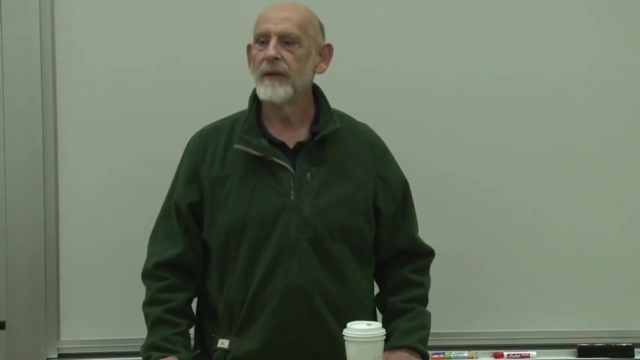 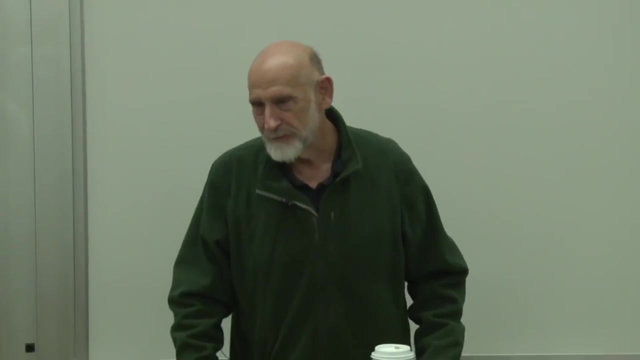 field to make a scalar out of it, Integrated. I was thinking of I'm not sure why integrating a vector would give a scalar. so Reverse the gradient operation. Oh, oh, I see what you mean. You mean construct the potential. Yeah, that would be one construction. 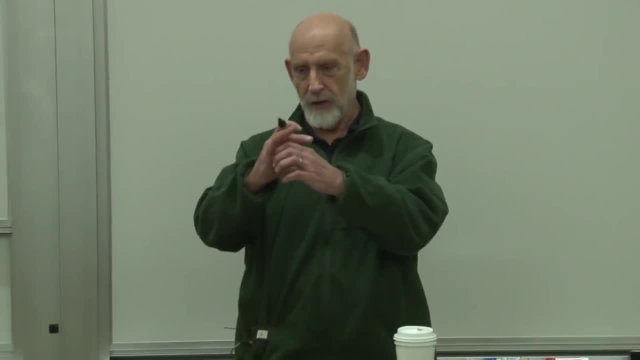 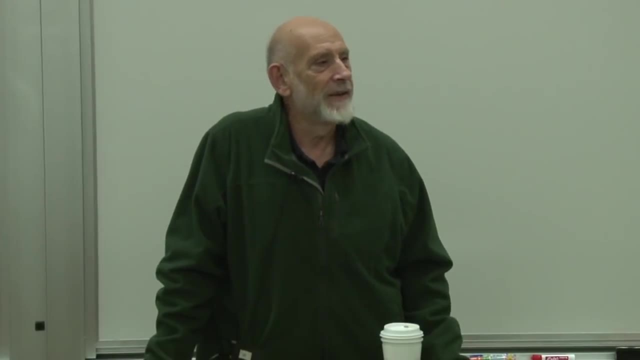 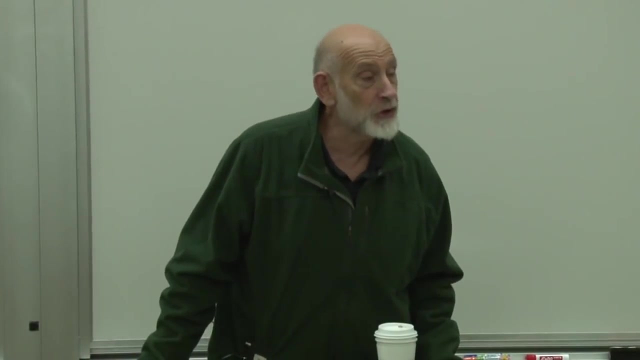 How about a local construction where you can get the answer only by looking within a small region? Yeah, this is a very simple answer: Use what is it? How about taking the inner product with itself, Namely just the square of the electric field, the square of the magnitude of the electric field? 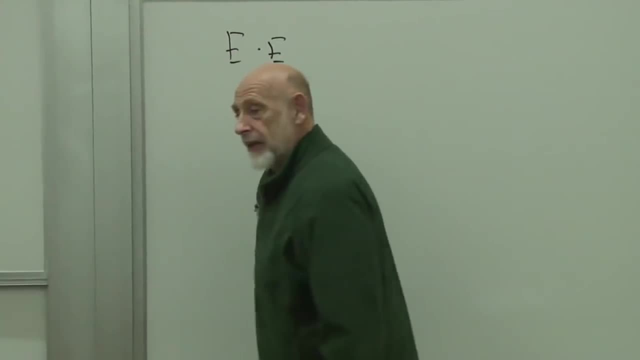 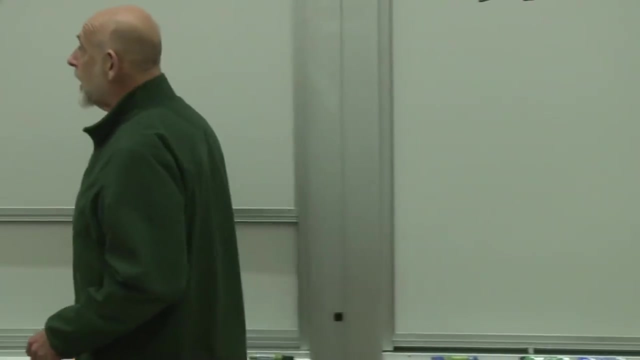 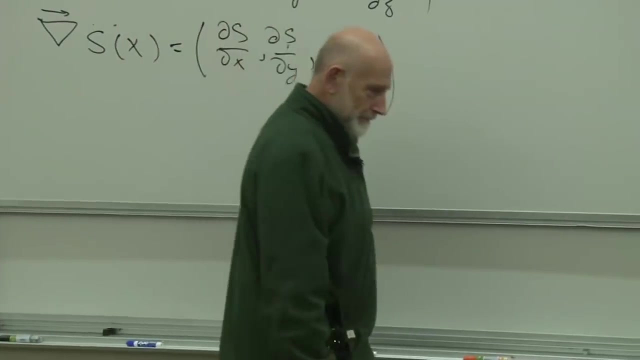 Electric field dot. electric field: X component squared plus Y component squared, plus Z component squared. That happens to be a scalar. The scalar could be anything. It could be a scalar that 's made by squaring some other vector. it could be any scalar, as long as it's a scalar. 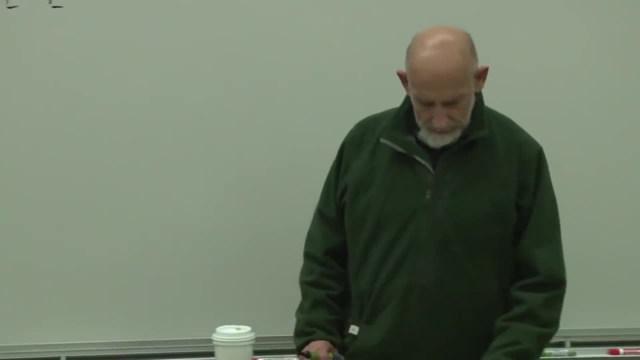 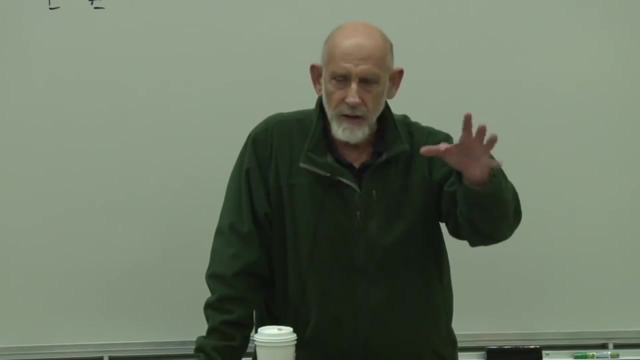 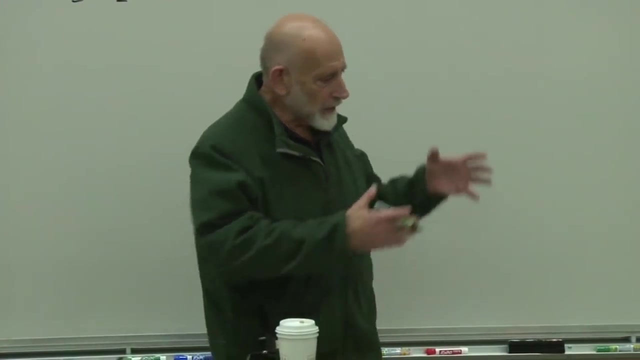 Incidentally, there's more to saying it thinks it's a scalar than just that it has one component. It means something in addition. It means that whatever direction you look at it from, it always has the same value. okay, If you look at the temperature from the north, the temperature 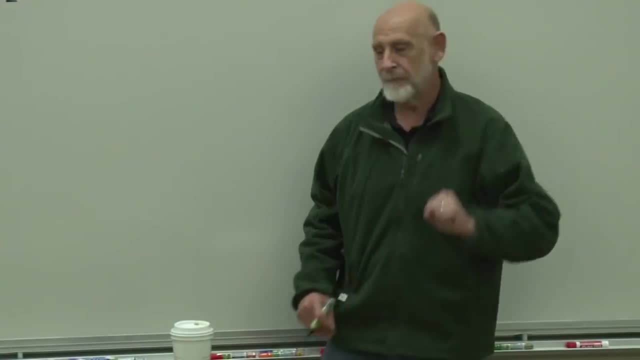 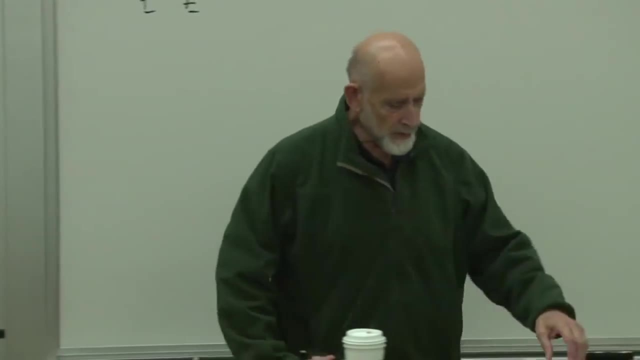 over here. you get the same answer as if you look at it from the south or whatever. It doesn't have an. OK, I'm sorry, But it doesn't really matter, right? So it's. it hasn't really orientation, it's simply a scalar. Okay, so here's what you can do with a. 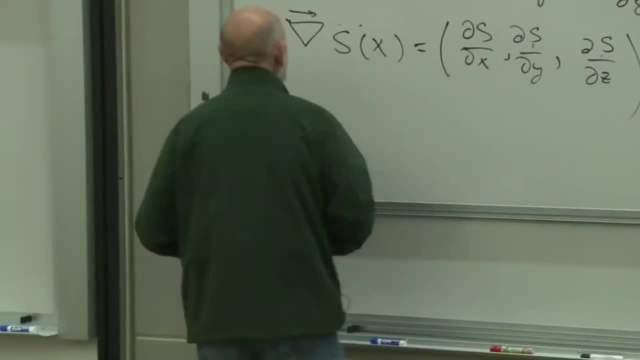 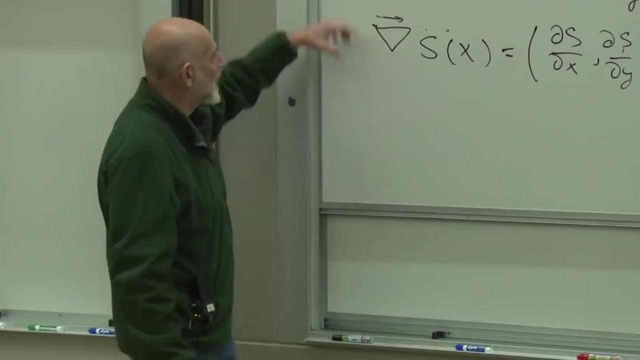 scalar by applying the del symbol to it. The scalar has no directionality. the del symbol can be thought of as being a vector in some fictitious sense, but the product of del with s, you can think of it formally as the product of two vectors. 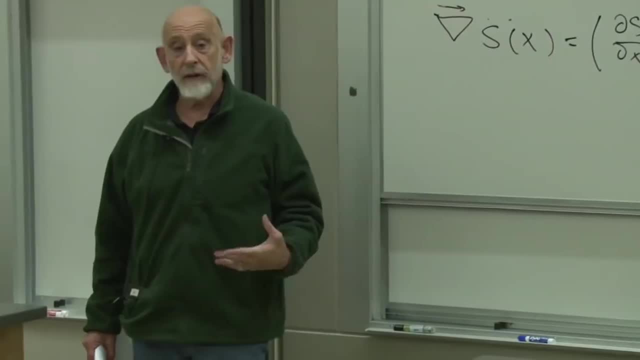 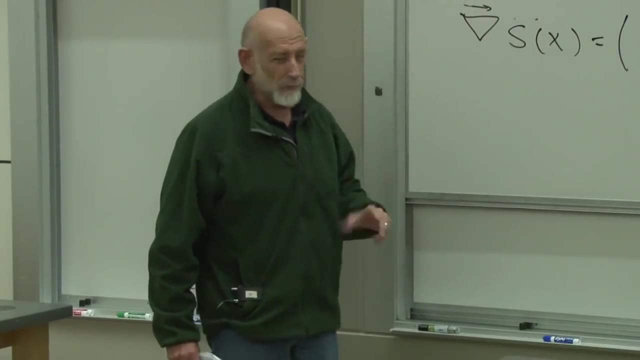 as a product of a vector and a scalar. What do you get when you multiply a vector by a scalar? A vector, Okay. so when you multiply del by s, you're not really multiplying, you're acting with del on s, you get a vector, Okay, what? 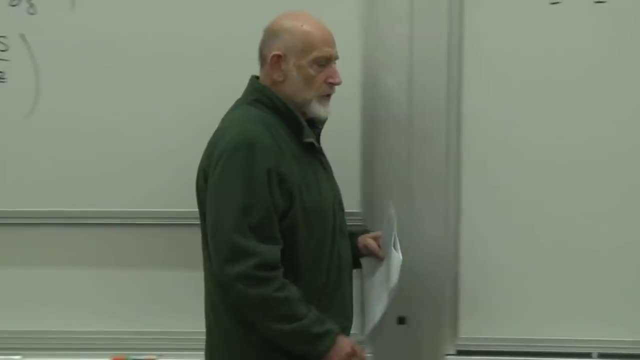 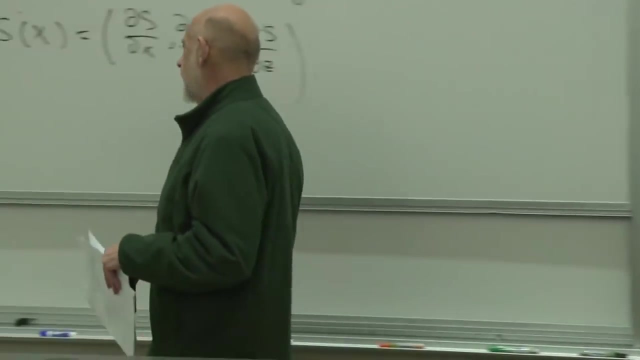 happens? if you apply del to a vector, What can you make? Well, the first thing you can make is a scalar. Again, if you think of del as a fictitious vector and you have another fictitious vector, let's call it A. 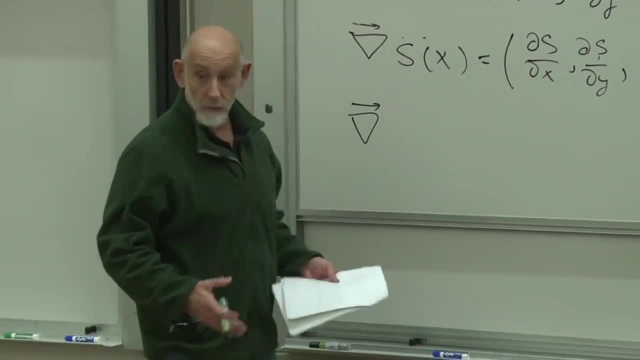 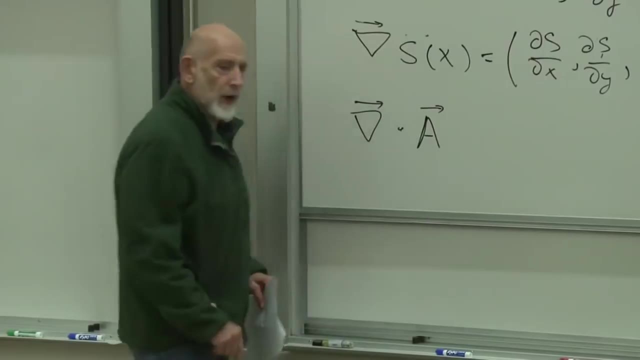 Is del a vector, A vector, And there's a second, fictitious, second, real vector, I'm sorry, a real vector field called A. One thing you can do is take the dot product between them. If this was a real vector, then this would make sense. And what would it? what would? 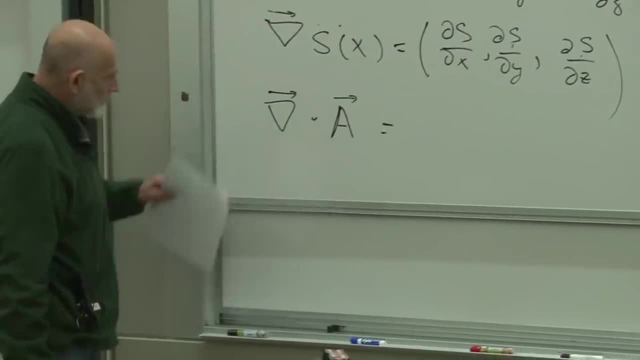 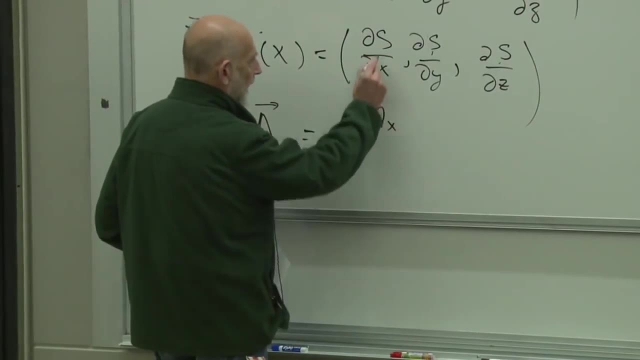 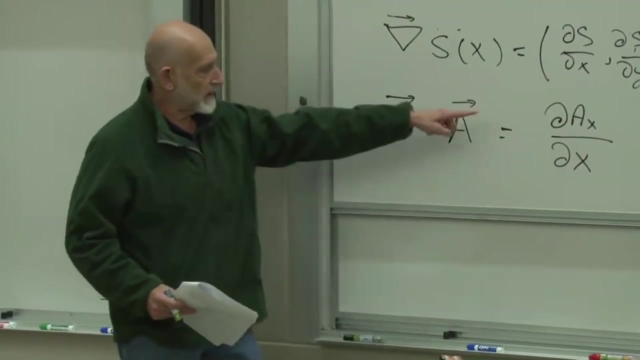 the sense be It would be: you take the x component of del, multiply it by the x component of A That is replaced by the derivative of A, x with respect to x. You take the x component of del, that's d by dx, and you multiply it by the x. 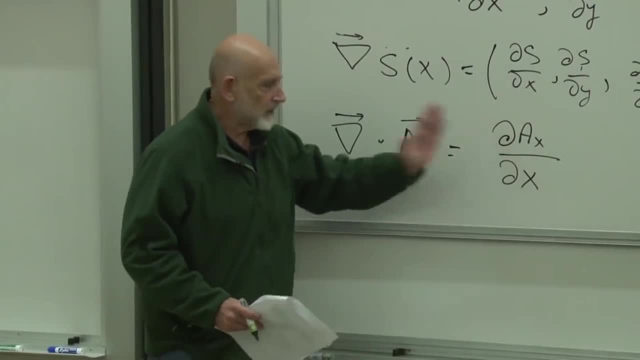 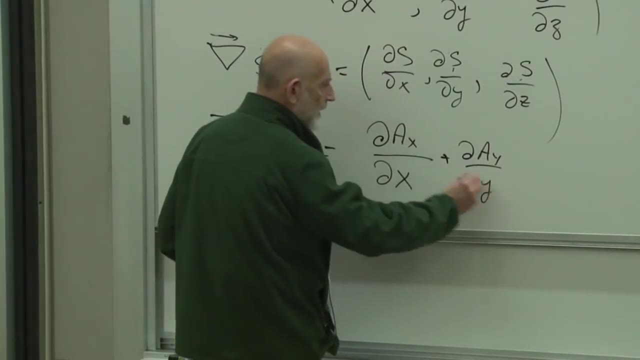 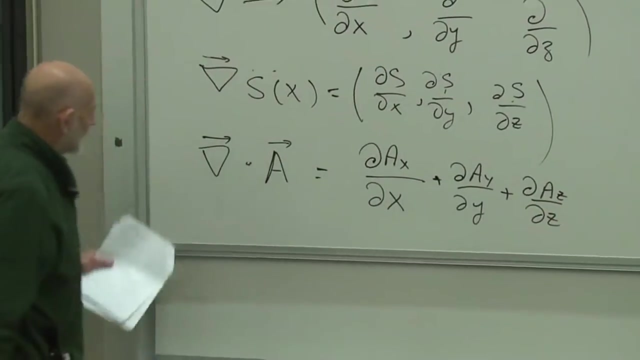 component of A. you don't really multiply, you act right. But then you add Derivative of Ay with respect to y plus the derivative of Az with respect to z, and that's the dot product of del and A and it's called the divergence. It's a scalar. whenever you're. 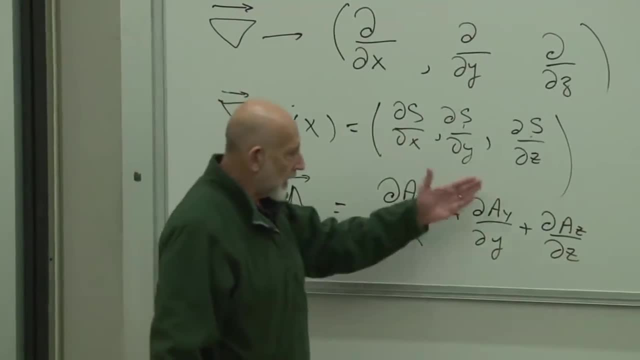 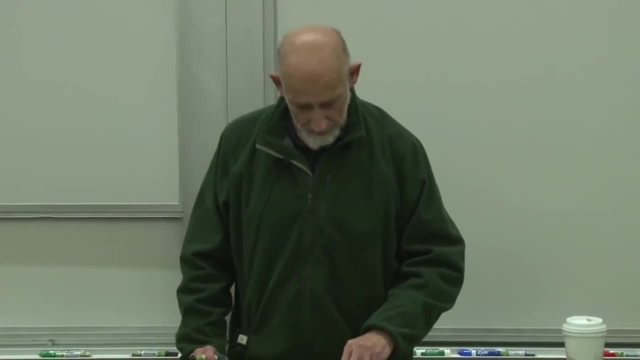 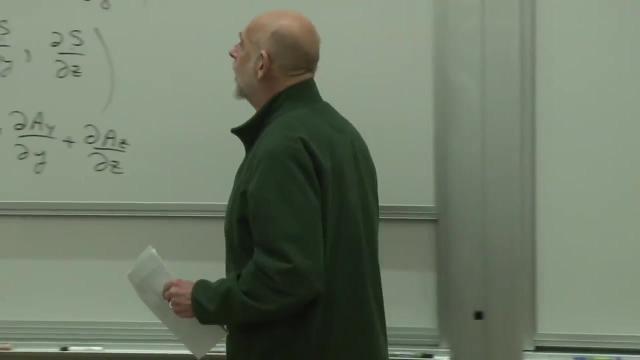 you take the dot product between two vectors, you get a scalar and that scalar is the divergence of the vector A. We've talked about the divergence before, but now we're spelling it out again in some detail. Okay, next Let's talk about cross products. First, before we take the cross product of 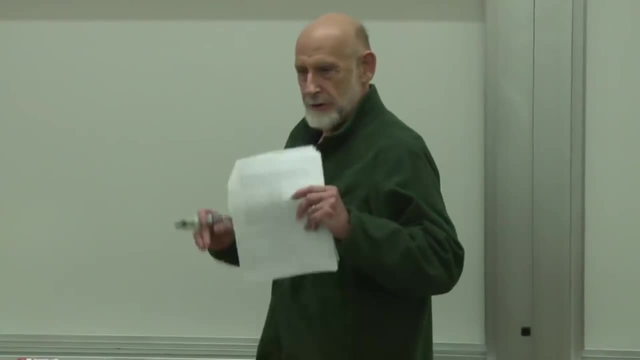 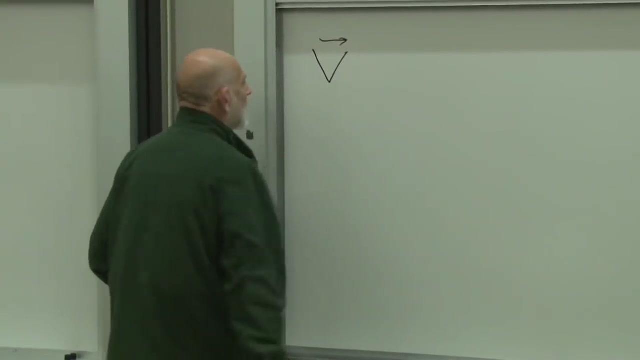 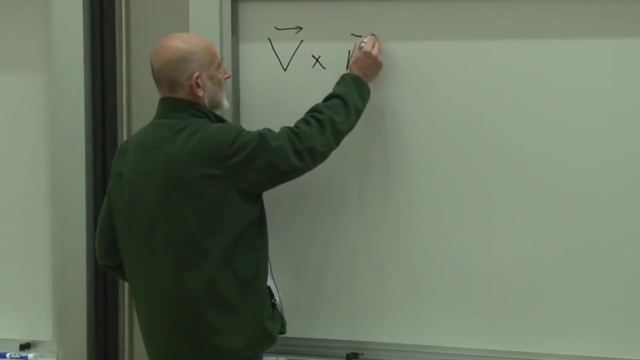 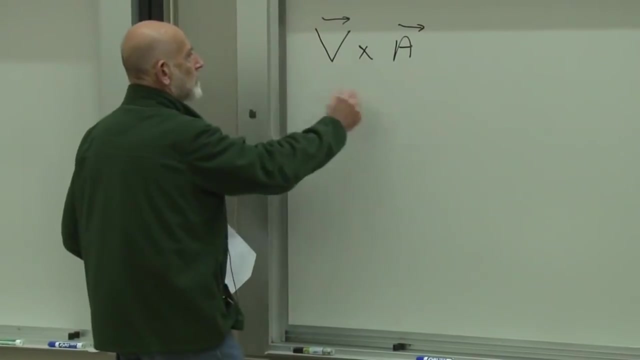 del with something. let's just talk about cross products in general. Let's suppose we have a vector v and we take the cross product of vector v with vector A. That's the standard cross product. It has a set of components. Let's write the components down First of. 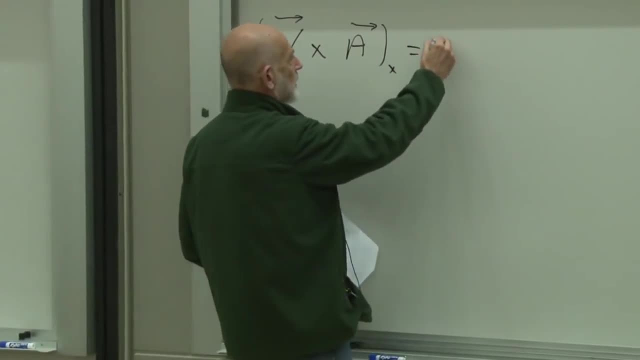 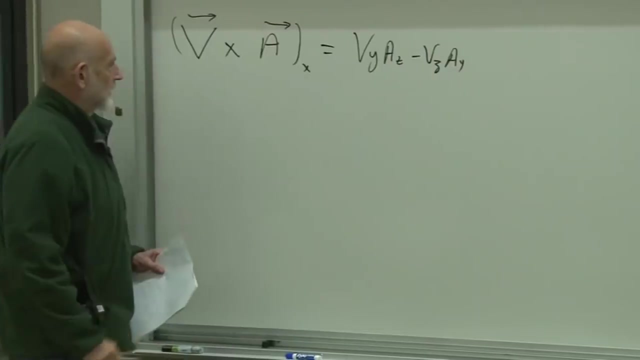 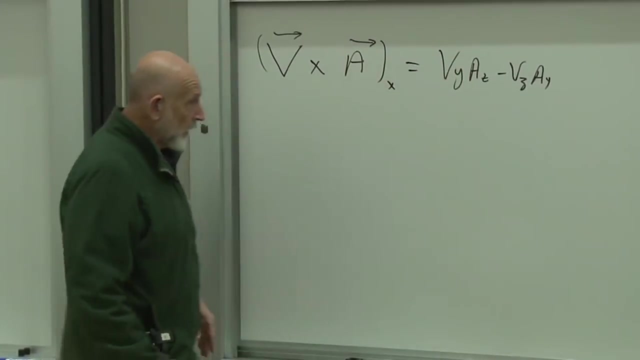 all, there's the x component, and the x component is the delta Right component is equal to VyAz minus VzAy. that's the definition, if you like, of the x component of the cross product of V and A. And now you get all the other components by a rule which: 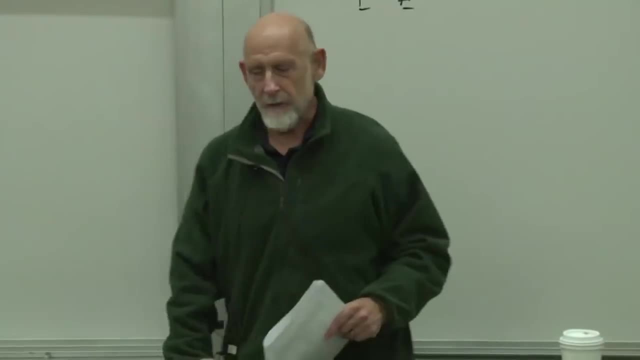 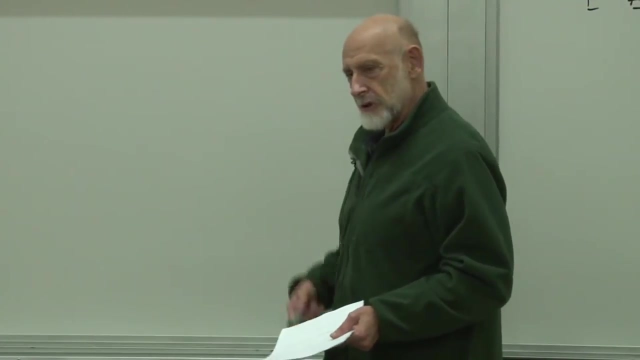 I've emphasized over and over through the years. it's the way I remember it. you only have to remember one of these and the rest you cycle through. You cycle through x to y, y to z, z to x, One to two, two to three, x, y, z. I'm sometimes going to identify as: 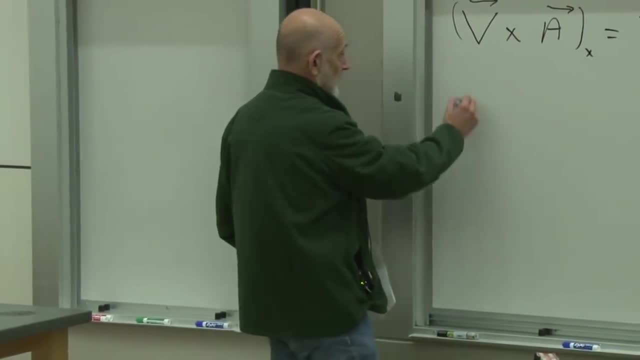 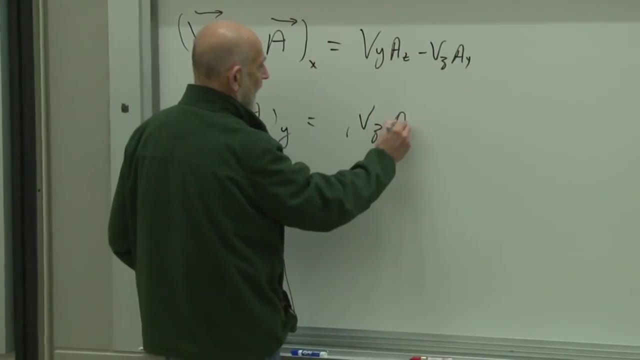 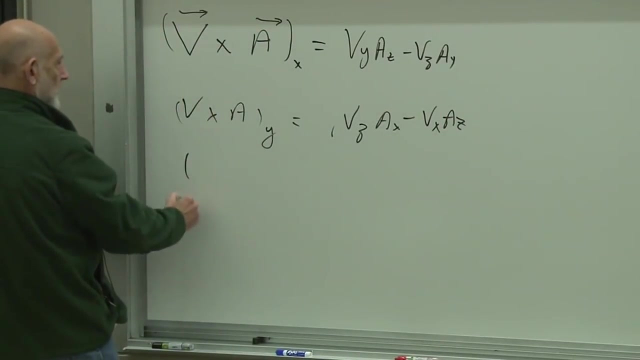 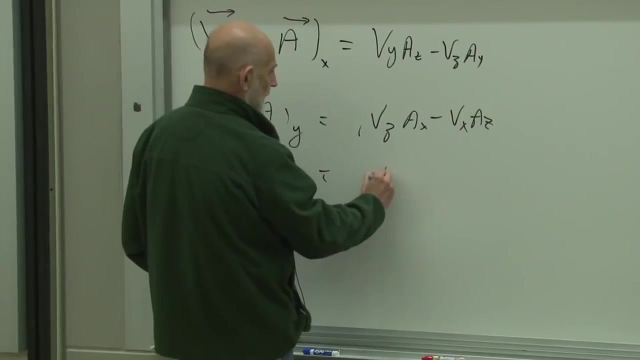 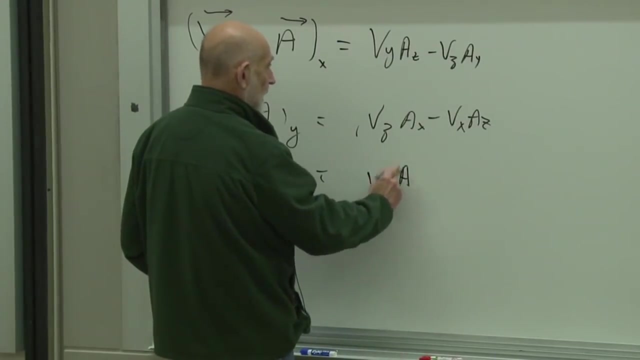 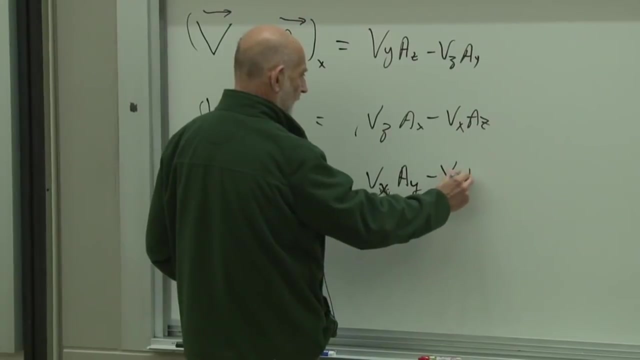 one, two, three. But alright, so the next one would be V cross A. the y component of it is VzAx minus VxAz. And likewise for the last component, V cross A, the z component is two, I Vz, sorry, VyZx Ay minus Vyax. Alright, those are the three components of the cross. 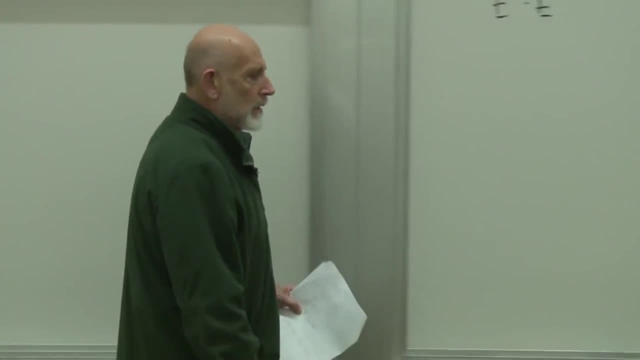 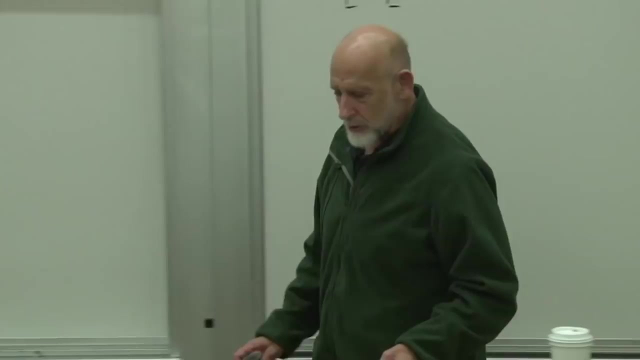 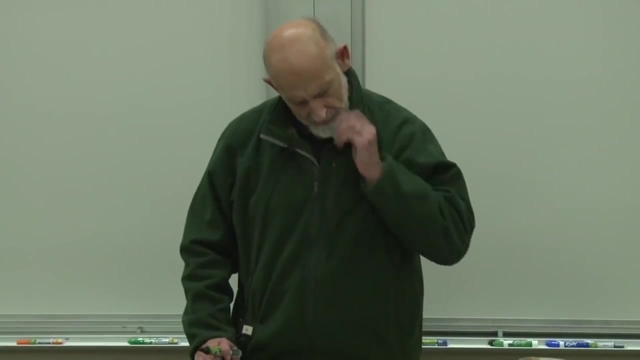 product. I assume you're all familiar with them. What you may or may not be familiar with is a condensed notation for all of this. A condensed notation using a symbol called the Levy-Civita symbol- Levy-Civita, I assume, was an Italian mathematician. 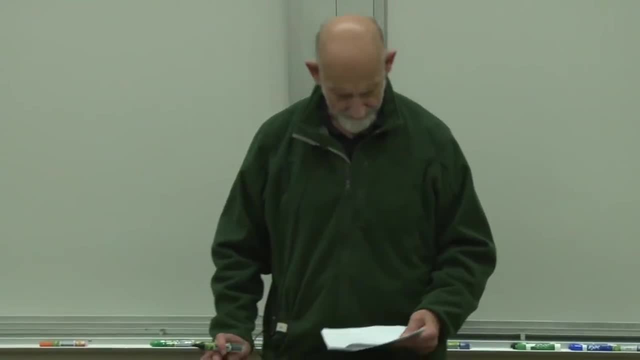 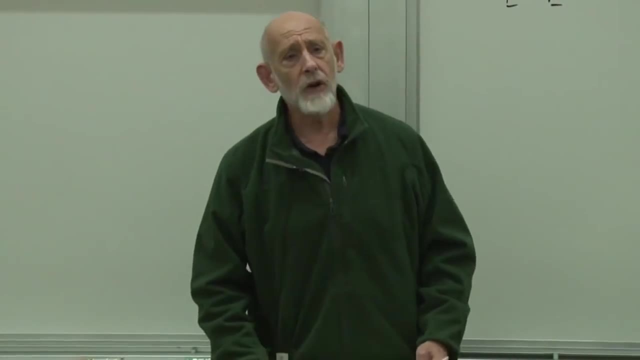 presumably a Jewish-Italian mathematician with a name like Levy, but I don't know really- And he invented a symbol. He did other things too, besides inventing a single symbol. So did Kronecker. Both Kronecker and Levy-Civita invented symbols, and that's what they're. 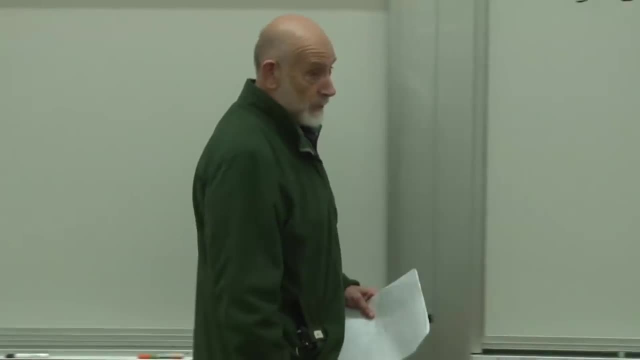 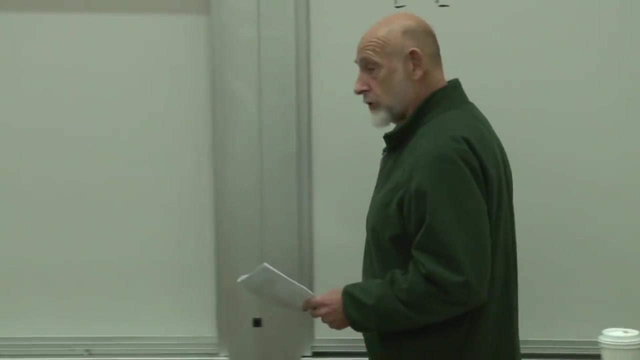 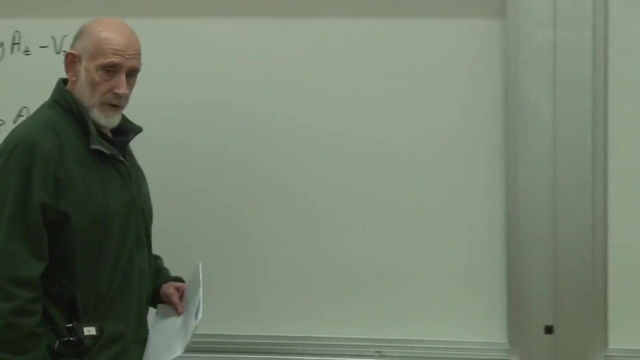 most famous for these very simple, it's true, these very simple symbols, but both of them had a long history of contributions to mathematics. Let me just remind you about first the Kronecker symbol, the Kronecker delta, delta ij. Delta ij is a number, is a. 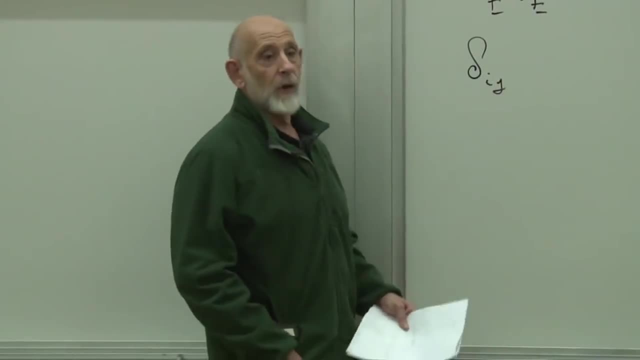 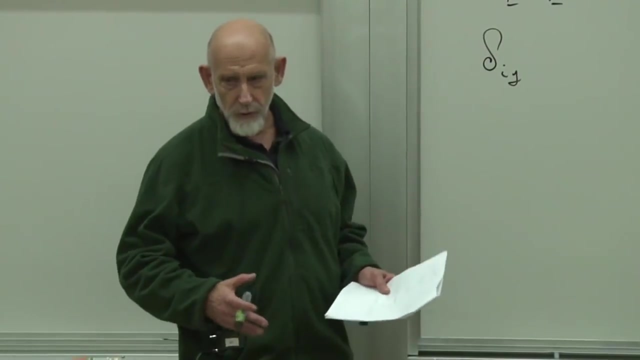 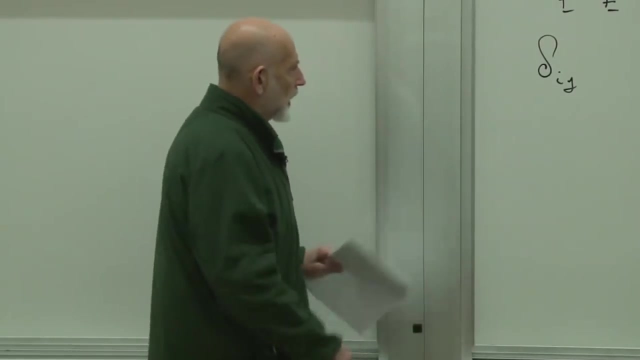 takes on a value for i and j equal one, two or three or equivalently x, y and z. Whenever I use the notation one, two and three for three-dimensional coordinates, it's always one. It's synonymous with x, y and z. The delta ij. we know what that is, that's just. 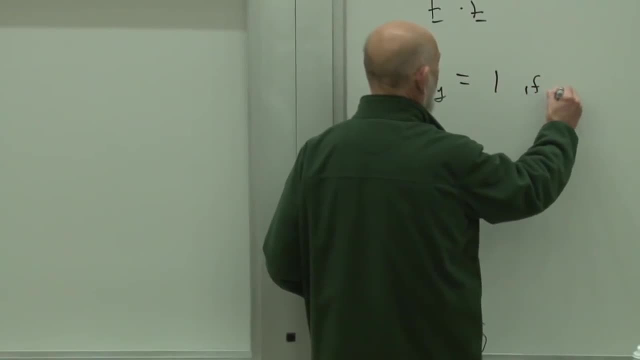 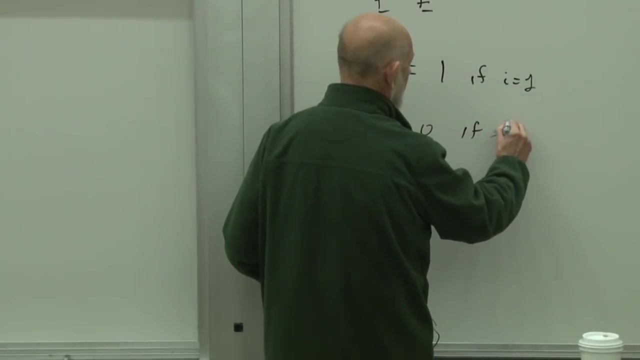 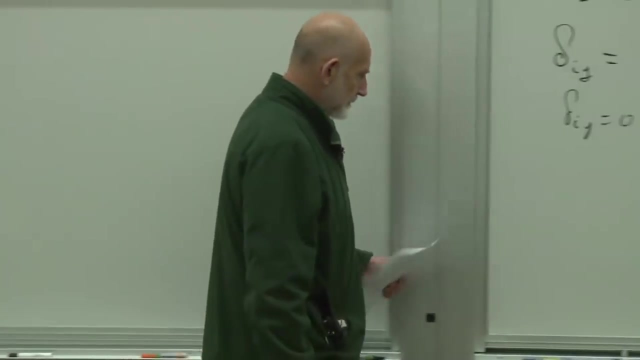 either zero or one. It's one if i equals j and it is zero if i not equal to j. All right, that's Kronecker's symbol and it's very useful. Okay, The Levy-Civita symbol has three indices. 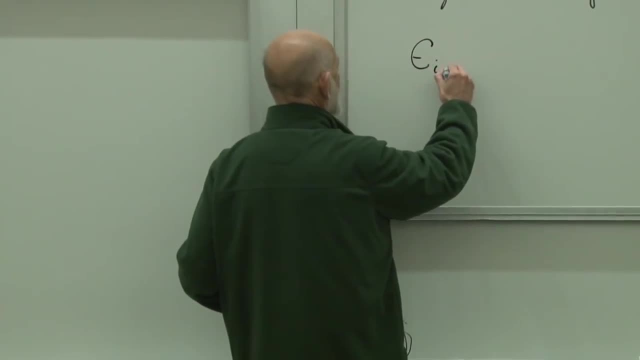 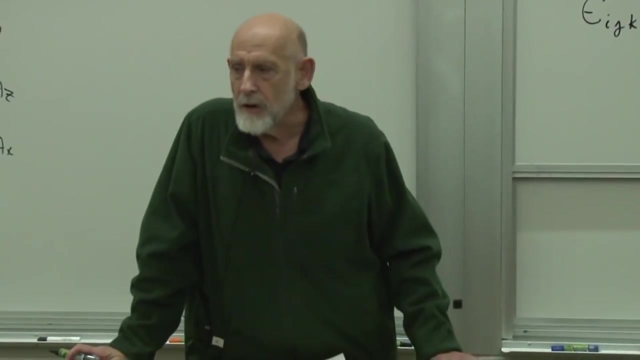 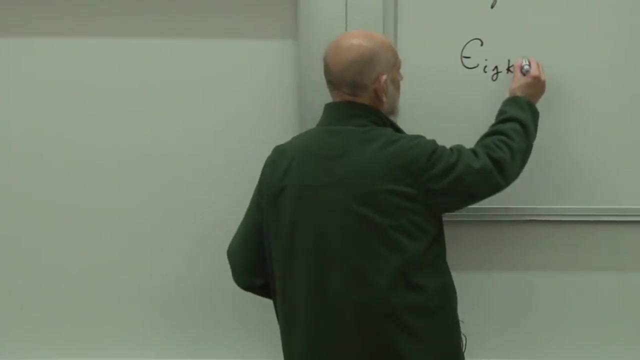 and it's called epsilon, Epsilon ij, J, k. The values that epsilon takes on are either zero, one or minus one, depending on the following. First of all, it's zero. if any, I don't want to write, shall I write? 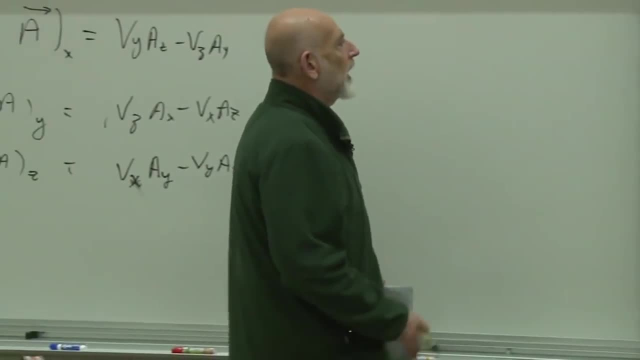 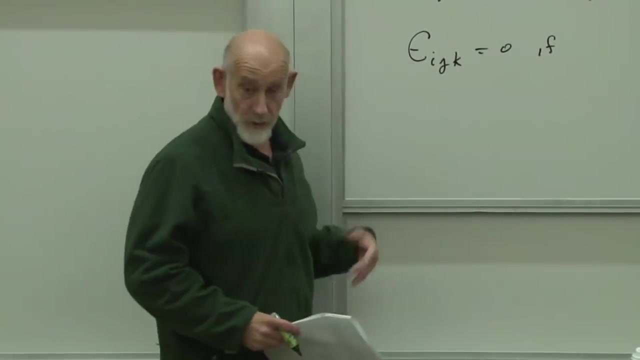 this. No, I'm tired of writing. It's zero if any two of the indices are the same. All three of them are the same is a special case. All three of them. it could be epsilon 1, 1, 1, or epsilon 2, 2, 2, they're all zero. 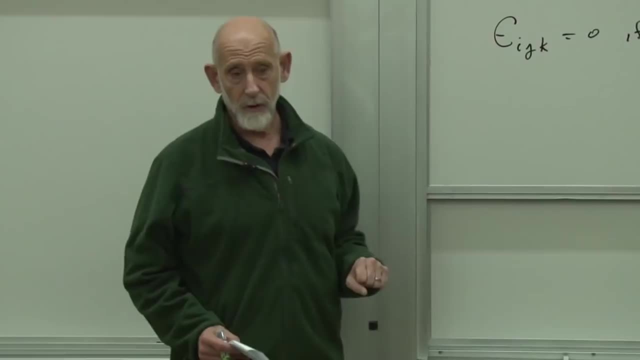 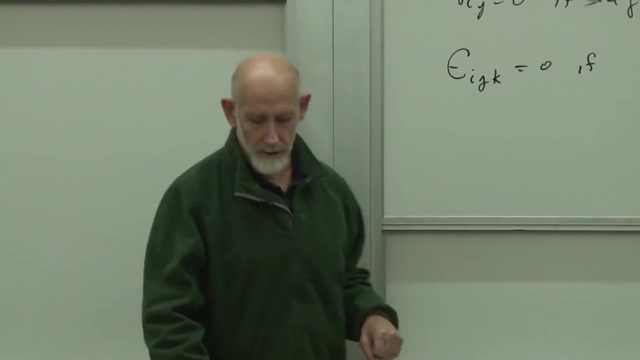 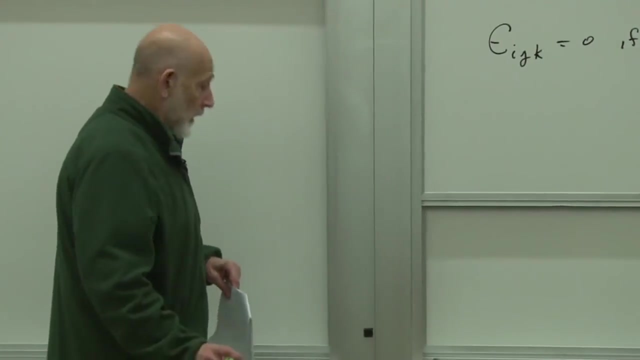 But so is epsilon 1, 2.. Sorry, epsilon 1, 1, 2.. Epsilon 1, 1, 2 is also zero, so if any pair of them are the same, the epsilon symbol is zero. The only time when it's not zero is: 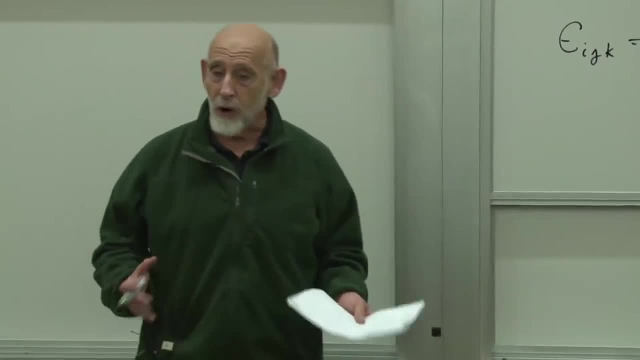 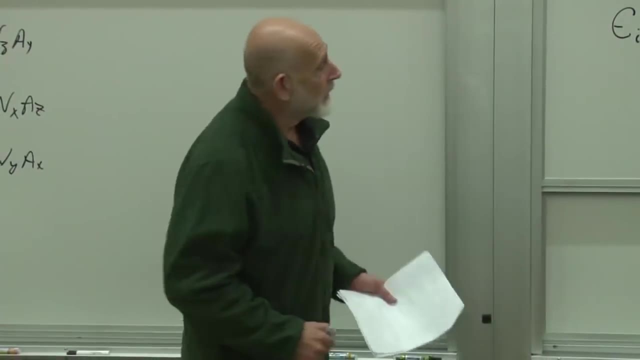 when all three indices are different. Now, what can they be If they're all different? they have to be one, Two and three, But they could also be three, two and one, Or two, three and one All. 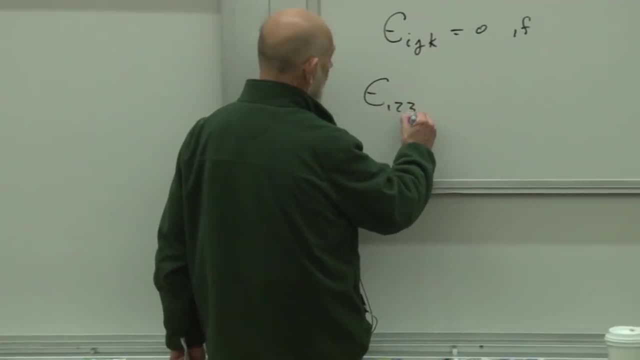 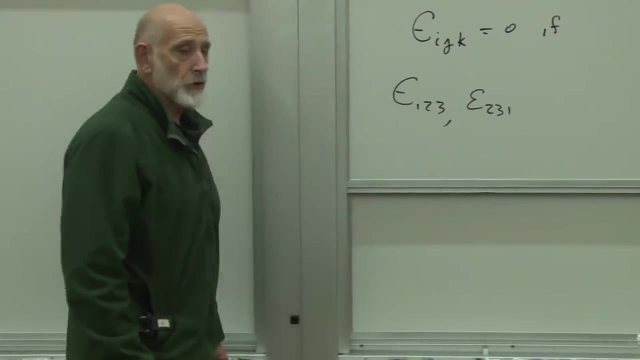 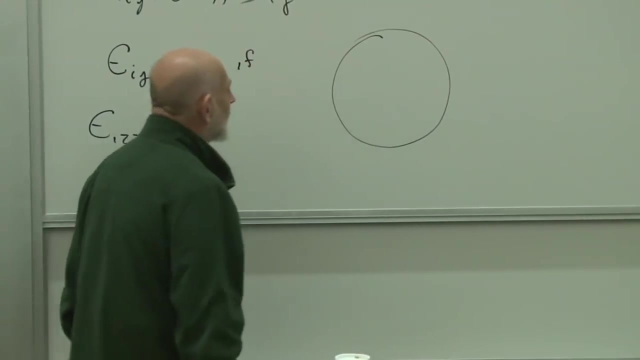 of those: epsilon 1,, 2,, 3, epsilon 2,, 3, 1,. they're all either equal to plus or minus one, according to the following rule: Draw yourself a clock And on the clock there. 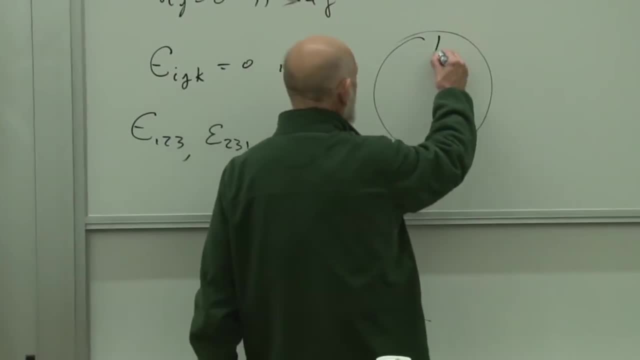 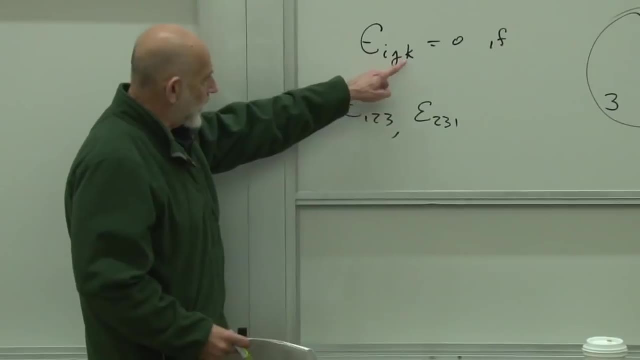 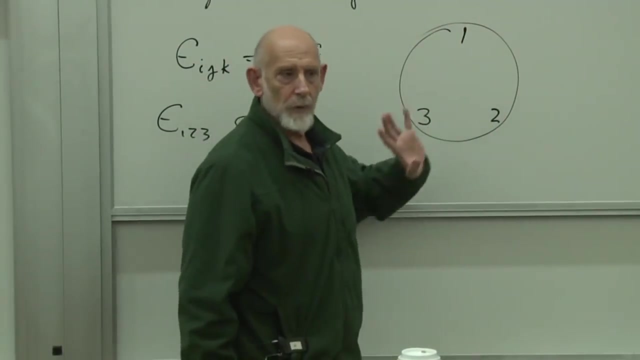 are three hours on this clock Hour: one hour two and hour three. Okay, If the sequence i, j and k, in this case one, two and three, corresponds to a clockwise per – let's call it permutation – if it corresponds to a clockwise permutation, 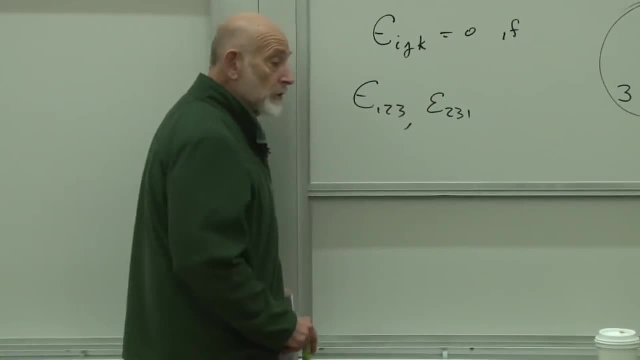 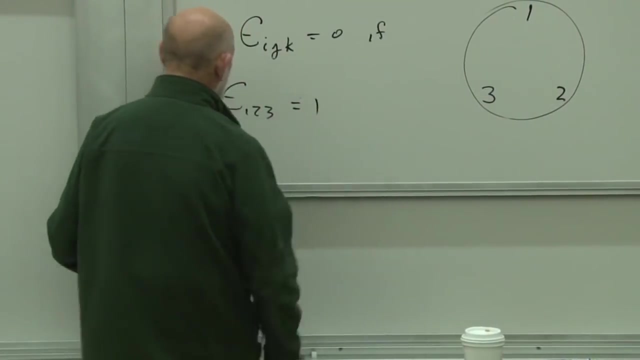 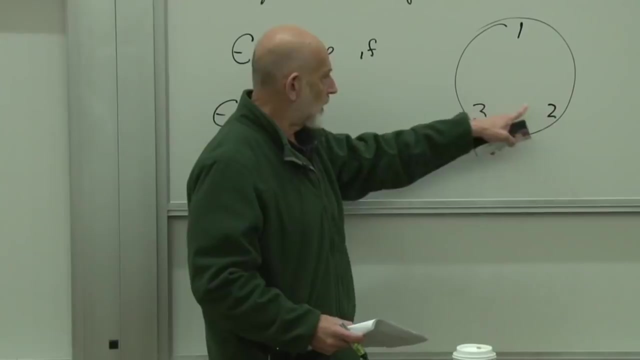 then the epsilon symbol is one. So epsilon 1,, 2, 3 is equal to one. Likewise epsilon 2,, 3, 1.. Start with 2, go to 3, go to 1.. That's also clockwise, That's also 1.. 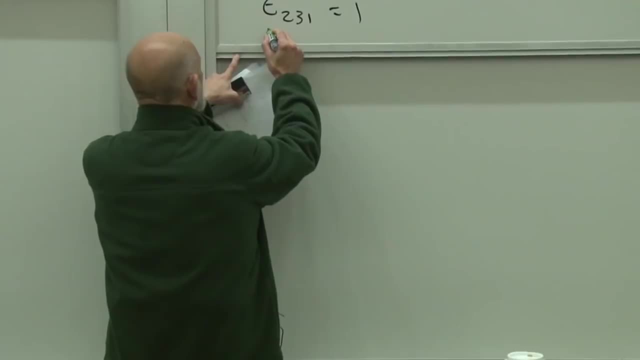 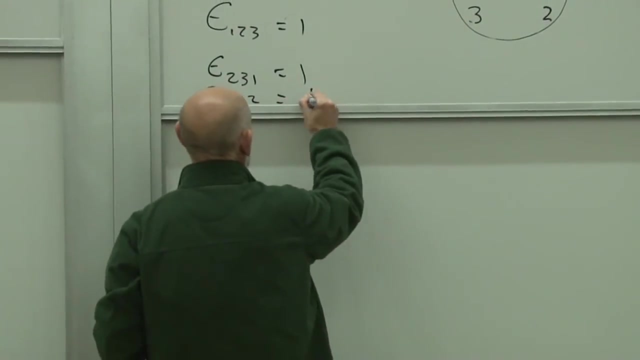 And there's a third one. What's the third one? Epsilon: 3, 1, 2.. 3, 1, 2 is also equal to 1.. On the other hand, there's epsilon. let's start at 1 and go counterclockwise. 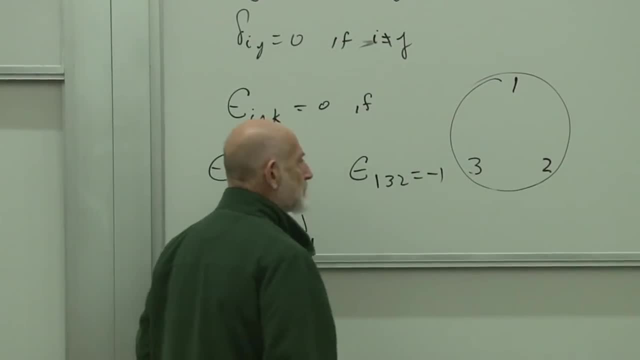 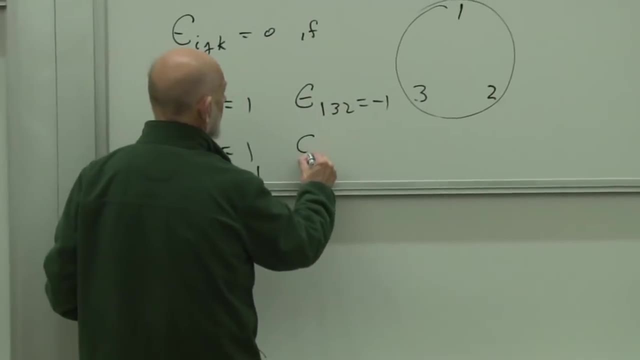 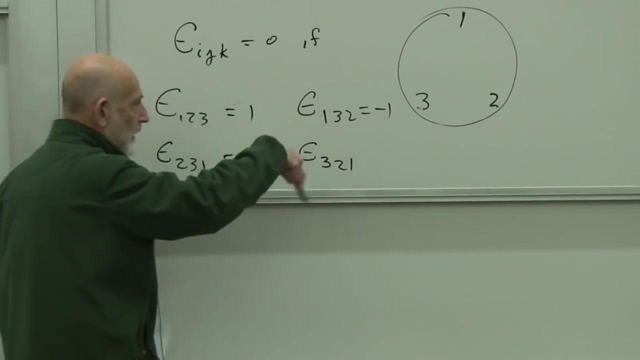 1, 3, 2, that's minus 1.. I think I want to write one more: 1, 2, 3, epsilon, yeah, 3, 2, 1.. That's counterclockwise. That's also equal to minus 1.. 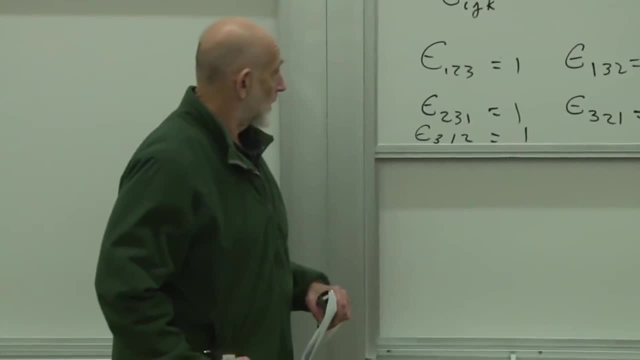 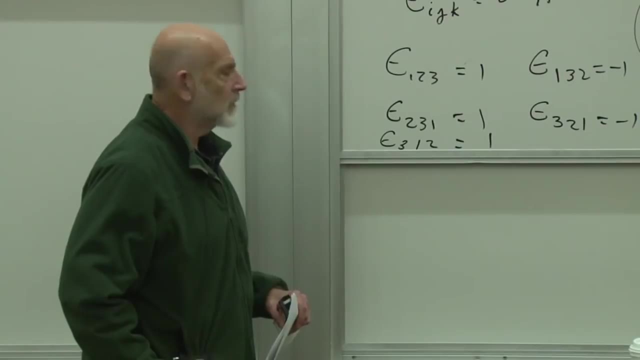 And there's a third one. Is that right? 2, 1, 3.. Yeah, one more: 2, 1, 3.. 2, 1, 3.. Yeah, this is the last one. 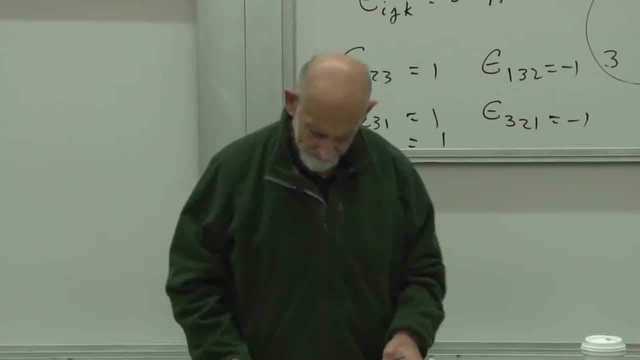 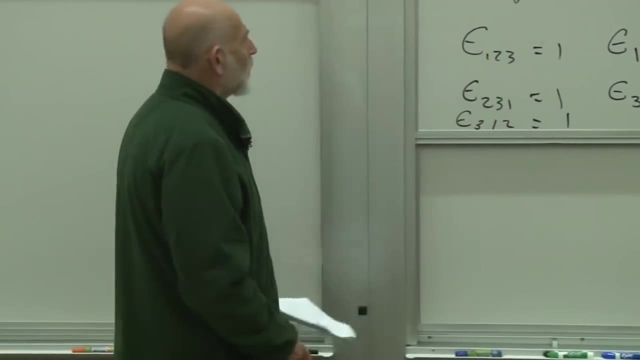 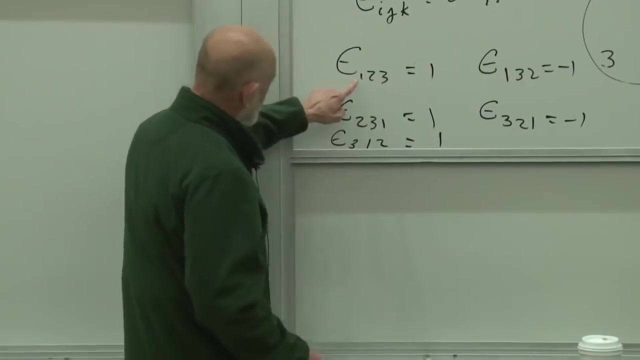 Last one. I just don't have room on the blackboard. That's a useful symbol. Notice some of its properties, or one of its properties anyway: it's anti-symmetric. Anti-symmetric if you interchange any two indices. For example, if you interchange 1 and 2 here, you'll go to epsilon 2, 1, 3.. 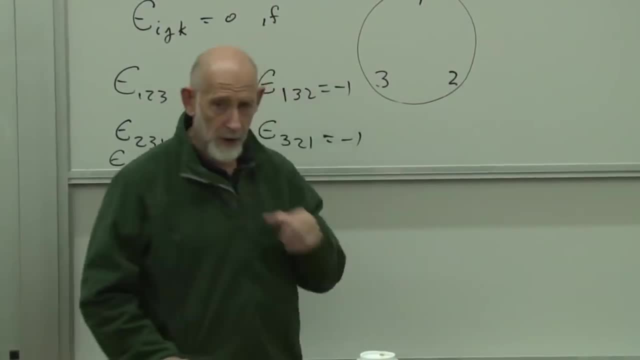 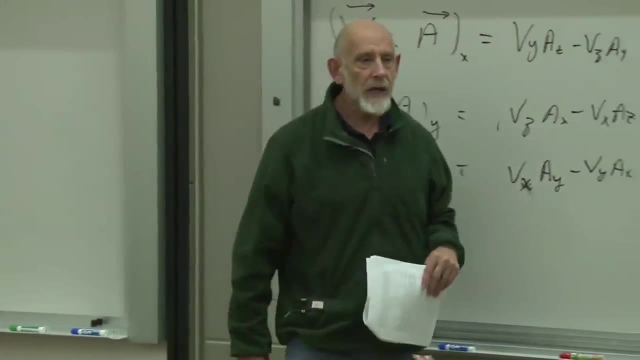 1, 2, 3 is clockwise. 2, 1, 3 is anti-symmetric. 2, 1, 3 is anti-clockwise or counter-clockwise, And so the epsilon symbol is anti-symmetric with respect to the exchange of any two indices. 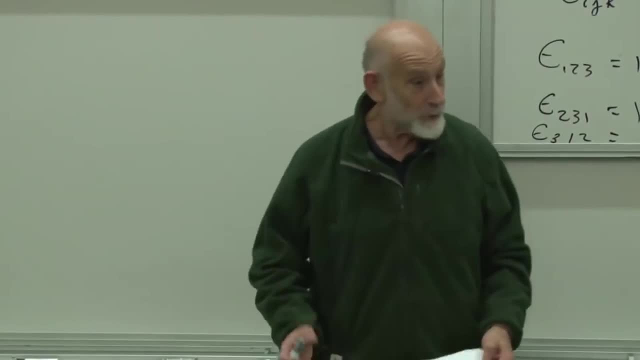 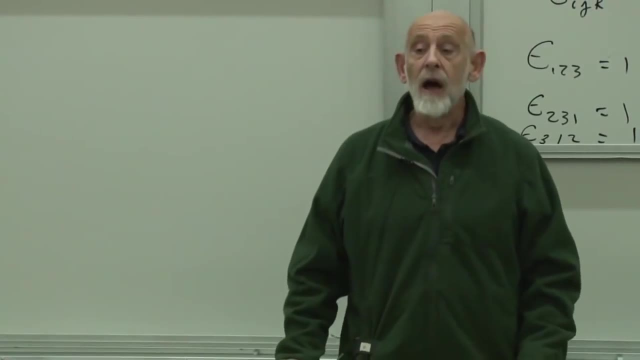 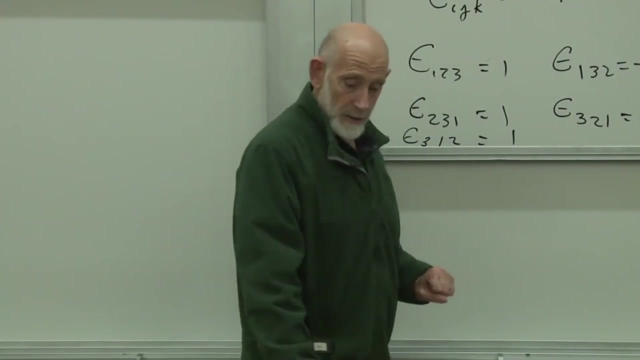 So it's often called the anti-symmetric epsilon symbol, And that, in fact, is enough to completely determine it apart from the magnitude of its entries. Its entries are 1 and minus 1, rather than 2 and minus 2.. 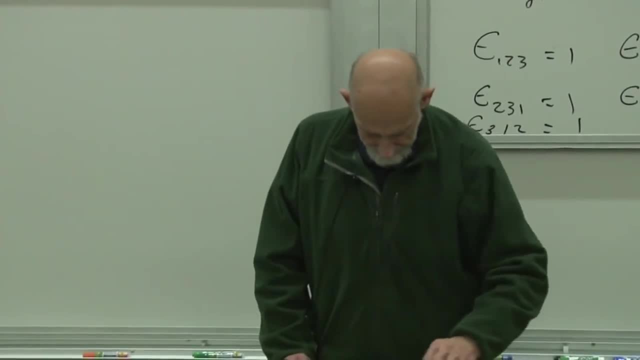 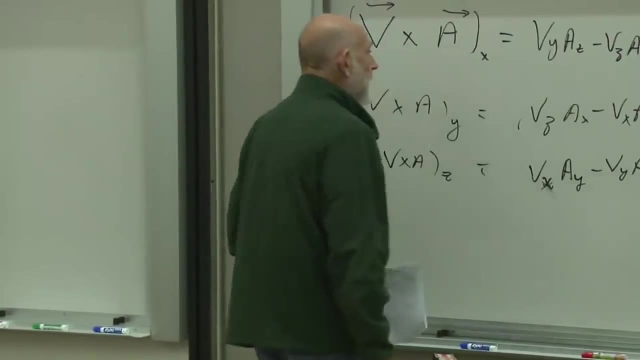 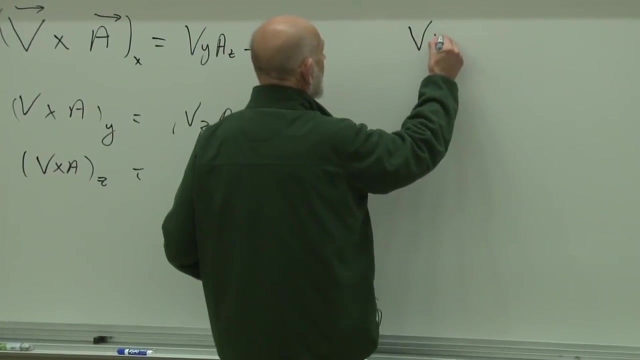 It's the same. this two defines the epsilon symbol. All right, now we can write these equations in the following form, and then we'll check it. All of them can be summarized by v, cross a, the ith component of it. 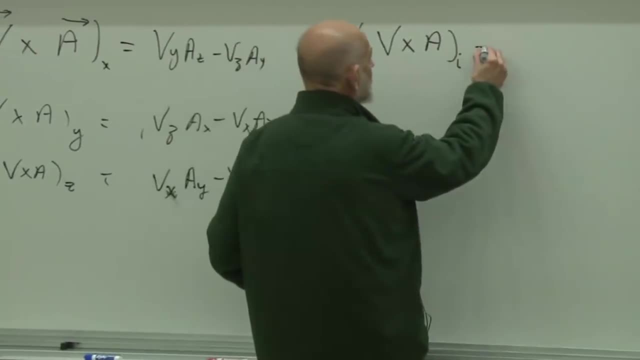 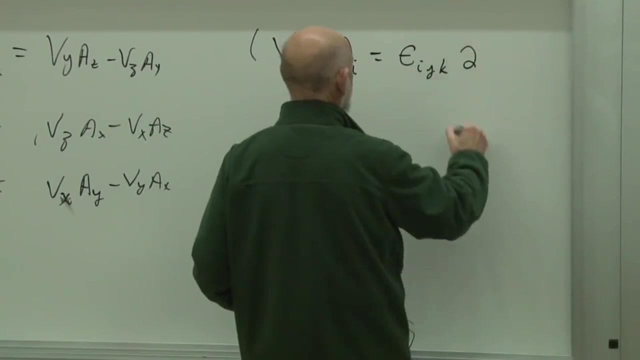 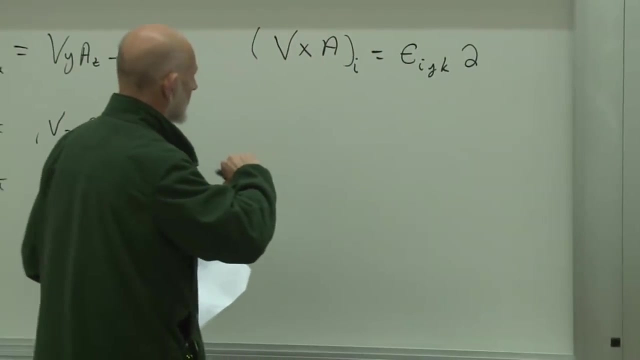 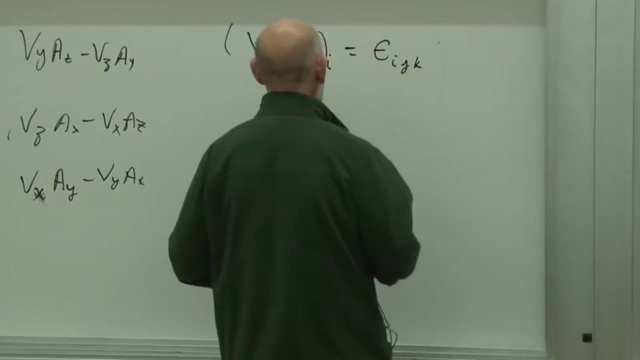 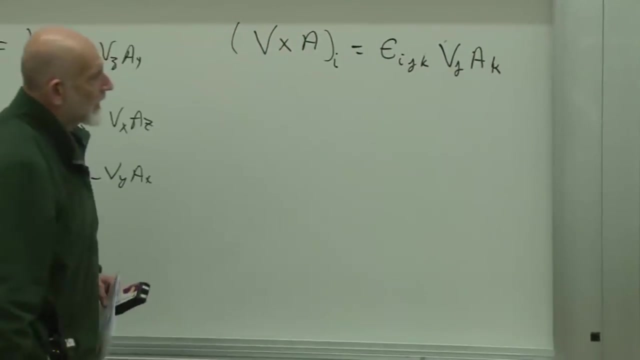 i can be one. two or three is equal to epsilon. i j k. derivative of Sorry, v. no derivative v v sub j, a sub k. There's only one term, but really there's two terms. 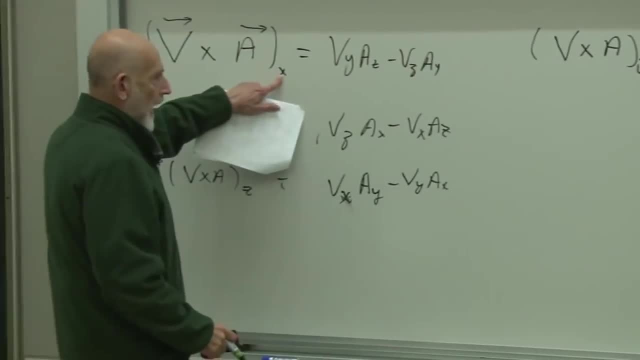 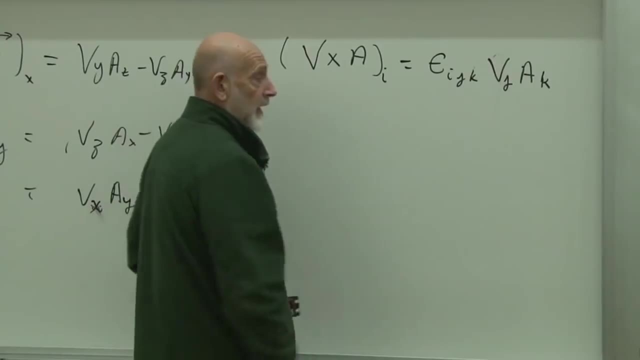 Pick any i. Let's say, let's pick i- equals x. Let's just check this: If i is equal to x, in other words, if i is equal to one, then j and k must not be equal to one. In fact, they must not be equal to each other. 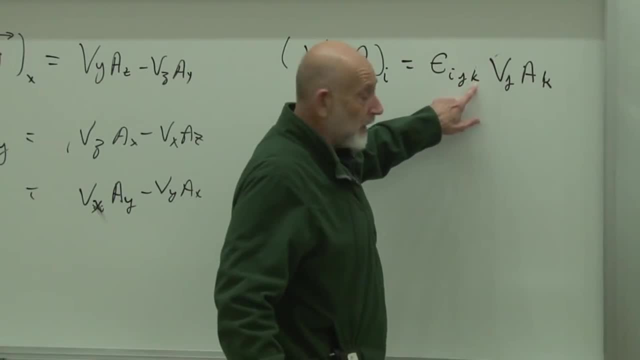 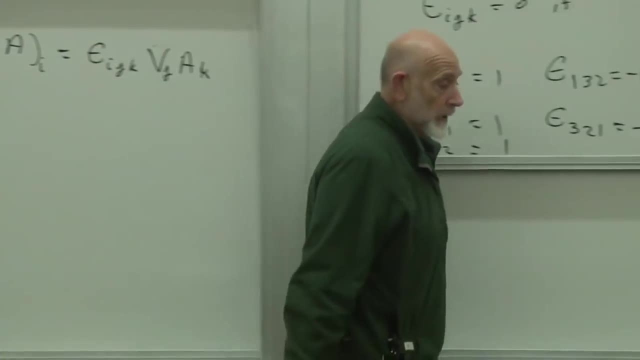 So that means either j is two and k is three, or j is three and k is two. Oh, I am using, incidentally, and I've probably been using. I've been using it all quarter. I've been using the summation convention. 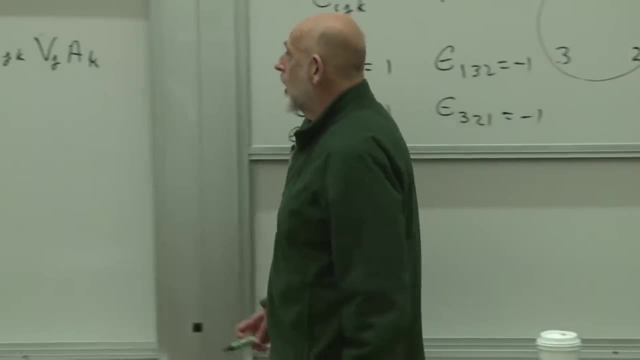 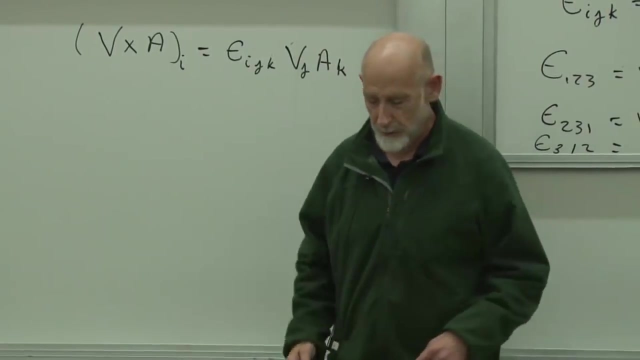 So let me tell you what the summation convention is, just for completeness. Whenever an index is repeated- j with j or k with k- it's summed over. Most of you know that and I will continue to use the summation convention. 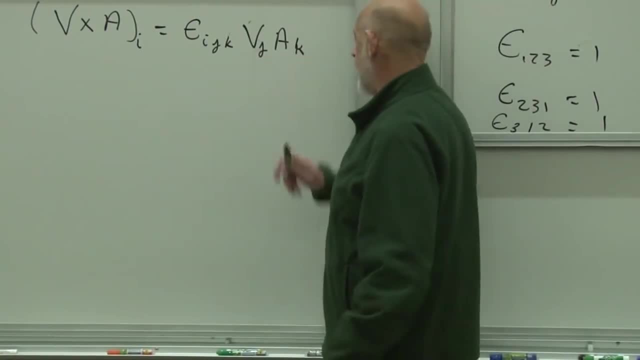 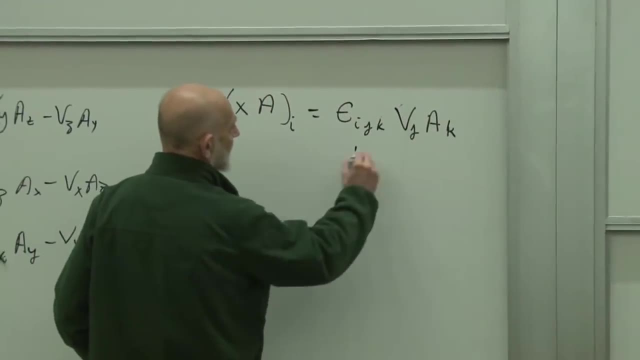 So this literally means sum over j and k, but in this case, if i is one, then there's only two terms. There's only two possibilities: This is two and this is three, or this is three and this is two. So let's see what it says. 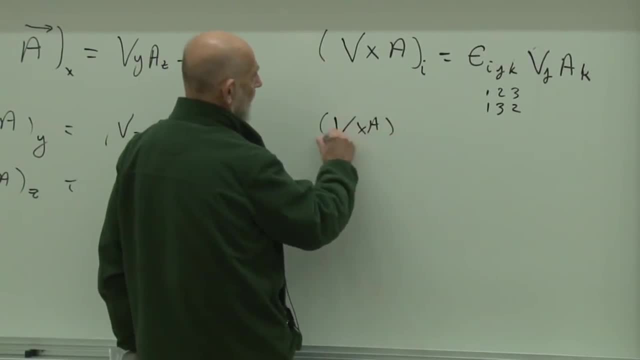 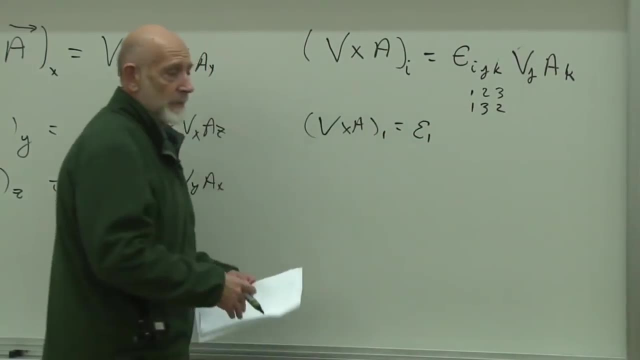 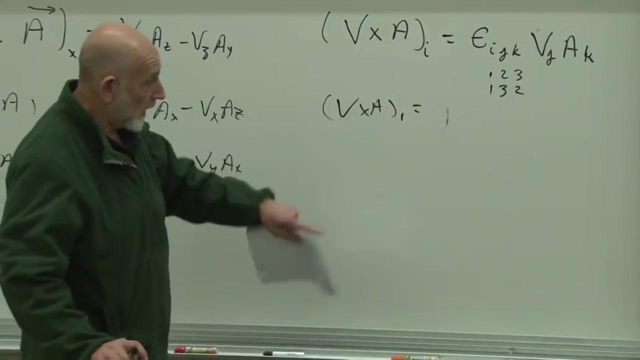 It says that v cross a. the first component of it is equal to epsilon one, then it can be two, three. Let's not write it down: Epsilon one, two, three is one, That's clockwise, And then it will be v two. 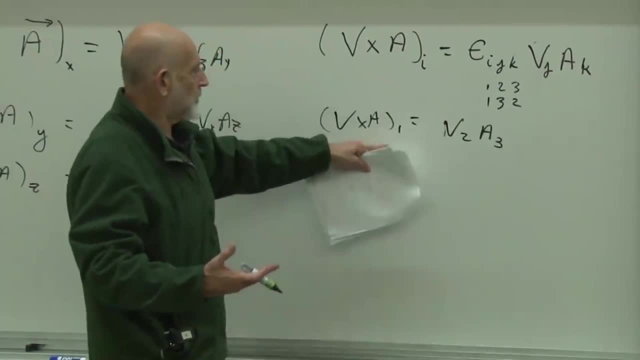 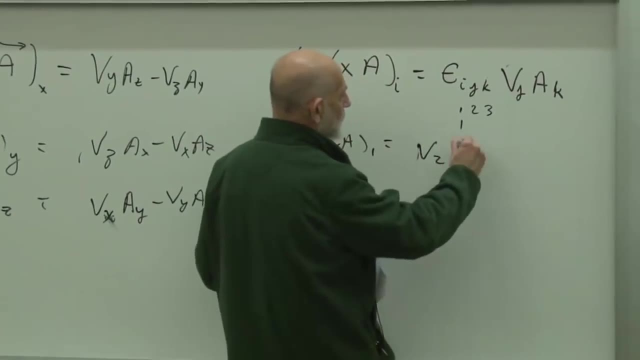 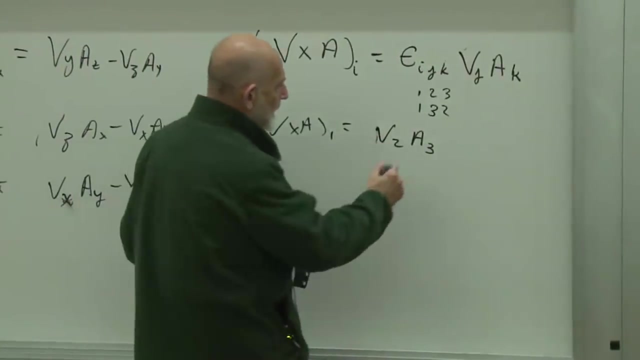 a three or equivalent, or x component, y component, z component. But then there's the other possibility that it's one three two. One three two is counterclockwise, And so epsilon: one three two is minus. 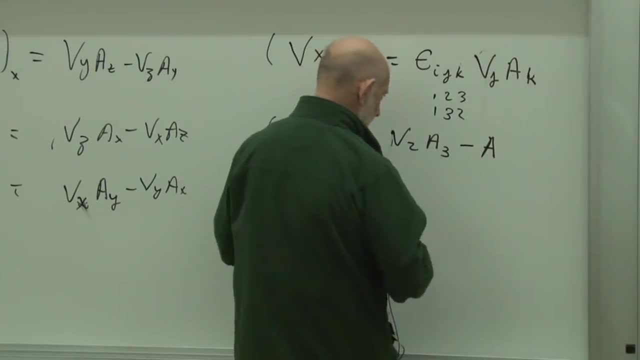 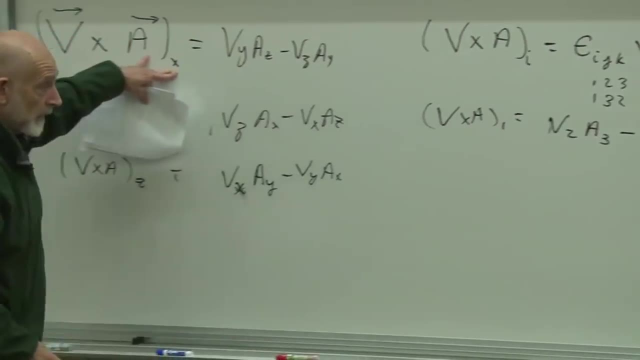 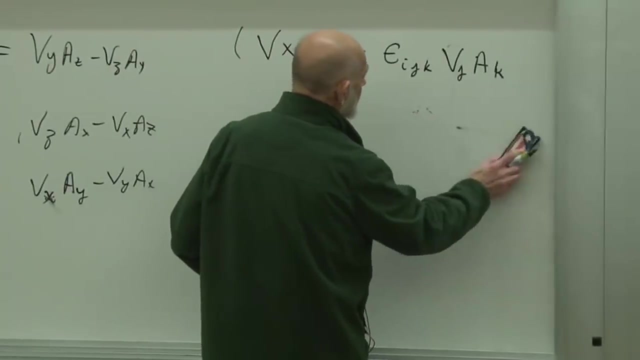 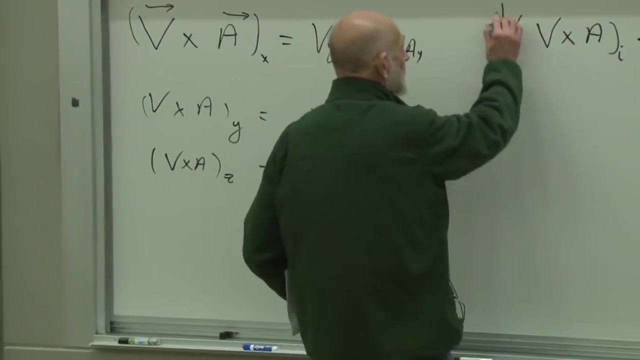 And then that's v three, a two. Well, that's exactly what's written here, And if you go through all of them, you'll see that this is equivalent. This simple expression here is equivalent to the collection of equations here. So this is a definition, if you like. 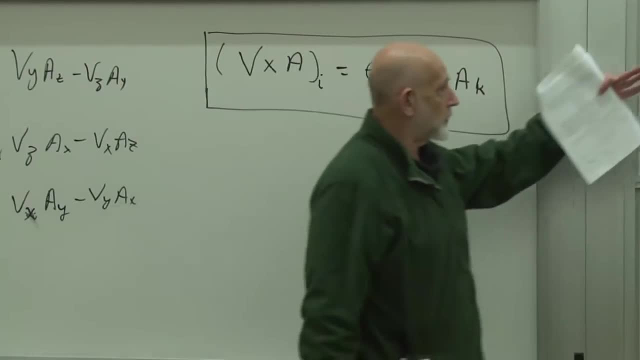 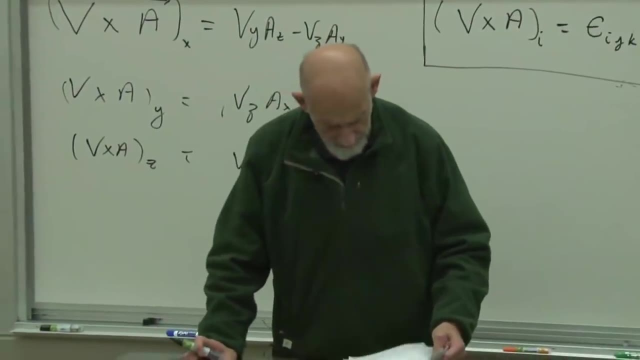 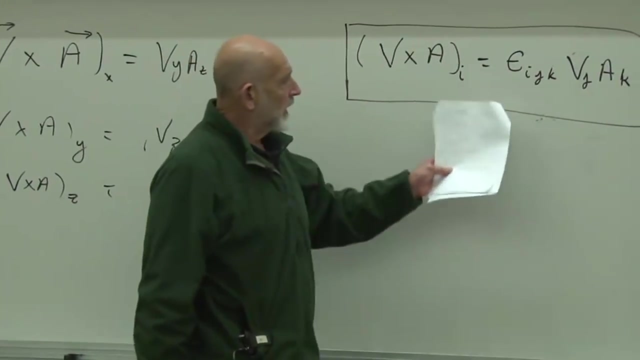 of the cross product. It relies on a definition of the epsilon symbol. but once you know the epsilon symbol, then this becomes the definition of cross product. There's another way you can write it, incidentally, Instead of writing the i component in terms of: 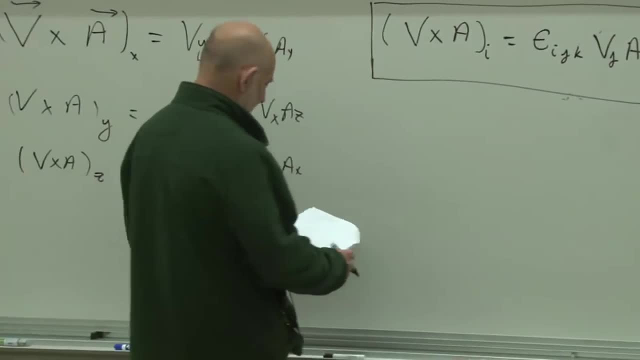 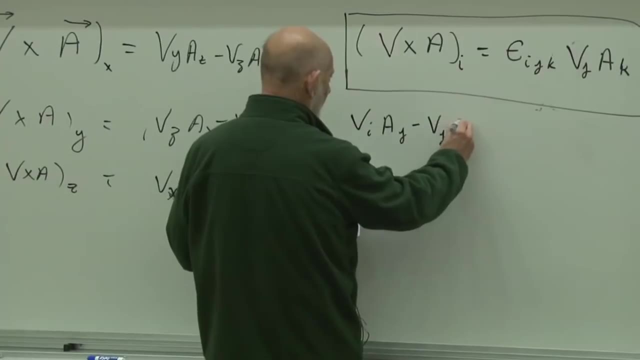 in this form. you can write it another way. I'll write it the other way. Here's the other way to write it: v i a j minus v j a i. Now, this left-hand thing is a thing with two indices. 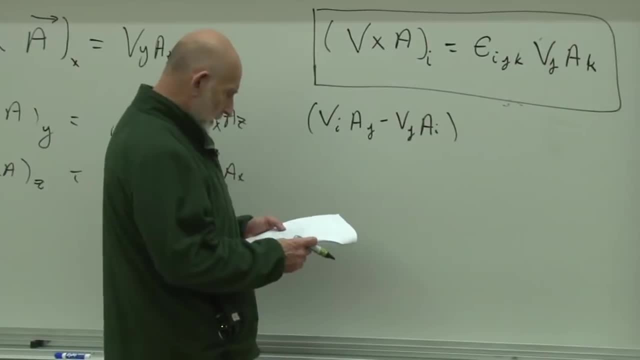 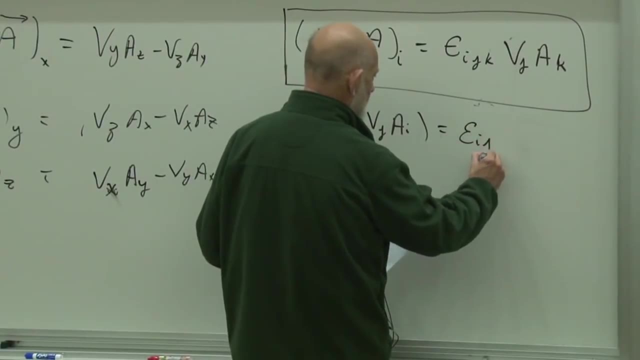 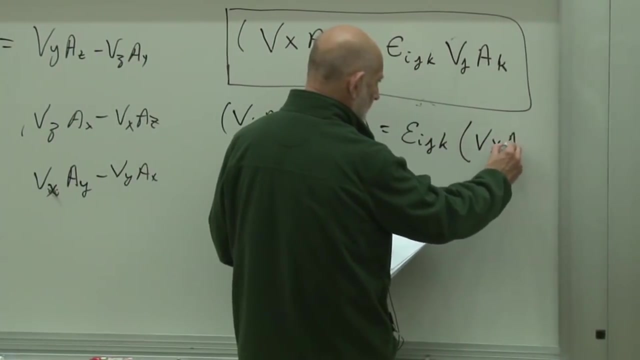 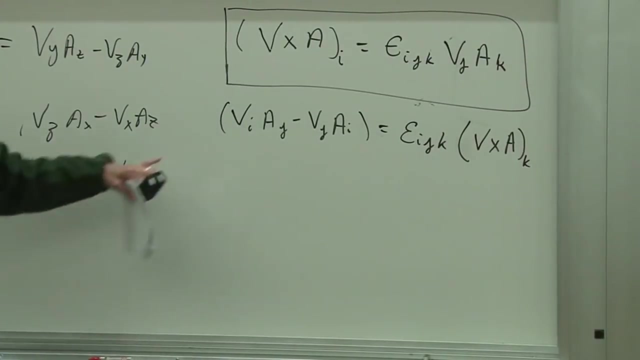 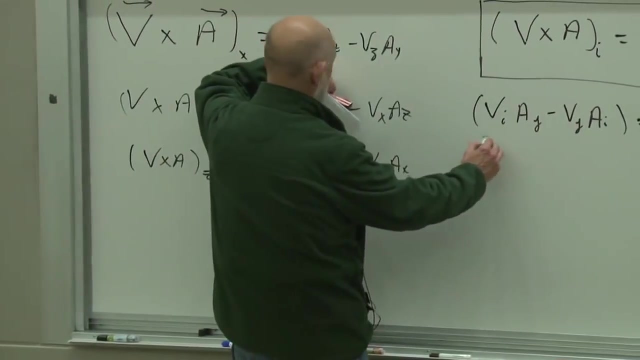 i and j is equal to epsilon i, j k times the k component of v cross a. Let's just check this one. Let's check one term. For example, here's v y. so this would be, i would be two. 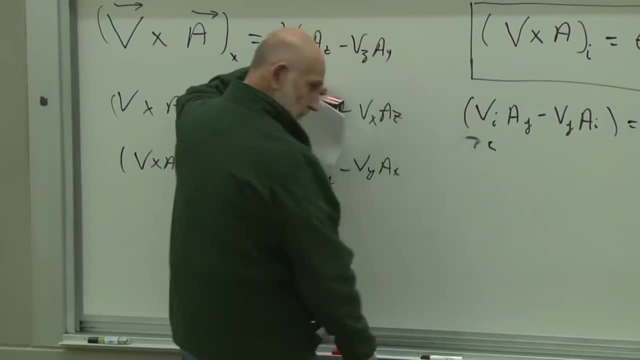 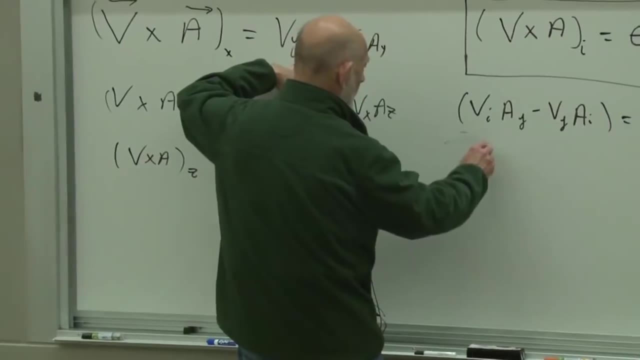 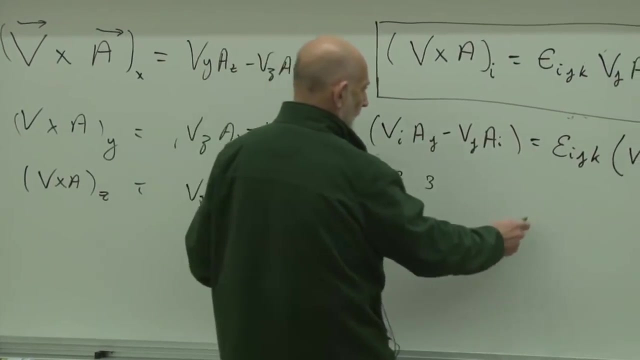 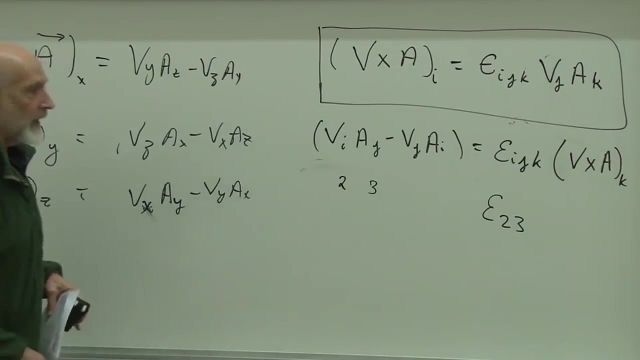 over here. i would be two and j would be three. This would be epsilon two- three. i and j are two and three. What's the last one got to be? It can only be one right. 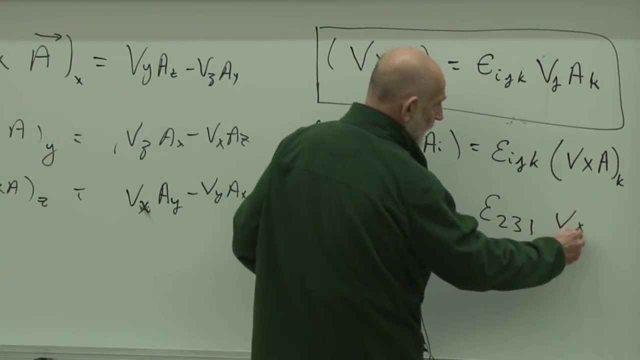 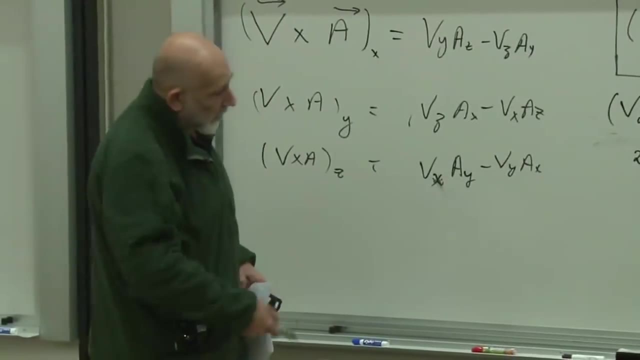 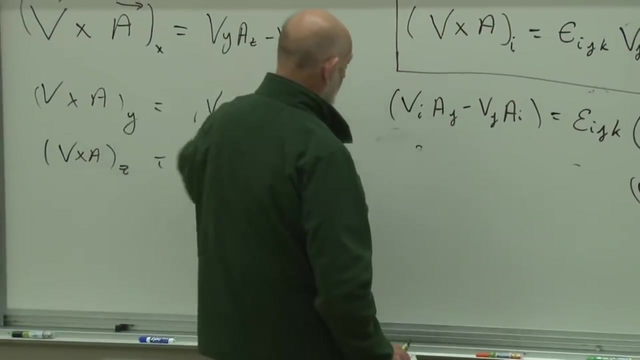 times v cross a, the first component, Epsilon, two, three, one is plus. That's a clockwise permutation, and so this just says the same thing that the first component. they say the same thing. 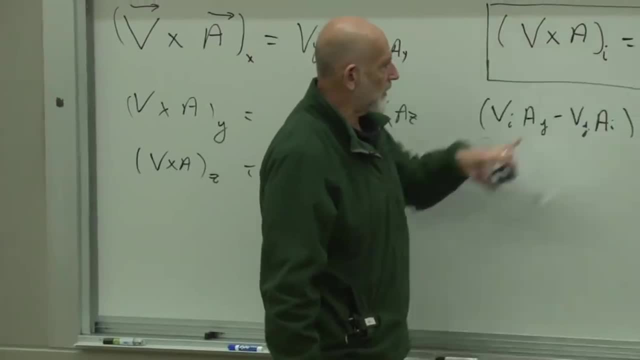 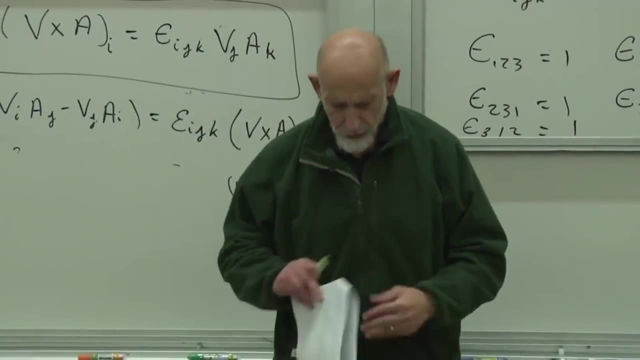 In one case we say that the cross the component. yeah, you can see, they say the same thing. Okay, that's the notion of a cross product and you all know the notion of a cross product. But now we can. 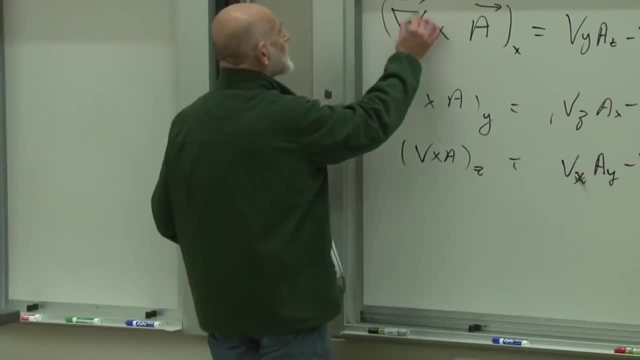 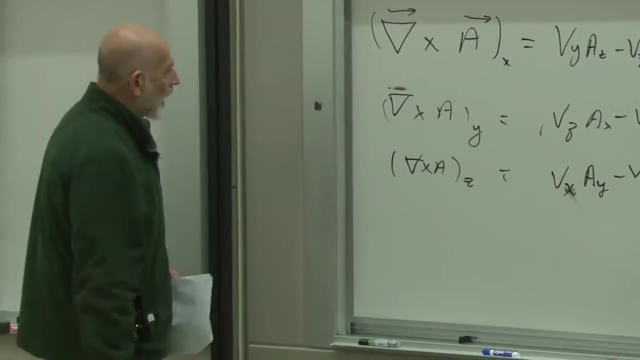 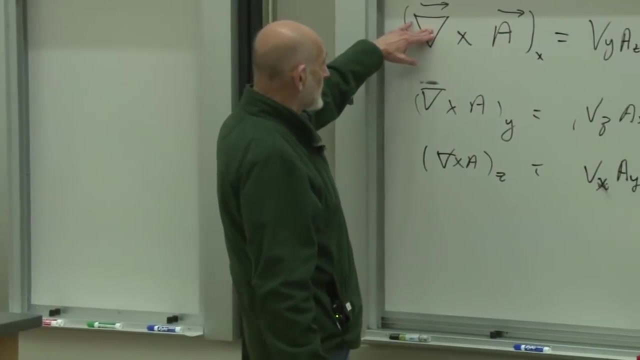 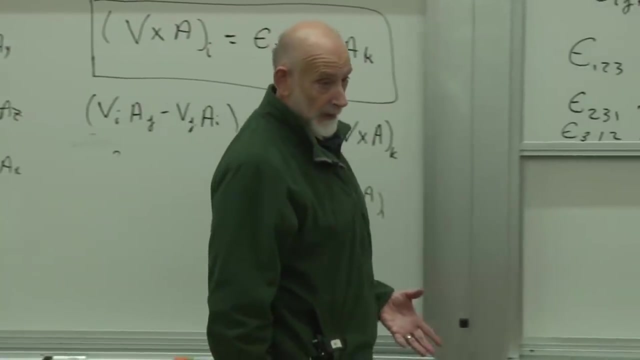 ask what happens if you take the cross product of del. we should put of del with a vector field, a. Then we replace the components of del by the derivative operations. What do we get? We get a thing called the curl of the vector field. 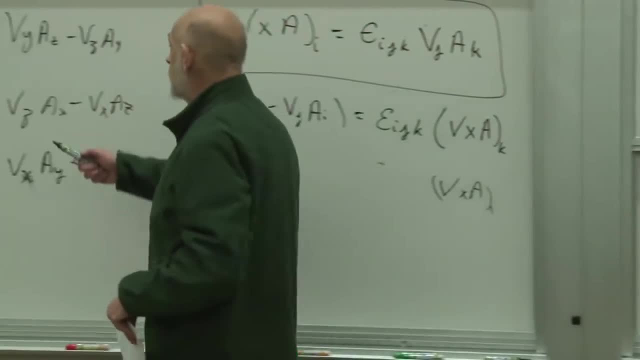 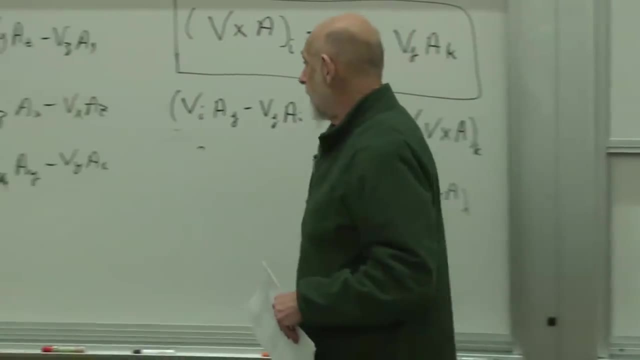 The curl, just as the cross product of two vectors is another vector, the curl of a vector field is also another vector field. It has three components and let's work out what they are. We can read it right off here: 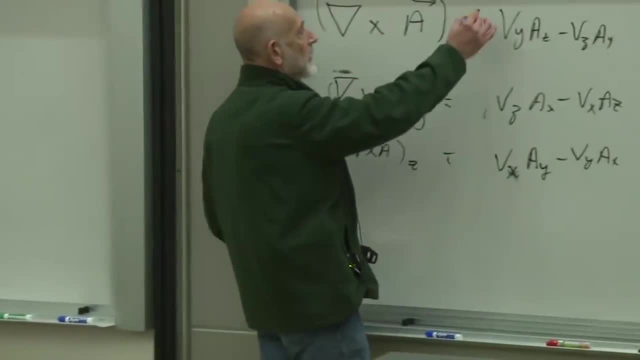 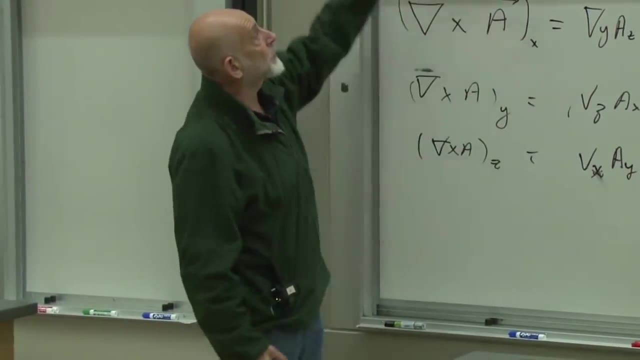 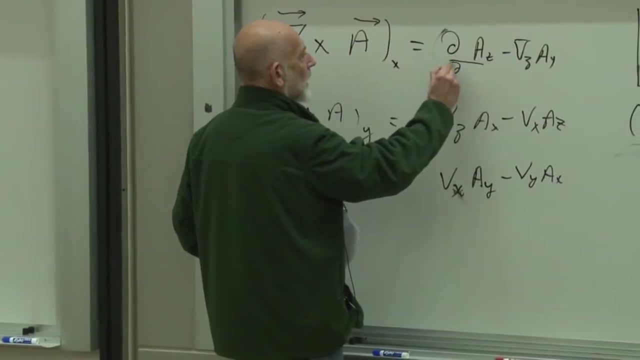 We don't have to do any more work, We just replace these by del's. But then what does del mean? Del means derivative with respect to y, So this becomes derivative with respect to y of a. 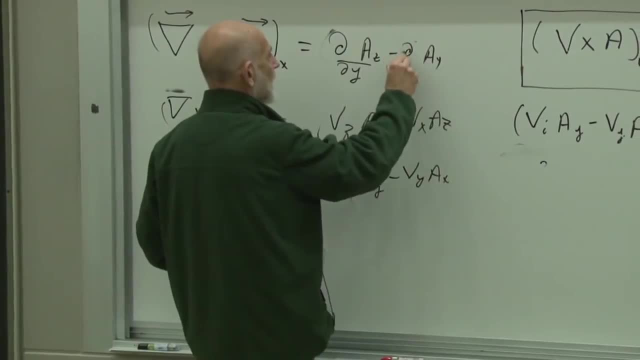 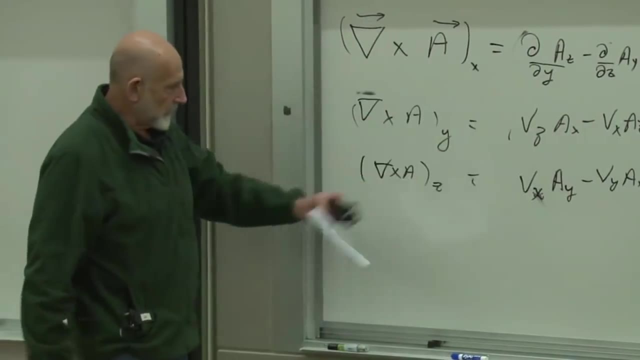 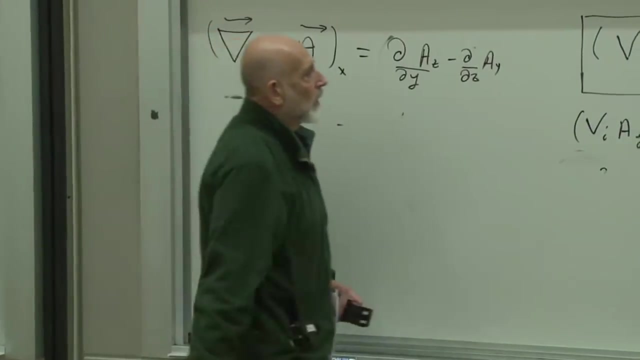 minus the derivative with respect to z of a. I'm not going to write the rest of these, Let's just forget them. You go. how do you get the rest of them? You cycle Or we can write. 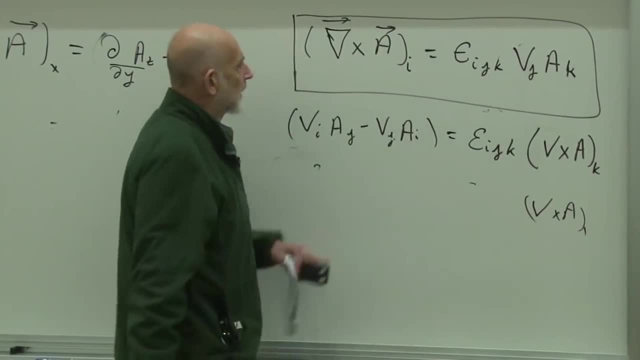 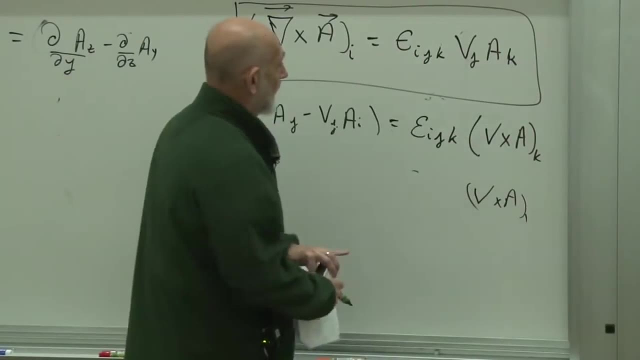 that the curl of a vector is defined, the ith component of it. excuse me, the ith component is epsilon times derivative with respect to x. 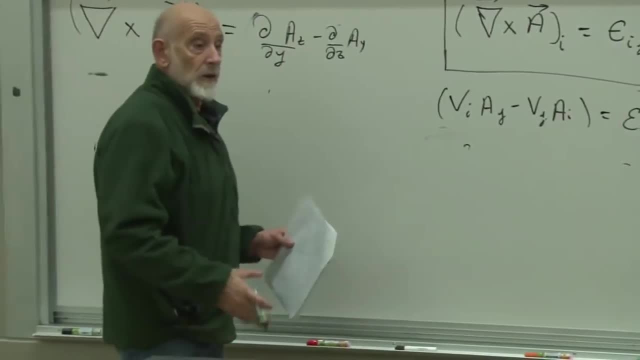 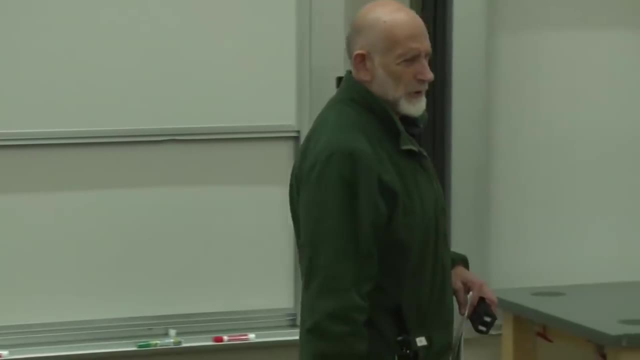 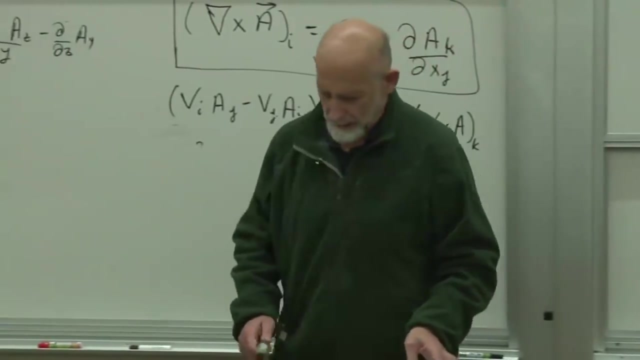 of a. That's the notion of the curl of a field. You may ask what kind of information is contained in the curl, What kind of information, first, is contained in the divergence of a field? Well, it's the tendency. 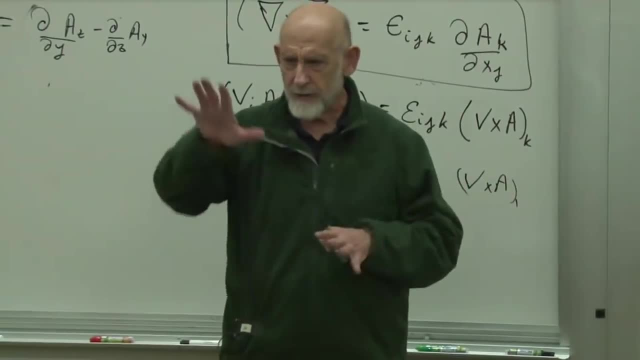 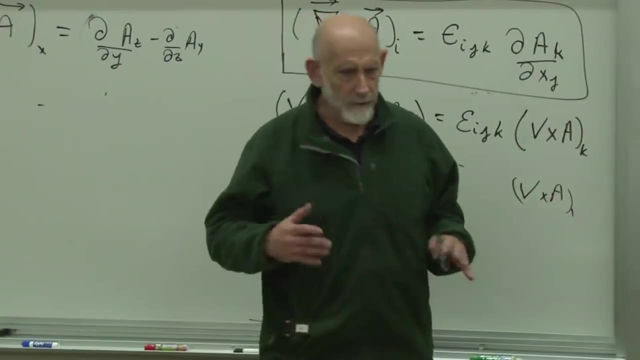 the divergence sort of measures, the tendency for the field to spread out away from a point. Roughly speaking, it's a very, very rough idea. In fluid dynamics it represents the source of a new fluid coming into a system. 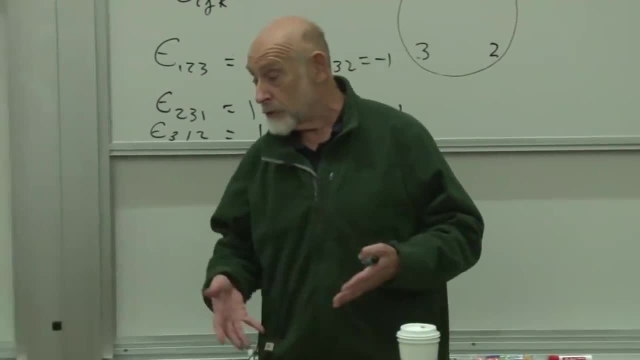 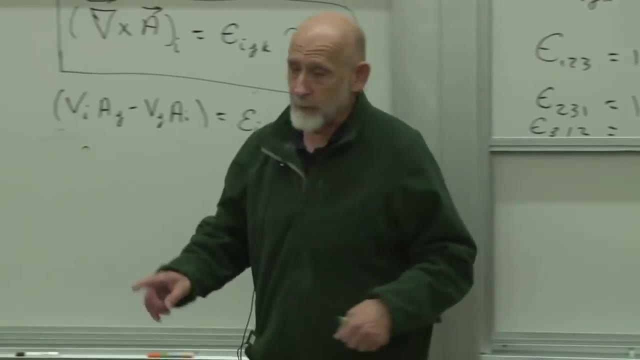 but it's the spreading idea. Of course. if the divergence is negative, then it's the sense that the fluid is flowing together. The curl represents a tendency for the fluid to circulate around some. 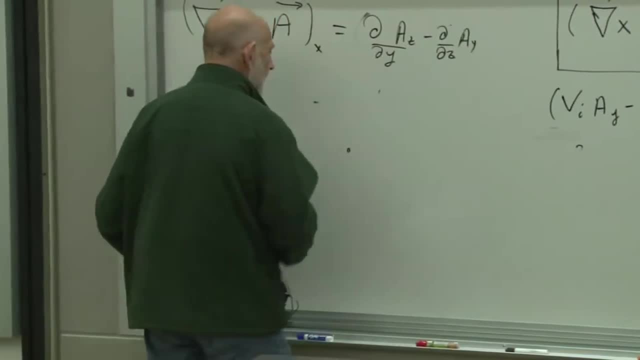 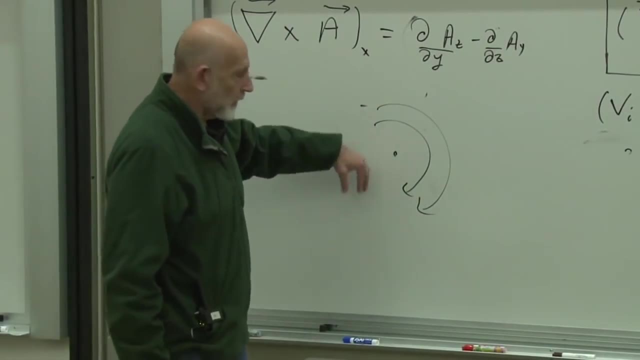 some point. So, in particular, if you had a, if you had a fluid which was circulating around a point, there would be a large curl to the fluid at the point where it's circulating around. So curl is representing exactly what it says. 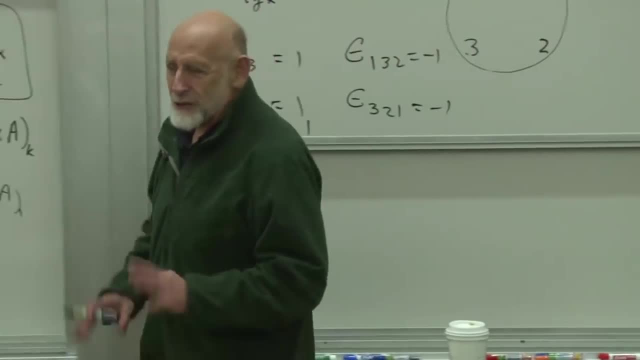 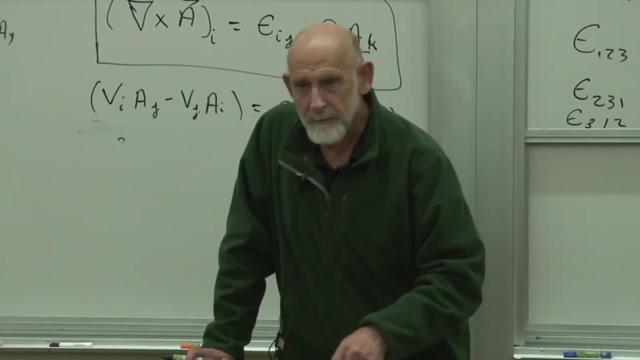 the sort of curliness of the flow, but it's not always so easy to see what. the what, the Yeah question. No, no question. 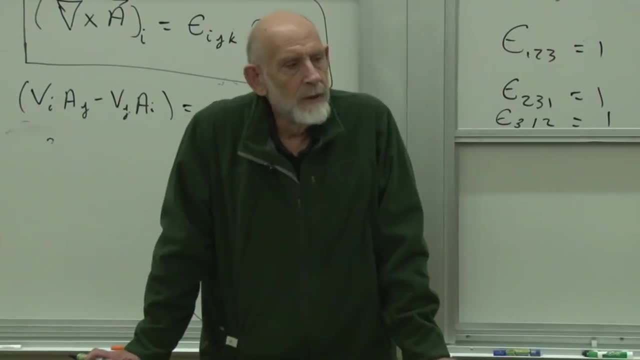 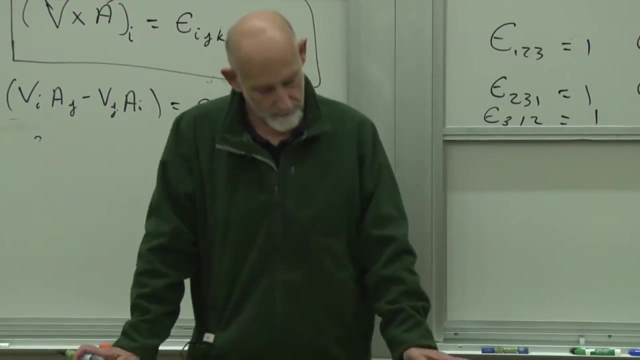 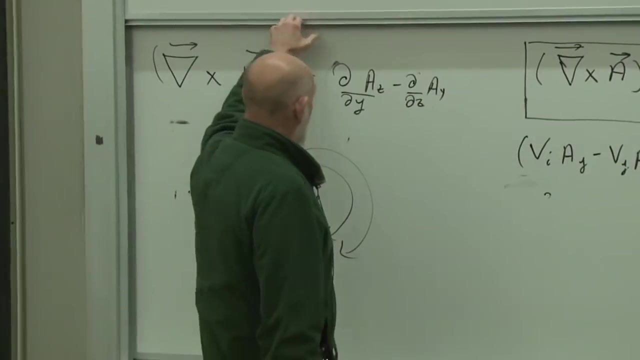 Does that notation and the idea of curls and cross products? does that have any meaning except in three dimensions? No, Well, I Yes, but a different meaning. You can either. Okay, so you can either think. 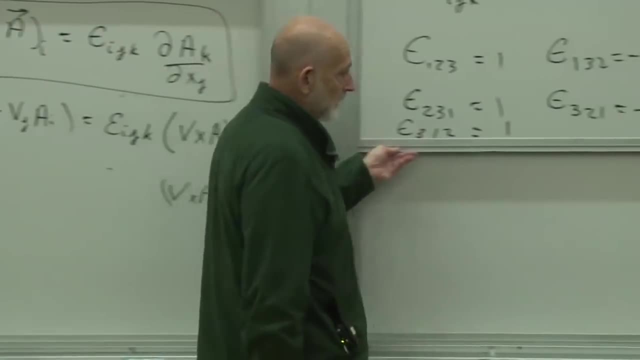 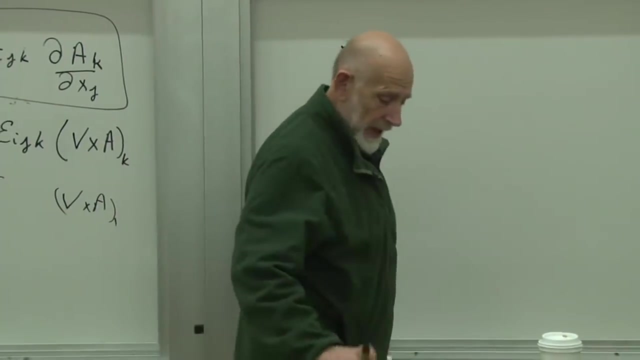 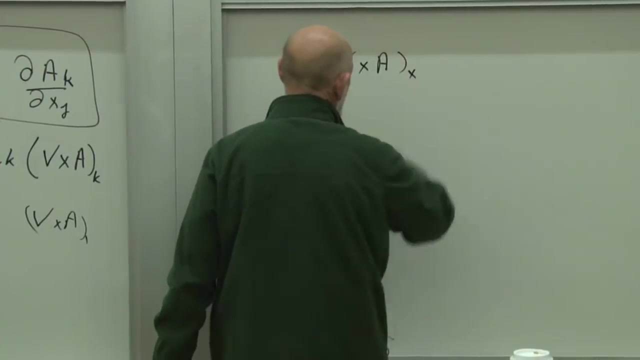 of the cross product as giving you another vector. let's take the cross product of v and a again. you can write it as del- sorry, not del, but v cross a- and it has three components: x, y and z. 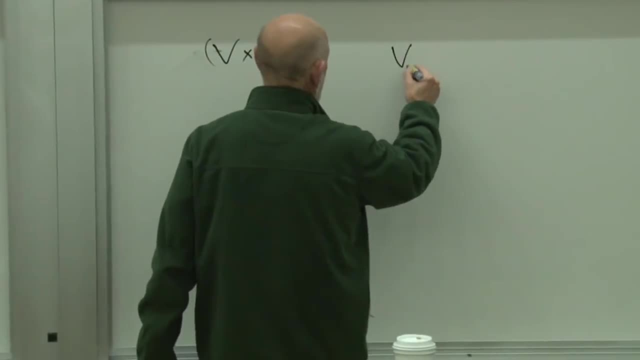 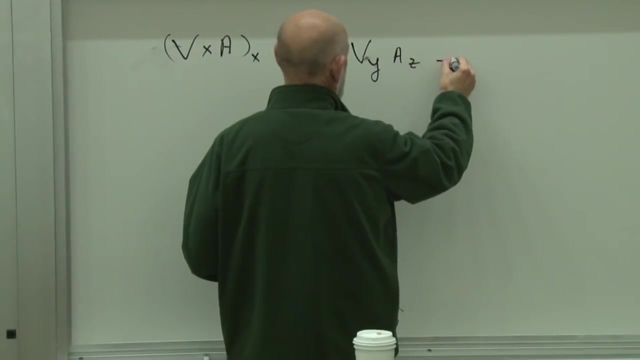 You can also write it as well, for example v y a z minus, v z a y or whatever it is, and you can think of it as: 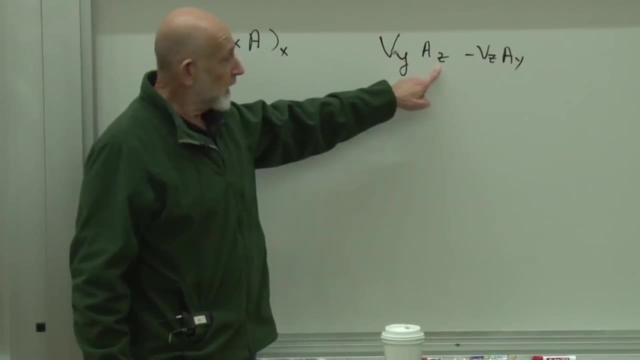 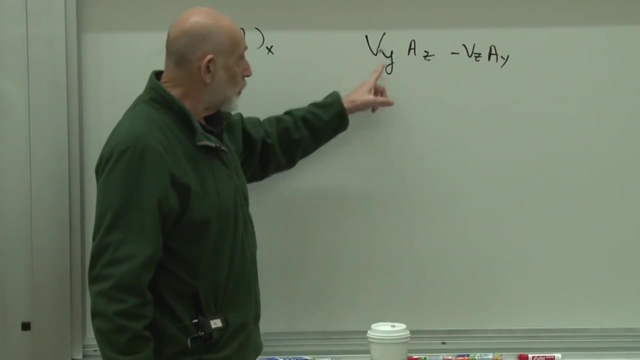 you can think of it as a thing with two components. It's anti-symmetric, it's an anti-symmetric object, a two-by sorry, a three-by-three matrix, so to speak. You can make a matrix out of it. 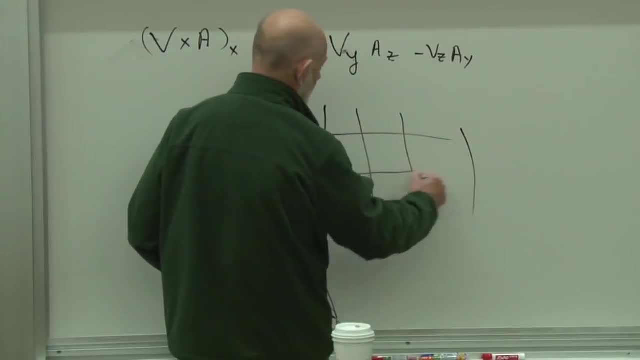 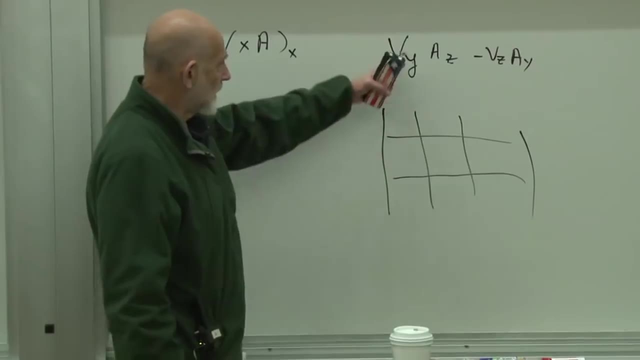 and in each entry in the matrix, what kind of things are on the diagonal of this matrix Zero? The diagonal elements are zero: v y a y minus v y a y. 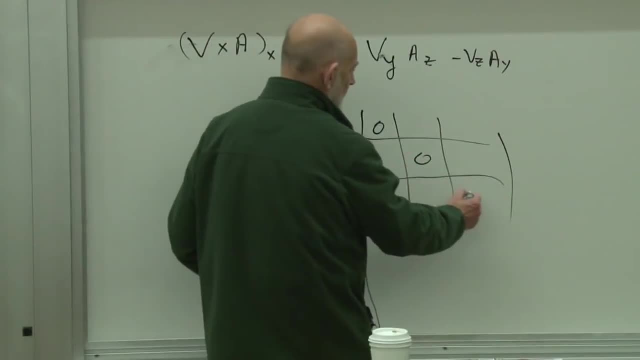 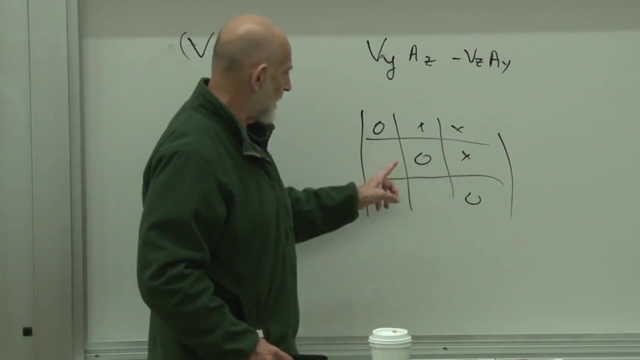 is just zero, Zero on the diagonal, some things off the diagonal. this would be the y z component. let's see, here would be. here would be the y z component. 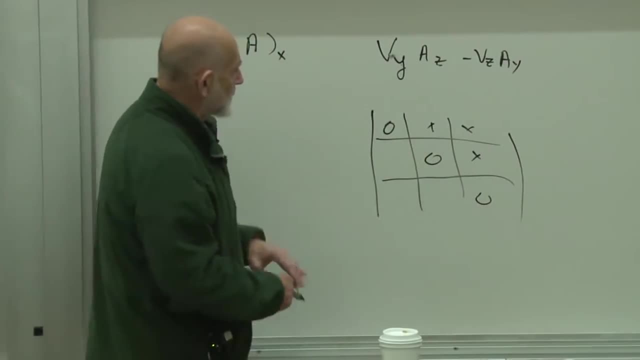 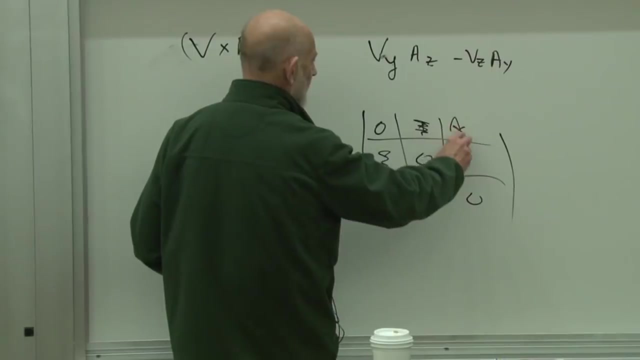 right, over here, all right, and it's anti-symmetric. so whatever its value is over here, its value is the opposite over here, minus and and. 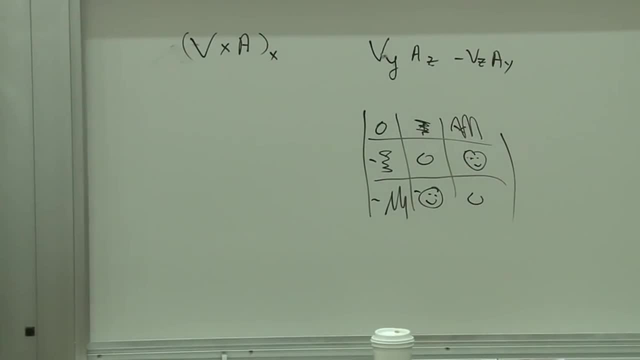 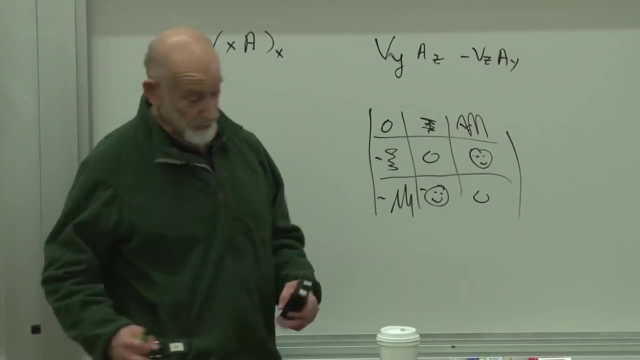 minus over here. okay, so it's anti-symmetric. and how many components does an anti-symmetric matrix have? How many independent components? One, two, three? these are not independent. 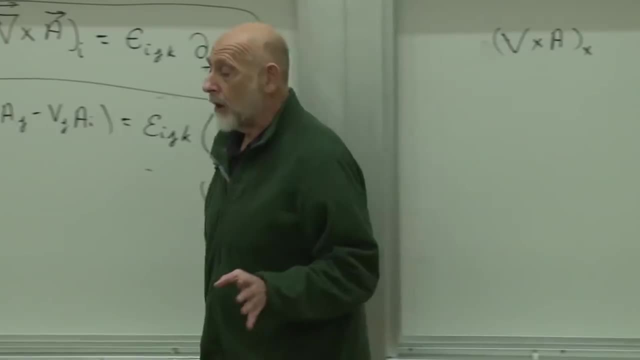 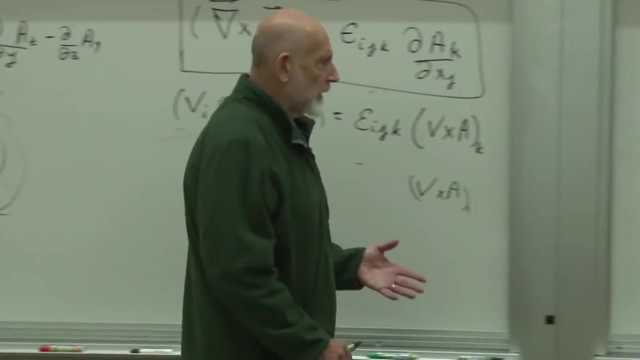 they're just the negatives of the ones up here. so the amount of the number of quantities, number of components of an anti-symmetric matrix in three dimensions is also three. 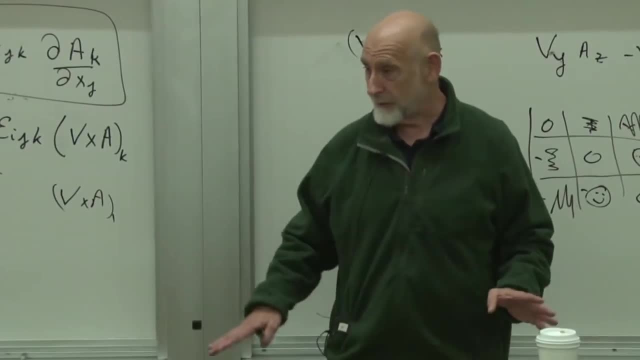 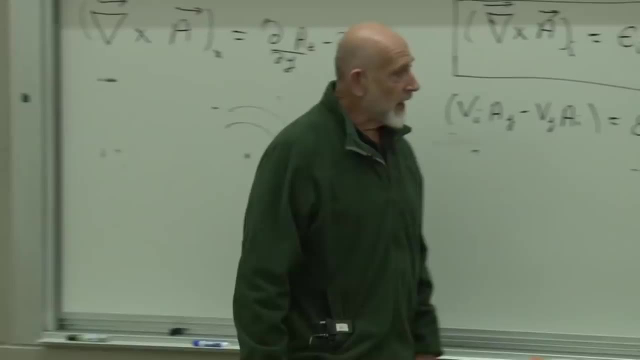 that matches the three components of the vector. that's why you can identify them. now what about in four dimensions? let's go to four dimensions. how many components of a vector are there? four? 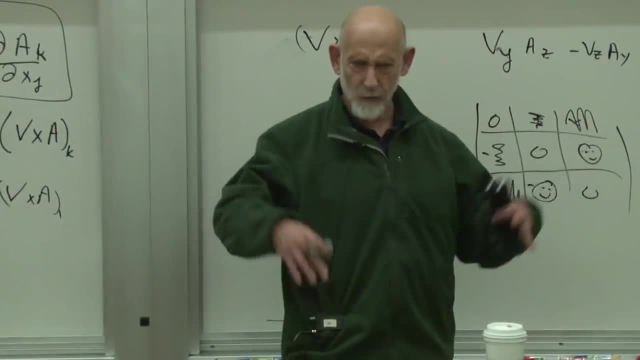 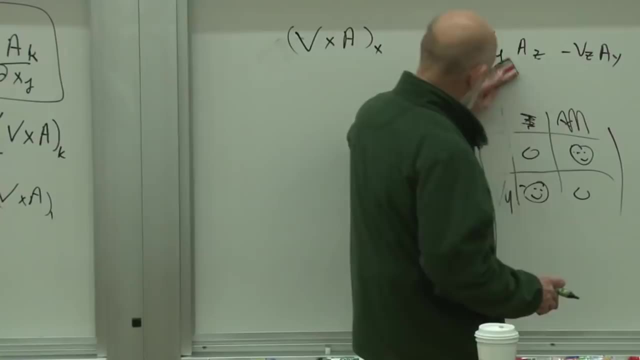 four. we're not thinking about relativity now, just a four-dimensional space, four-dimensional space, four-dimensional space has four component vectors. how many components are there to an anti-symmetric matrix? 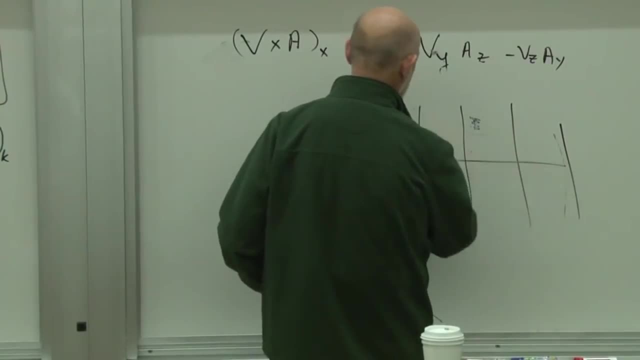 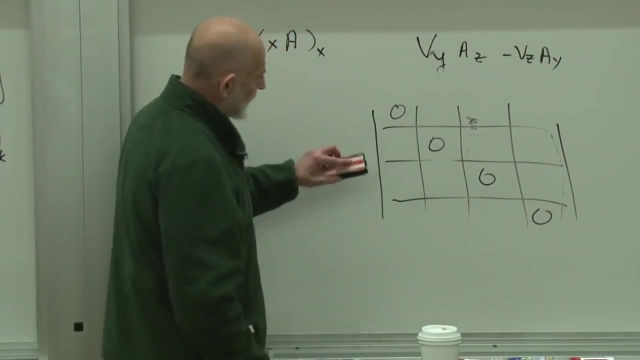 all right. so now we have four by fours, zero on the diagonal. it's anti-symmetric, so the off, so the lower. the lower half here is just the same as the upper half. 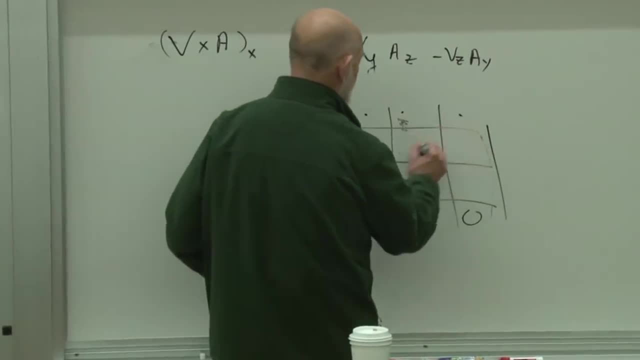 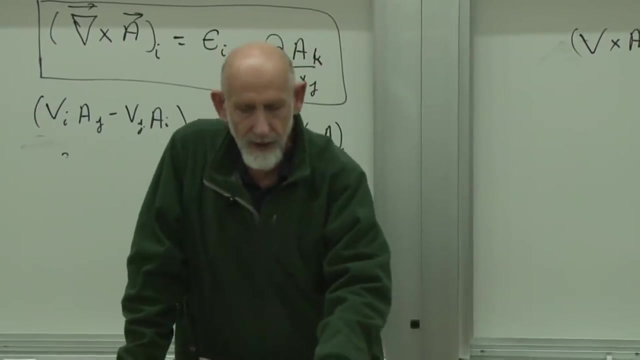 except for the sign. but then there's one, two, three, four and seven dependent components, so you cannot in other dimensions identify anti-symmetric matrices. 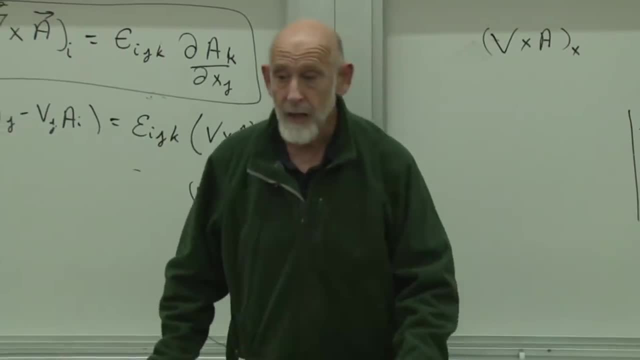 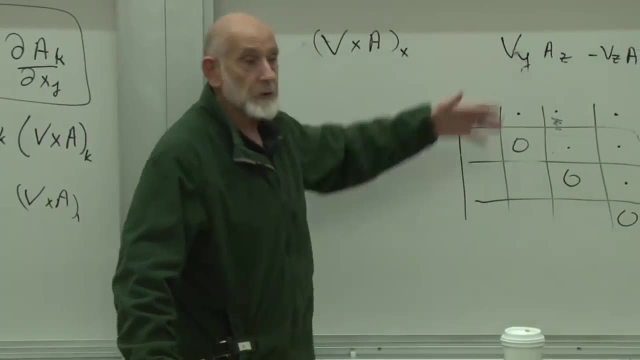 with vectors. that's a special to three dimensions, all right. on the other hand, the anti-symmetric matrix of components like this always exists and it's a generalization of the cross product. 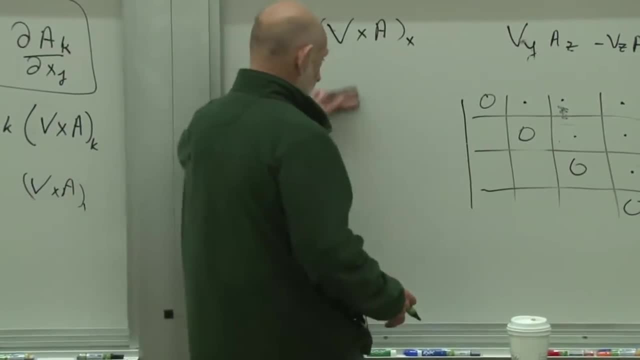 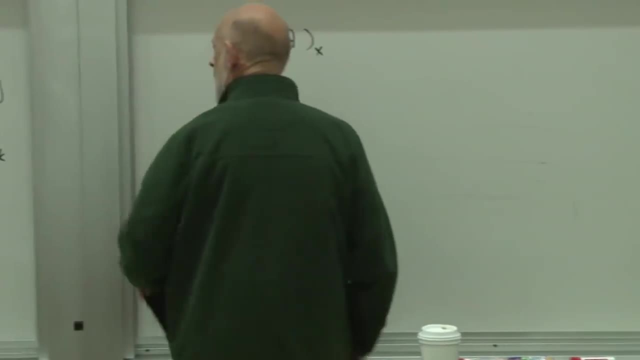 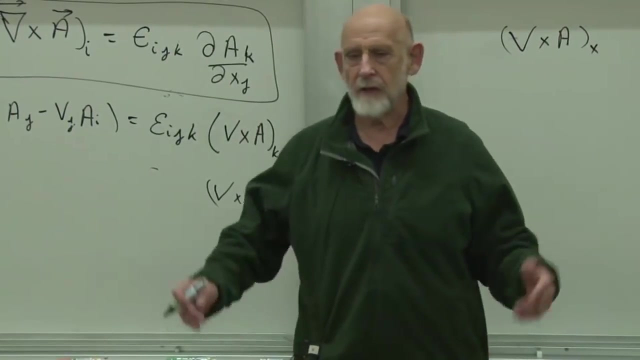 but cross product in other dimensions is not itself a vector. but let's not, let's. let's stick with three dimensions for tonight. what's the name of a thing? a field which is anti-symmetric, like that anti-symmetric tensor field? it's called a form. 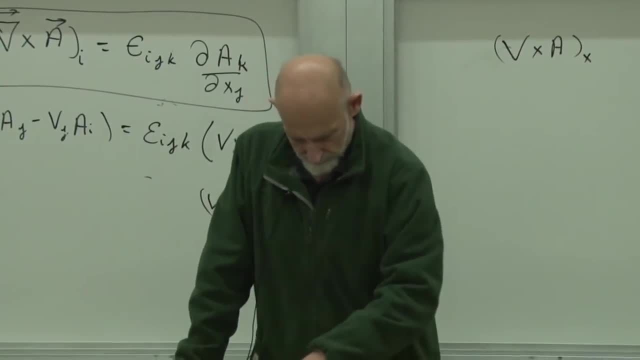 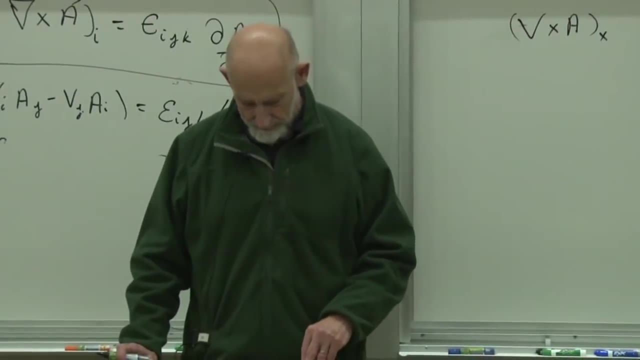 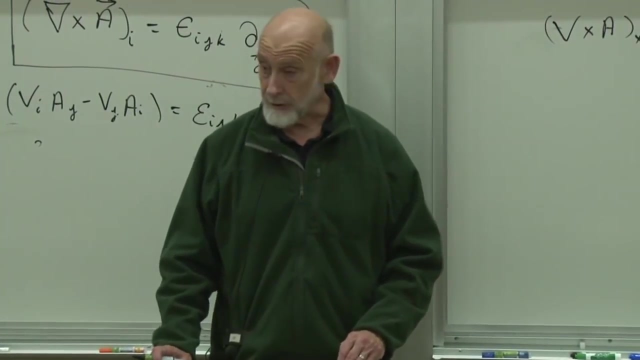 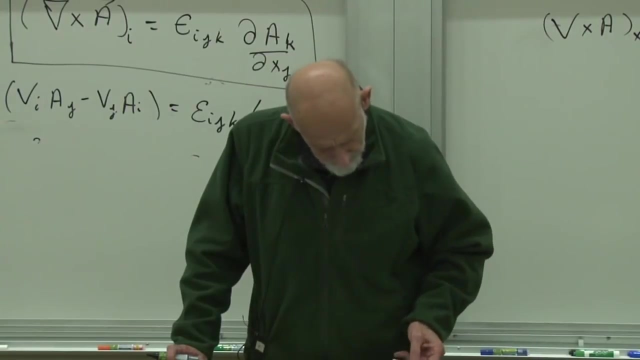 it's called a form, but what's in a name? okay, now we have divergence, curl and so forth, gradient. gradient is just something which acts on a scalar, and i want to state some theorems. these are theorems which are easy to prove, so easy to. 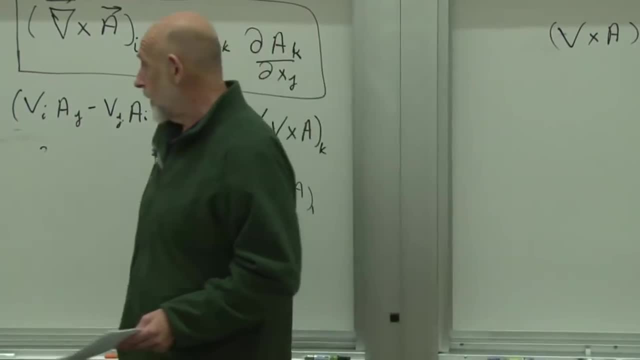 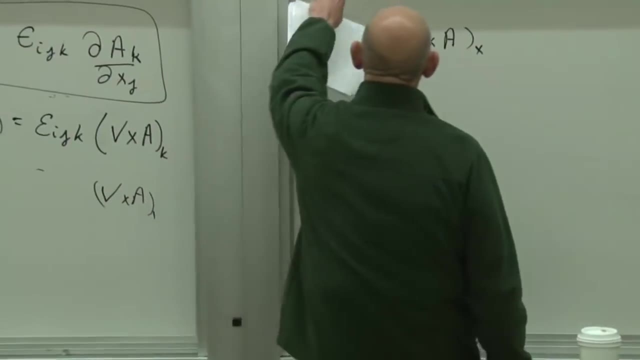 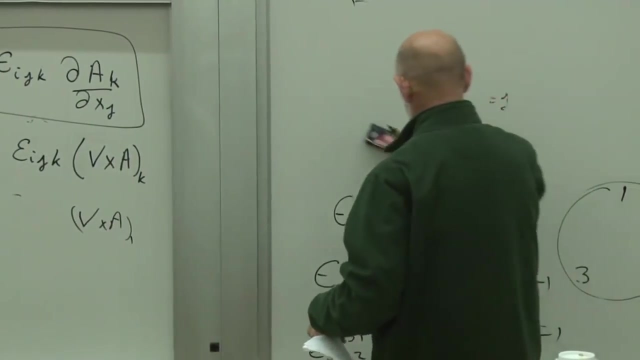 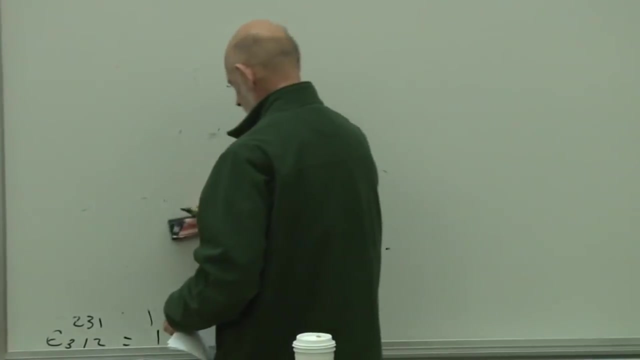 prove. they tell you, you just write them down and you will see it immediately. the first theorem: and these are your homework. okay, these are your homework. you will be tested on them. next week there'll be a short pop quiz and i'm looking forward tremendously to grading it. 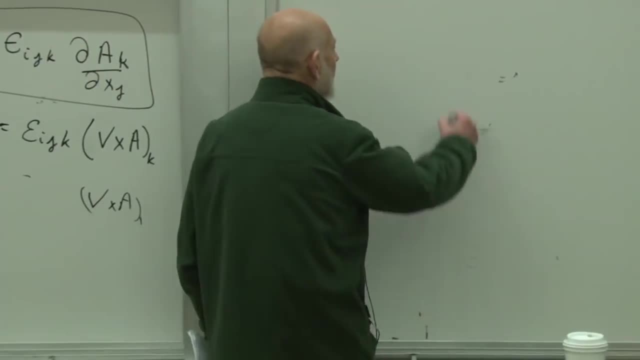 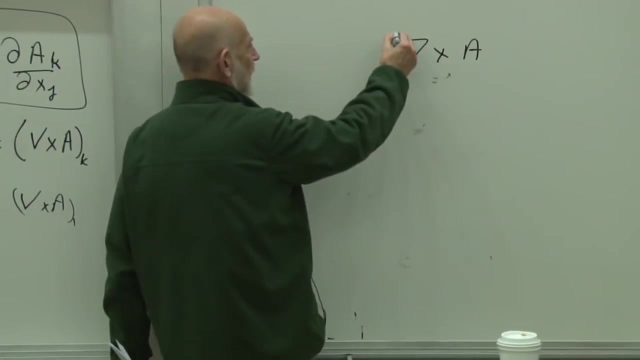 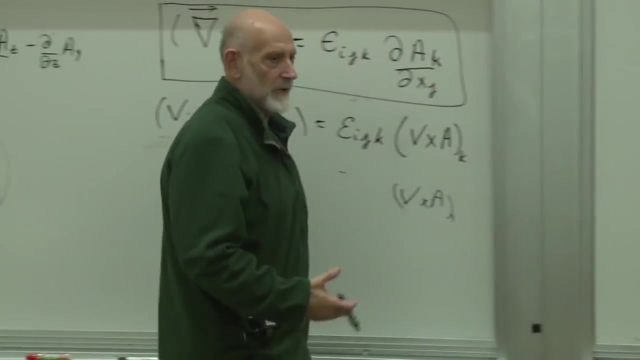 the first thing is to prove that if you have a curl of anything, a is anything. i'm going to stop drawing arrow. well, let's, let's draw some arrows. okay, this is a vector, right, and it's a field. it itself is a vector in a field. i put some brackets around it. 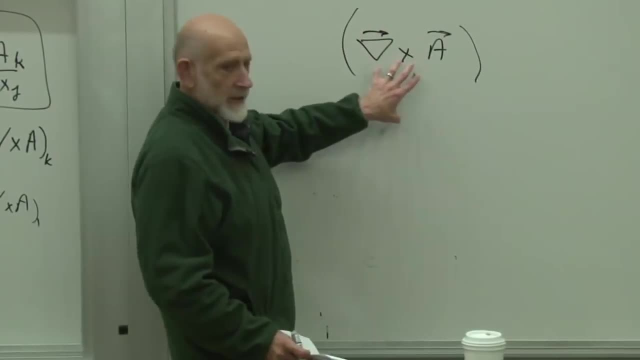 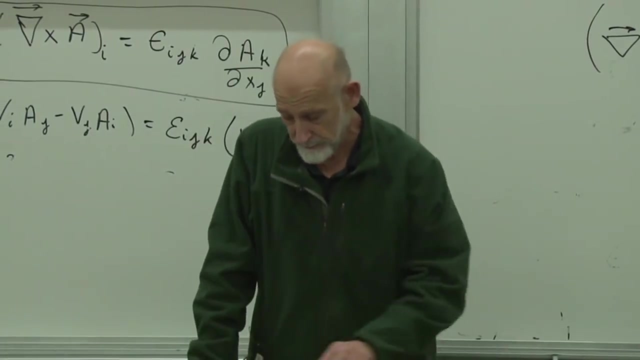 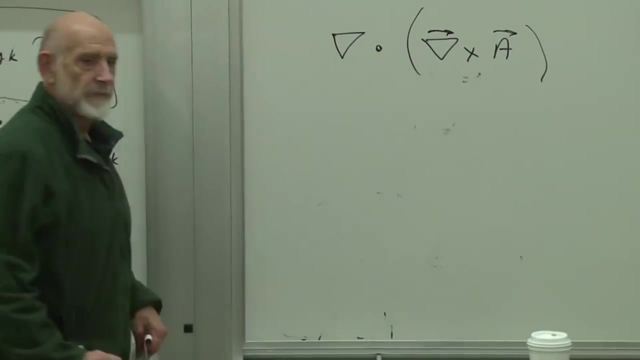 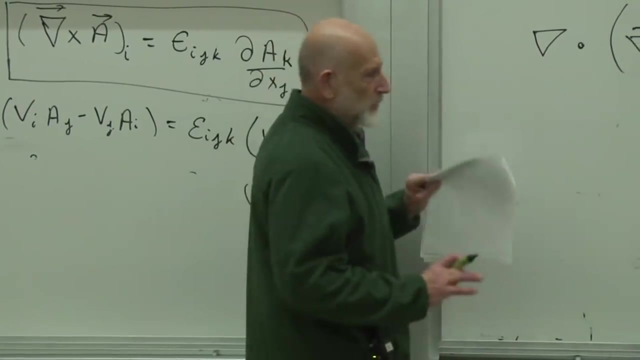 to indicate that. uh, you know, it's a structure on its own and it is a vector field. given any vector field, you can compute the divergence of the vector field. okay, so you can take the divergence of a curl. the first theorem is that the divergence of any curl is always zero. 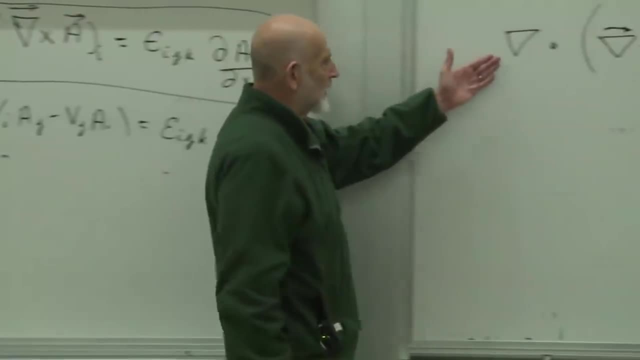 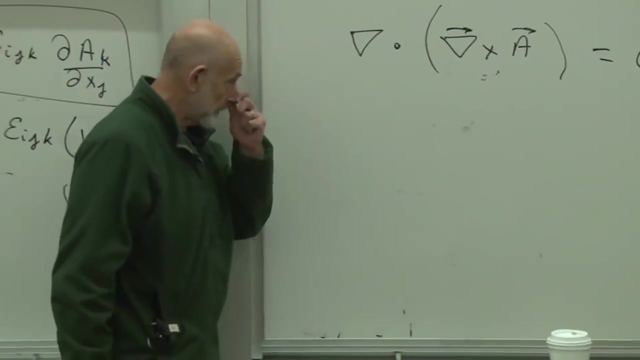 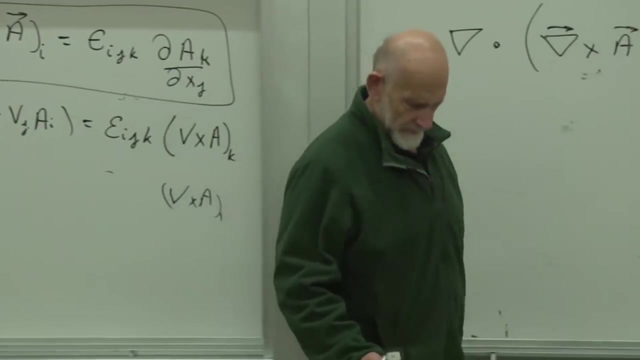 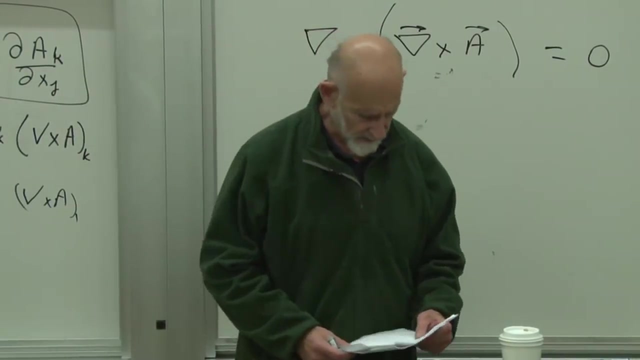 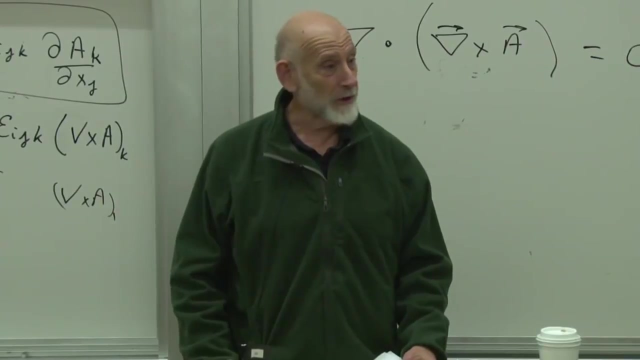 this is not a tricky proof. you just write it down, what these things are, and you find out they all cancel among themselves. several different terms cancel. So the divergence of any curl is equal to zero. There's a harder theorem, which is that if the divergence of a field is zero, then that field must be a curl. That's harder. 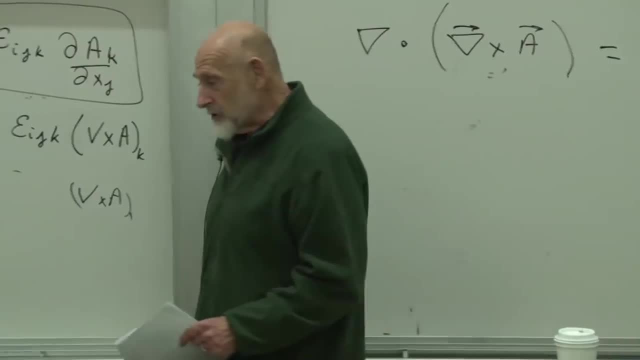 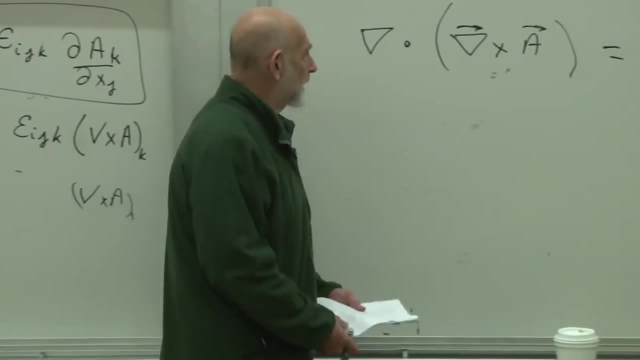 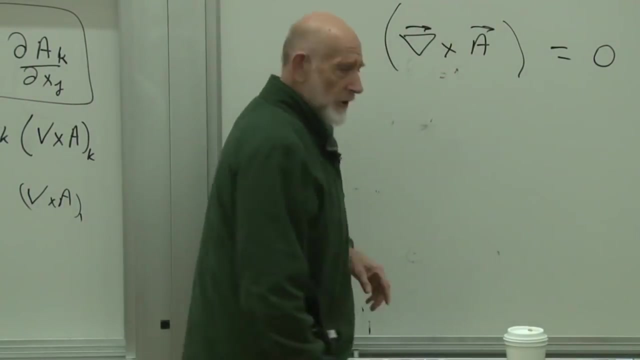 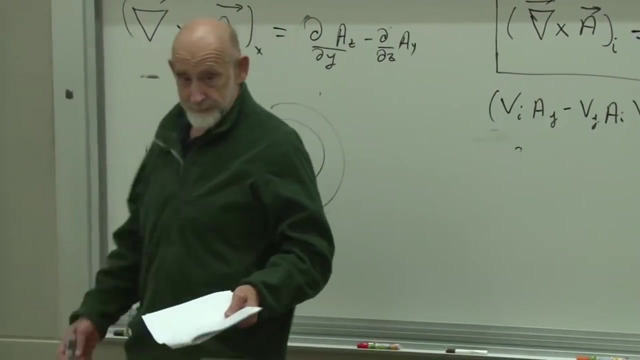 This is one of these if and only if statements. One side of it is easy to prove, The other side is harder to prove. But if, and only if, a field is a curl, then its divergence is equal to zero. So you can identify things with divergence zero with curls in general. 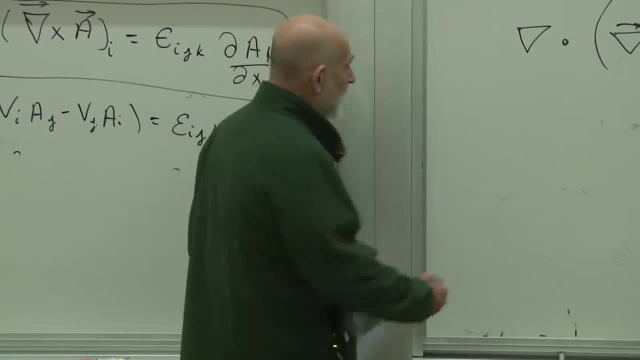 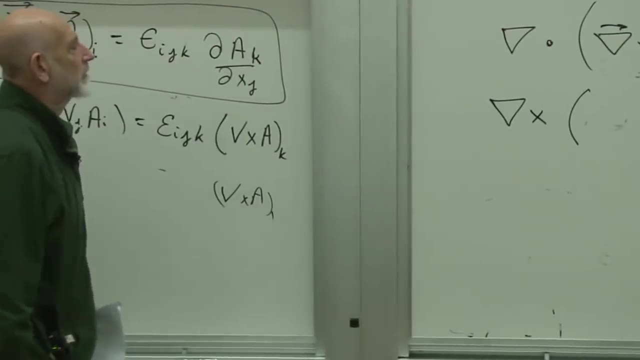 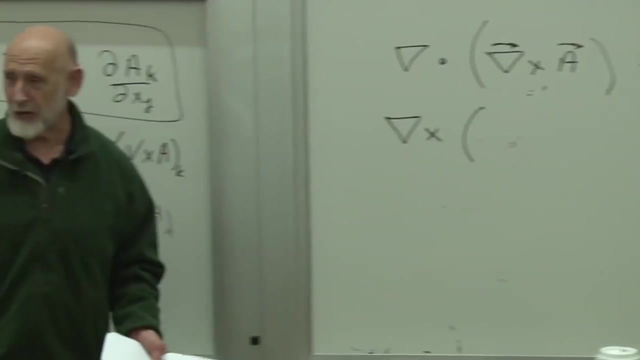 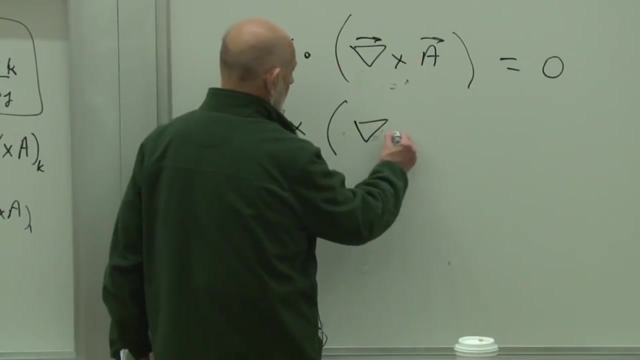 Then there's another similar theorem that talks about the curls of. can you guess what it's? a curl of The curl of a gradient? It couldn't be the curl of a divergence. A divergence is a scalar and you can't take the curl of a scalar, But you can take the curl of a gradient: Gradient. 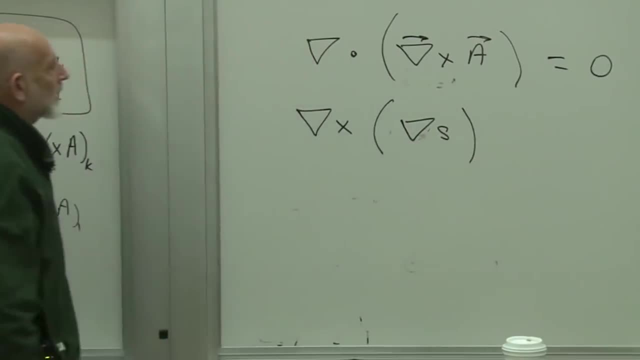 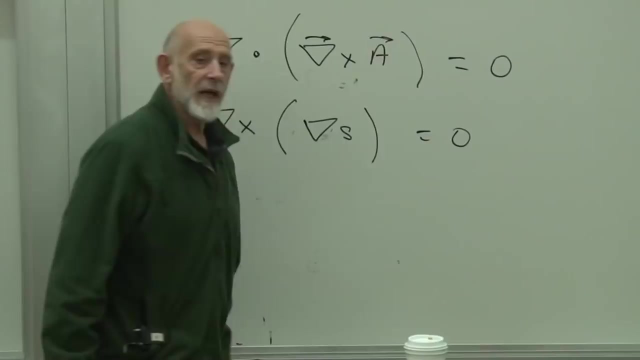 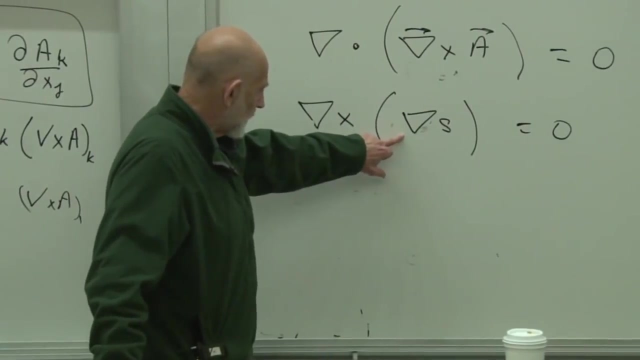 of a scalar Same thing. The curl of any gradient is also equal to zero. And again, it's an if and only if statement. So if and only if. If something has a vanishing curl, then that thing itself must be a gradient. 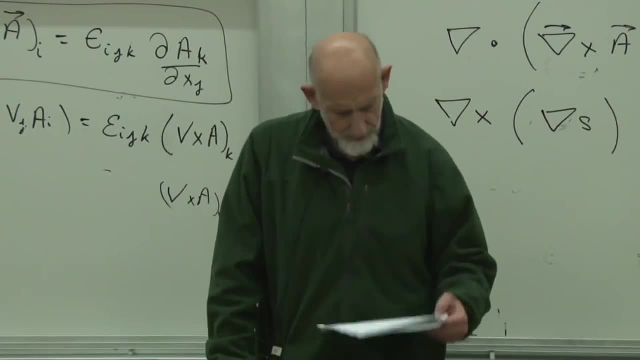 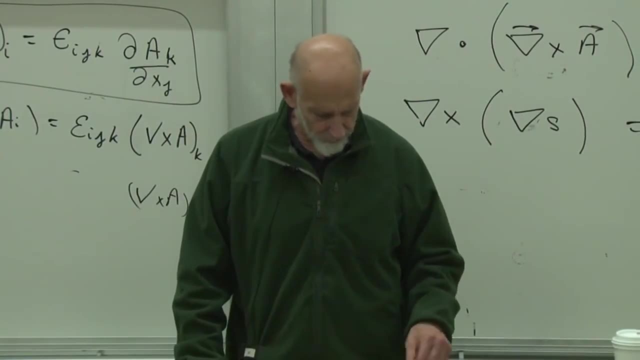 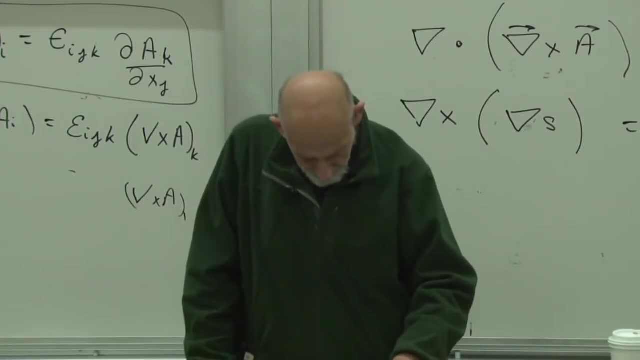 So these are little homework problems that I assign you. As I said, I only assign the easy part. The hard part I can prove, but so can you, I think. But you have to. it's more work and it's trickier. 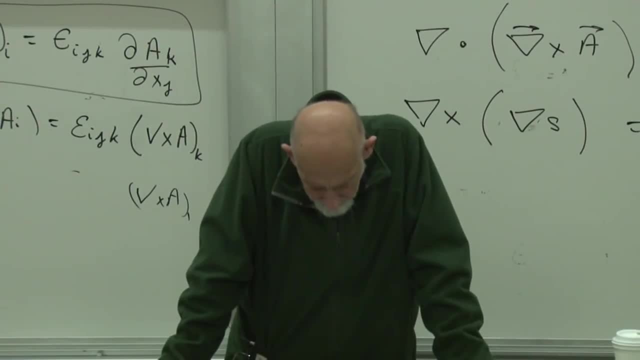 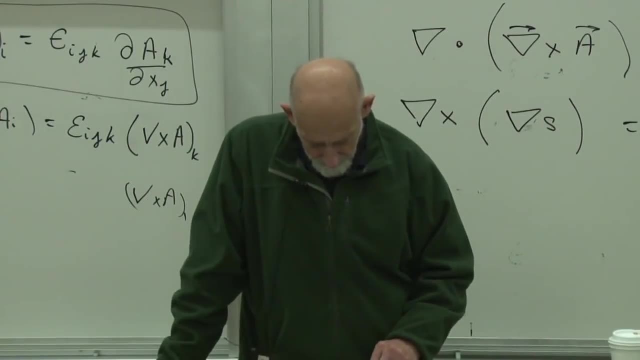 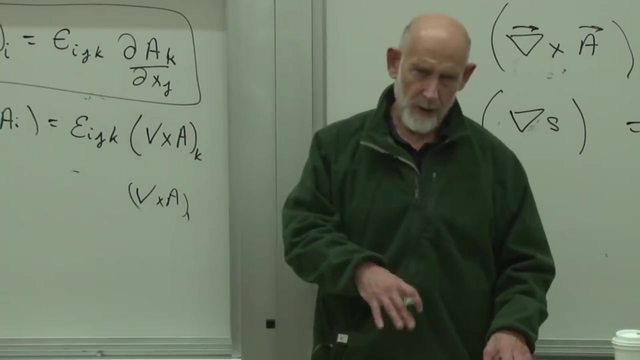 Okay, So Now, Now we have some machinery, Vector calculus, We'll call it vector calculus. We have some machinery, some simple theorems, And we're ready to think about magnetic fields, Electric fields are. we'll come back to electric fields, Those are straightforward, Those. there's nothing. 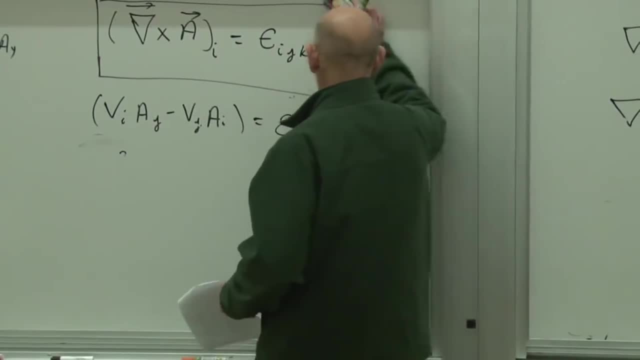 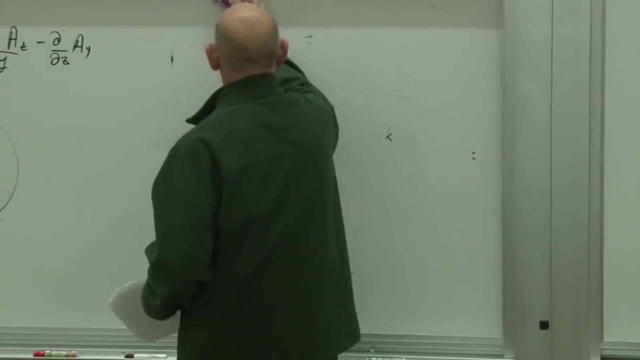 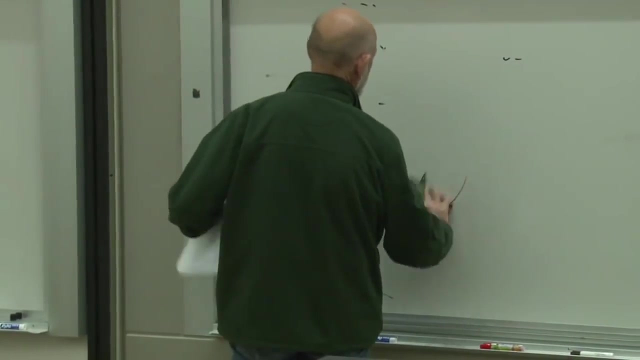 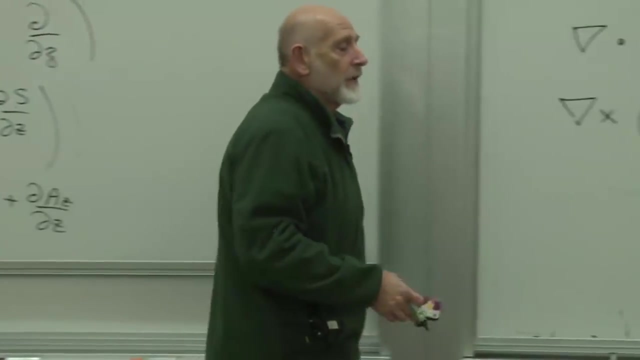 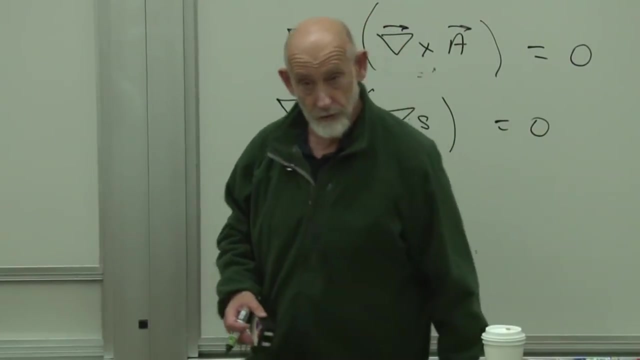 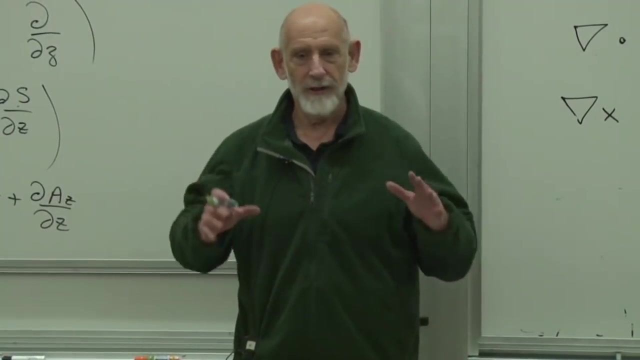 tremendously subtle about electric forces. It's magnetic forces that we really want to explore. Okay, Okay, Okay, Okay, Okay. Now, of course, a magnetic field is defined by definition, through its action on charged particles or charged currents, currents of flow. 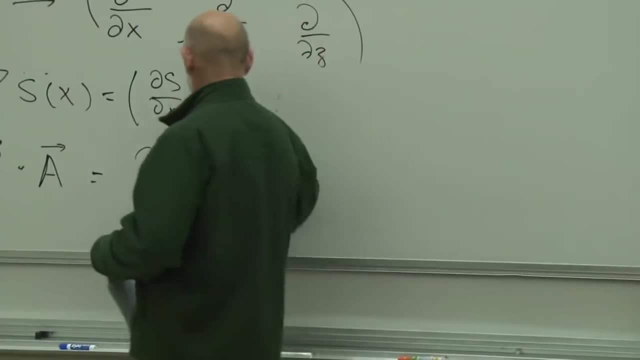 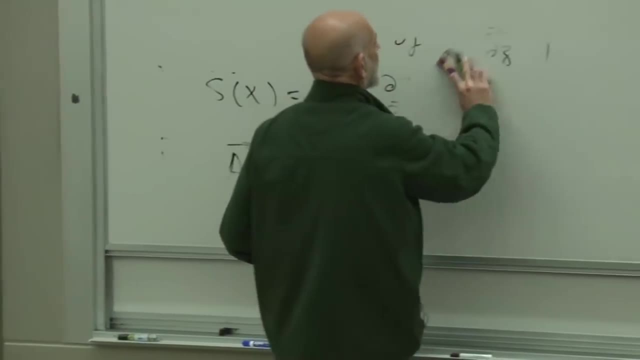 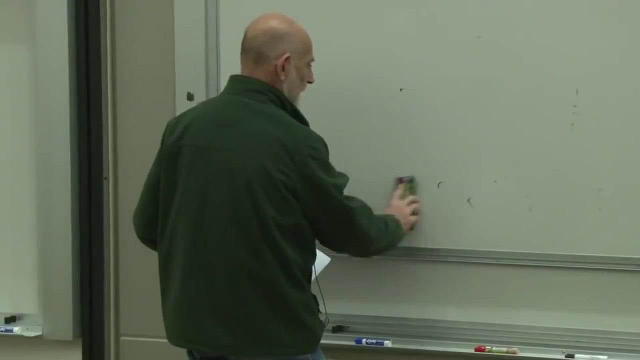 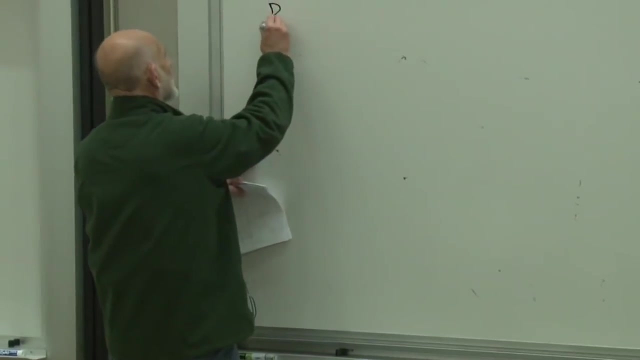 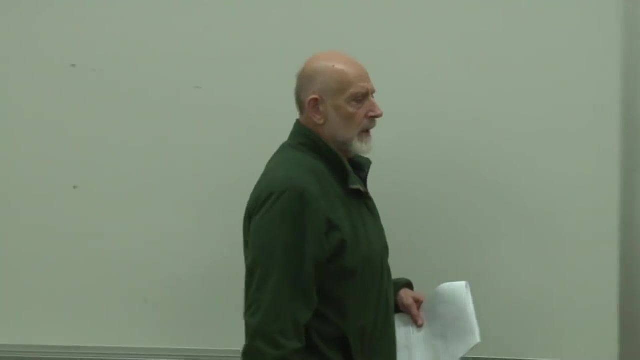 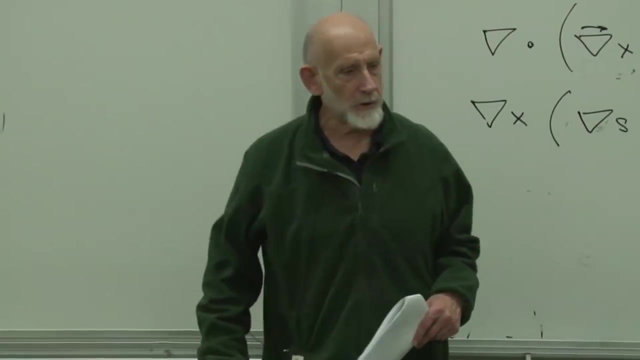 magnetic field. It's labeled with a B, B for bagmatic field. I do not know who was the first to call the magnetic field B. It's a vector and it has a one important property. It's important property is that its divergence is always equal to zero. Now, what is the 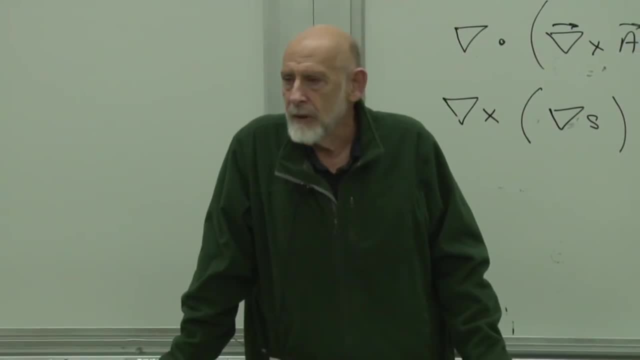 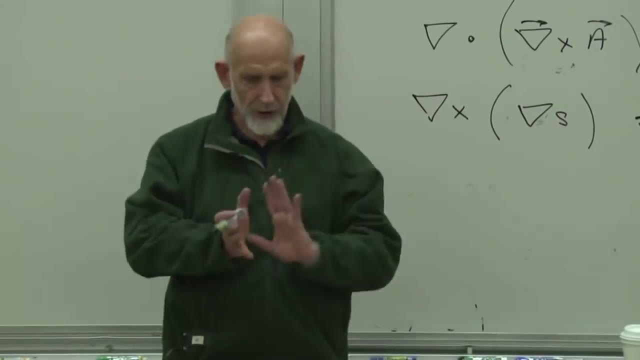 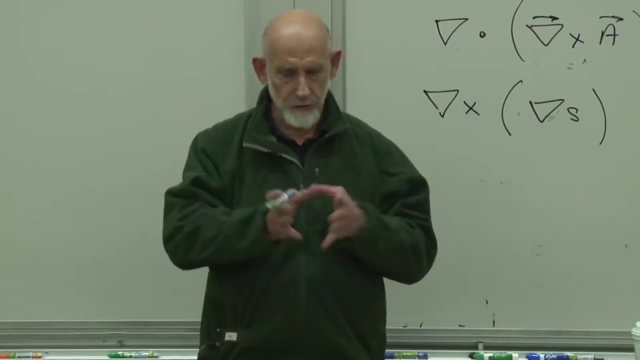 divergence of an electric field, It's the charge density. Okay, So wherever there's a charge, the field spreads out from that charge and the divergence is nothing but the response due to the charges and the field flowing out of it- Magnetic field and the charge you call the source of the field. 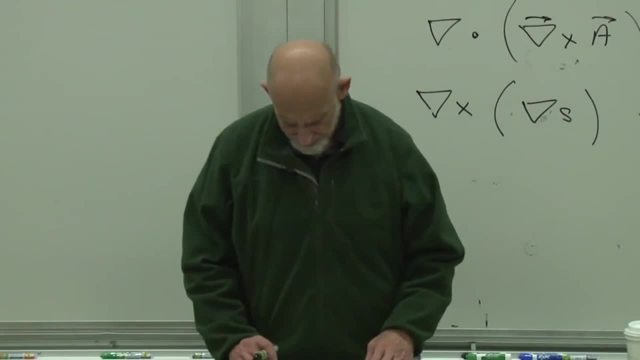 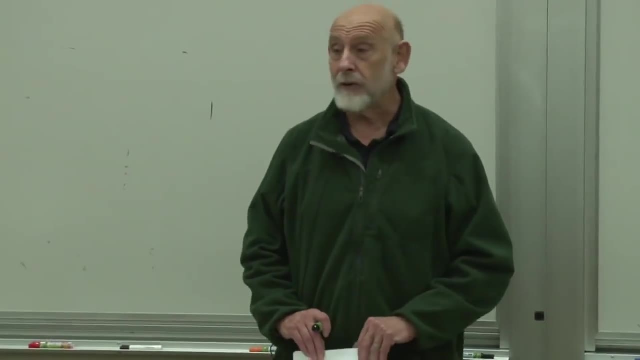 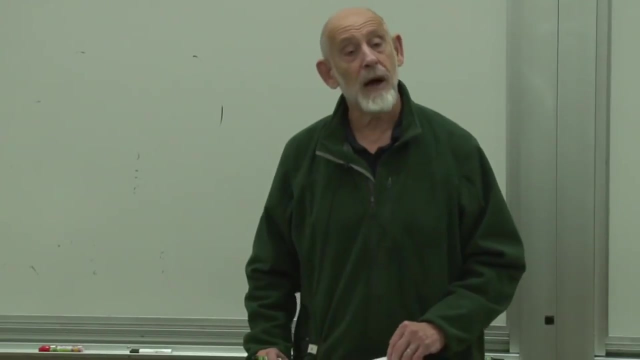 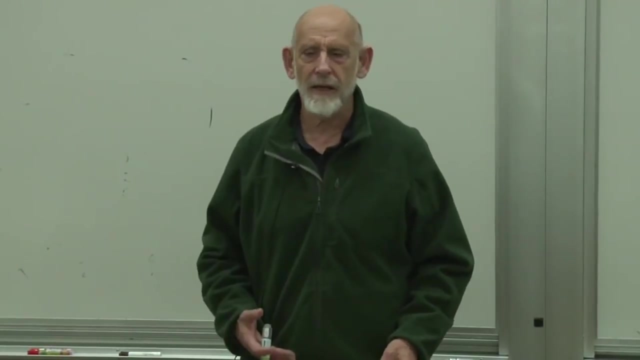 in the same sense as a source of a fluid. Magnetic fields have no sources. At least magnetic fields have no sources, No sources that we have confirmed by experiment. If magnetic monopoles are discovered, then we will have to backtrack on this And everybody fully expects that they do exist, but they're. 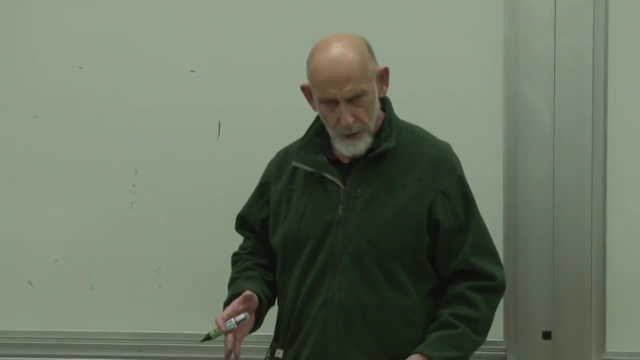 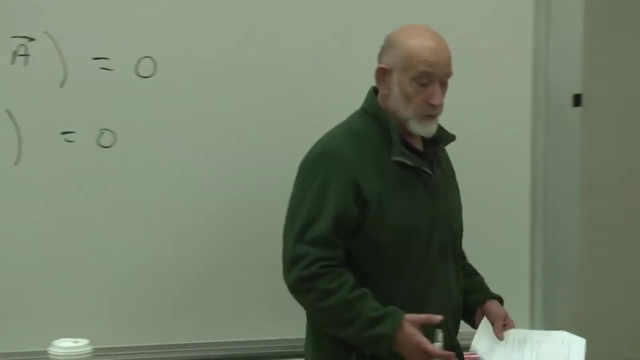 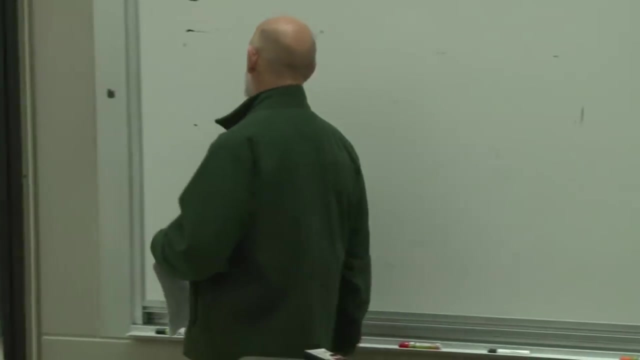 probably so heavy that they're out of range of any experiment. So for the ordinary electromagnetic theory, which doesn't involve monopoles, charged monopoles- the source of the magnetic field is zero, And that means that the divergence of a magnetic 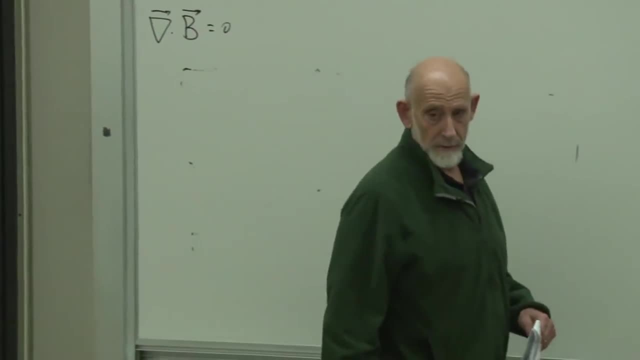 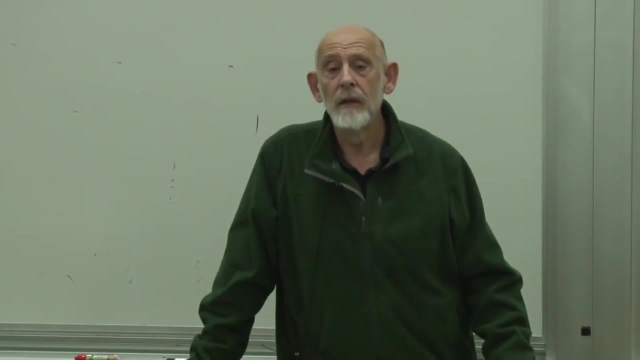 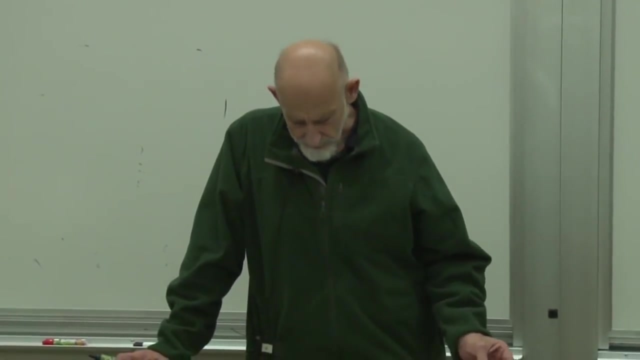 field is equal to zero. What would these magnetic monopoles be? Just as an aside, What would it be? Yeah, You say, everybody thinks there are some, but there are very. Yeah, I know. I mean most-most unified theories of field theory which contain charged particles. and so forth-. I'm sorry ーヾ. Eternal one-topzing夺 or fast blijante declarations. Yeah, Thank you salt —, Mphh, Mphh In the last two or so sheer numbers. an perturbation conflict over this theory in B, and in B is essentially labeled B. 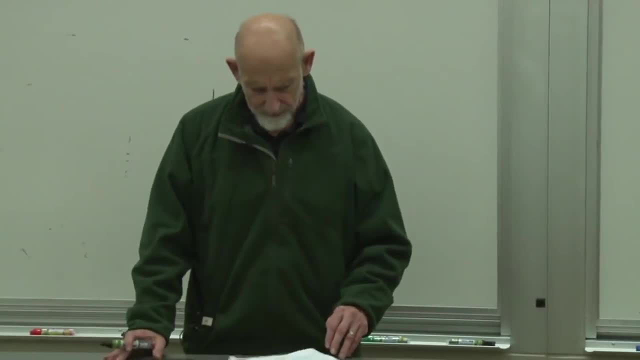 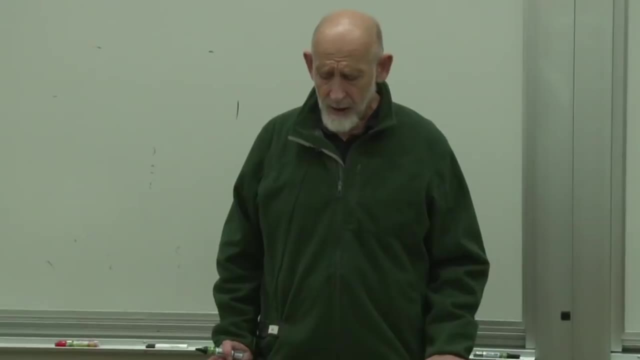 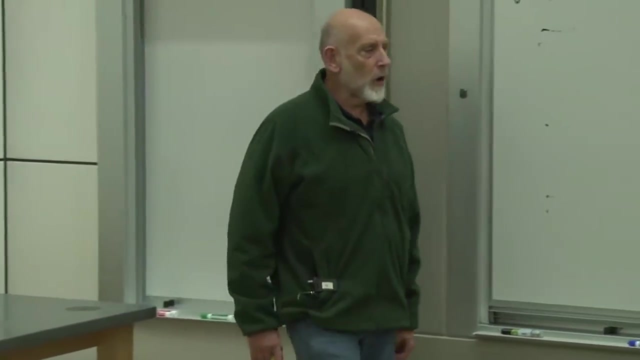 also contain. this is not the time for that. let's not try to get into it. they would be magnetic monopoles, which means what is? alright? let me tell you what a magnetic monopole is. you all know that there are magnets and that magnets have two poles. 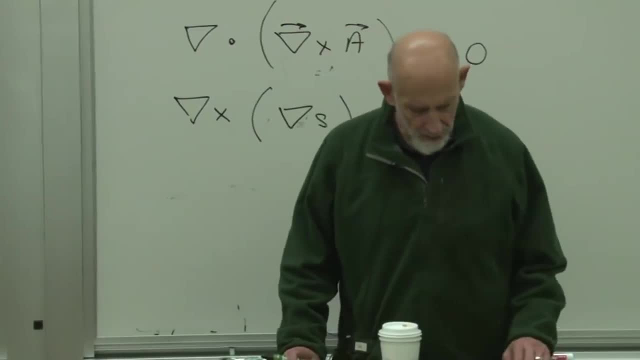 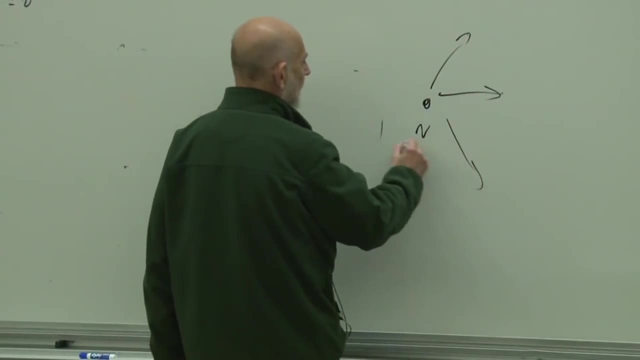 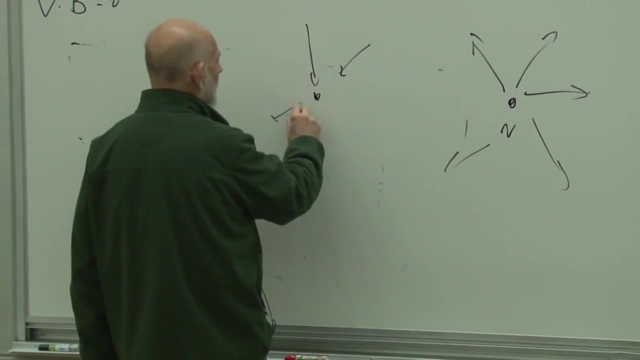 a north pole and a south pole. okay, the north pole is a point that the magnetic field comes out of, like that. the south pole is a field that the magnetic field sort of flows into. so offhand it looks like the north and south poles of a magnetic, of a magnet. 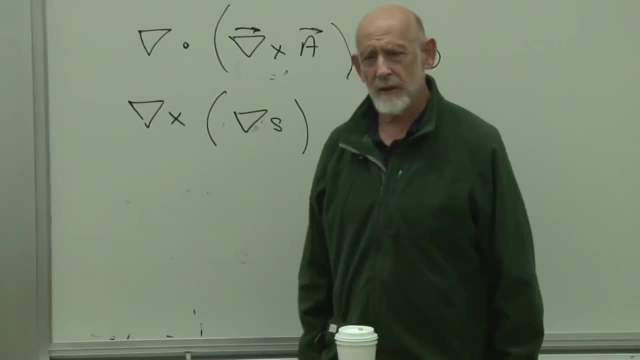 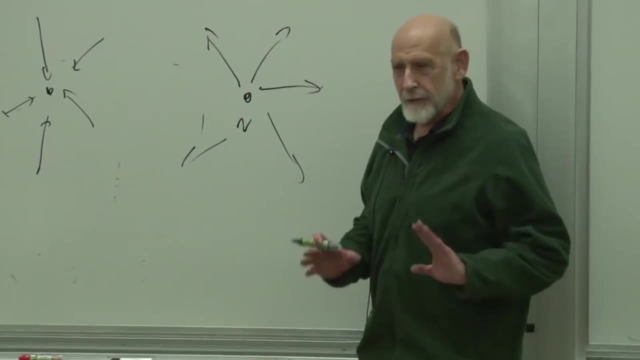 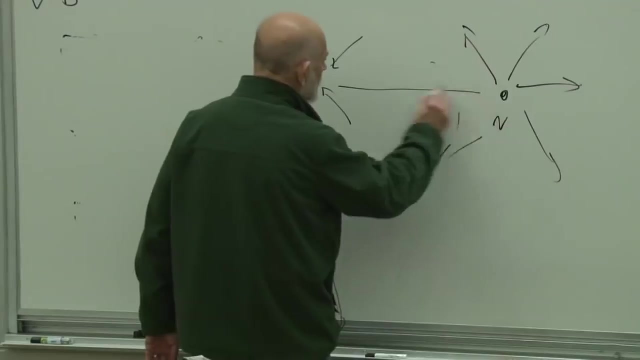 are sources of the magnetic field, meaning to say that the divergence is non-zero at the magnet, at the at the point of the poles. but if you really look at the field carefully, it doesn't look like this. what it looks like is: the field comes in here, flows along the magnet. 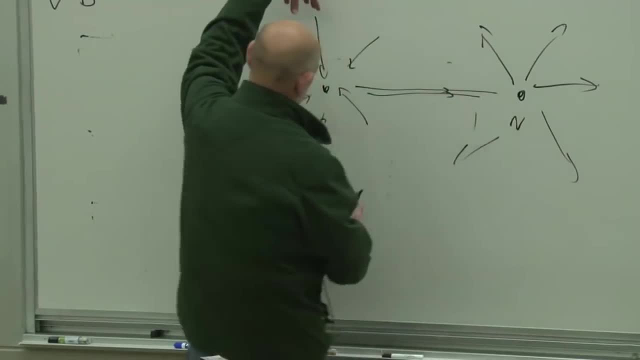 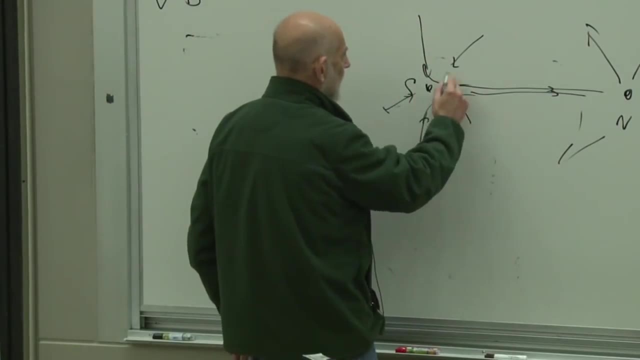 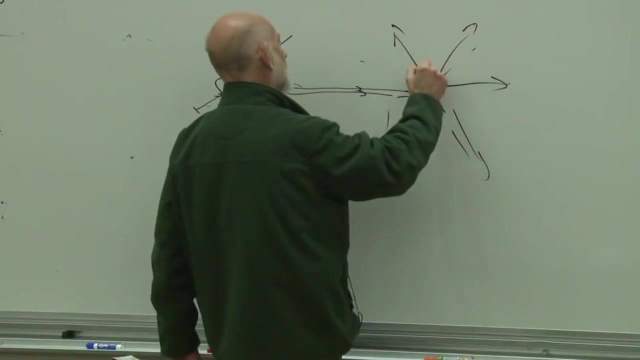 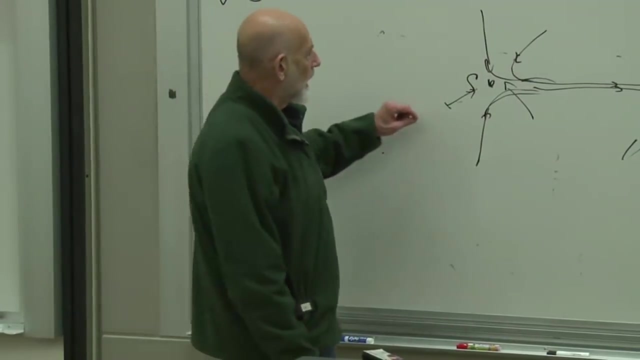 if there's a magnet between here and here, flux lines, magnetic field lines come in to the south pole and bend around and go out the north pole. so there is no net source. whatever comes in, it's as if you had a fluid that appeared to come in over here, go out over here, but there was a secret pipe between them. that allowed the fluid to go from one to another, then you would say no, there was no source and the divergence of the fluid would really literally be zero everywheres. the same is true of the magnetic field. electric fields are different. charged particles don't need to have a pipe of electricity. 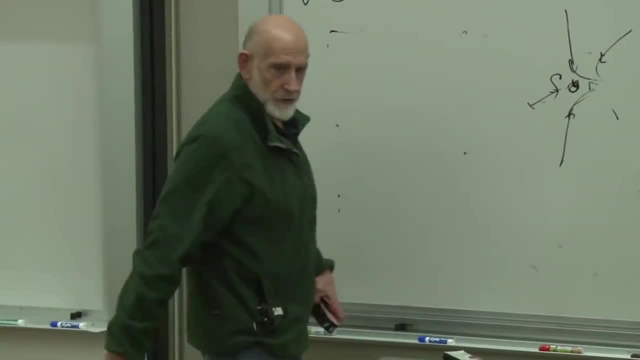 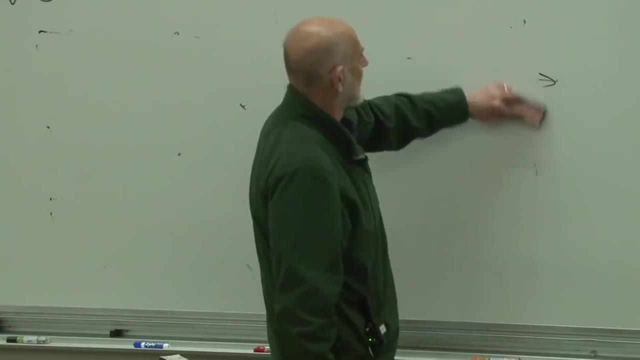 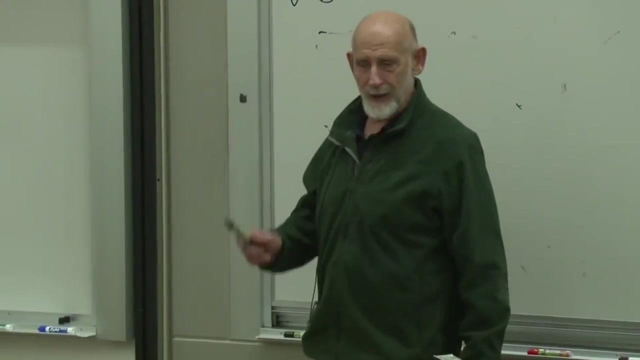 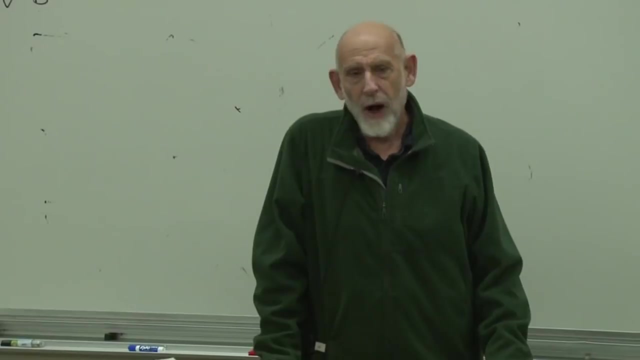 they don't need to have electric field between them. they are the sources of the electric field: electrically charged particles. okay, so the magnetic field is divergence free- that's the words that we would use for it- or that it has no divergence, and from that, why we would want to do this is another question. 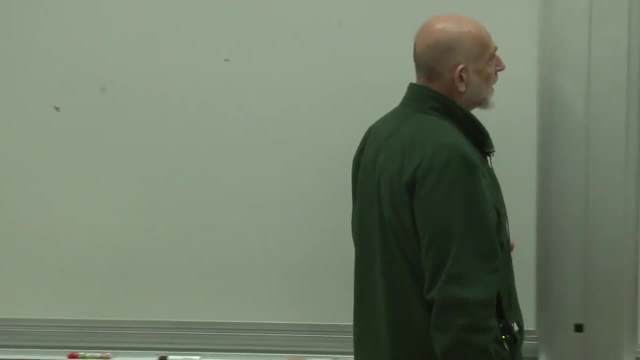 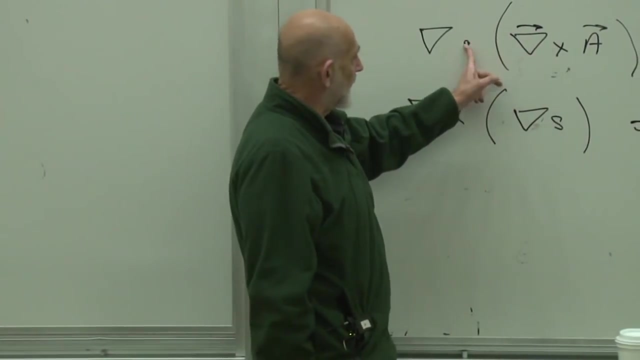 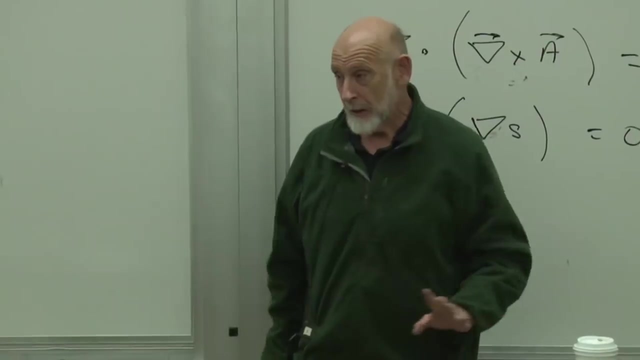 but we can do it. what we can do is we can say: well, this if and only if, statement: anything which has divergence zero, anything which has divergence zero- here's the thing that has divergence zero- is itself a curl of something. that's the harder part of the theorem. 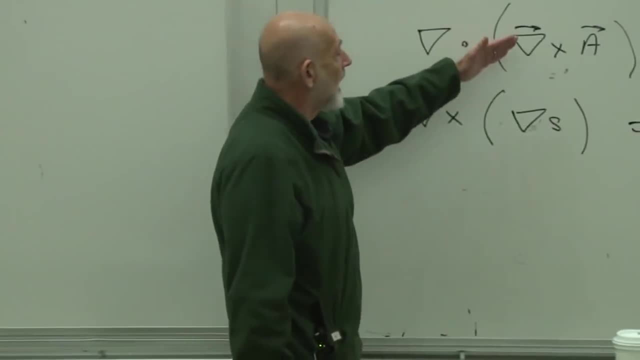 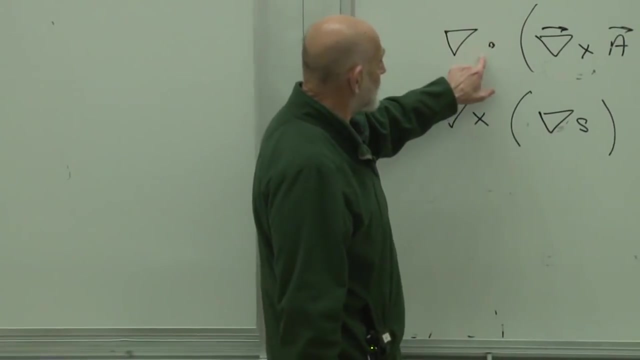 to show that anything. as I said, the easy part of the theorem is say, take a curl and then take its divergence and prove that's zero. the harder part is to say: I have a field whose divergence is zero, therefore I can prove that it itself is a curl. 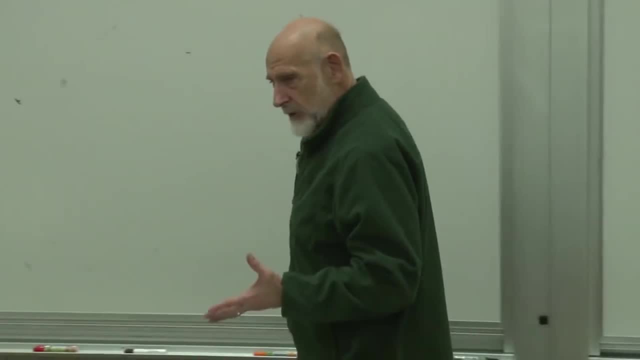 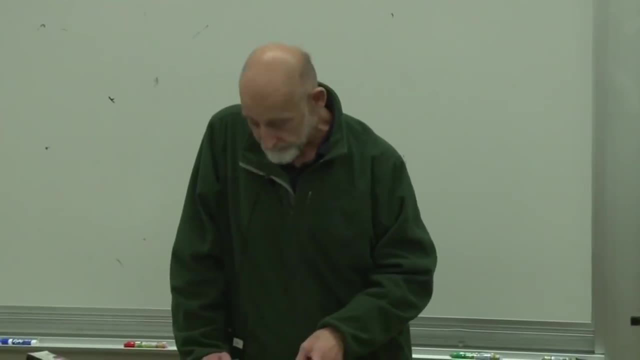 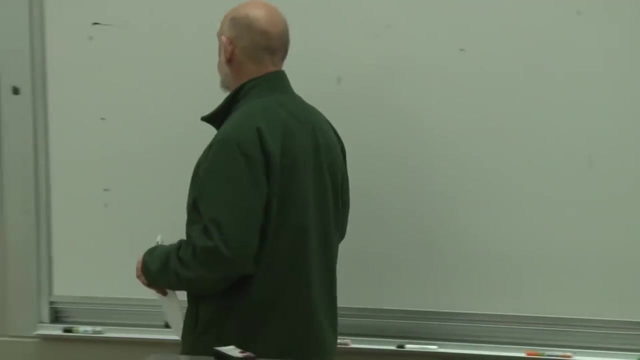 so it follows from this if, and only if, statement that the magnetic field can always be written as the curl of something. the thing that it's a curl of is called A, it's called the vector potential, and exactly why we would want to do this is, at this moment, unclear. 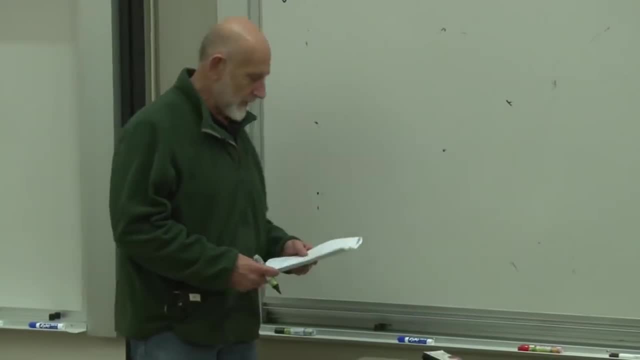 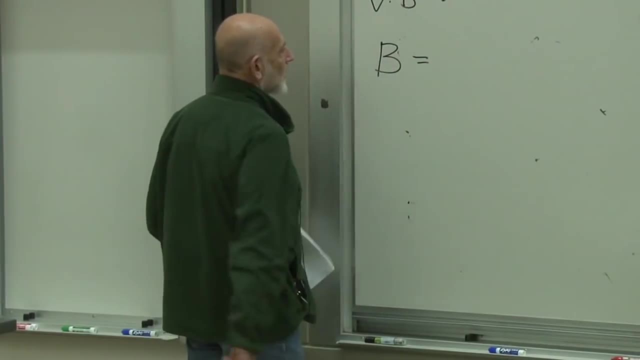 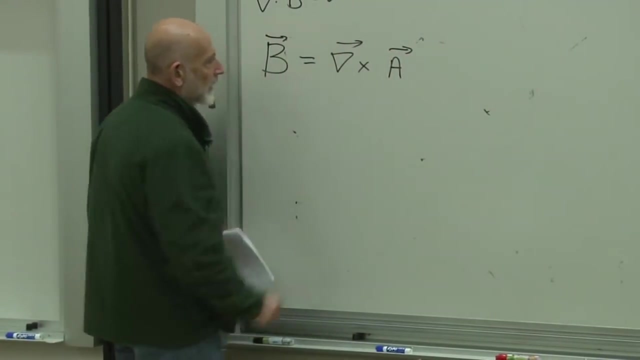 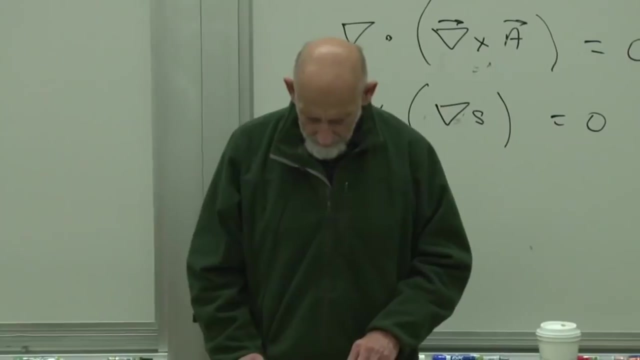 there will be. I think by the end of the evening we will have explained why one does this, but we can do it. we can always write that B is the curl of something that we'll call A. A is also a field. A is also a field, but there's a funny glitch about it. 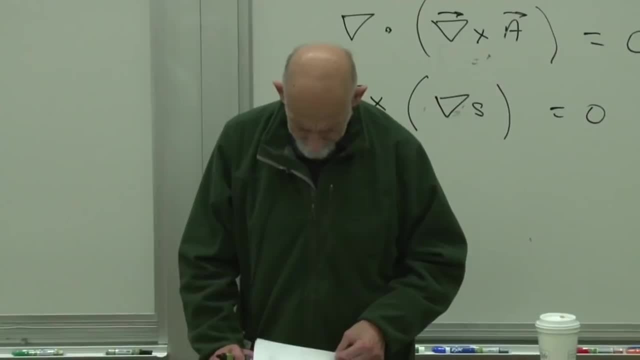 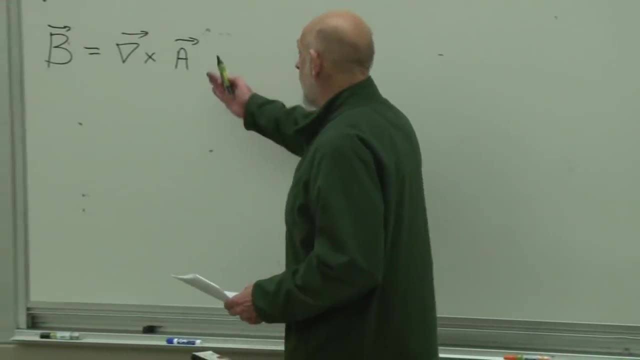 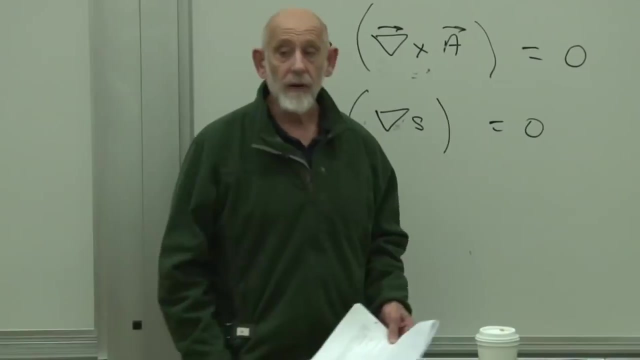 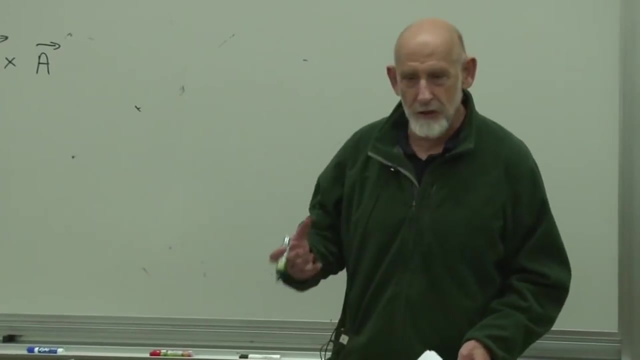 we're going to see soon enough. what is the glitch? the glitch is that A is not unique. A is not unique. there are many, many A's for a given magnetic field. there's not a one-to-one relationship between them, given a B field- and B, of course, is the physical thing. 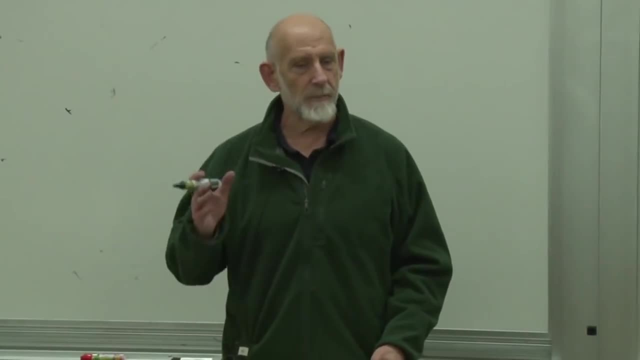 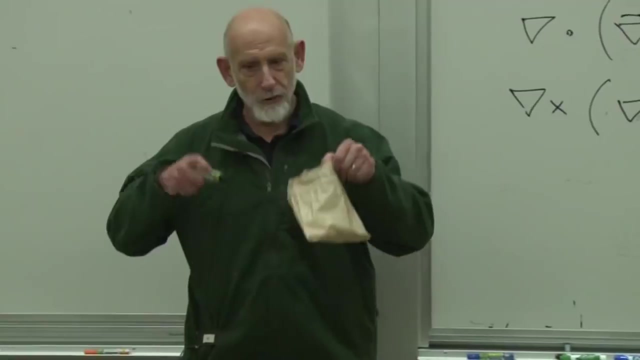 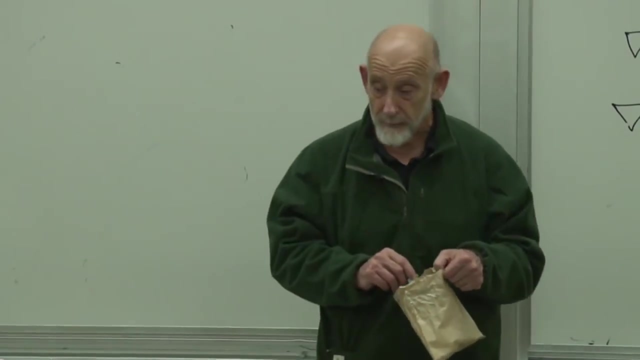 the forces on charged particles are associated with the magnetic field. if you know the magnetic field again in this bag and a charged particle comes into it, then the force on the charged particle in the bag is only sensitive to the magnetic field in the bag. a charge out here. 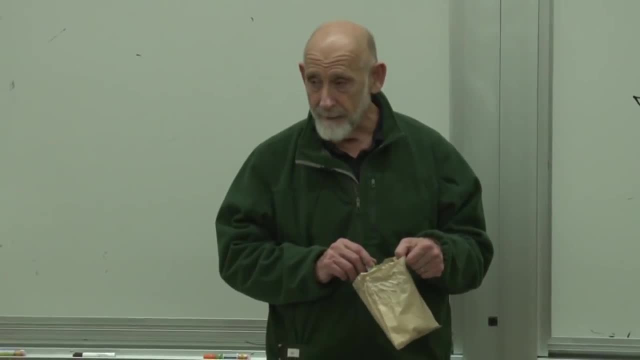 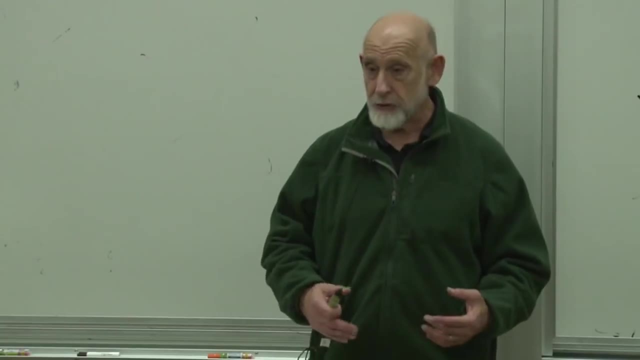 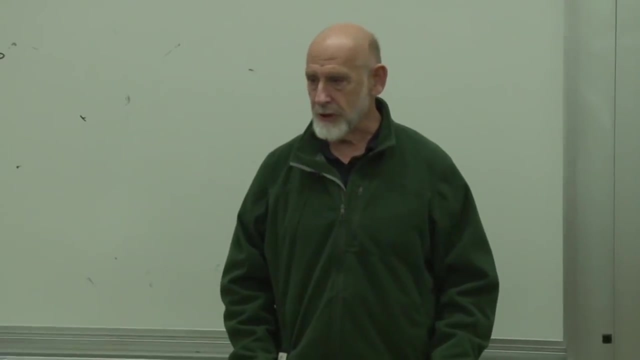 does not experience a force due to the magnetic field in the bag, and so that's a local connection. the magnetic field is measurable. in that sense it's a real thing that you can measure by an experiment, and you can measure it locally. A is not in the same sense a real thing. in other words, you can't measure it locally, and one way to observe that is by realizing that A is not unique. B is the real thing that has a measurable meaning, and A is only defined by the rule that, whatever it is, its curl is equal to the B field. 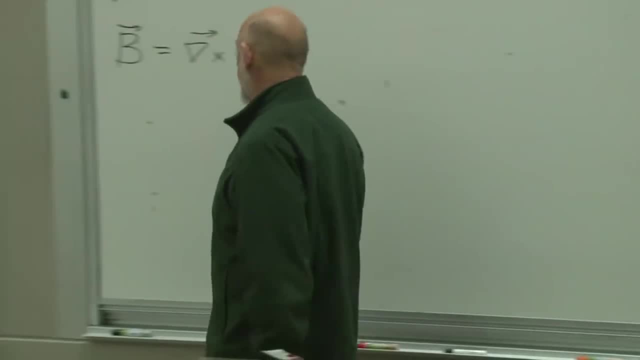 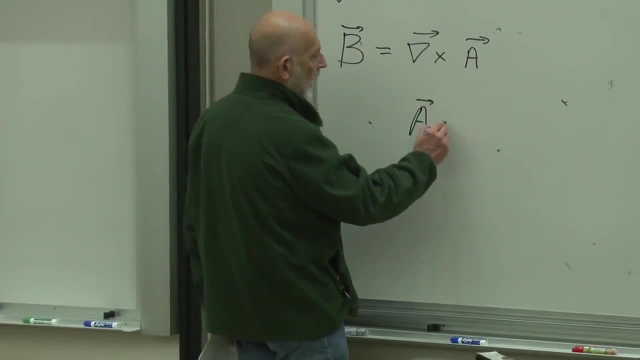 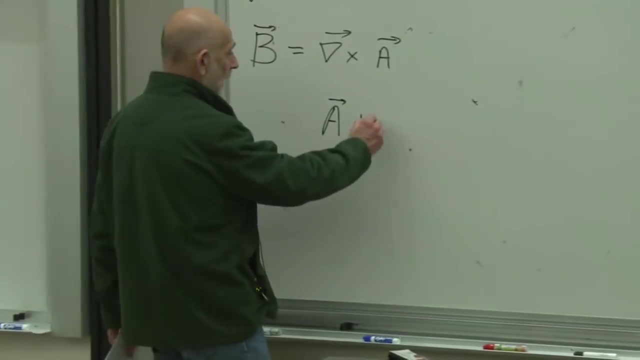 to what extent is A unique? well, I'll tell you right now: it's not. and here's the way to show it. supposing you take A, whatever it is, and you add to it a gradient. supposing you add a gradient of anything, let's call it S. 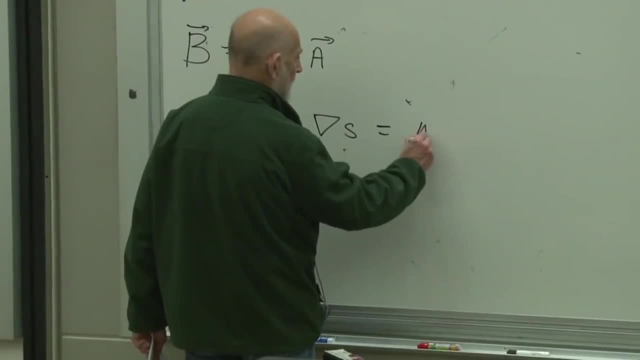 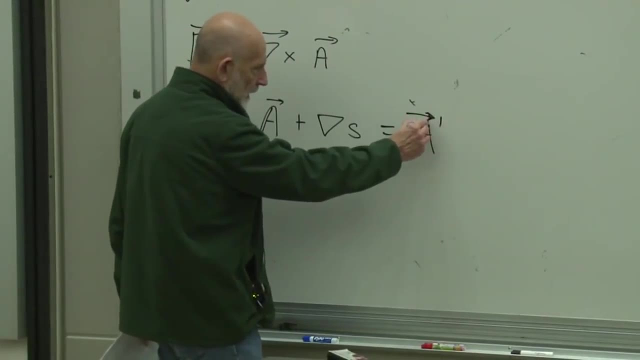 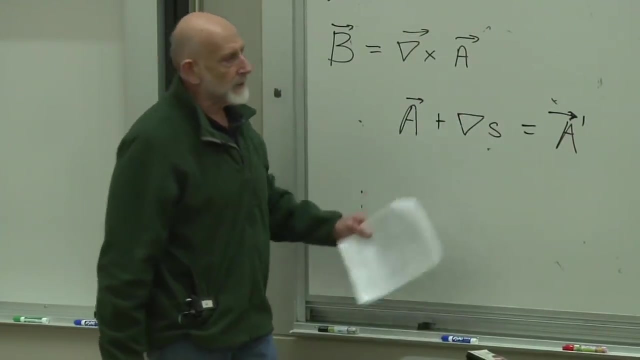 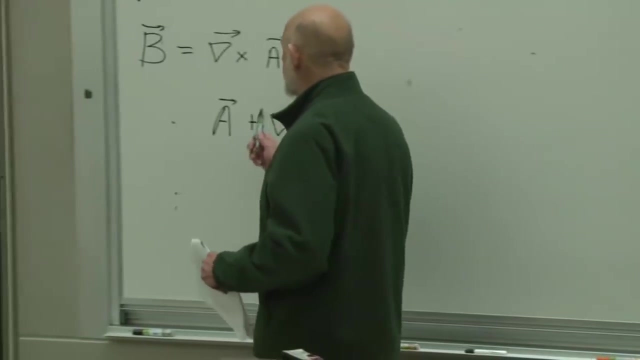 and call that new thing A prime. then what's the curl of A prime? the curl of A prime will be equal to the curl of A plus the curl of the gradient. but the curl of a gradient is always equal to zero, so that means that A is undefined. 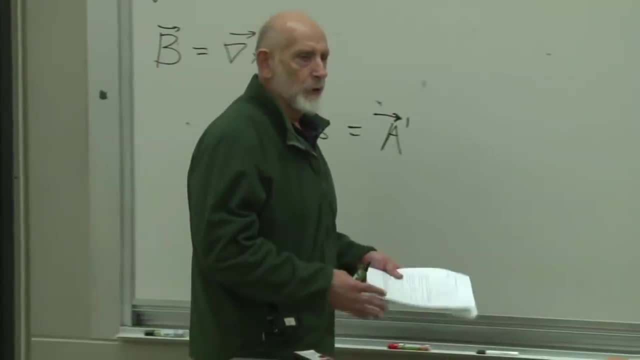 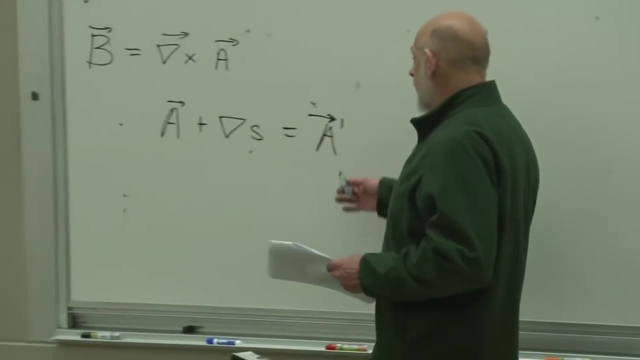 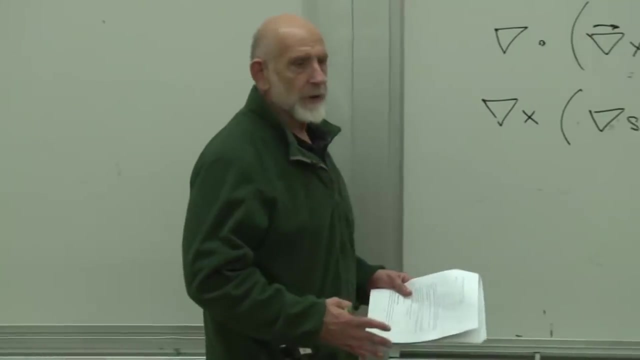 or ill-defined, up to the addition of the gradient of a scalar. that's a kind of transformation on the A field which should have no physical effect on the motion of charged particles. why? because the motion of charged particles is determined by the magnetic field alone and also the electric field. 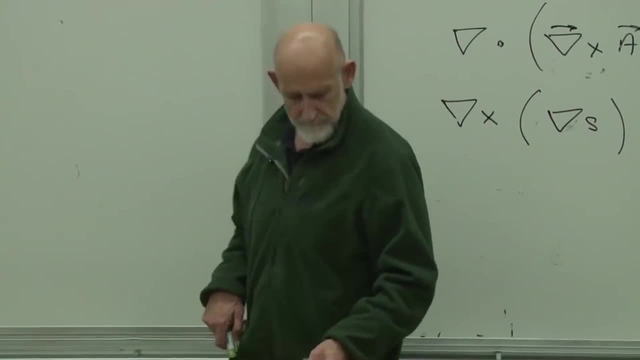 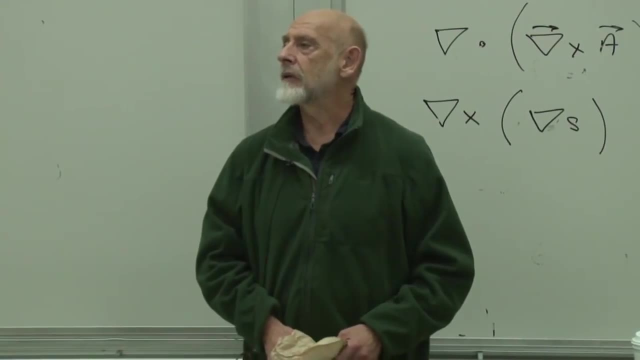 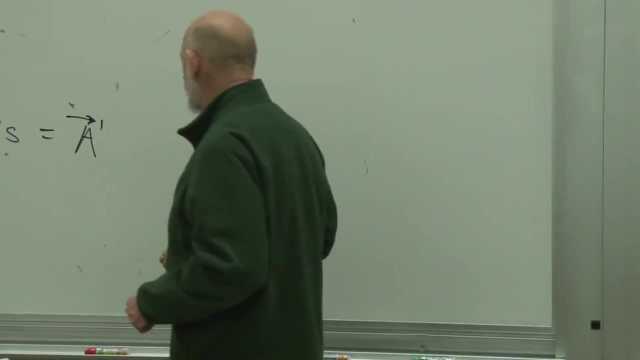 but let's shut off all electric fields. yeah, is that the complete description of of the non-uniqueness that is? you've shown that, yeah, yeah, we've shown, yeah, and in fact, if there's any A prime such that delta cross A prime is B. 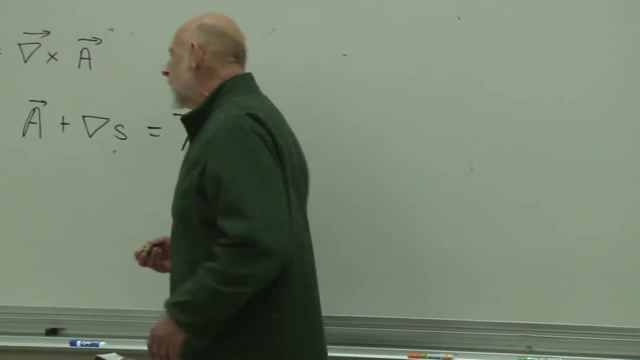 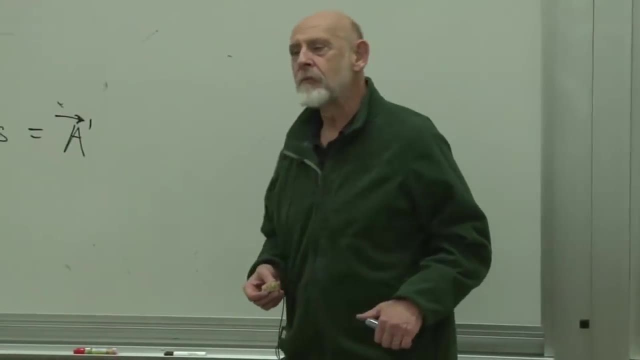 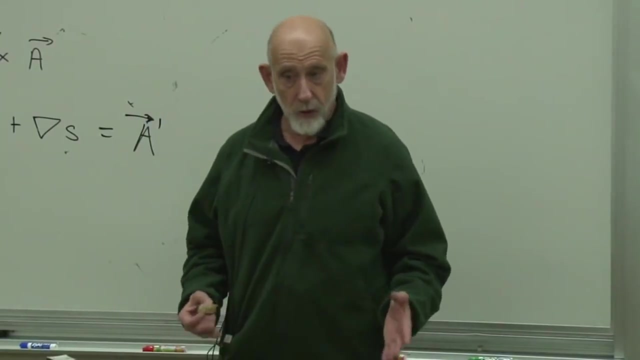 then A prime has to be of that form. yeah, okay, these if and only if, statements are enough to see that. okay, so, plus a constant. so this is a transformation that you can do on the vector potential. A is called the vector potential. it doesn't change anything. 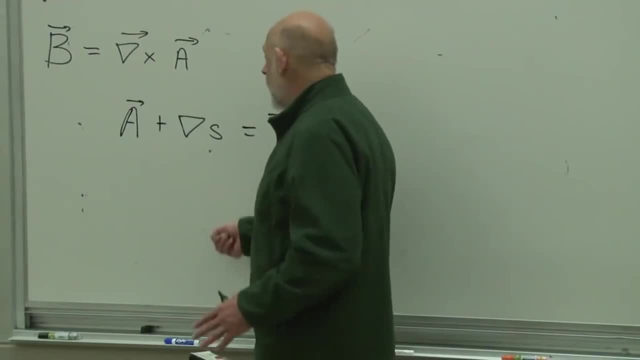 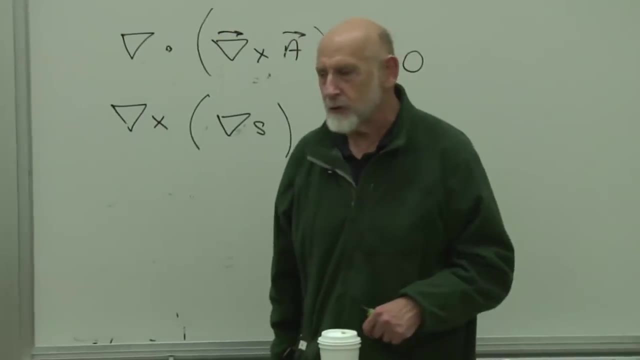 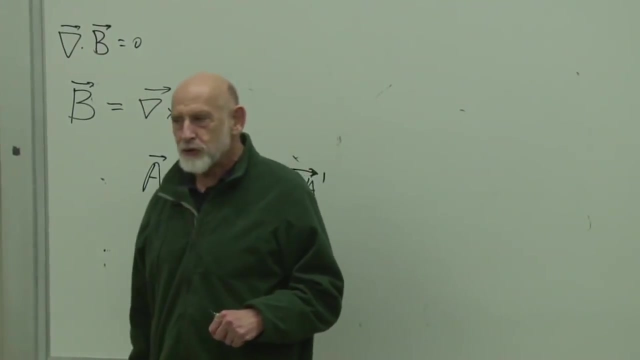 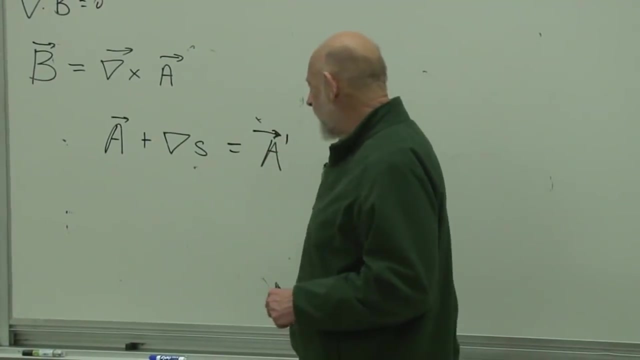 that transformation, a transformation like this, is called a gauge transformation: G A, not gouache. anybody who says gouache fails the course. there's always somebody who says gouache, it's a gauge and it's not a gouache transformation. it's a gauge transformation. it's a gauge transformation of the vector potential. 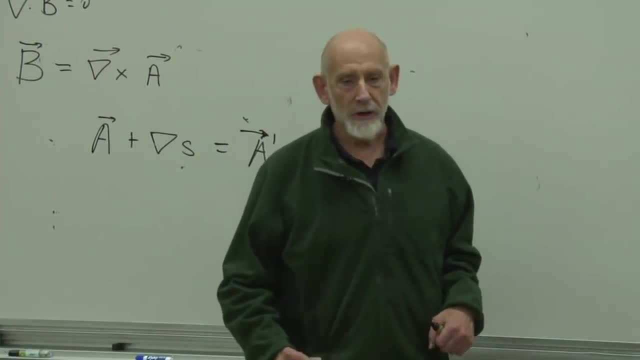 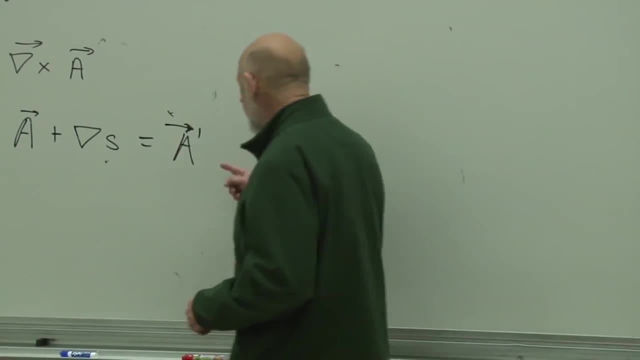 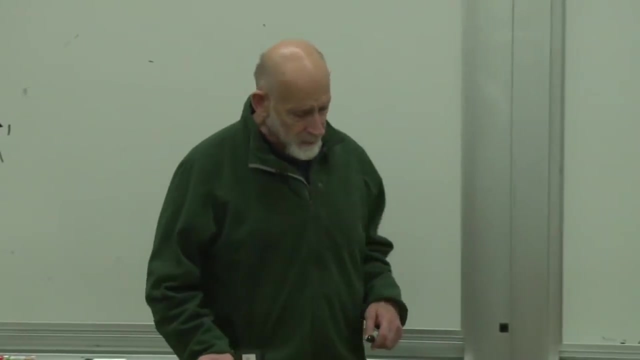 by an arbitrary function, S, and the words that would go with this is that the physics, the physical forces on charged particles are gauge invariant. the magnetic field is gauge invariant. it doesn't change when you change the vector potential this way. that's called a gauge transformation. where did the word gauge come from? 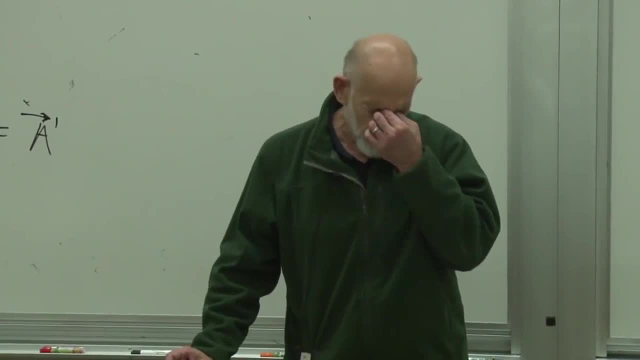 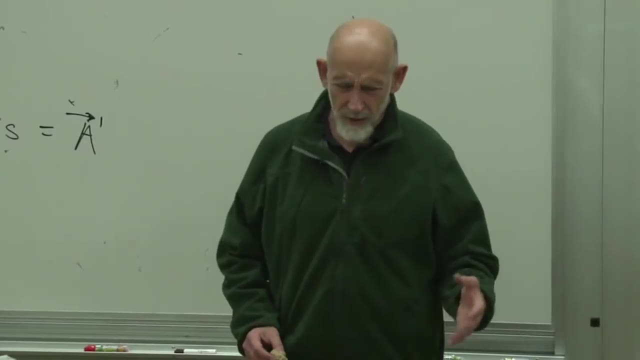 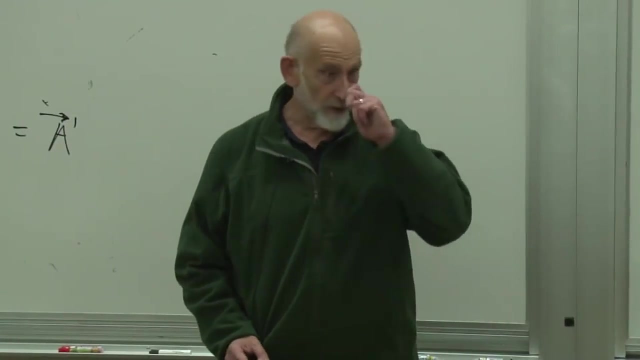 it's a historical glitch that at one time it was thought that all of this had to do had something to do with ambiguities in measuring lengths at different places. it doesn't. that has nothing to do with that and or gauging lengths in different places. 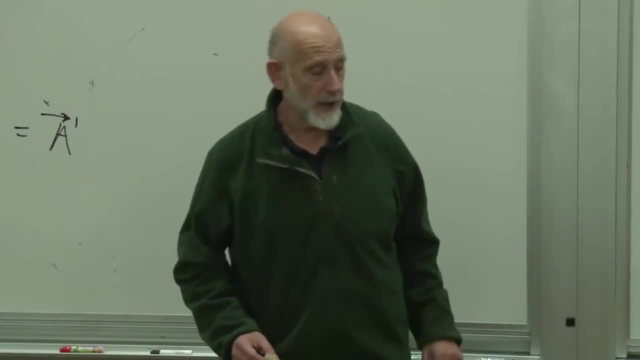 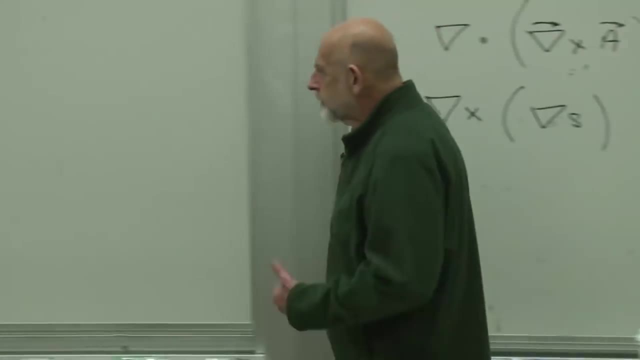 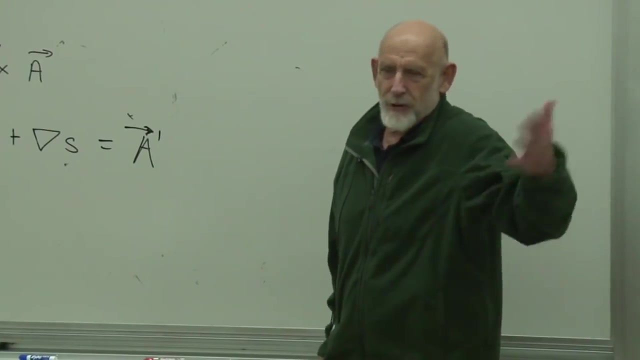 right. it has nothing to do with that, and so the terminology gauge is: a is a. you know it's not a. I don't think the word is anachronism. anachronism means old fashioned. it just means it came from some history that has nothing to do with the real meaning of it. 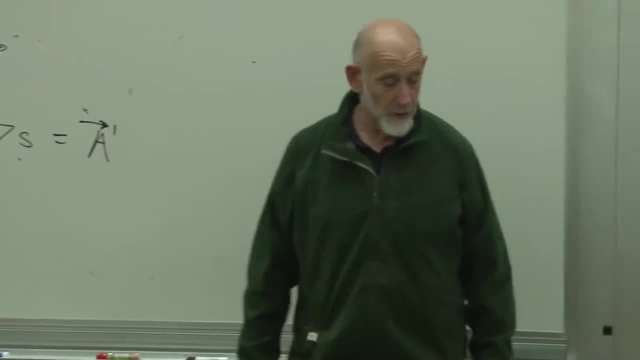 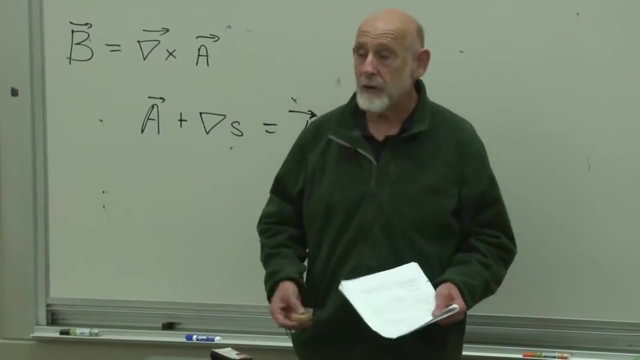 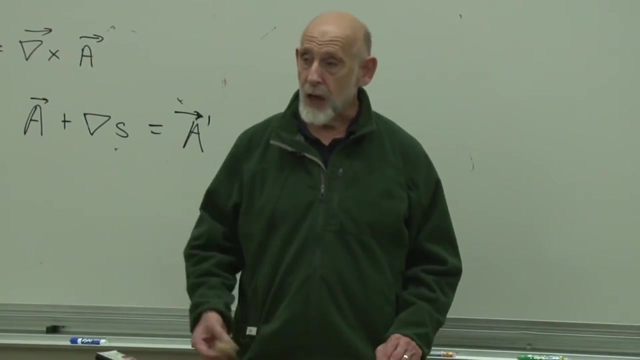 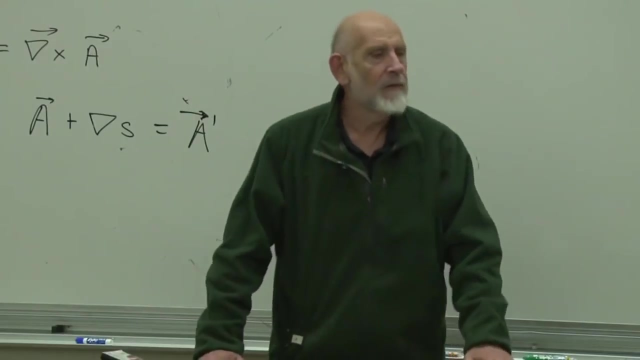 A's are sometimes called gauge fields. they're sometimes called gauge fields- fields that you can transform in this way without changing the physical character of the influence of the field. gauge transformations apply to gauge fields, so can you just clarify the definition? when you say gauge transformation, you mean specifically. 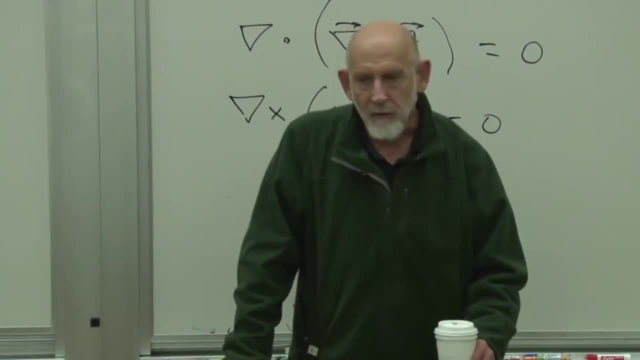 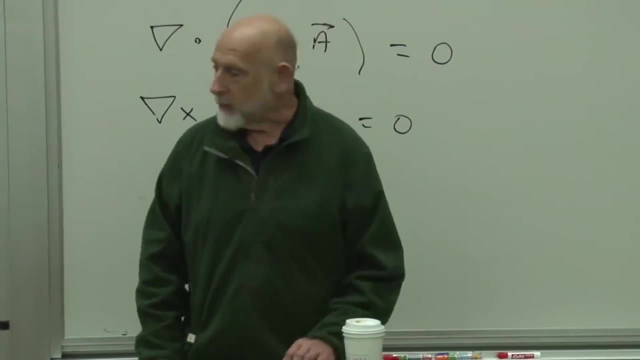 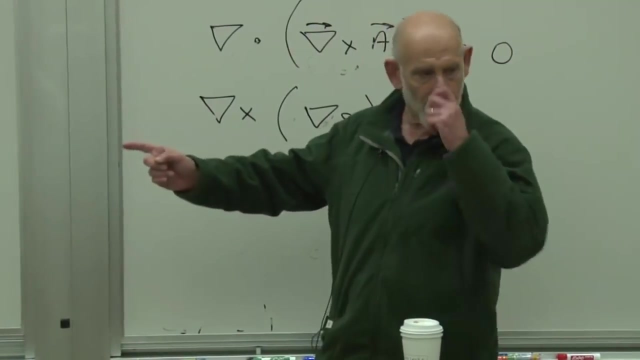 transforming A by adding an A prime. yeah, now there are generalizations of this to other kinds of fields, but when thinking about things like electromagnetism or Yang-Mills theory, this is what's meant, or approximately this is what's always meant, for electromagnetism. 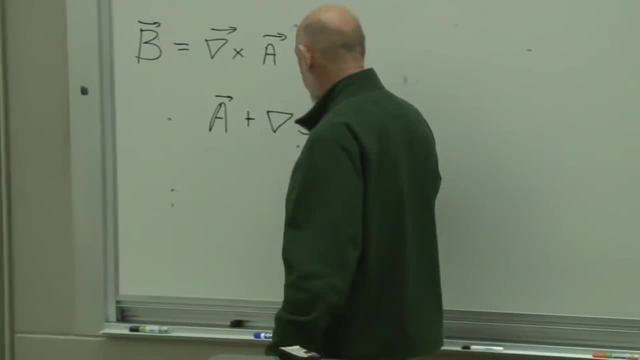 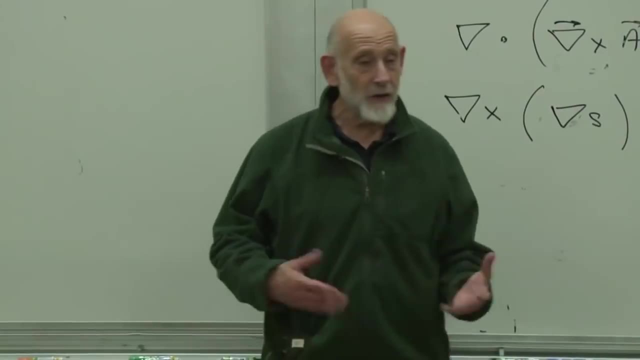 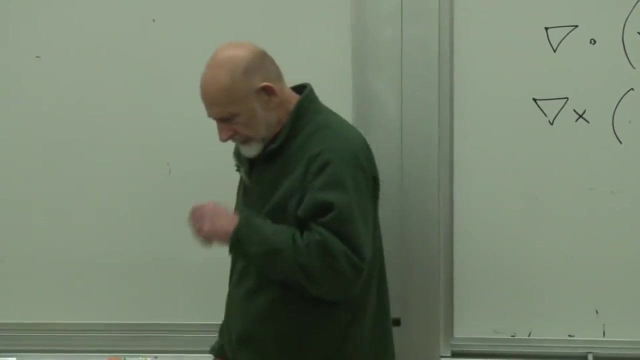 this is all it's meant. so the question comes up: if this A field is so non-unique and really doesn't have any physical meaning in a localized region of space, why do we introduce it? we introduce it because without it, we couldn't describe the 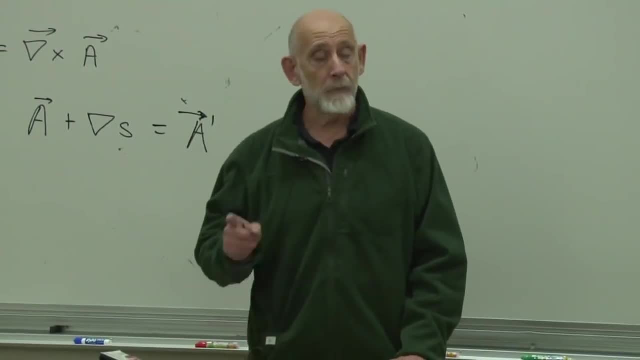 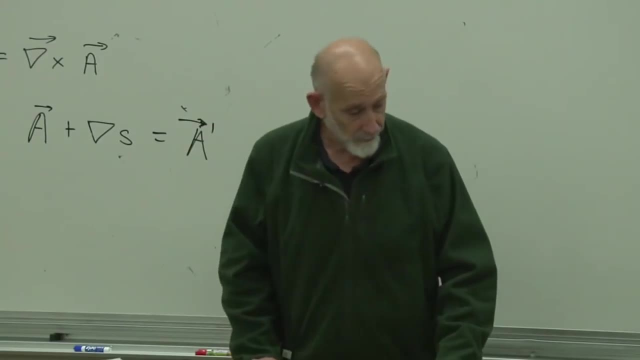 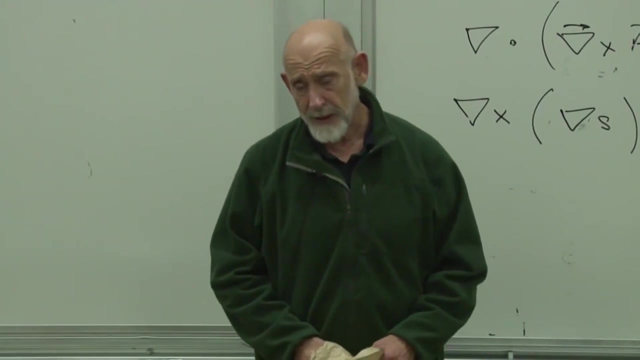 the motion of charged particles using the principle of least action, Lagrangians, Hamiltonians and so forth. yeah, is there an underlying physical reason why we have to escape freedom? well, yes there is, but I think the best way to get at it is to work with it a while. 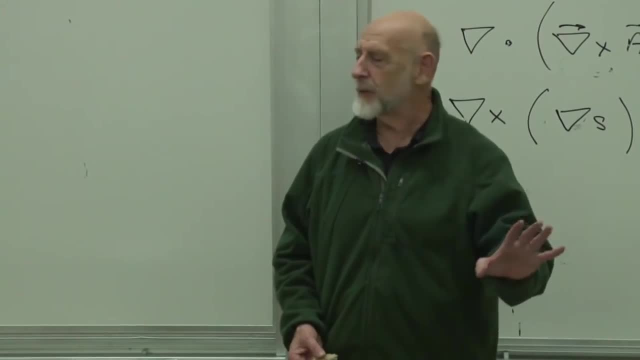 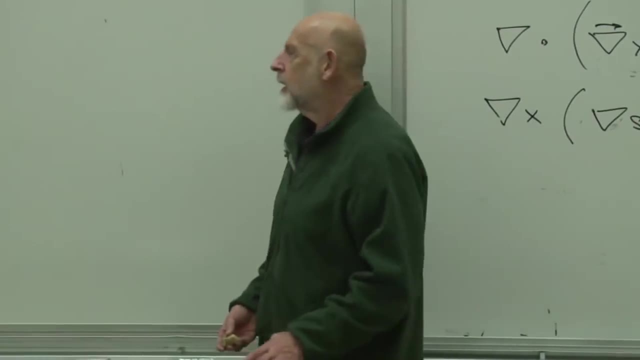 and then come back after we understand it a little better and say, by the time we understand it a little better, we won't need to just accept it for the time being that this is important and we'll eventually see why it's important. okay, but for now it's. 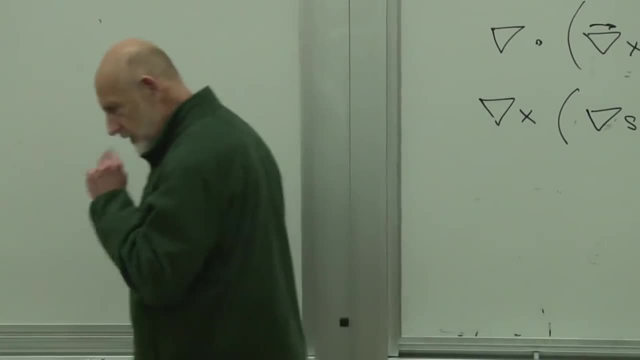 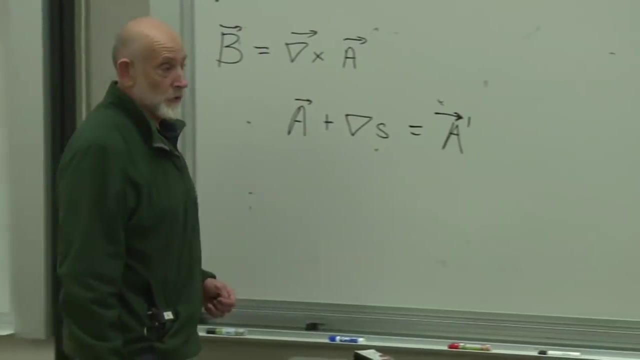 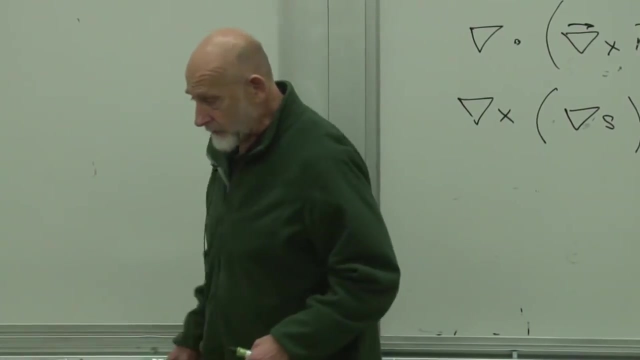 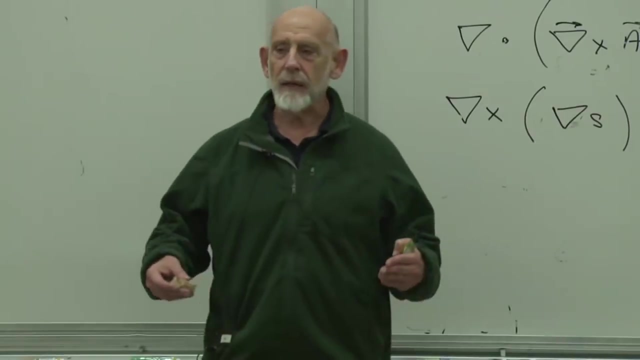 it's just a mathematical fact, a set of mathematical facts. okay, now I've talked about the forces exerted by electric and magnetic fields on charged particles. I think it's time we wrote down that force law and, in a sense, the force law is the goal. we're going to want to write a theory. 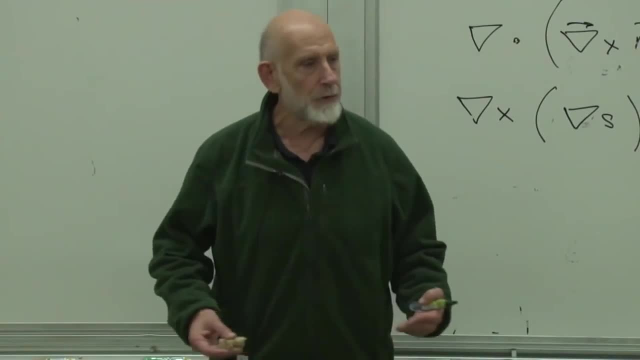 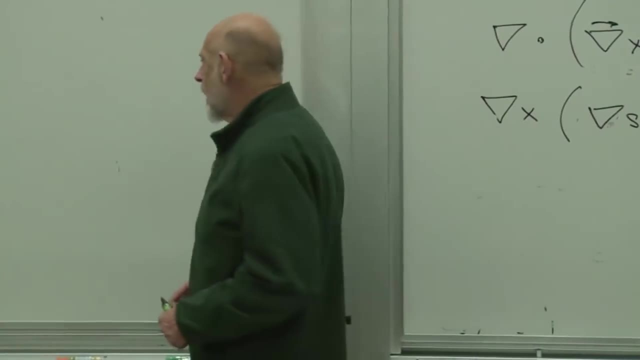 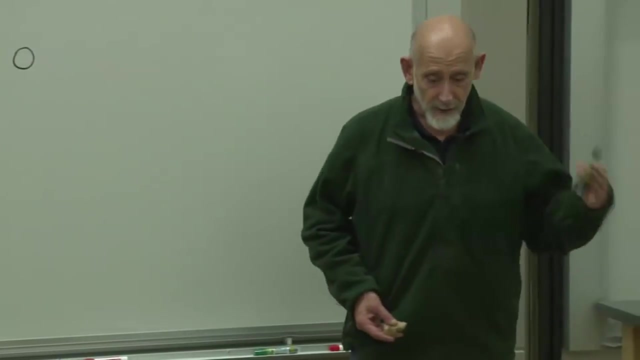 based on the principle of least action, based on Lagrangian mechanics and so forth, which gives rise to forces, which are basically what I'm going to write on the blackboard now. now, forces, by definition, are the left-hand side of F, equals mA. so on the left-hand side, 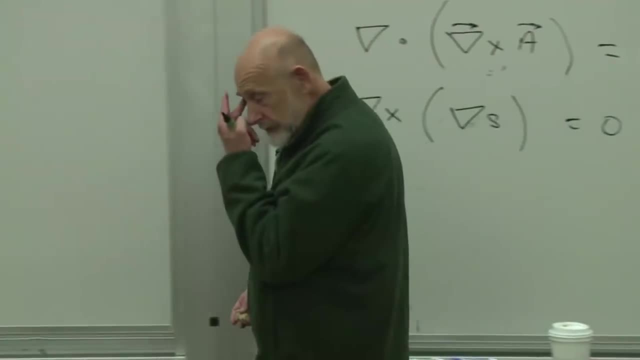 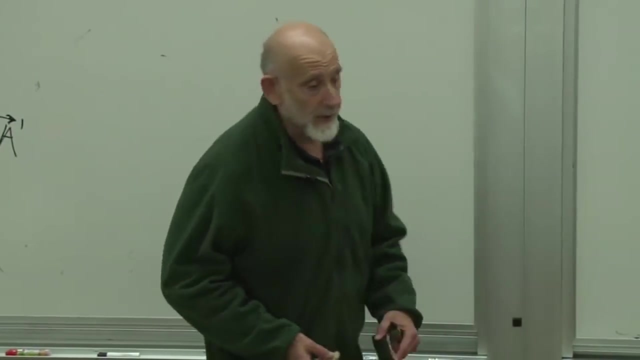 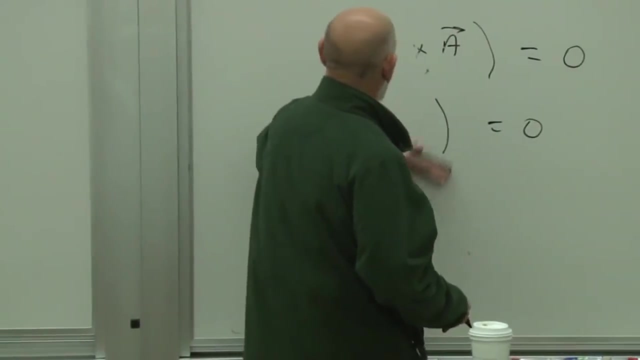 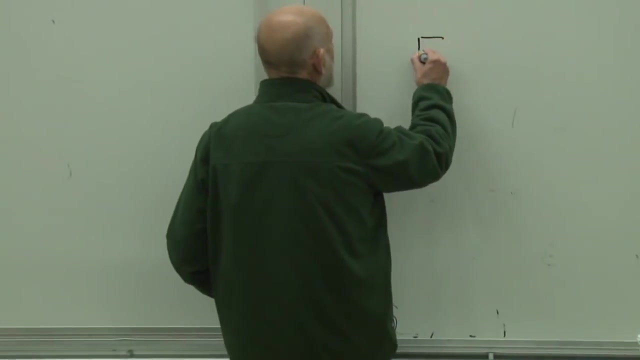 we have forces on the right-hand side, we have mass times, acceleration, but you don't know nothing unless somebody tells you what the rule for the forces are. given: a magnetic field, an electric and magnetic field, here's what the force is. F on a charged particle is first of all. 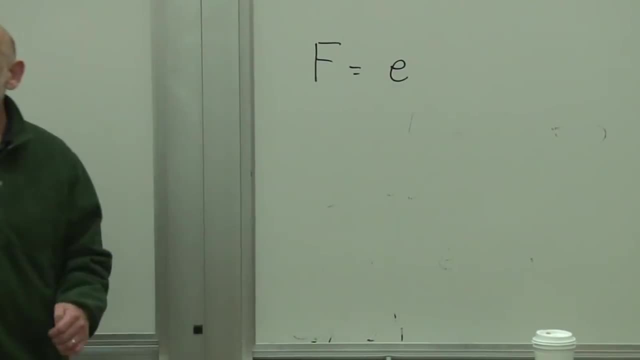 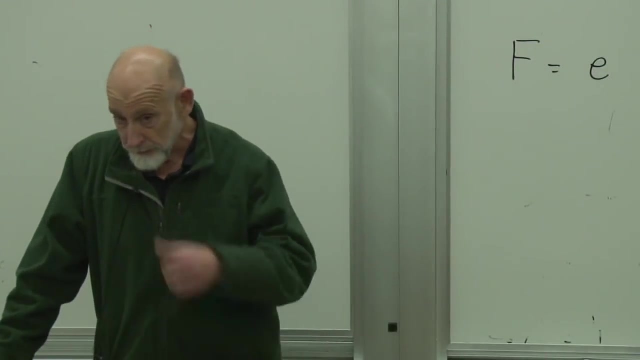 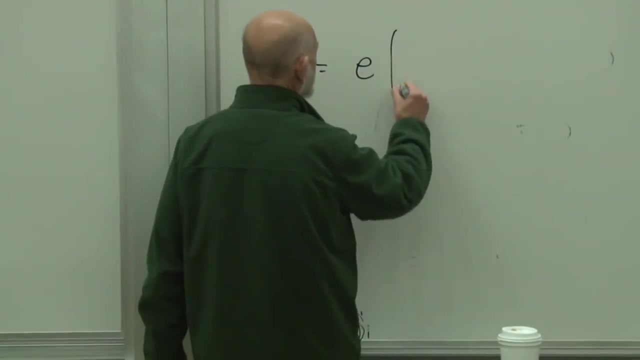 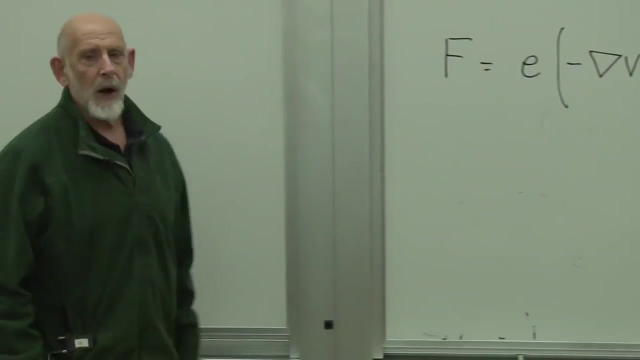 the electric charge times the gradient, or minus the gradient of a certain function. that's called the scalar potential or just the potential. it's called V minus the gradient of V. V is not quite the potential energy let's use. for the potential energy, let's use the symbol U. 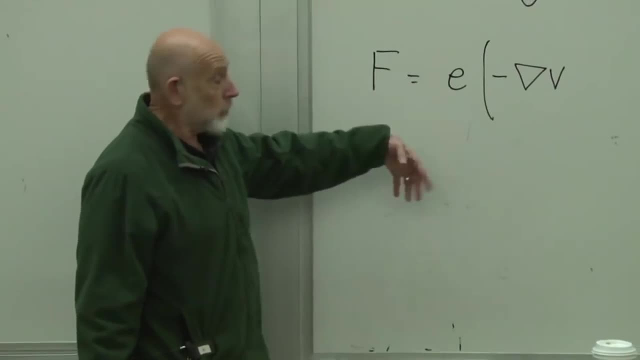 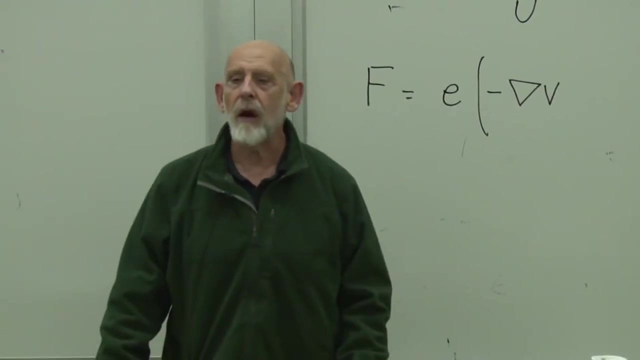 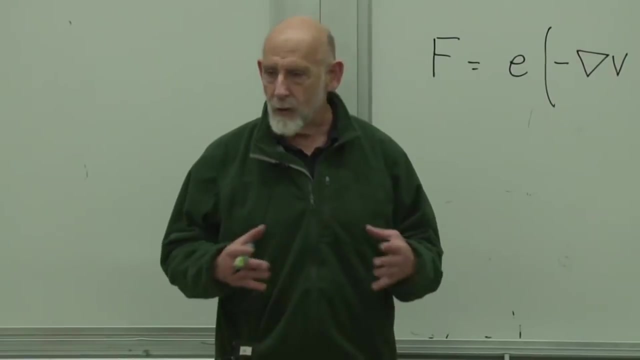 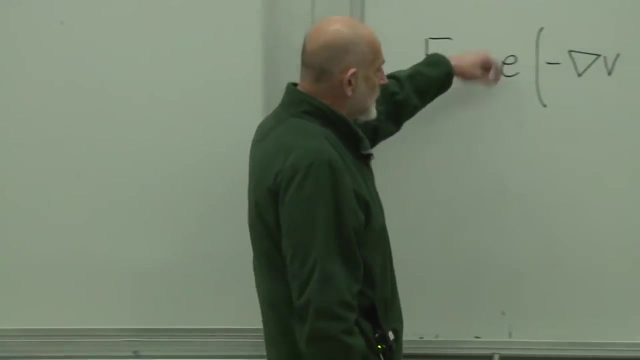 E. E is the electric charge, E is the charge of the particle, a numerical electric charge of the particle measured in some units. we're not doing. our goal tonight is not the electrodynamics, it's understanding the mathematical formalism of the motion of charged particles, but the units and so forth. 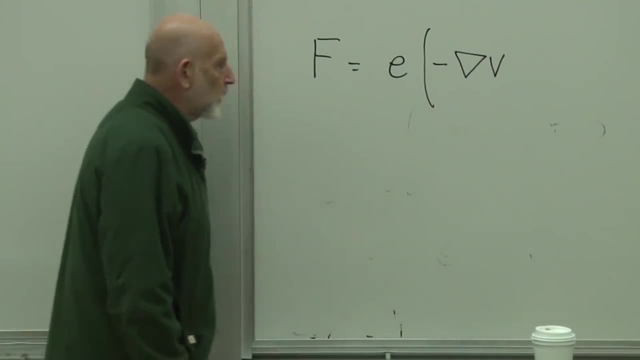 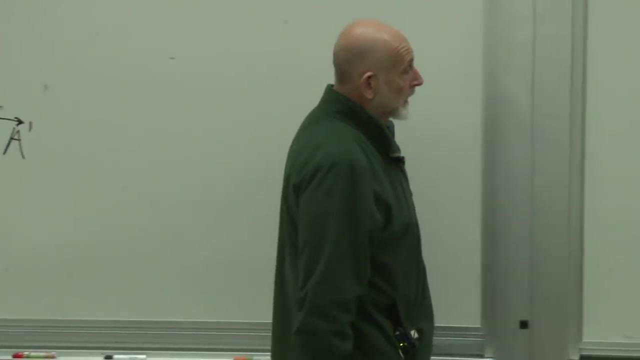 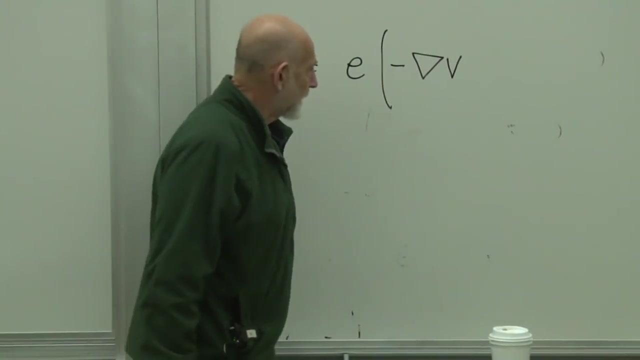 will take care of themselves. E is measured in whatever units. it takes to make the units consistent. let's just say it that way. and V is measured in volts. E is measured in coulombs. V is measured in volts. it doesn't matter. it doesn't matter. 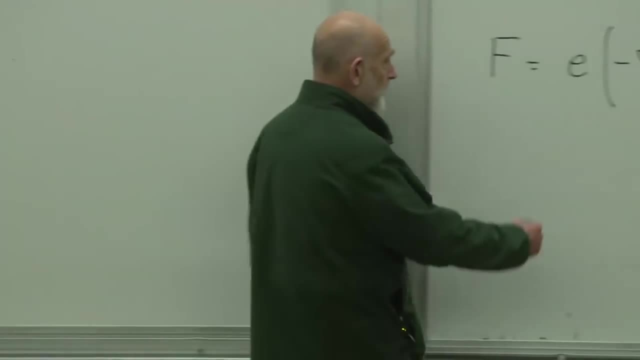 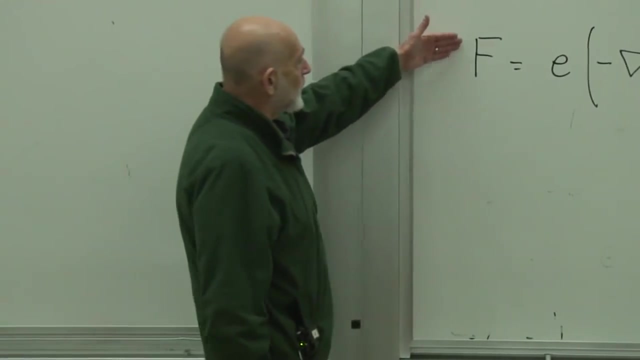 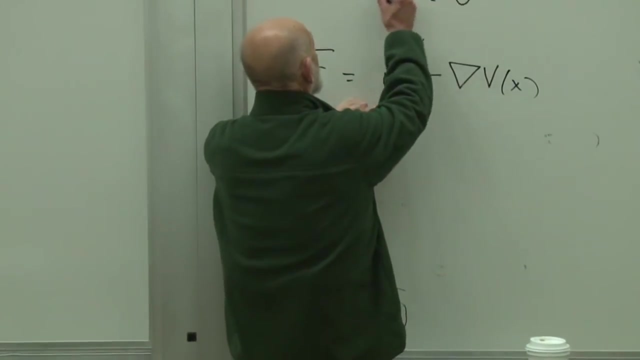 what the units are and what is V. V is a function of X. now, this is basically the same equation that we write down whenever we write that a force is equal to minus the gradient of a potential energy. it's just that the potential energy is the electric charge times V. 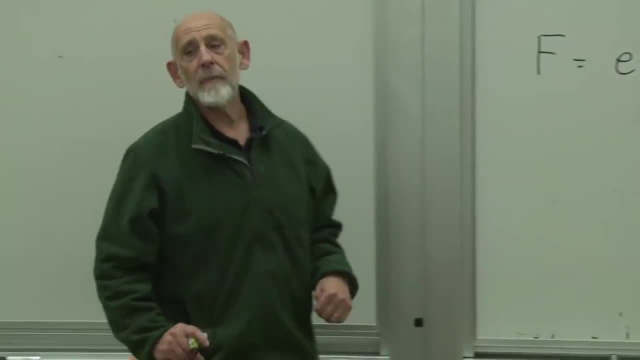 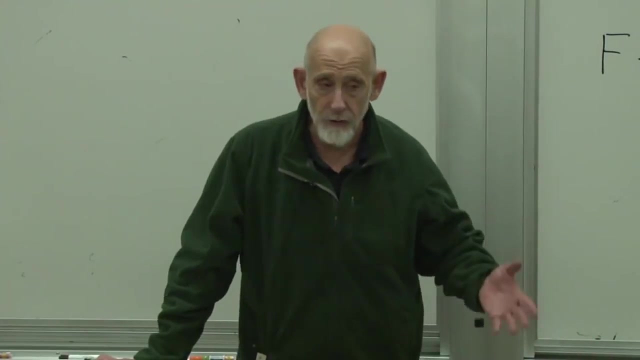 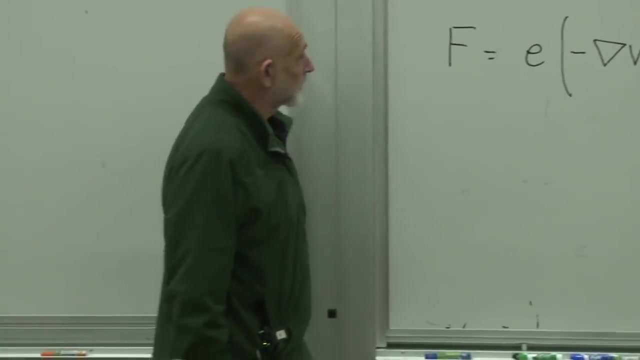 why do we bother breaking it up this way? because there are particles of different electric charge. you can have a particle of two units of charge, three units of charge, four units of charge, and the forces on them will be proportional to the electric charge. all right, the electric force. 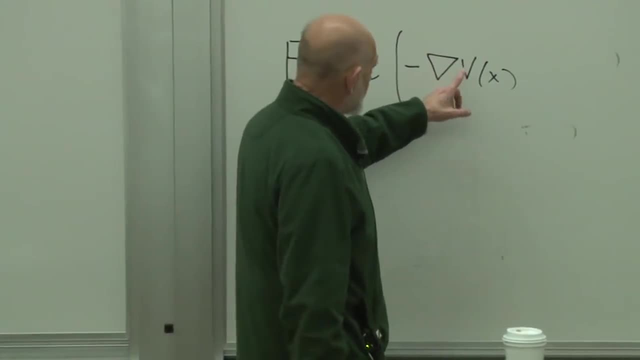 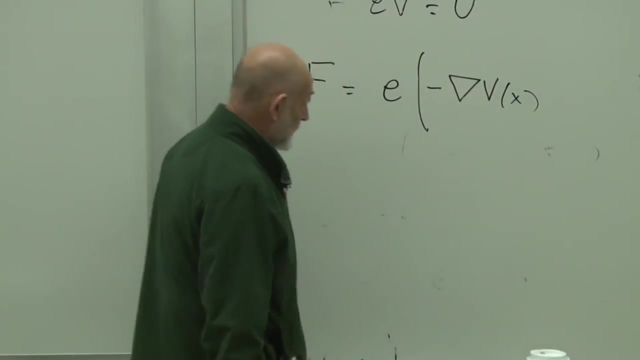 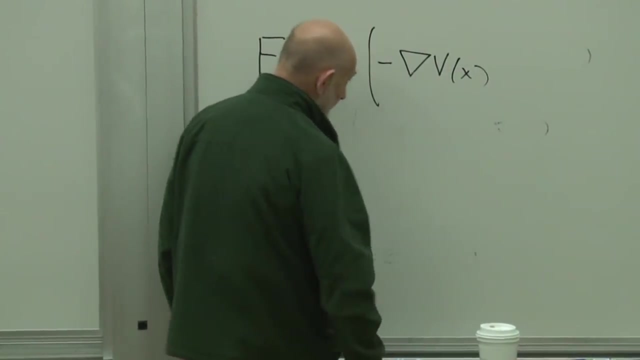 the electrostatic force. the electrostatic force is just the gradient of a potential energy, where the potential energy is the charge times, whatever V of X is. there's nothing new here. the gradient of the electrostatic potential is also called the electric field. all right, so this term here. 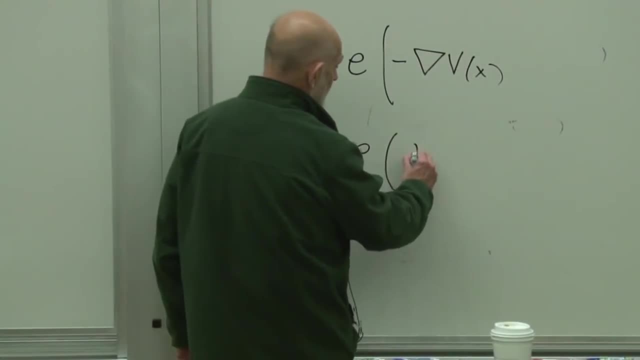 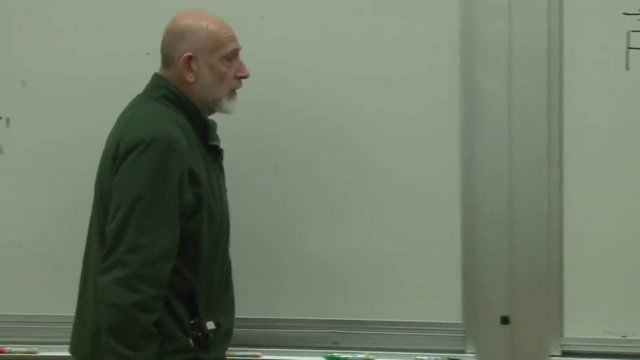 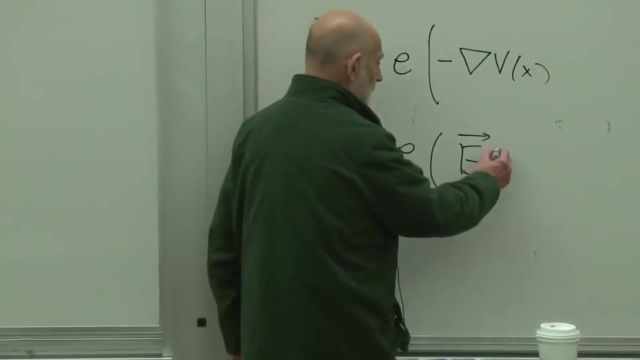 is just the electric charge times, the electric field. the electric field is a vector because the force is a vector. okay, so first of all, that's the first term and that's the easy term. there's nothing new about it at all. and E in general depends on position. 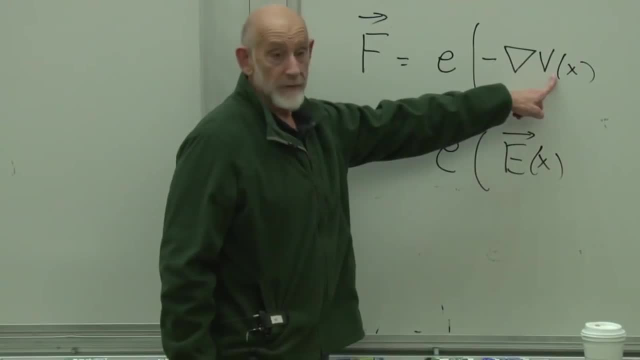 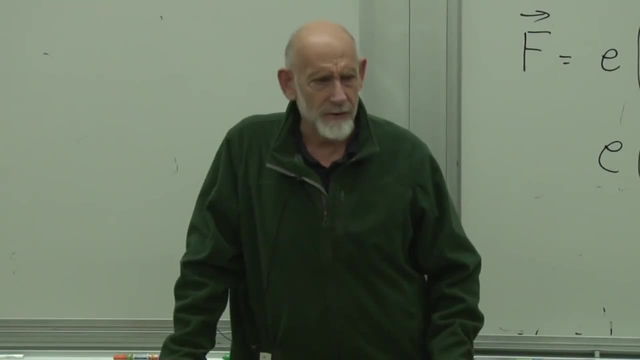 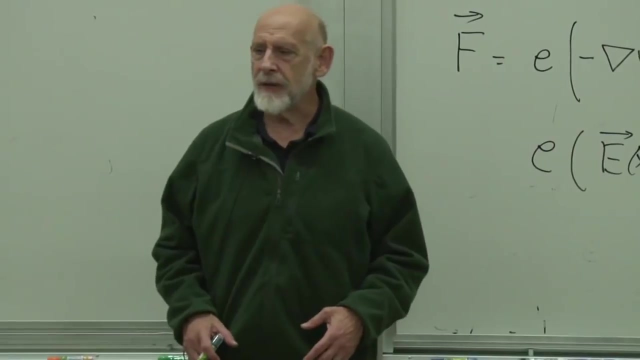 E is the gradient of V. V, incidentally, is not the velocity. we're going to have two fields, two V's in this problem. the velocity of the particle is also another important thing. then there's the magnetic force, and the magnetic force is something new, something that we haven't seen before. 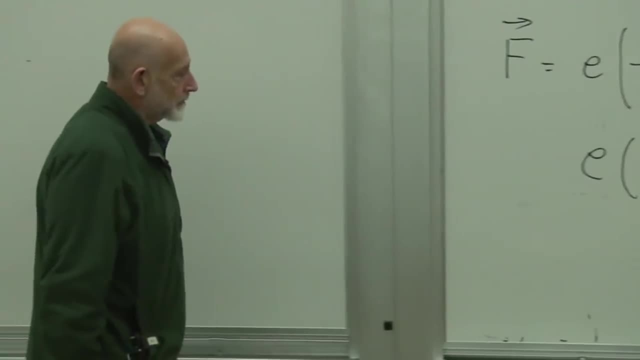 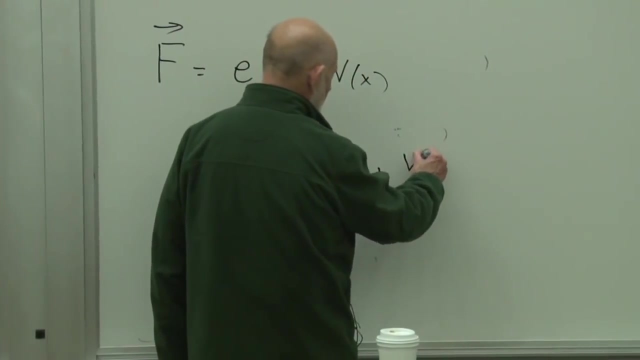 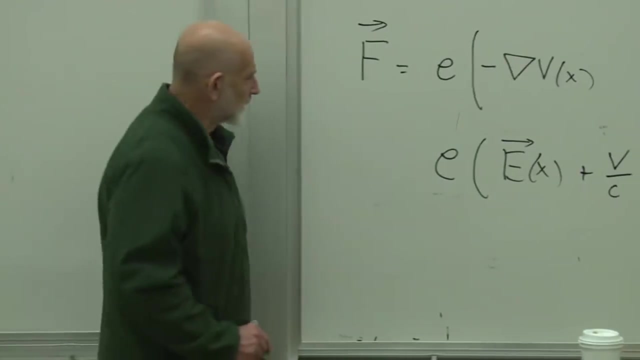 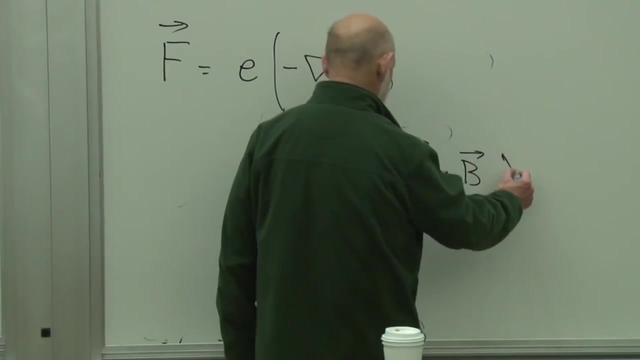 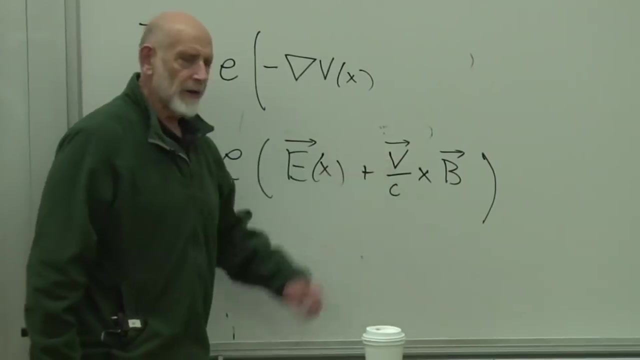 actually we have, and I'll tell you when in a minute. but the magnetic force involves the velocity of the particle divided by the speed of light across the magnetic field. the fact that there's a velocity of light in here means the particle has to be going damn fast. 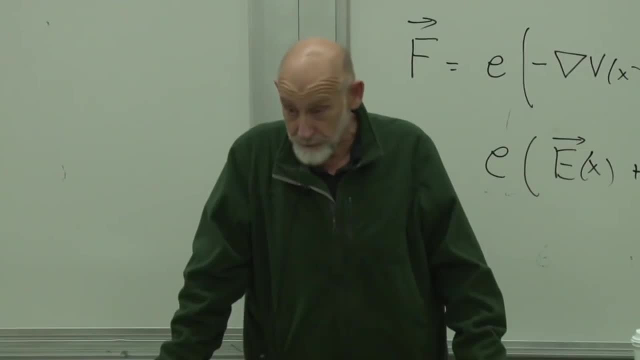 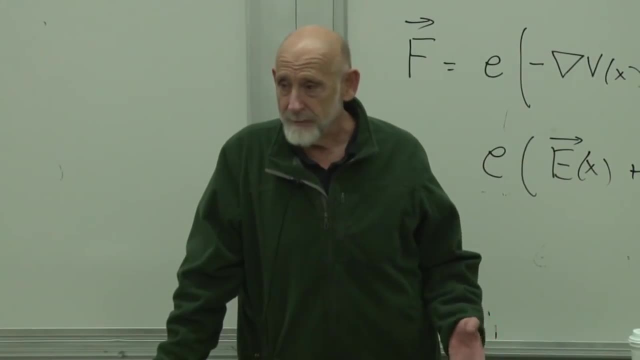 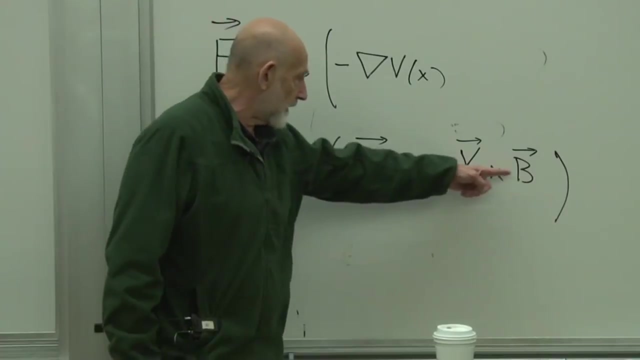 in order to experience any significant amount of magnetic force. of course electrons are very light and they can move pretty damn fast, but typically electric forces can be much stronger than magnetic forces for the simple reason that for magnetic and electric fields about comparable to each other, a particle has to be going pretty darn fast. 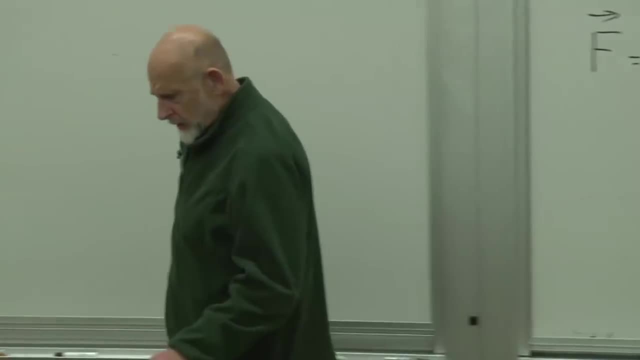 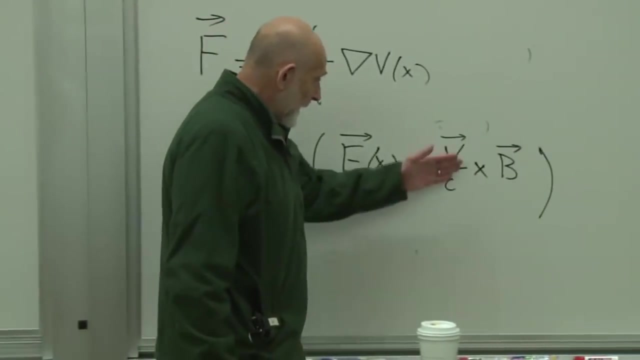 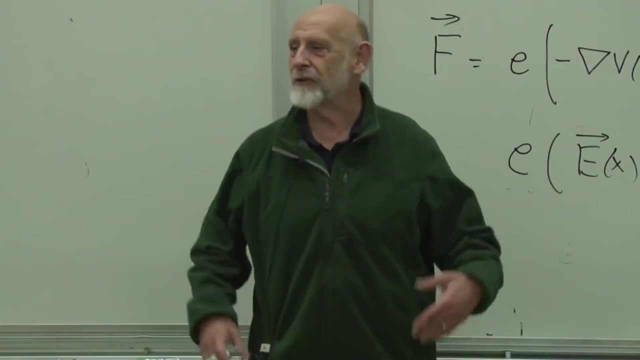 in order for V over C to be appreciable. okay, so magnetic forces are associated with motion. somehow, this is a kind of force that we haven't seen before, a force, of course. we have seen forces that depend on velocity, viscous forces for something moving through a viscous fluid. 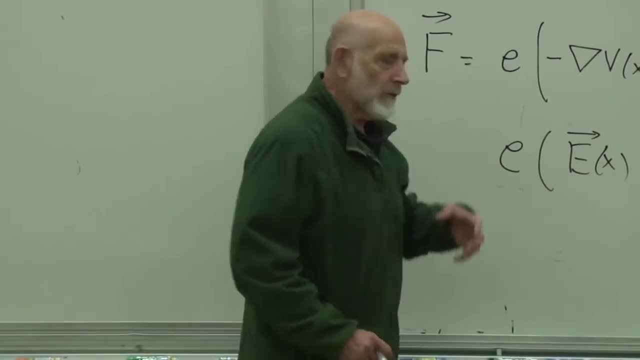 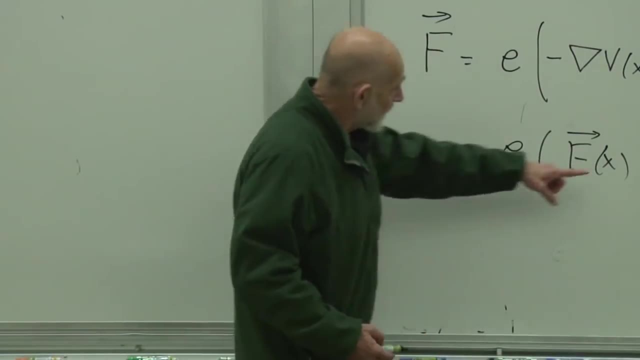 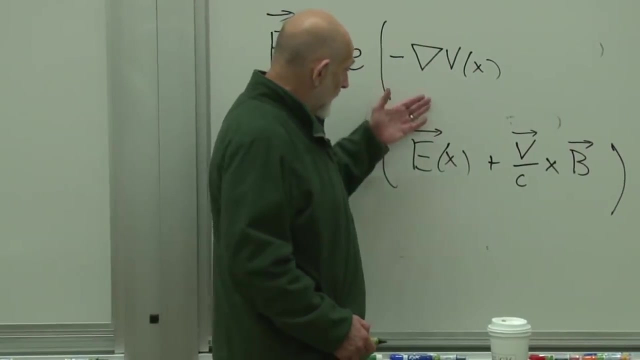 but this is not like that. it's very different. in particular, a viscous force acts along the direction of the velocity right opposite to it. usually, this force is perpendicular to both the velocity and the magnetic field. alright, so we have the electrostatic force. 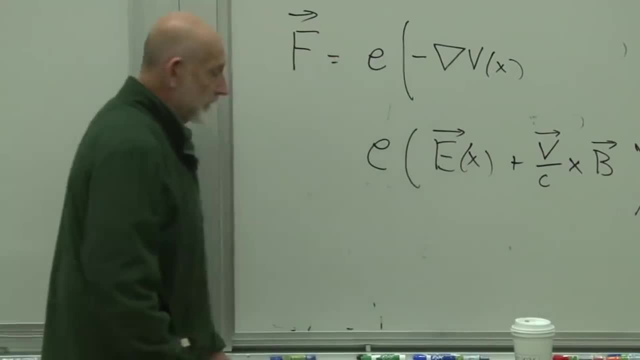 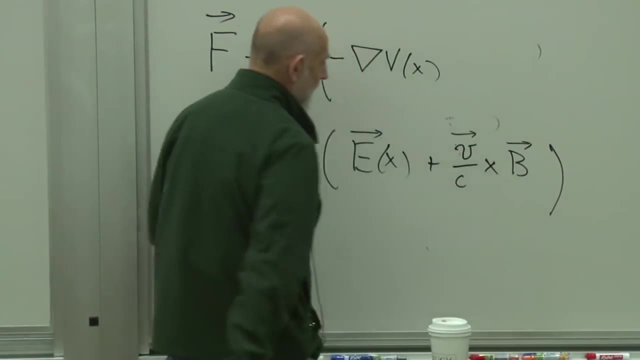 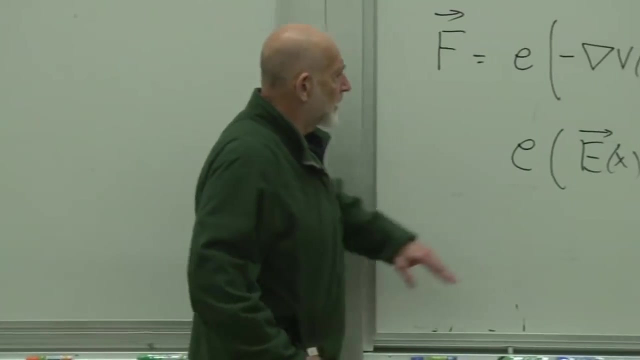 and we have the magnetic force velocity. let's not use big V, let's use small v. v cross b, where v is the velocity of the particle. okay, this has a name, this force. it's called the Lorentz force, the same Lorentz as Lorentz transformations. 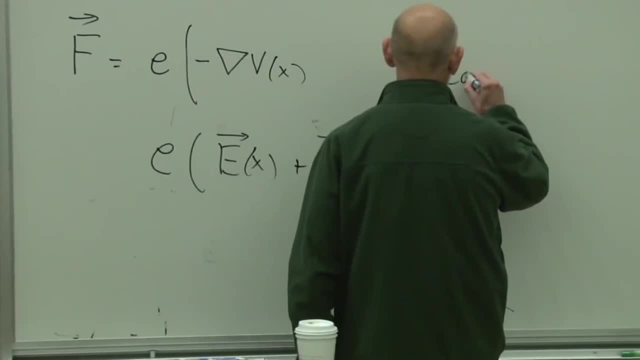 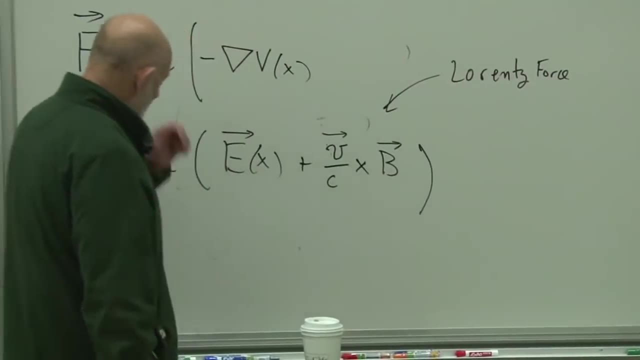 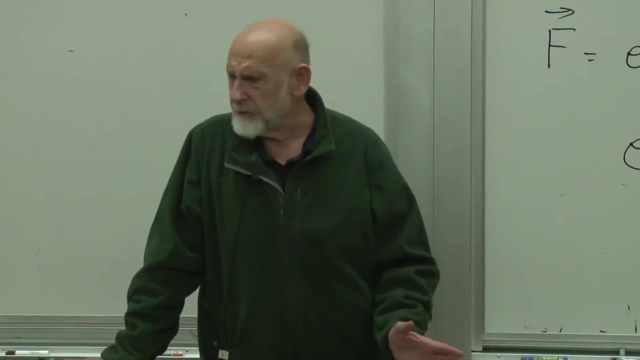 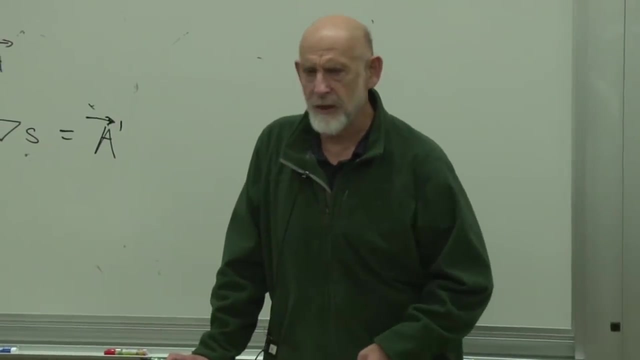 Lorentz force. it actually wasn't known and Lorentz was pretty late in the day. Lorentz was in the generation before Einstein. he was maybe, I don't know- maybe 50 years old when Einstein was a young man, and this was not known until Lorentz. 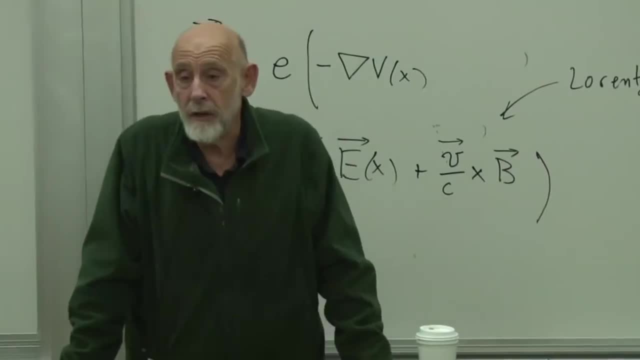 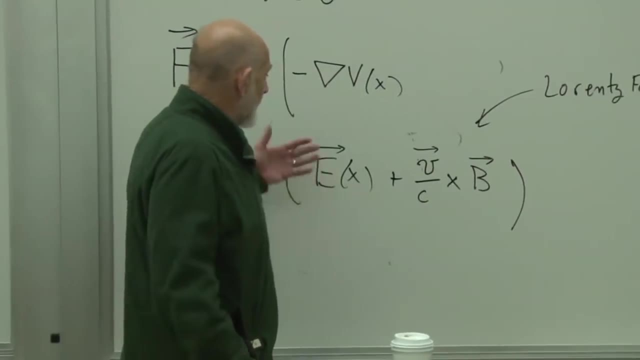 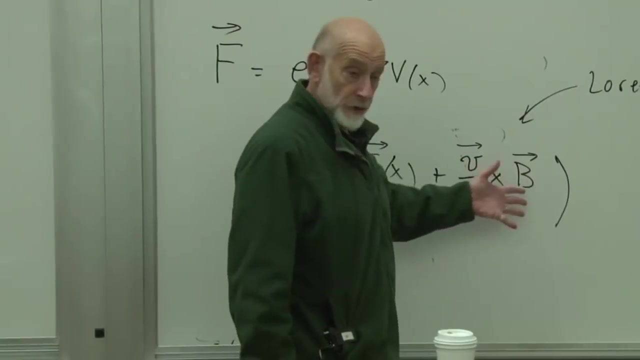 what was known was the forces on conducting wires with charge flowing through them, and Lorentz figured out correctly that in order to get that kind of force on wires with currents flowing through them, the force on an individual electron, for example, would have to be this: 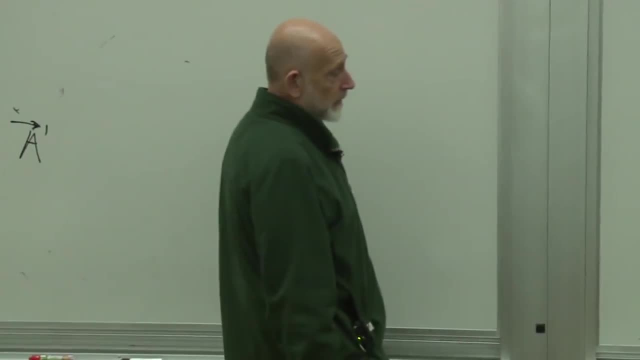 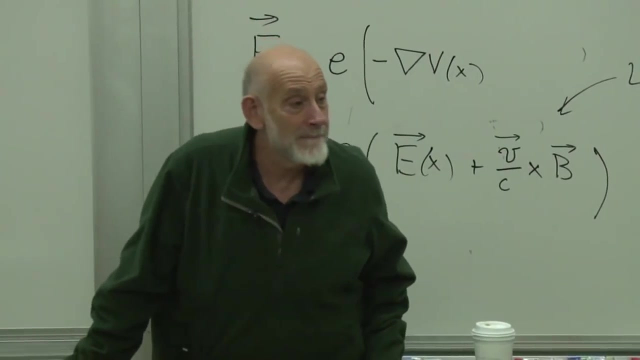 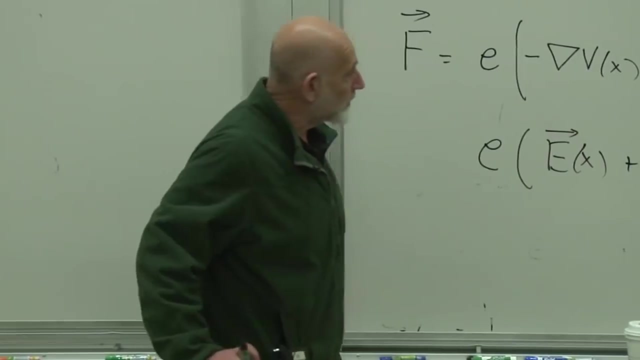 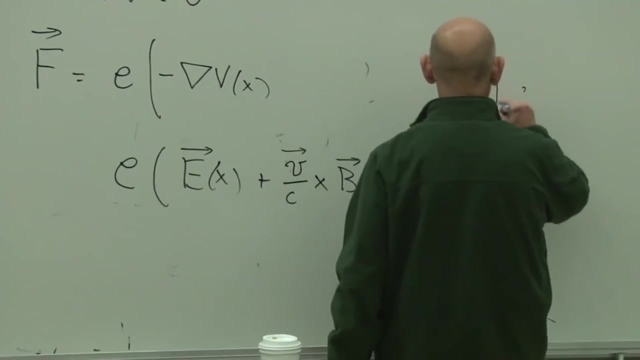 so perpendicular to the velocity, perpendicular to the magnetic field. do you ever remember seeing anything like that Coriolis force? let me just remind you what the Coriolis force was. the Coriolis force was a similar formula. the Coriolis force F Coriolis. 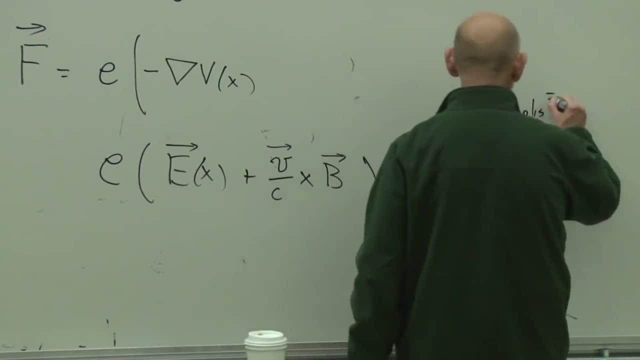 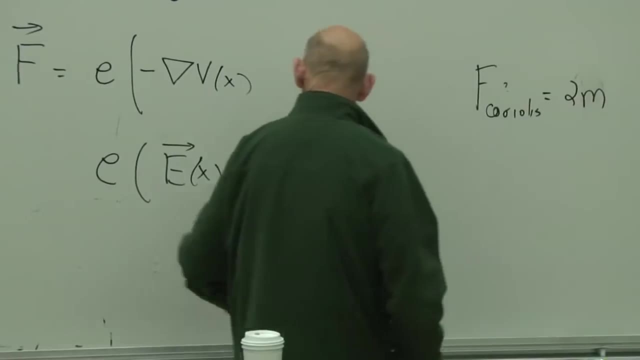 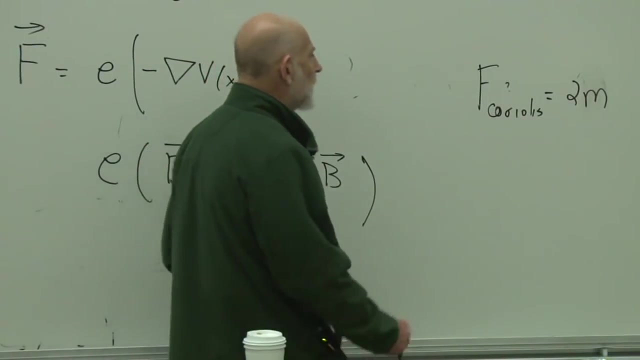 Coriolis is also V cross something. in fact it's twice- I think it's twice the mass of the particle. instead of having the electric charge, it has the mass of the particle. it doesn't have a C in the denominator- twice the mass of the particle. 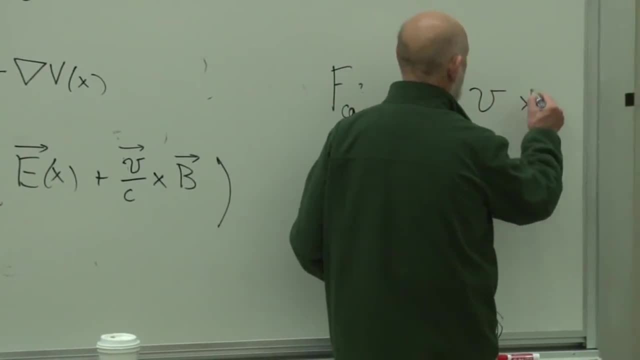 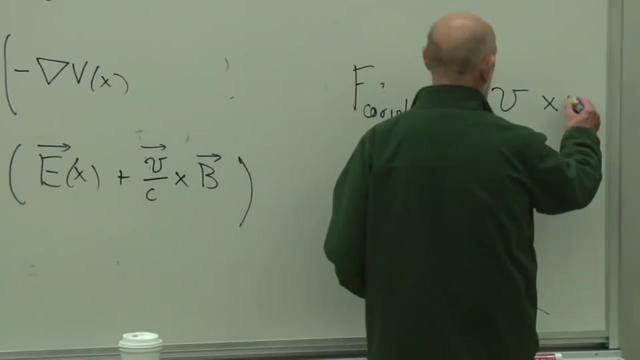 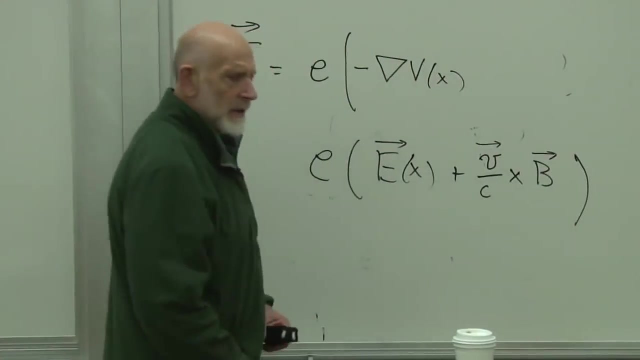 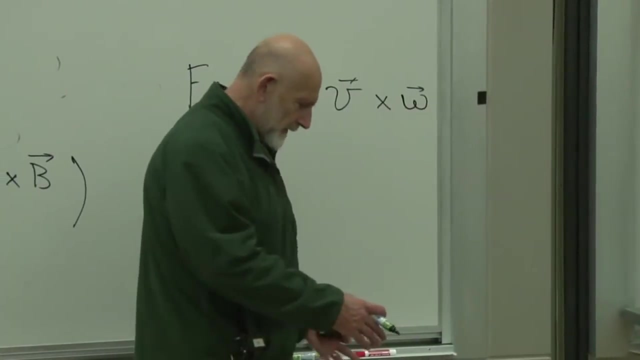 times the velocity cross. what omega? the angular velocity. sometimes I think I use the symbol small omega. sometimes big omega is used. what does this correspond to if you're on a rotating platform, for example? this platform can rotate if I'm on a rotating platform. 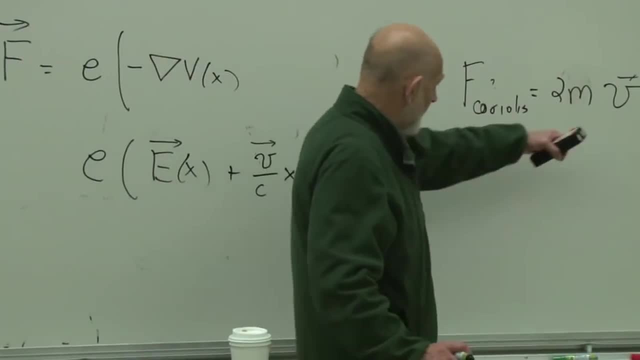 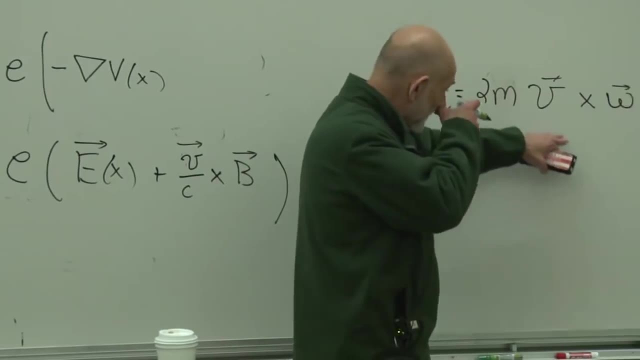 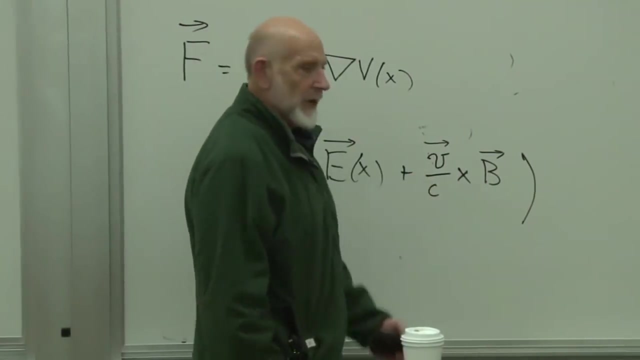 then there is an omega. the omega would be perpendicular to the plane of the of the flaw. there's a vertical, and this is a very similar sort of thing if we have a uniform magnetic field, let's say pointing straight upward the forces exerted on charged particles. 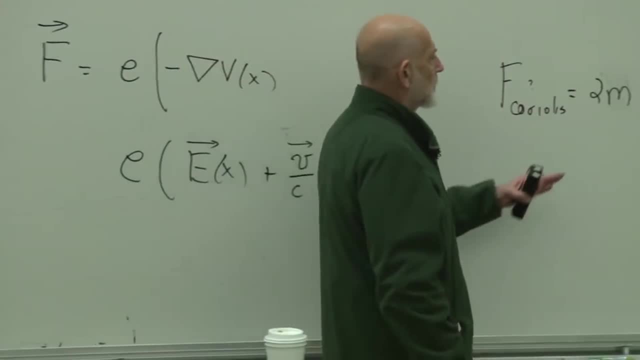 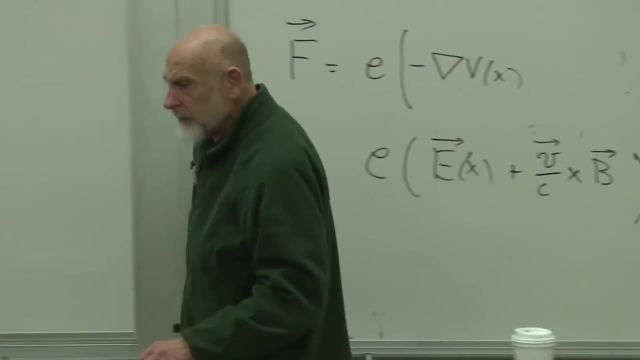 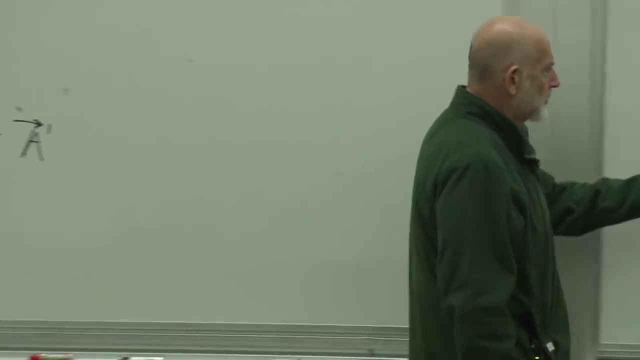 by that uniform magnetic field are essentially the same as the Coriolis force, with the magnetic field being replaced by the omega vector. so you have seen it before. it might be a good time to go back to it and remember a little about it. you have seen this sort of equation before. 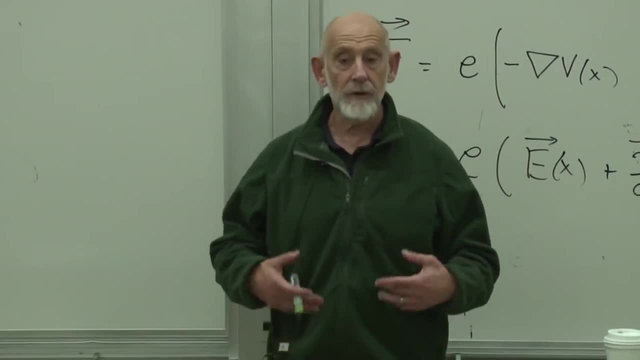 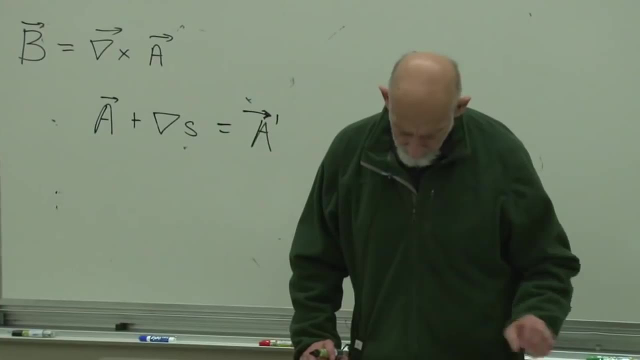 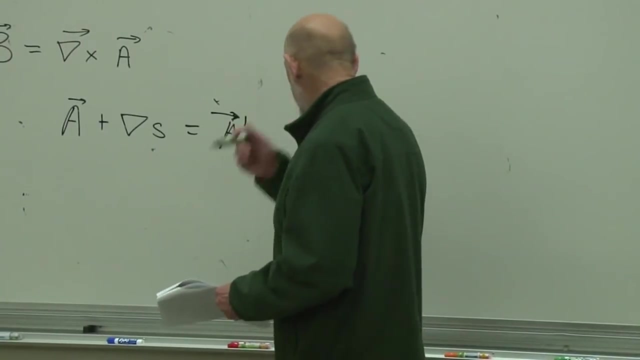 but we've never talked about it in the language of the Lagrangians, Hamiltonians and so forth- something new to explore. so the question comes up now. oh yeah, before we get into Lagrangians and Hamiltonians and so forth, let's just talk a little bit. 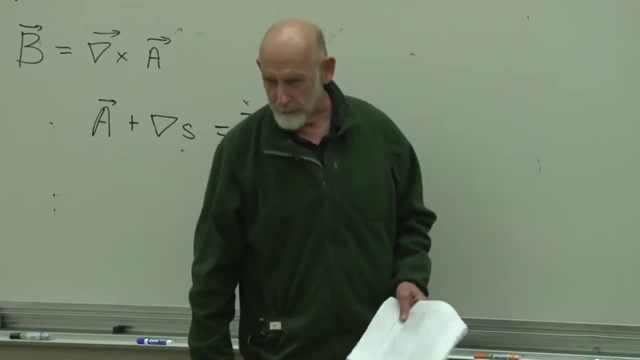 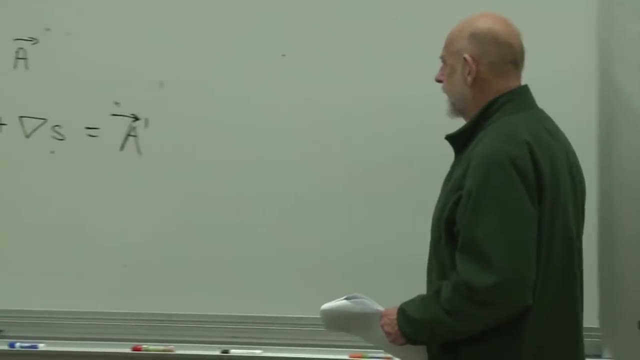 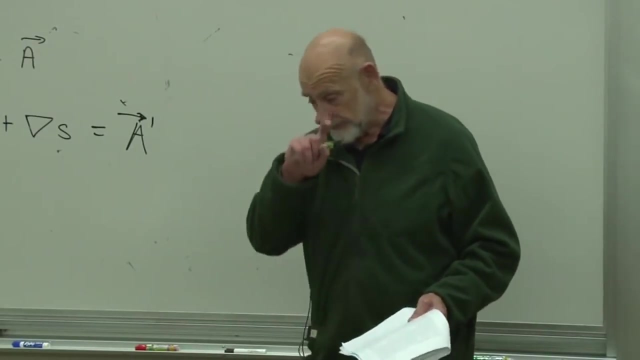 about this ambiguity in A and let me give you one or two examples of it, really just two examples of it's. one example of the ambiguity, two examples of a vector potential giving rise to exactly the same magnetic field, the simplest magnetic field of all, a constant magnetic field. 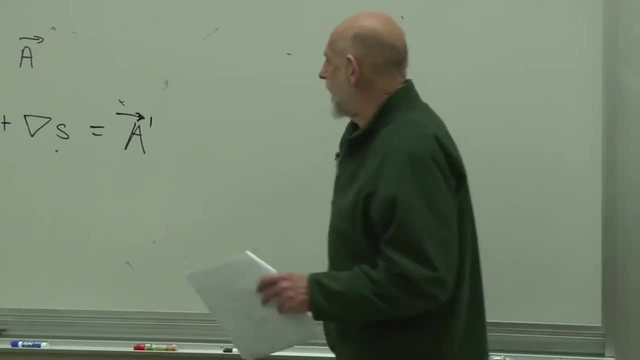 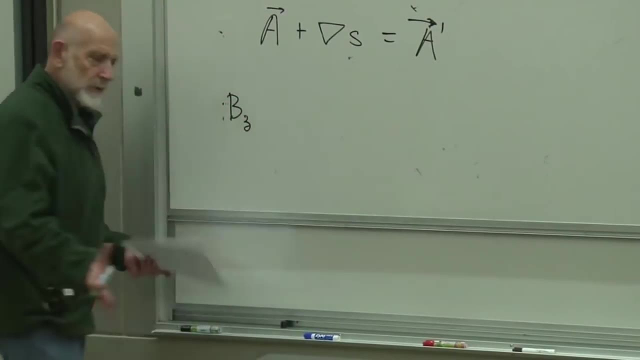 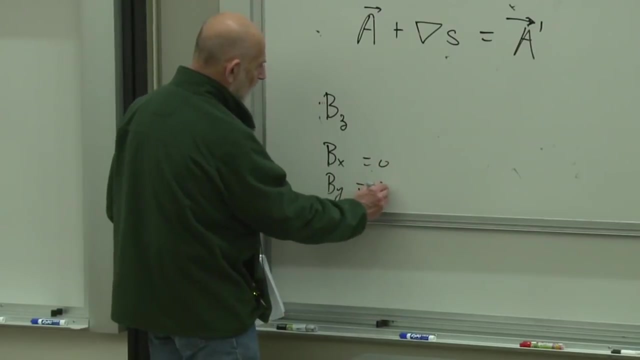 just a uniform magnetic field. let's say, in the z direction. b z is not equal to zero, b x and b y are equal to zero. and what about b z? it's along the z axis and I'm going to say that it's equal to zero. 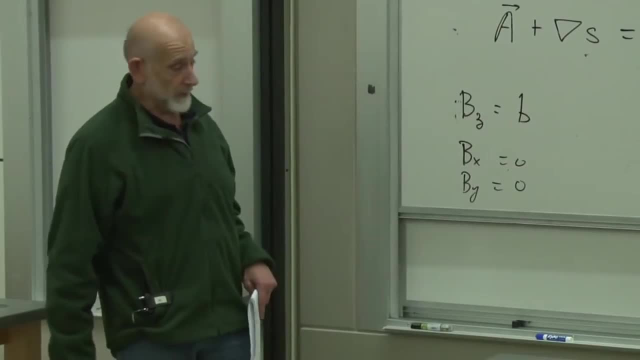 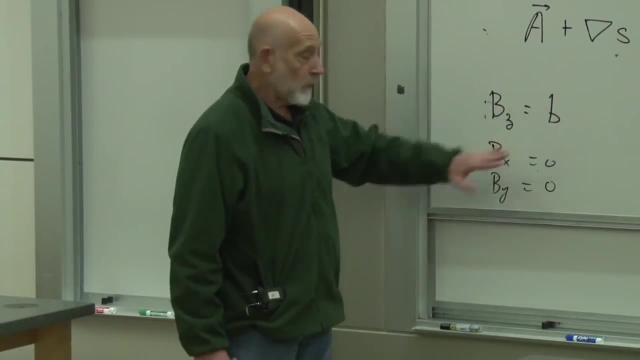 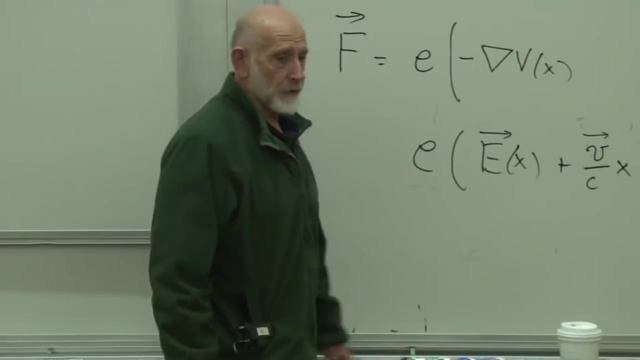 and that's the magnitude of the b field and the constant. constant doesn't vary from place to place. a uniform magnetic field about the z axis. can we find the vector potential which gives rise to this field? I'm going to write down two examples. both of them give rise. 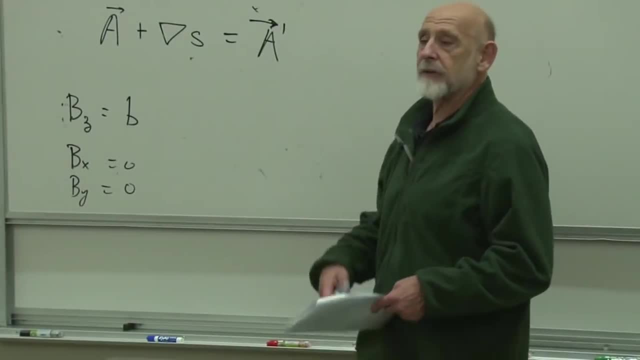 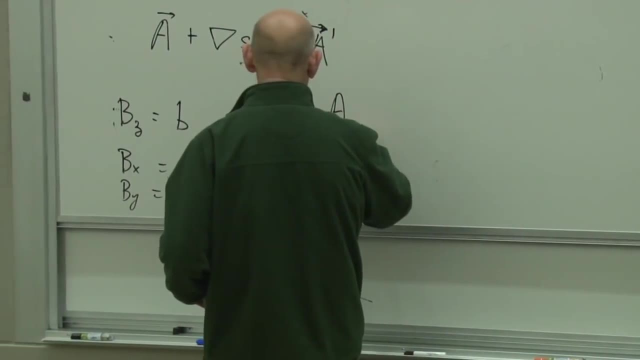 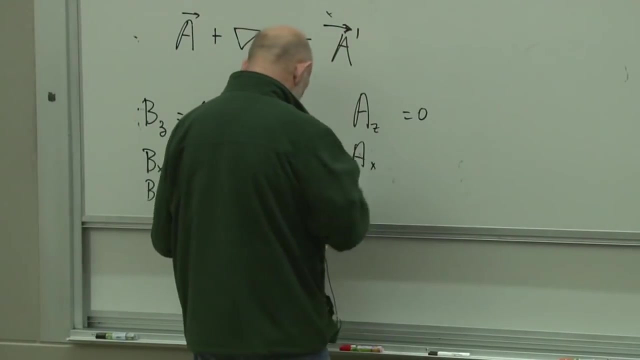 to the same magnetic field, and in fact we can write an infinite number of them. let me just write them down. here's: a. a sub z is equal to zero. a sub x, let's see. a sub x is also equal to zero. but a sub y is equal. 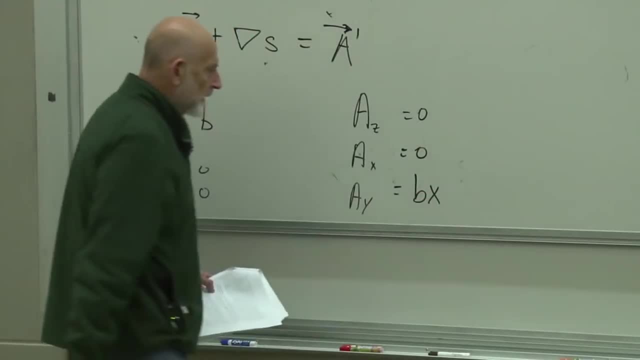 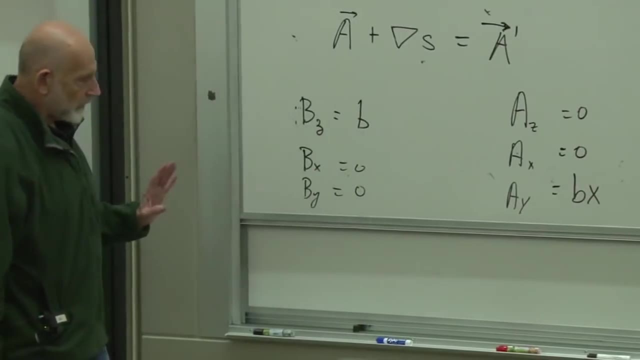 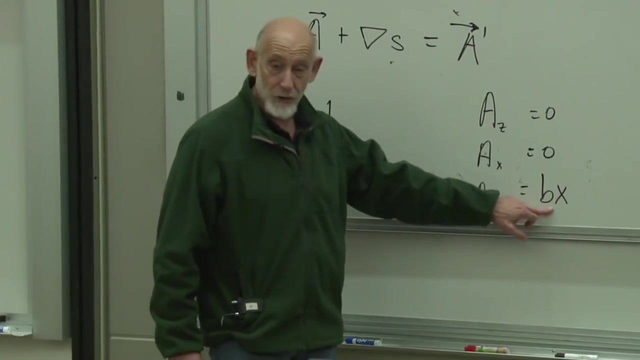 I think b times x. b is a number, but x varies from place to place. let's check, let's check the curl of a. the curl of a involves derivatives and there's only one thing to differentiate with with respect to x: there's no y dependence, there's no z dependence. 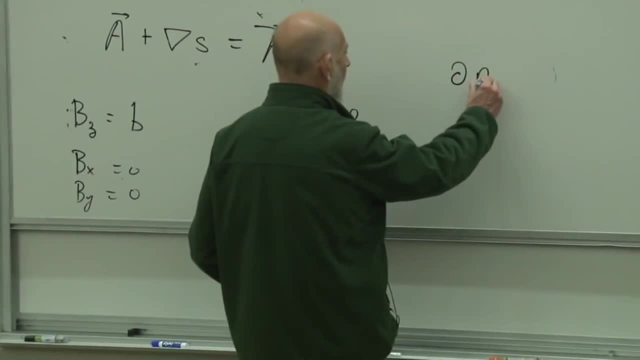 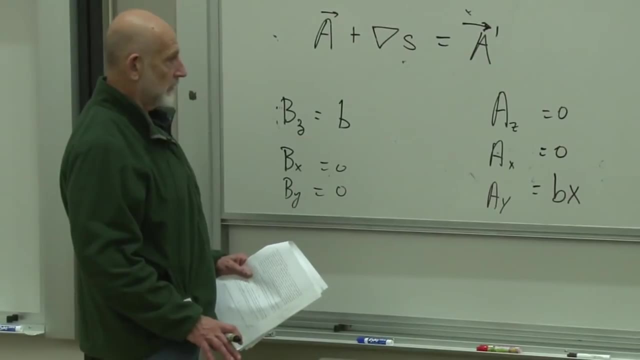 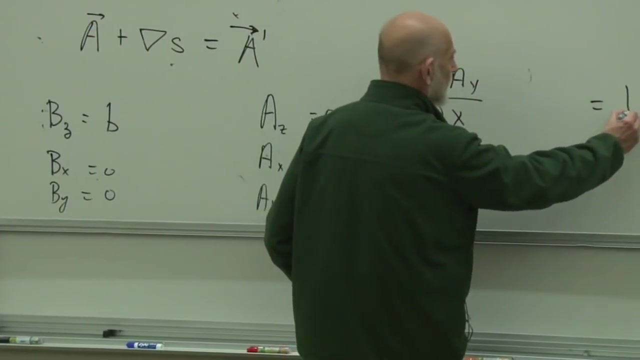 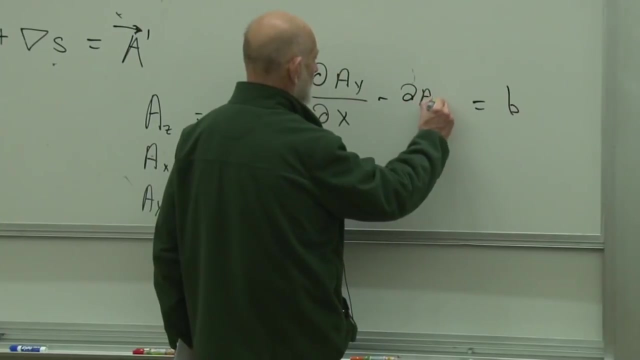 so the only thing around is derivative of ay with respect to x, that's all. there is no, yeah, no other derivatives around. and this is equal to b. well, for free, in this case, I can subtract off dx with respect to y, because ax is equal to zero. 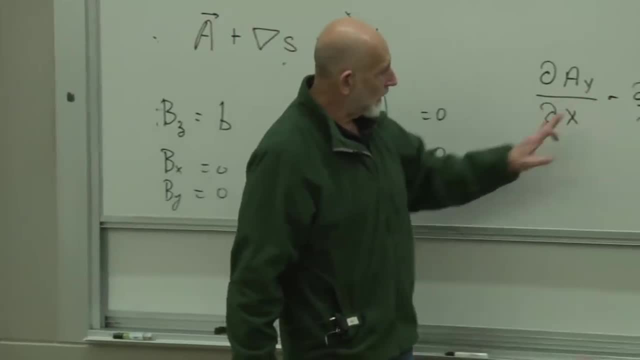 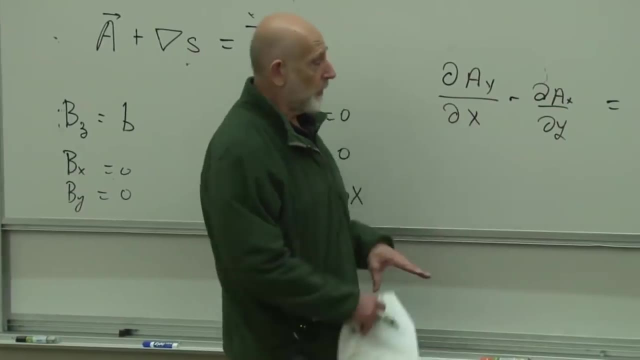 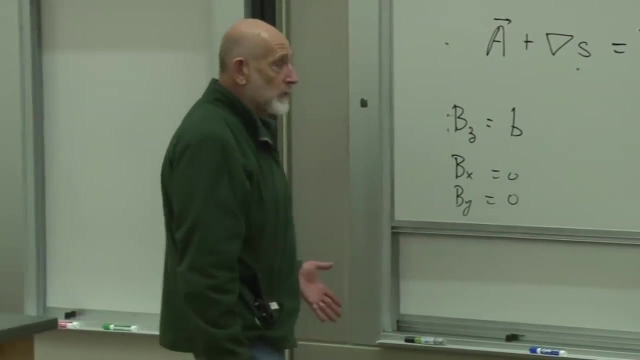 so that's free, I can put that in there. and what is this thing? this is the z component of the curl. alright, so it's the z component of the curl and therefore it should be bz. but that's exactly what we have here. what about the other components of the curl? 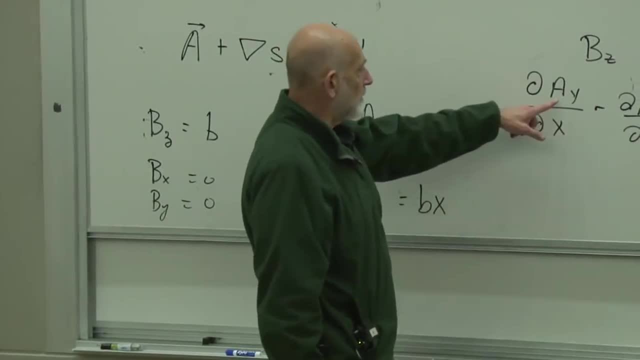 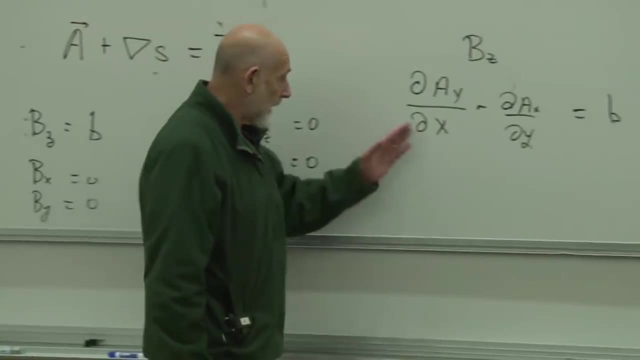 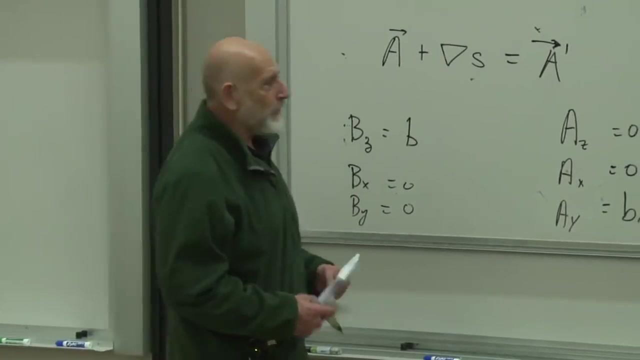 they're all zero. the only component that I can make is the ay by dx. that's the only thing around that varies. so this is a vector potential which generates a uniform magnetic field along the z axis. but there's something a little bit funny if you think about 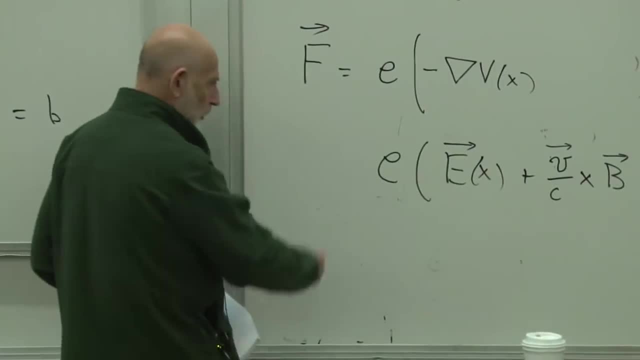 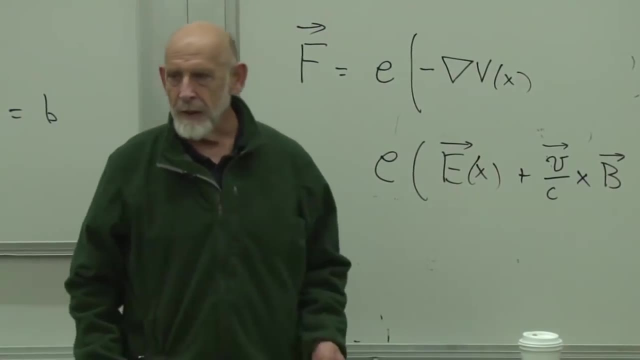 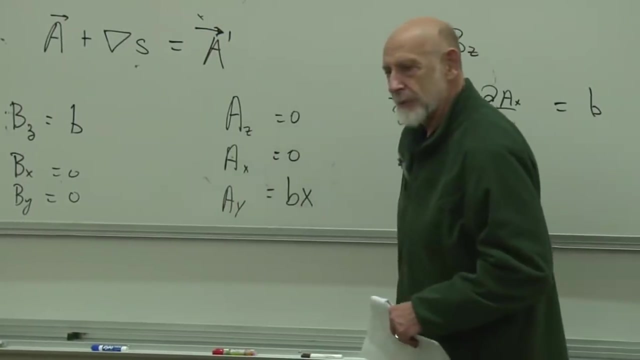 a magnetic field along the z axis. let's say the z axis is into the blackboard, you have a completely uniform magnetic field. it sure looks like everything is rotationally invariant. it doesn't. why does it pick out? why does it pick out the y component of the vector potential? 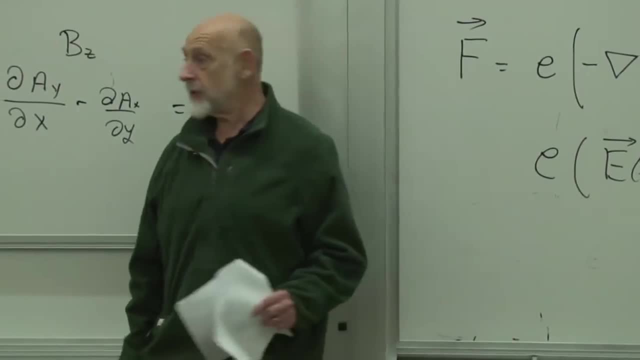 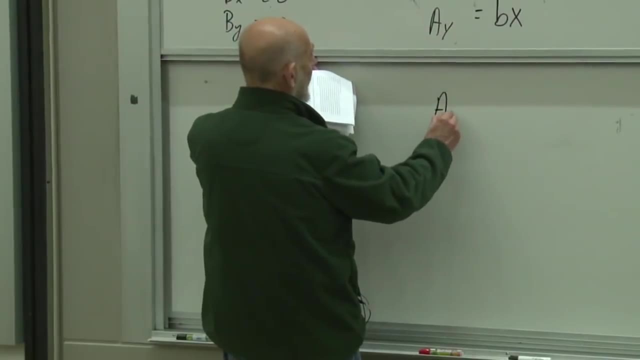 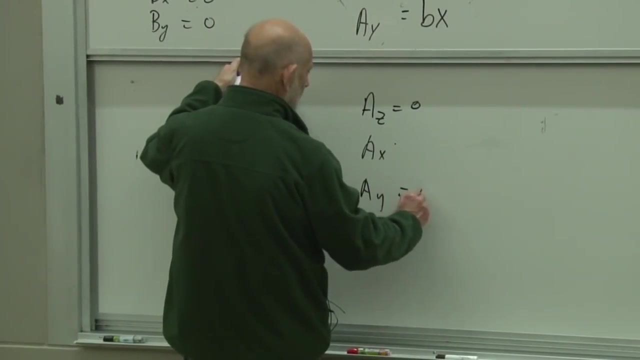 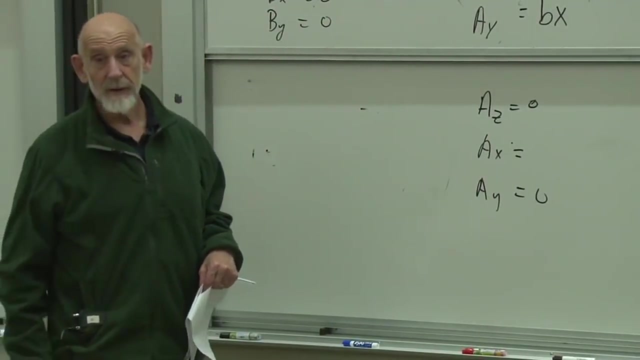 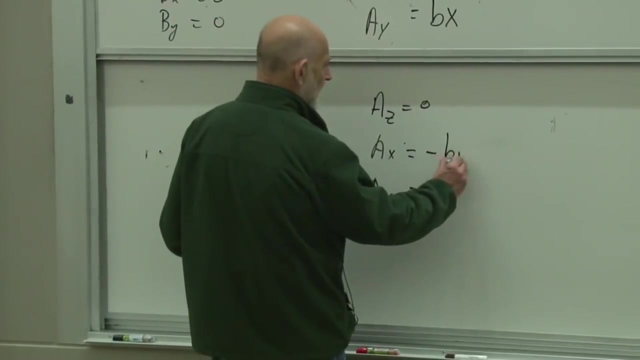 why not the x component of the vector potential? well, the answer is that there is at least one more representation, namely az equals zero, ax equals zero. ah sorry, ay equals zero and ax, you want to guess? ay, b y, b y, right, not quite, minus b? y, alright. so now what do we have? 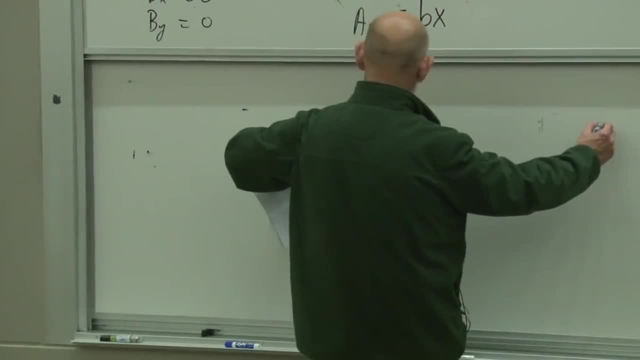 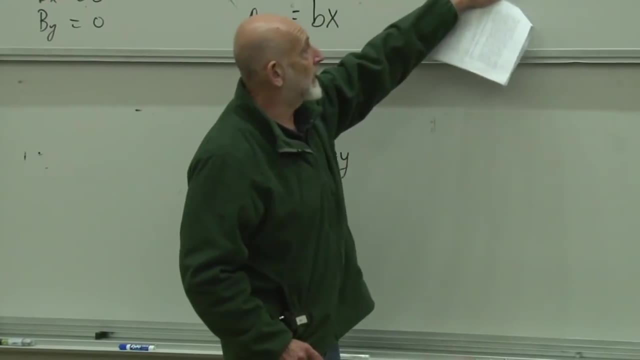 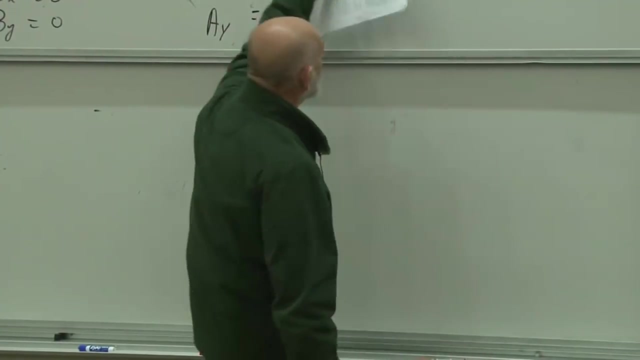 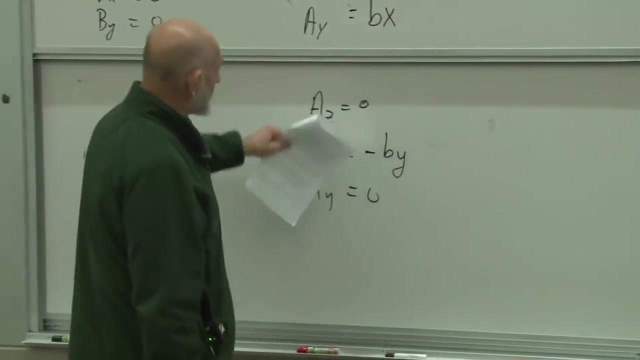 now we have: dax by dy is not equal to zero. everything else is zero, but dax by dy is minus b. two minus signs cancel and again we get the z component of the magnetic field just equal to b. so these are two different representations of the same magnetic field. 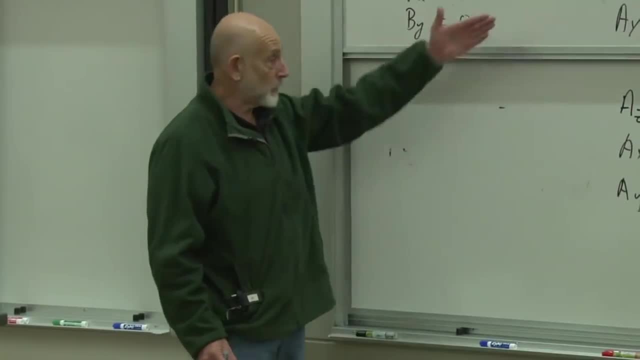 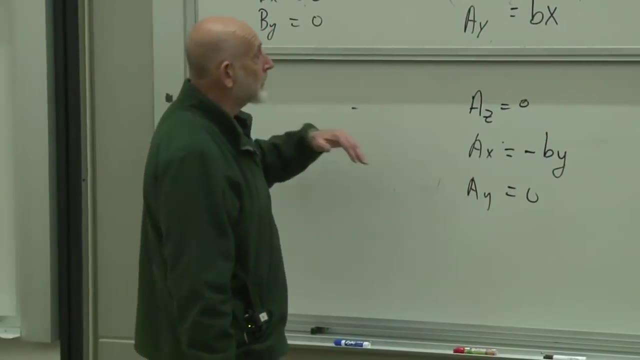 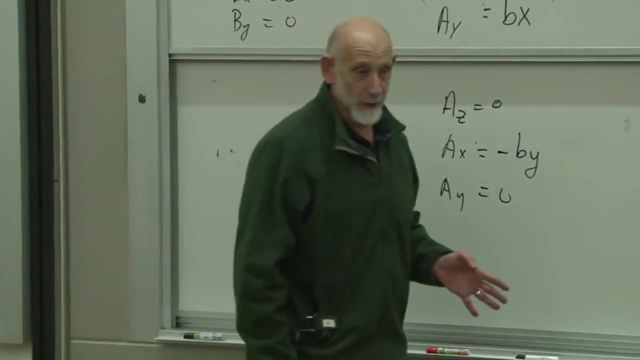 by vector potentials. how are they related? they are in fact related. the difference- this is a homework problem. again, the difference between these two vectors can be seen to be a gradient. you can figure out what it's a gradient of, or you can try, yes, you can figure out what it's a gradient of. 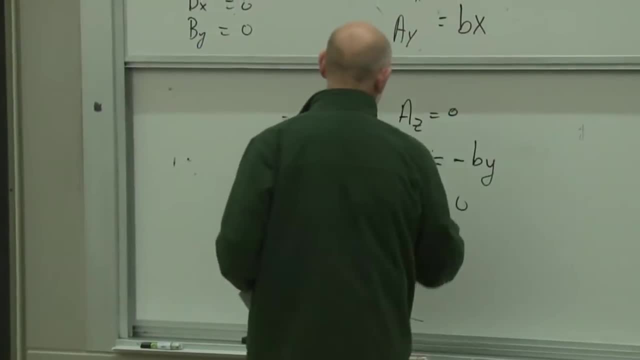 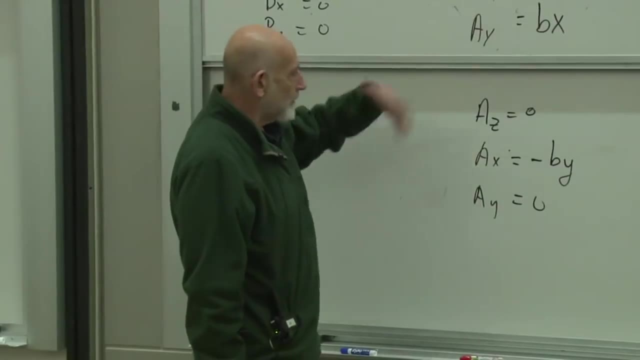 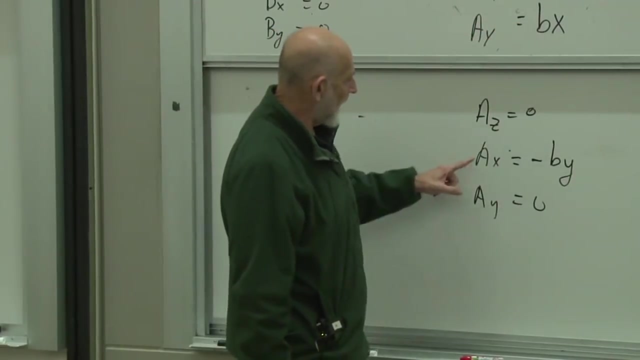 in fact you can. you can write more general answers. you can have combinations of both of these, a bit of ax and a bit of ay, adding up in such a way as to a bit of ay proportional to x and ax proportional to y. you can combine them. 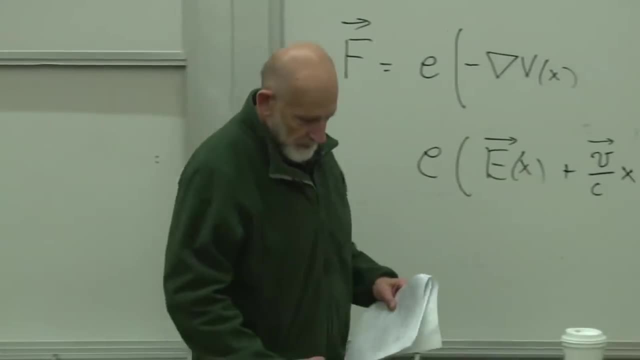 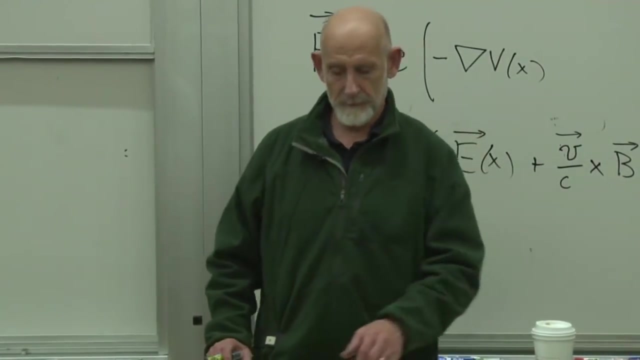 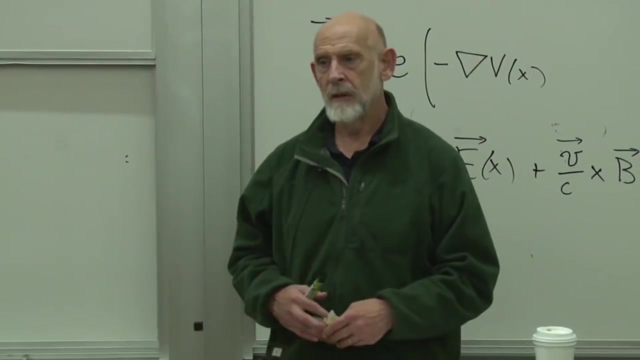 and basically get an infinite number of different representations. is that is that sort of equivalent to saying: if you wanted a magnetic field pointing perpendicular to the board and you had a coil of current, there's a lot of ways you could locate that coil, arrange it around. 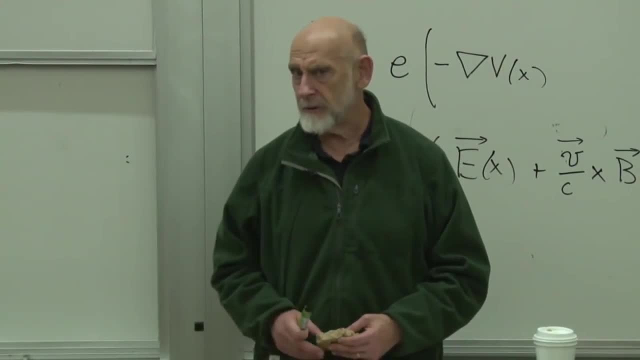 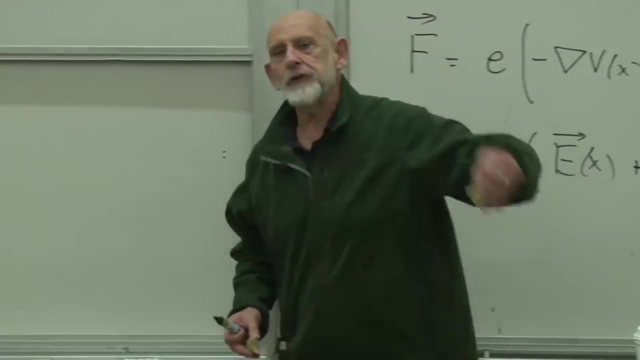 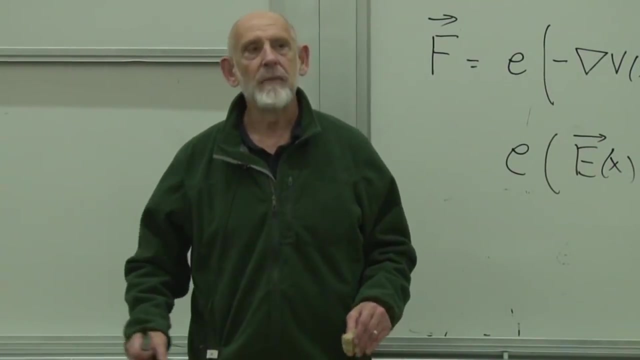 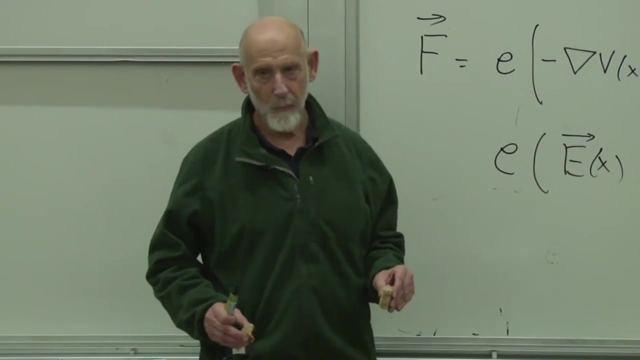 that's true, but this is a different ambiguity. this is a different ambiguity. however you change, however you arrange the wires. there is a definite magnetic field at all places in space, but there is not a definite vector potential, not right? couldn't you say that the geometry of this? 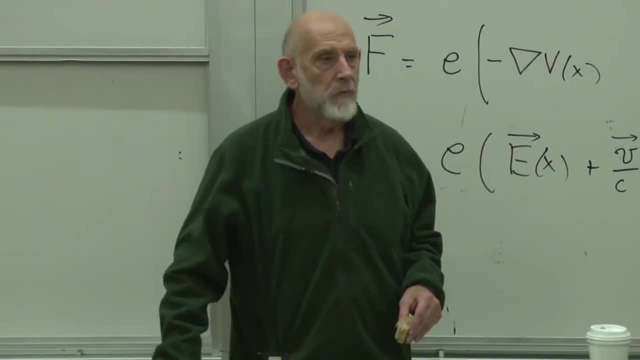 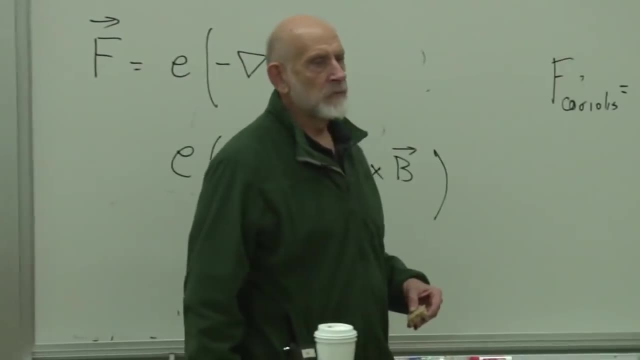 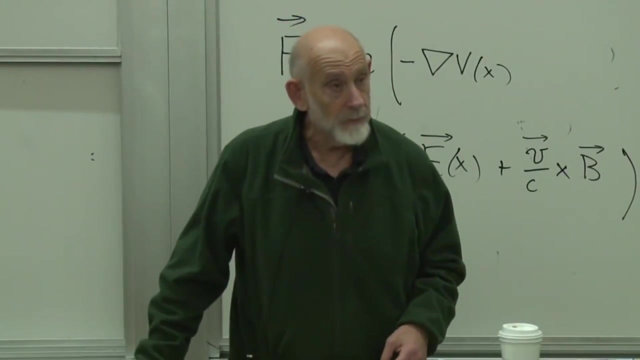 is. anytime you add any gradient, you're either stretching or compressing space, but you're not causing a twist, and the curl only cares about whether there's a twist, and that's why it's gradient. yeah, yeah, that's right, that is true. is there any relationship between? 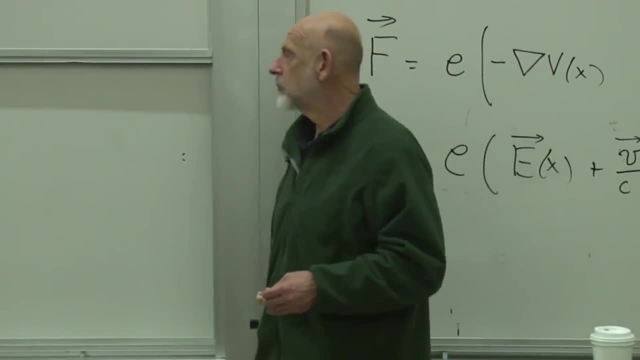 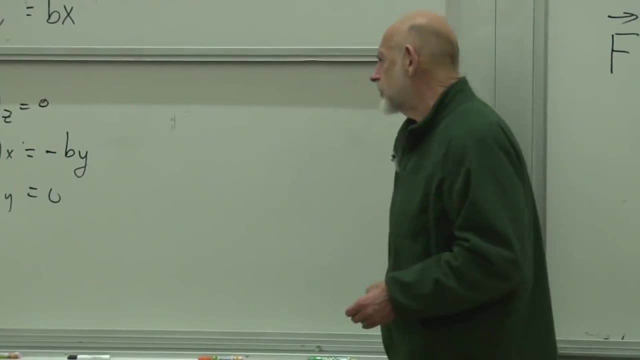 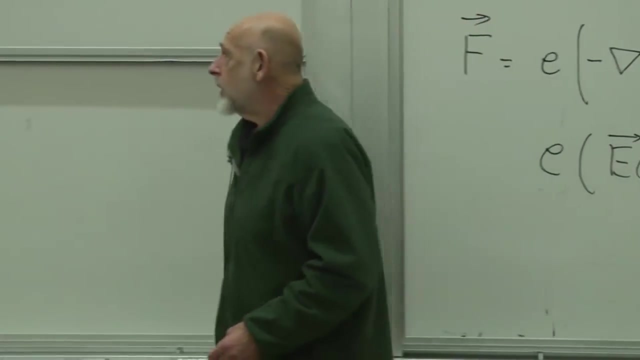 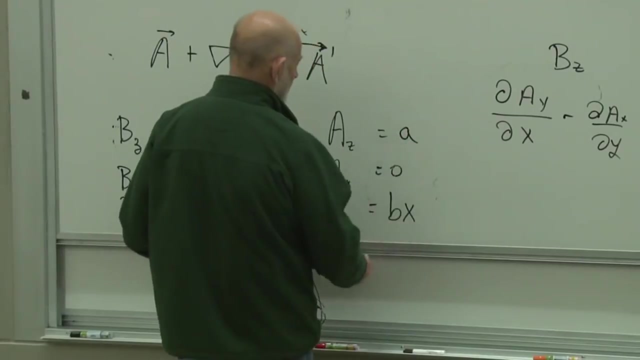 the direction of the magnetic field and the and the A potential. well, no unique connection in this case. it's pretty clear that the magnetic field is perpendicular to A, but we could add: I said Az is equal to zero. I could have let Az be a constant, since a constant. 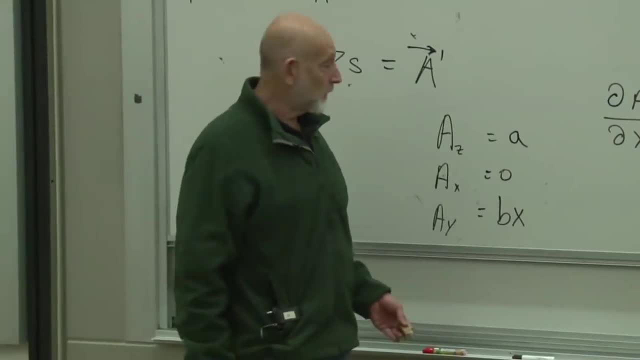 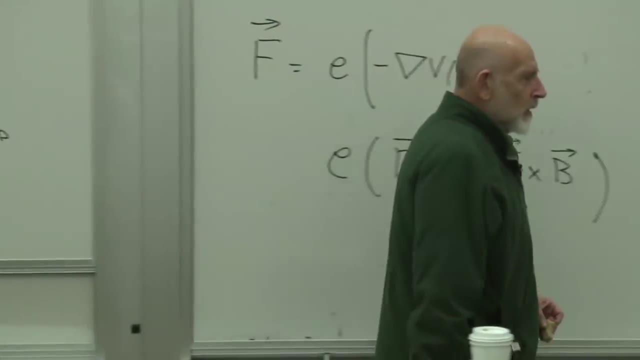 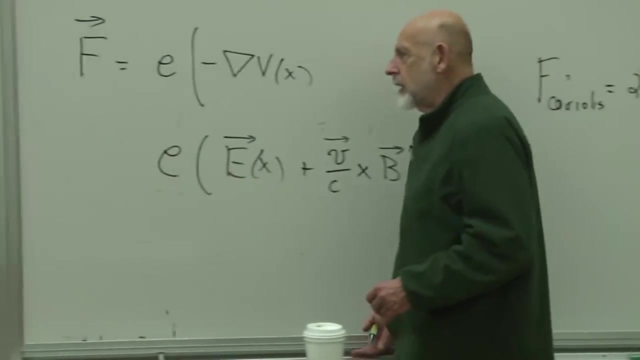 has no derivative, it wouldn't make any difference, and then A would not be perpendicular to the magnetic field. incidentally, there is another place where an ambiguity like this exists. it's a much milder ambiguity. let's go back to it for a minute, because it is. 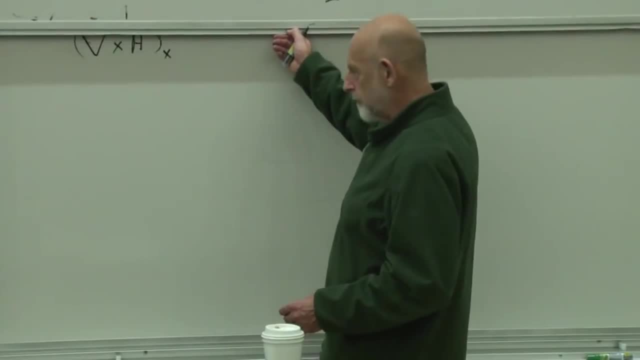 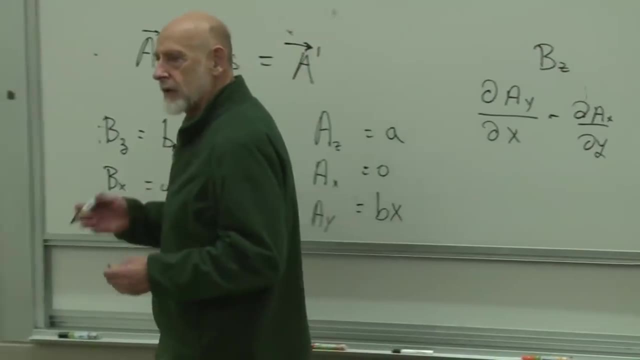 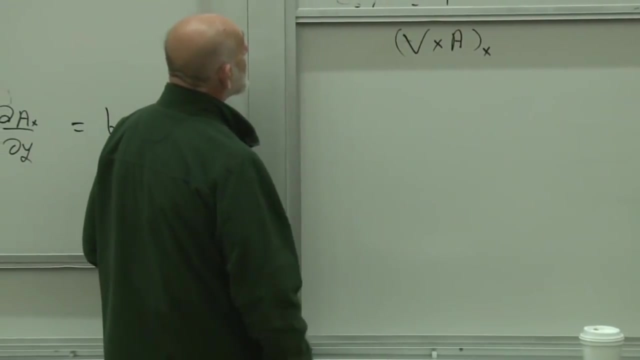 related and it's the source of some of the terminology. let's go back to either electric forces or just ordinary forces, that of the kind which come from differentiating a potential energy. we write that the force is equal to the gradient of the potential energy. well, here's an example. 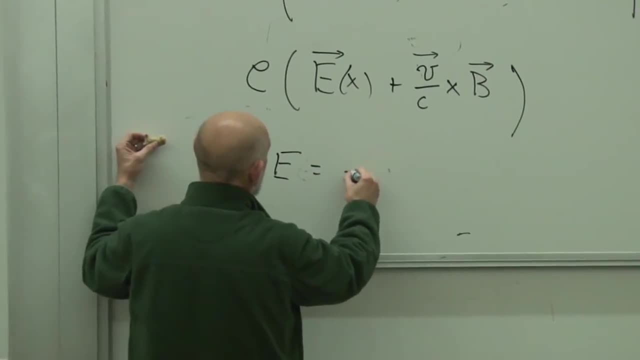 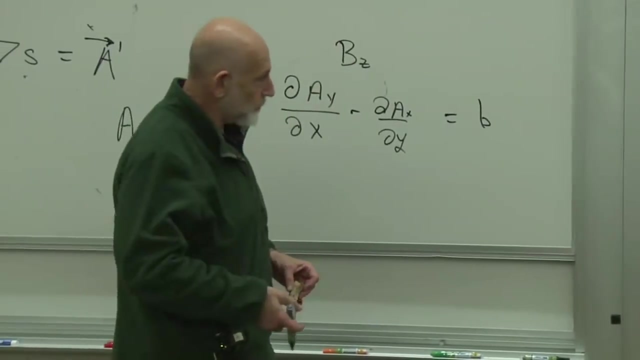 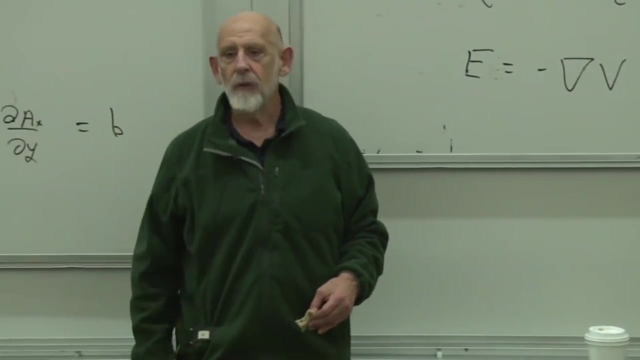 just the fact that the electric field is equal to minus the gradient of the thing that we call V, the voltage, the potential, the electrostatic potential. this does not completely tell you what V is, even if you know. the electric field everywhere is what's missing: an additive constant. 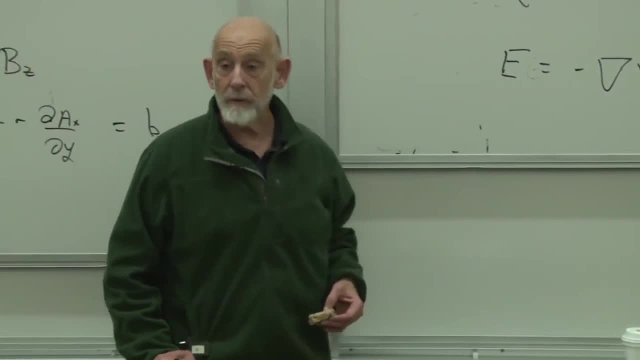 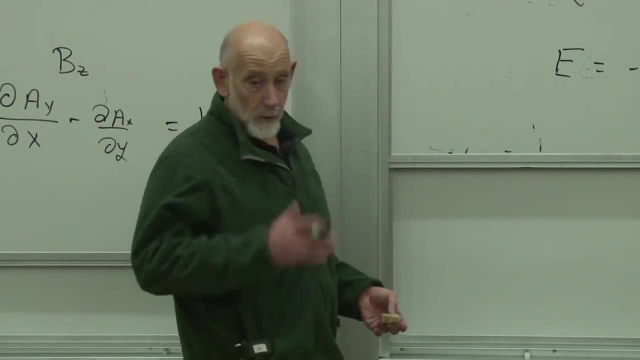 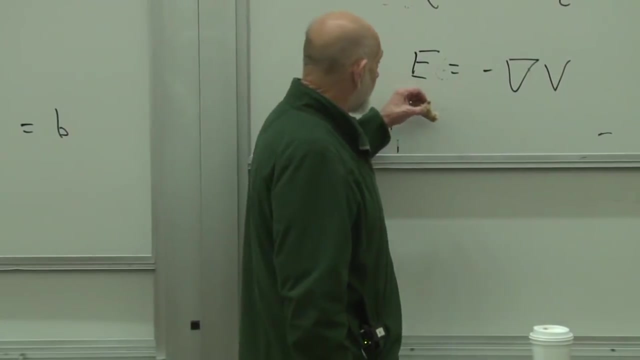 you can always add a constant to the potential without changing the value of the electric field. this is a similar ambiguity. it's a milder one. it's only a constant, but what you're doing is adding things which don't have the kind of derivative that leads. 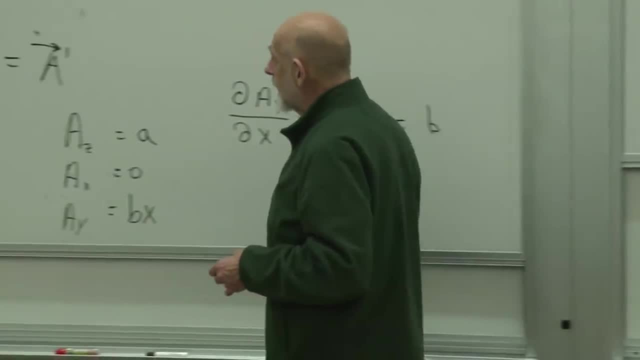 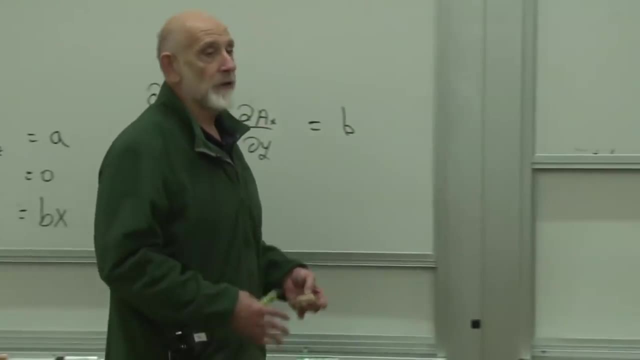 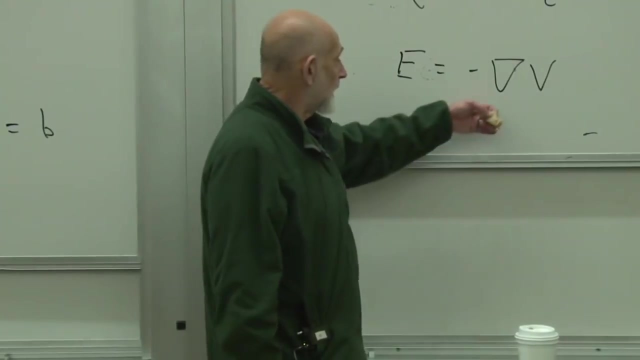 to an electric field. you're doing something very similar in the case of the magnetic field. you're adding something to A which is of the kind of thing which does not give rise to a magnetic field. okay, this is the source. incidentally, the idea of potential energy. 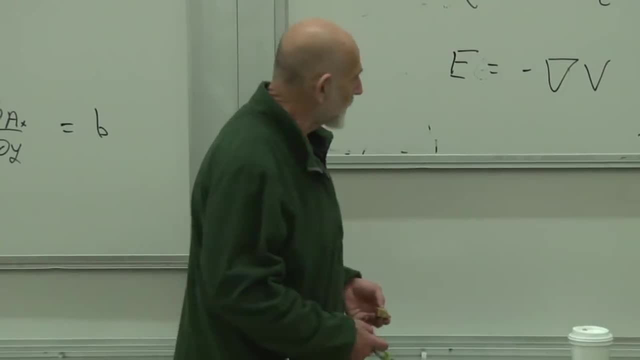 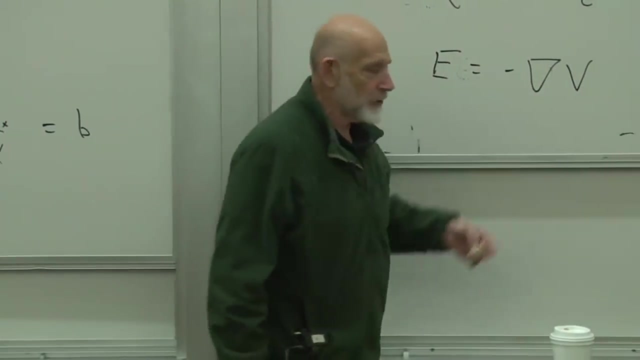 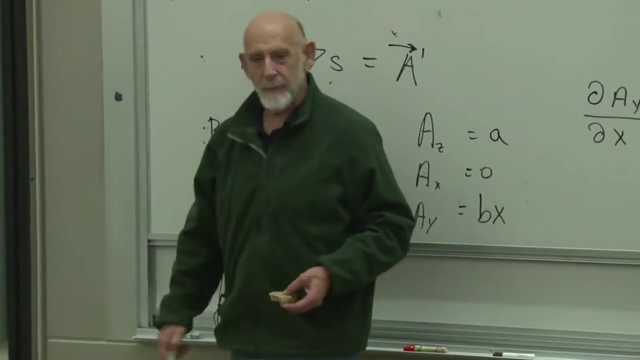 those words, of course, mean something we know. you're familiar with those: the idea of an electrostatic potential. well, that's connected with the fact that this is proportional to the potential energy, and when people started writing down magnetic fields and introducing vector potentials, they were talking about. 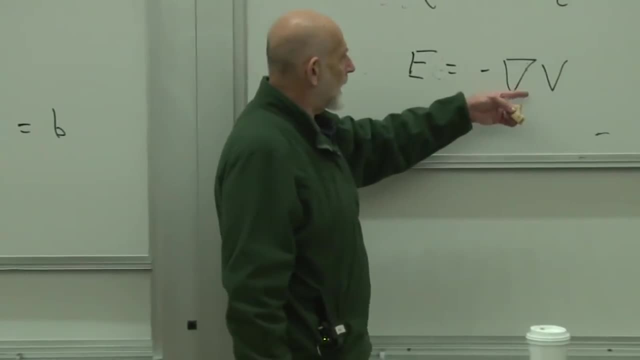 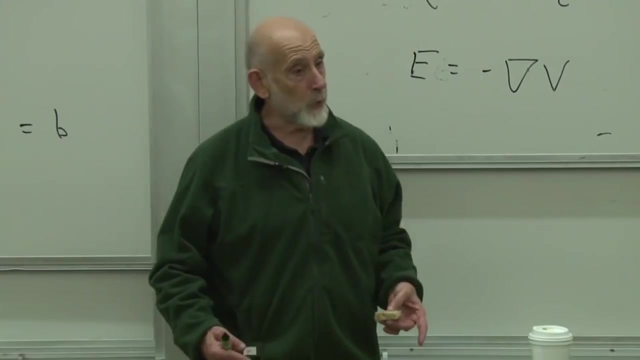 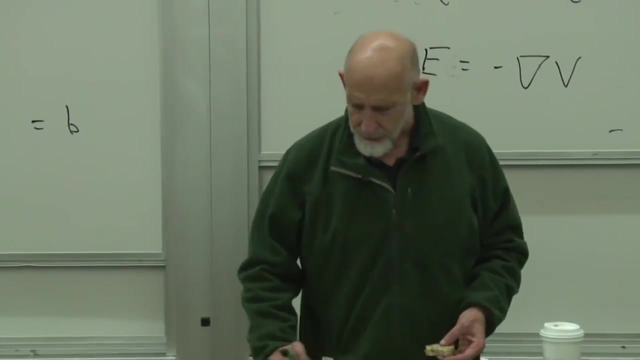 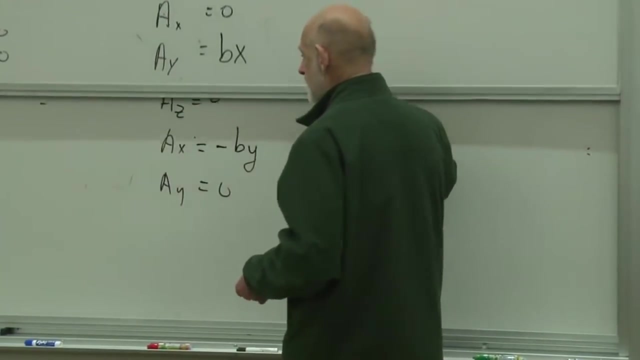 they used the word potential because it reminded them of the ambiguity in the potential energy, something that you can add but which doesn't give rise to a changed physical field. okay, so we have a lot of ideas. yeah, on your second equation, down there, the force, does it have a symbol? 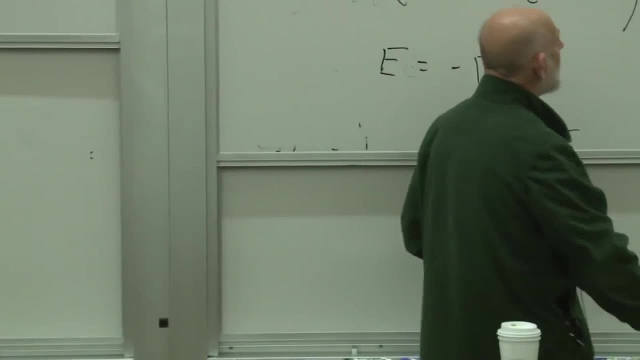 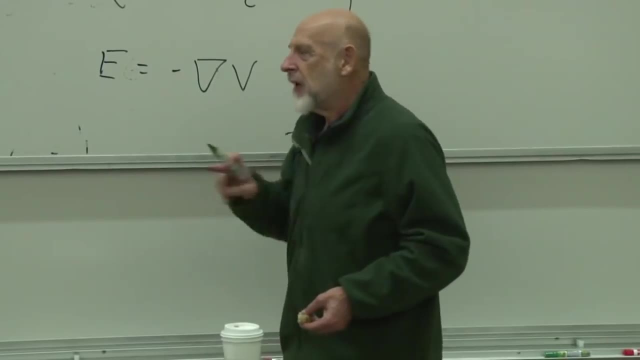 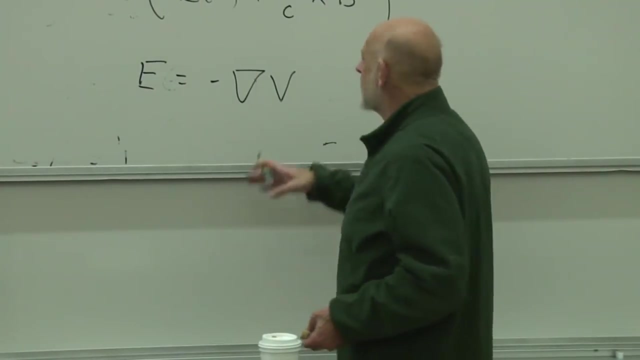 or a name or something. this one, no one of them. this one, yeah, that one, yes, it's called the Lorentz force. oh, the whole thing is the Lorentz force. I guess the whole thing is yeah, but this was no surprise. I think the whole thing is called the Lorentz force. 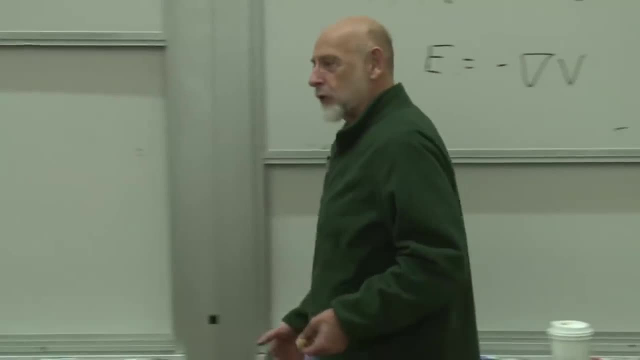 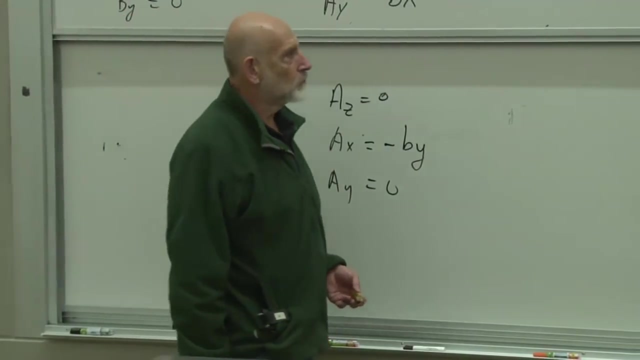 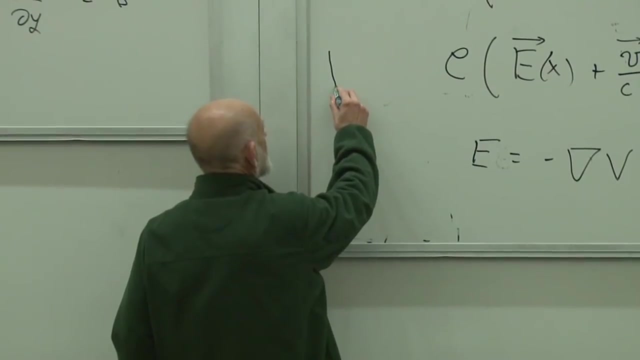 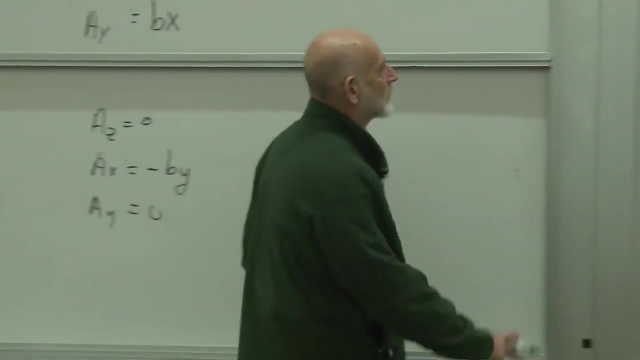 if I remember, but this is the piece which is which Lorentz properly gets credit for. is there a symbol for that whole thing? like up above you have F equals F, L. yeah, it's called the mass times, the acceleration. it's called force, yeah, force. 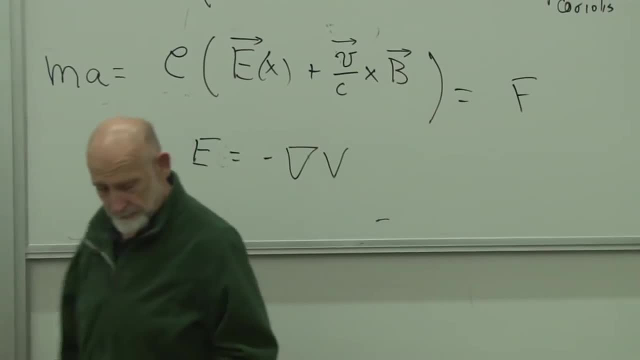 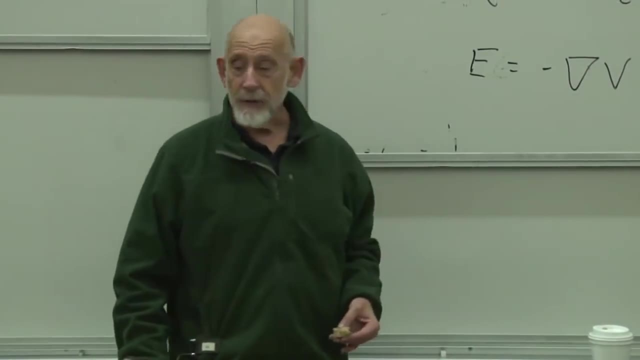 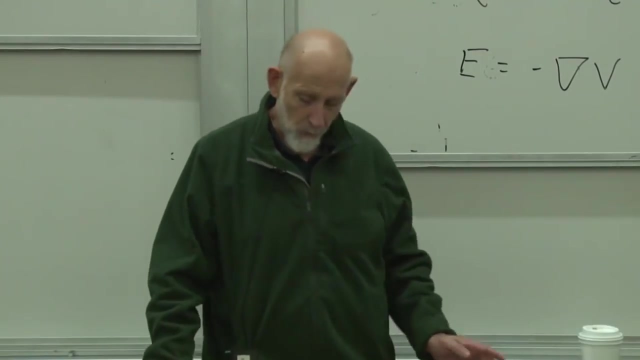 combined electric and magnetic force. now, of course they're deeply related to each other, the electric and the magnetic force, but they're related through relativity. so we're not. that's not where we're going tonight. yeah, I may remember this incorrectly, but I thought that the Coriolis force 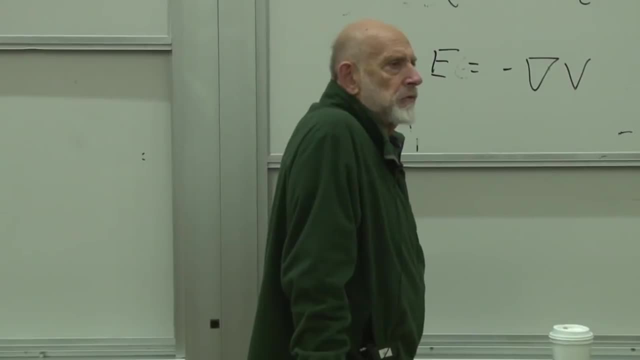 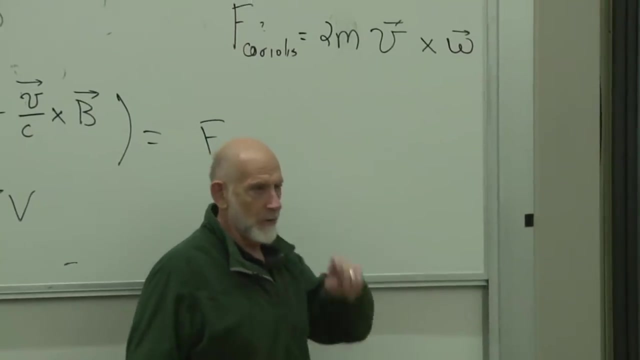 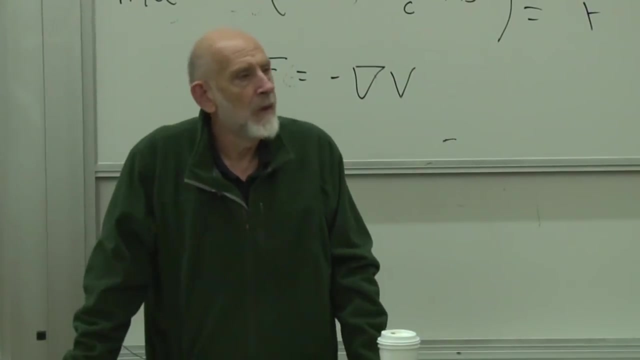 is not really a force, because it's a function of velocity, not acceleration. no, so you've got. there's the same thing there. so is that a real force associated with it, or which one? either Coriolis force or the electrical? I think the word real should be. 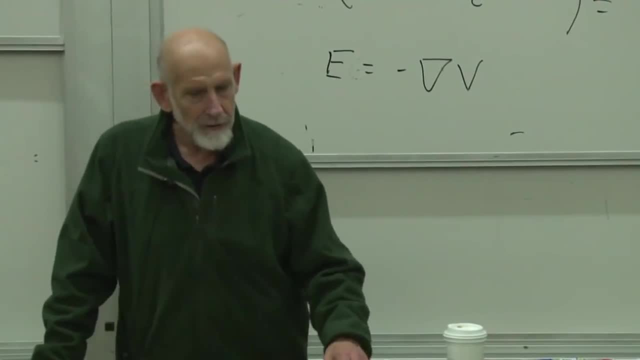 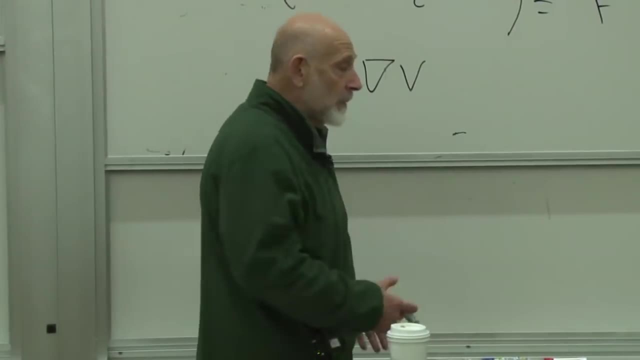 purged out of a physicist's vocabulary. does it exert a force that you could measure, or is it just part of the equation? if you're on this rotating turntable and you have a particle and you move it around with your hand, you'll feel a force on it. 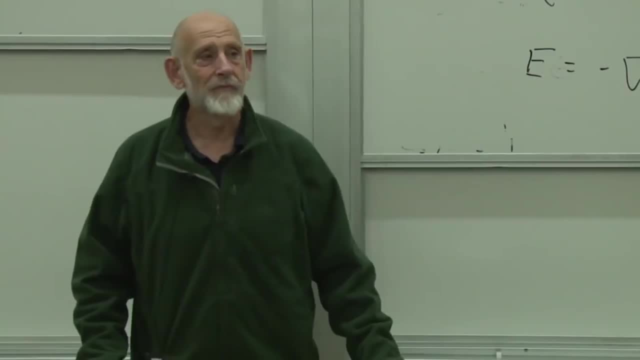 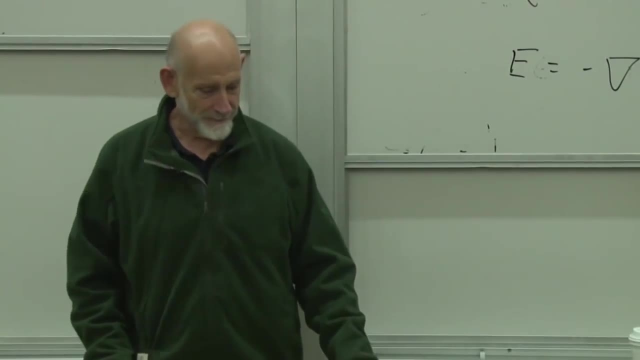 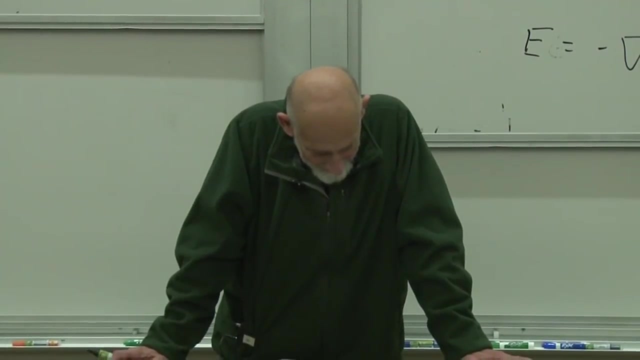 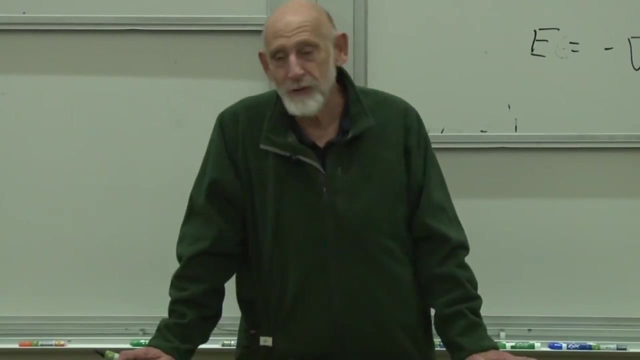 as real as anything. nevertheless, it's called a fictitious force. laughter, laughter, laughter, laughter, laughter. it doesn't exist in an inertial frame of reference. it doesn't exist in an inertial frame of reference, but to some extent, an inertial frame of reference is defined to be one for which it doesn't exist. 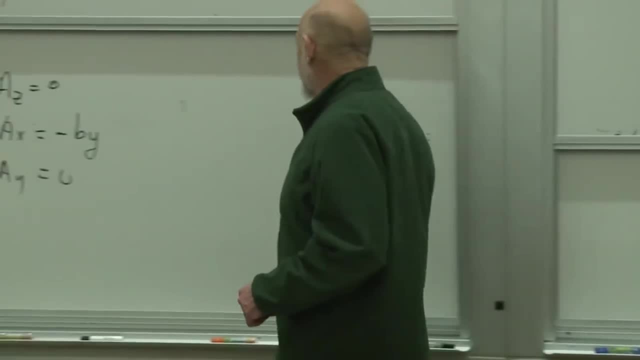 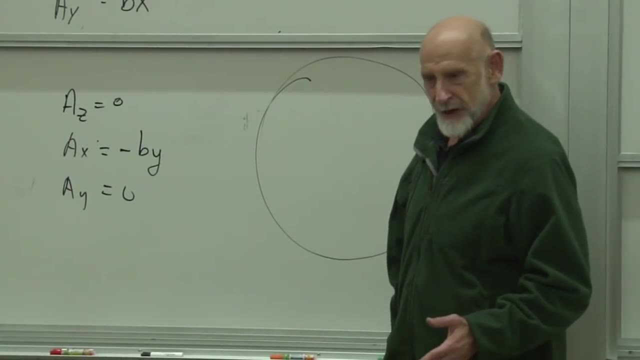 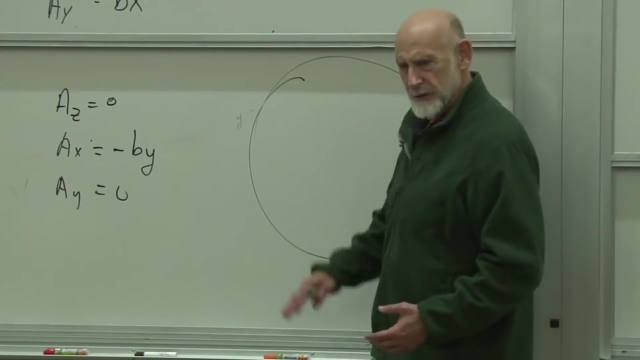 you can do some interesting tricks. incidentally, let's suppose you have a rotating turntable. now of course there is a centrifugal force. that's there. you could get rid of it by arranging some electrostatic attraction toward the center with an appropriate, with an appropriately distributed. 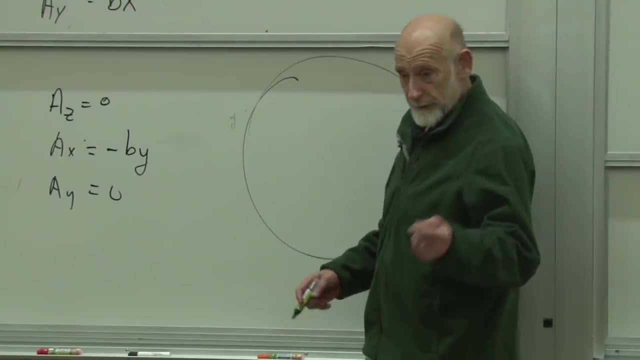 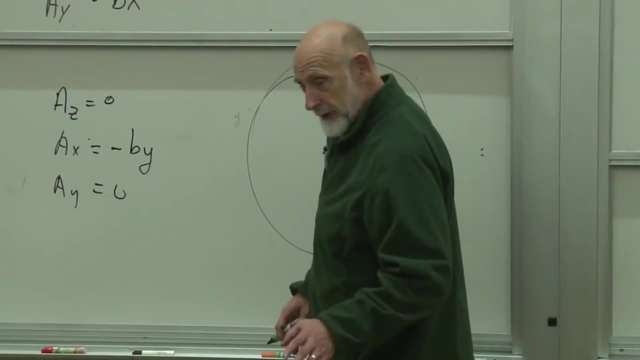 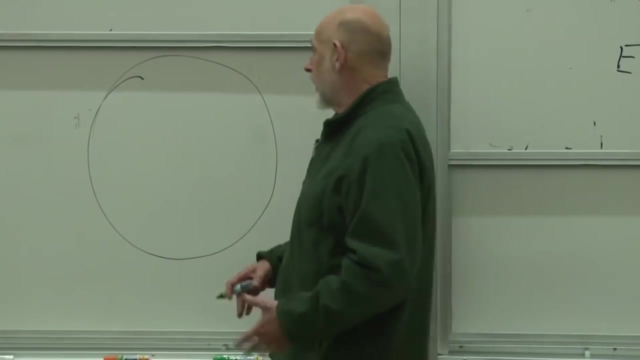 charge density for a charged particle. for a charged particle moving on this thing in the rotating reference frame, rotating in the reference frame charged particle, there will be a centrifugal force. it's pointed radially outward. can you get rid of it by a suitable distribution of charges in here? yes, you can get rid of it by a suitable distribution of charges which cancels the um, the centrifugal force. can you arrange a system of charges which will get rid of the Coriolis force? no, and the reason is: Coriolis force is proportional to the velocity. 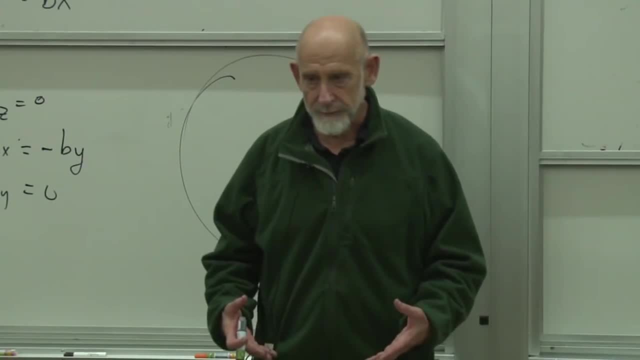 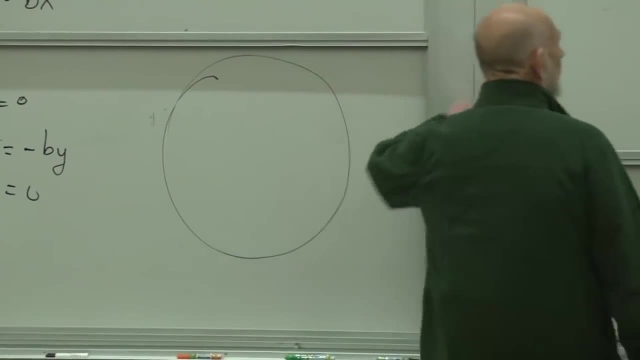 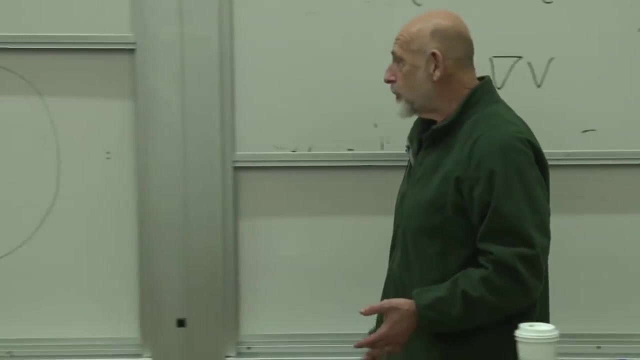 but electric forces, electrostatic forces are not. but what you can do is you can put a magnetic field of just the right magnitude that the Coriolis force and the magnetic force cancel each other. so with an appropriate distribution of charges and a uniform magnetic field of the right, 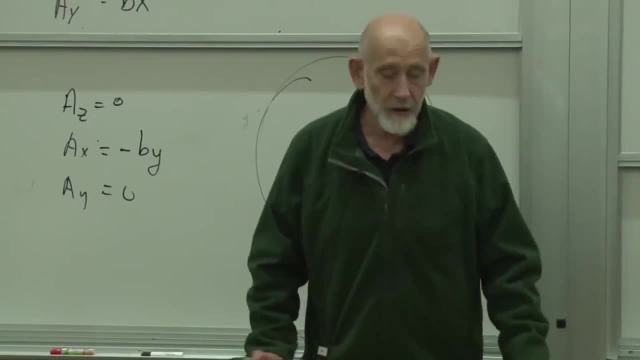 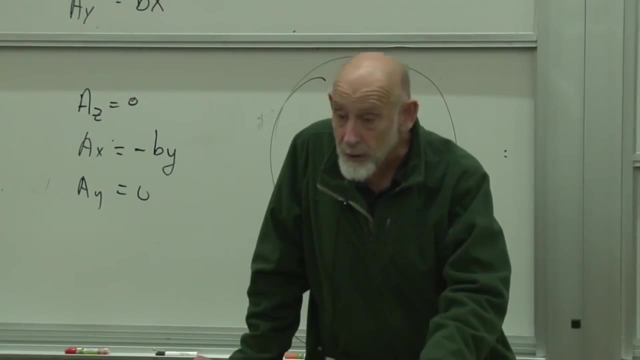 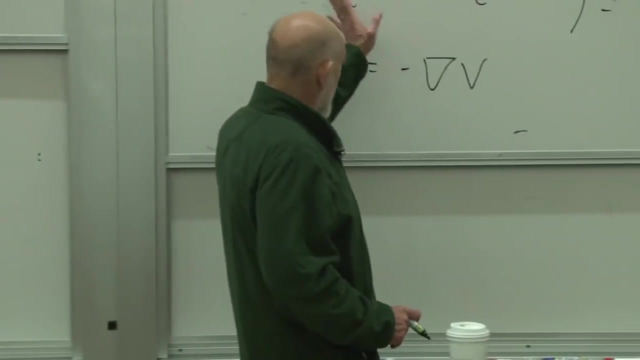 magnitude, you could get rid of all the fictitious forces on in a rotating, turntable situation. of course, if you did it for a particle of one charge, it wouldn't work for particles of other charges. why? because the magnetic forces and electric forces are proportional to the electric charge. 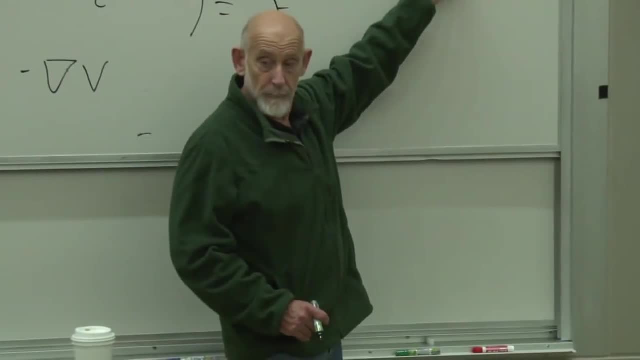 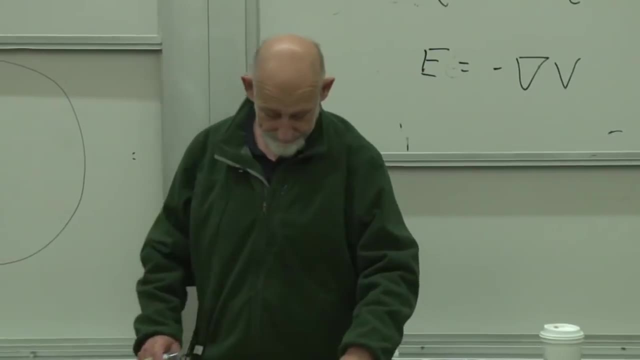 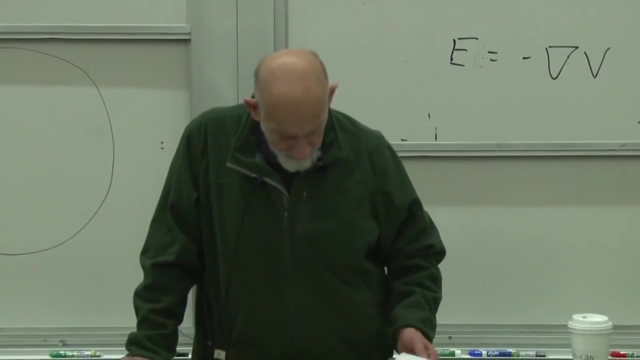 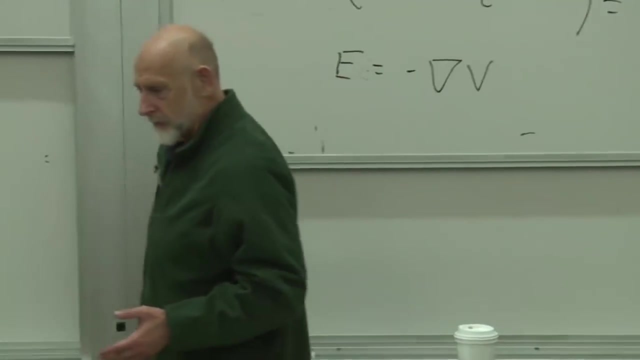 but these fictitious forces are not, so you can only cancel them for one value of charge, but you could cancel them for the electrons. okay, so now, what are we interested in now? we would like to know whether this force law can be derived from an action. 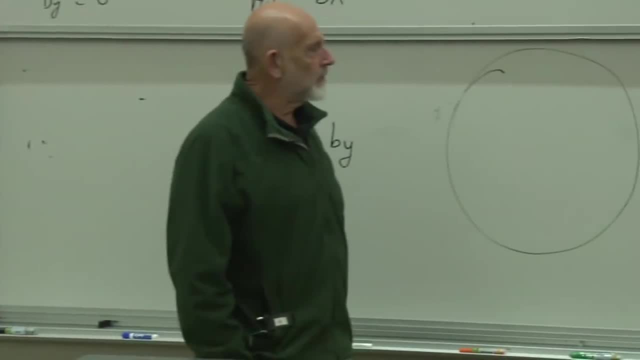 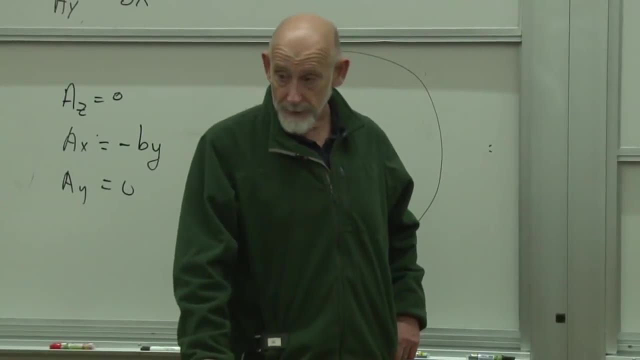 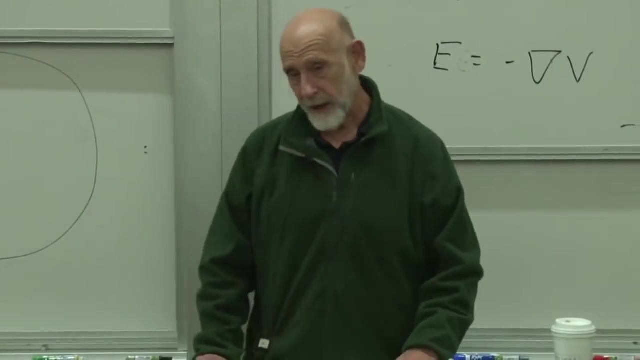 principle? um, the answer is yes, but it's at a cost, the cost being that you have to introduce the vector potential. you cannot do it without the vector potential. I'm going to let you try. I know how to prove it. I once proved it. I sat down and convinced myself. 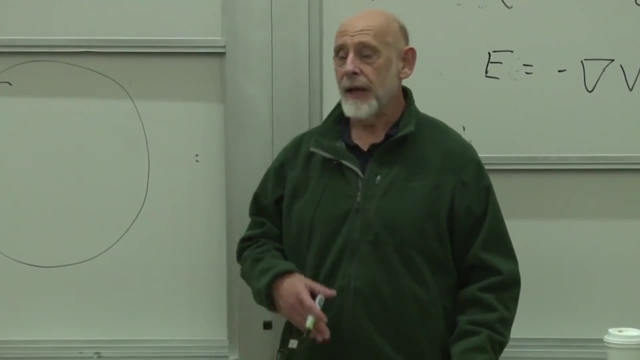 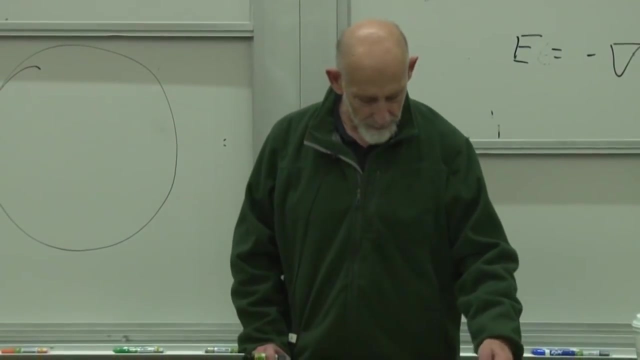 of a simple mathematical argument that with just the magnetic field alone and the particle, even with velocities and so forth, there's no way to do it. I will let you try to do it, but instead of trying to prove the theorem, what we're going to do is the opposite. 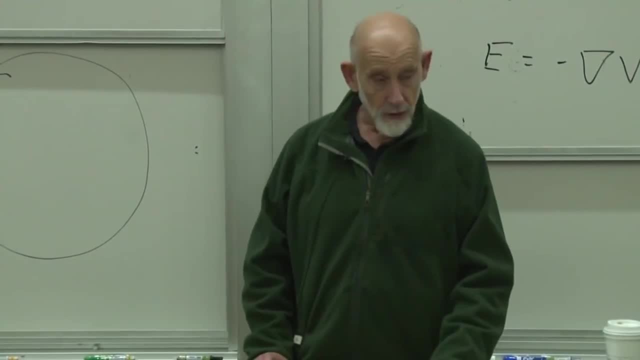 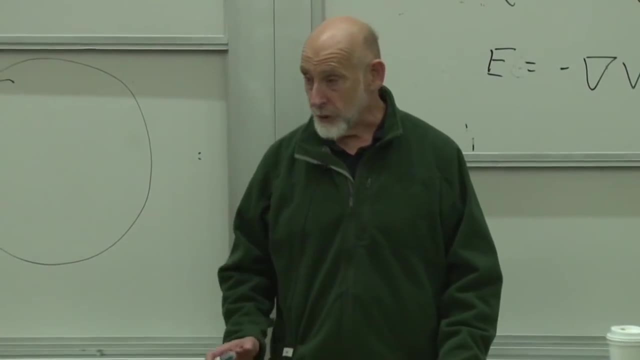 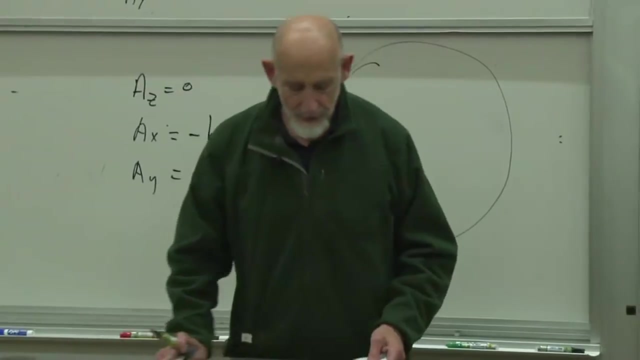 we're going to construct the Lagrangian and the equation Lagrangian- the action for a particle in a magnetic field, and then show that it gives exactly this force. the electric part of it is easy. I'm not even going to bother with the electric part of it. 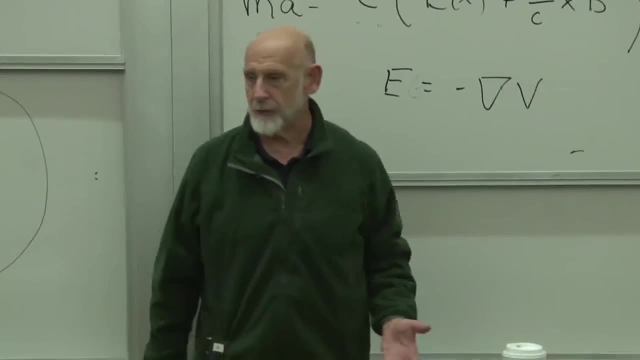 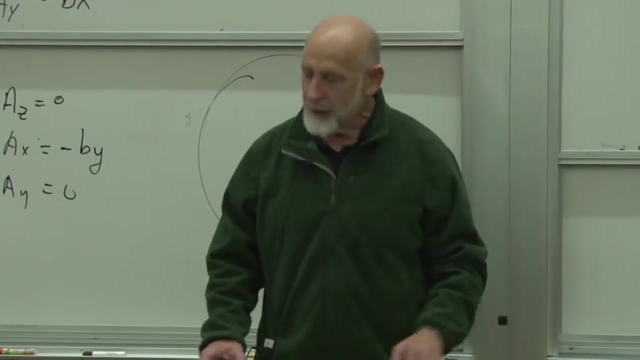 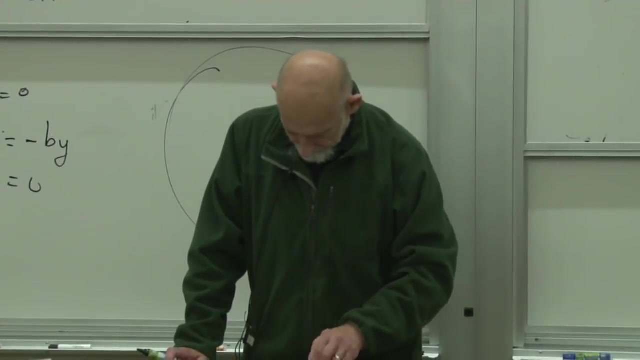 the electric part of it is just: the particle has a potential energy and you put it into the Lagrangian kinetic minus potential energy. that's standard. the non-standard thing is the magnetic force. so let's concentrate on that. let's think about the things that we could put into the Lagrangian. 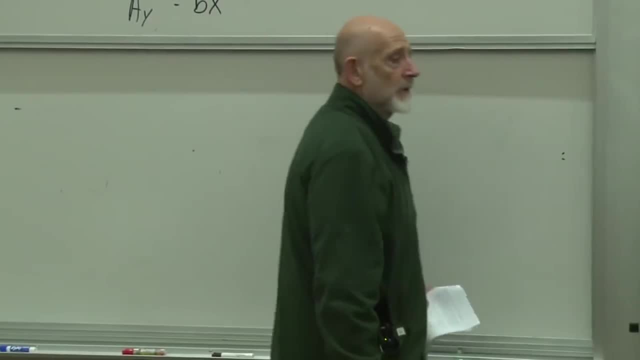 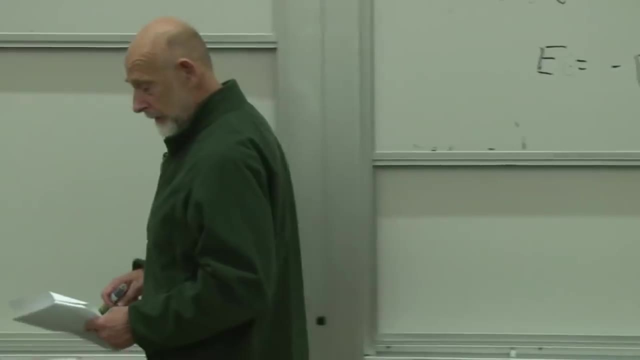 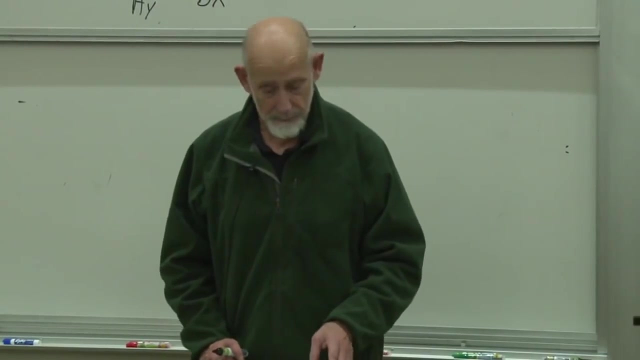 let's start with a particle with no forces. I don't know if we're going to get through it tonight or not. it's not important. we have another week. I'm not going to start a new subject next week, so we have time to do this slowly. 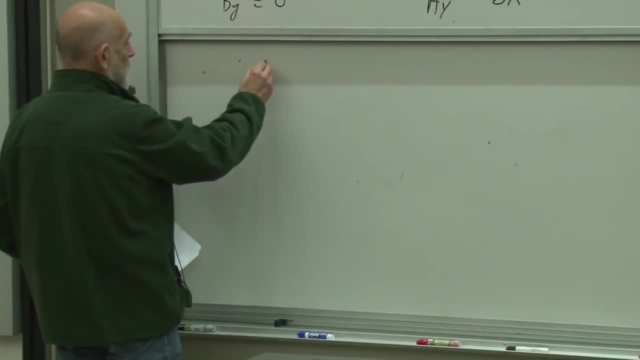 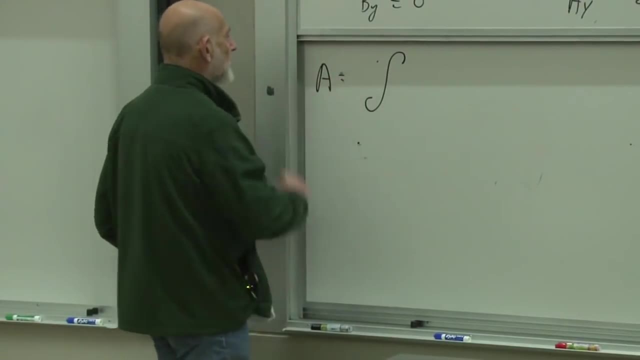 we have to build a Lagrangian. we're going to build an action principle. we're going to build an action principle and the action principle is that there exists an action. I'm sorry that action and vector potential have the same symbol. I can't help it. 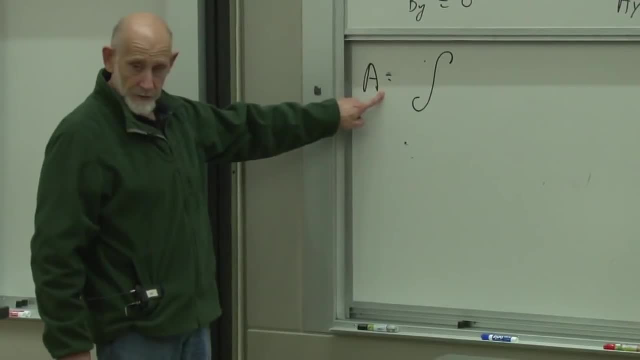 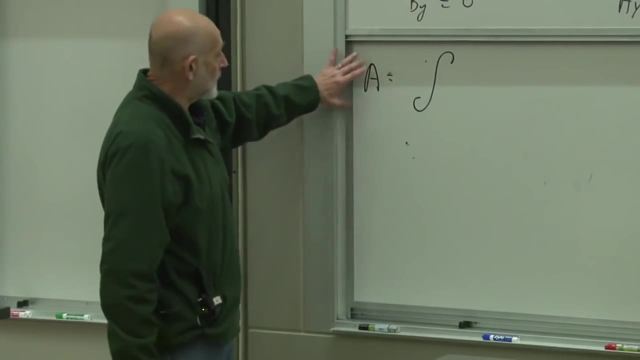 but I won't put an arrow on top of it and I won't give it indices, I won't give it components A just standing alone, like that doesn't stand for the vector potential, it just stands for the action. the action is always for a particle we're only talking about. 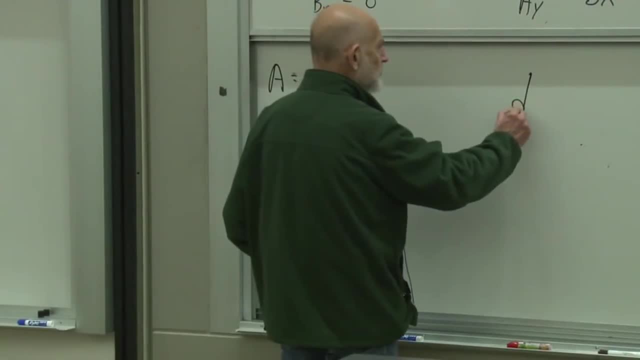 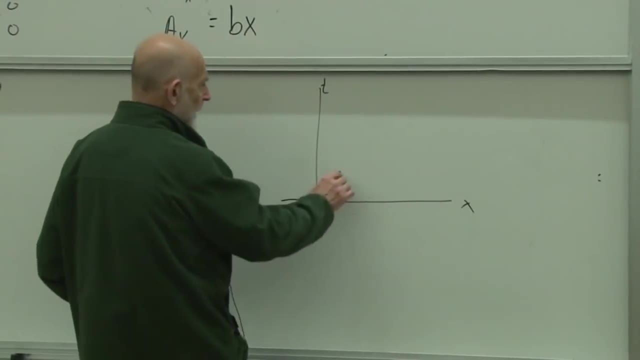 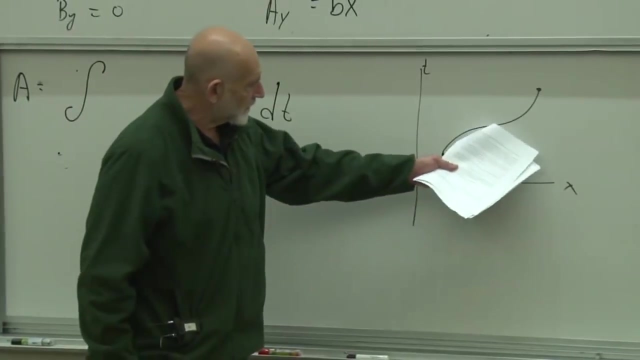 one particle. now it's an integral along the trajectory. here's a way to think about it. we have space and we have time, and the particle moves along some trajectory. it moves along some trajectory, moving awfully fast over here, isn't? it moves a huge distance. 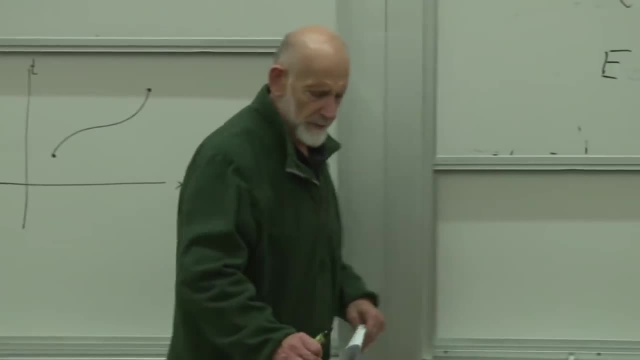 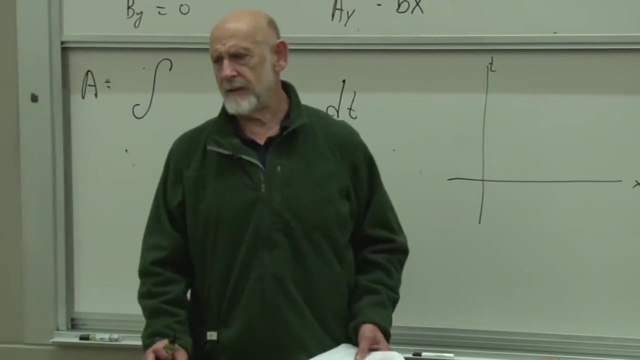 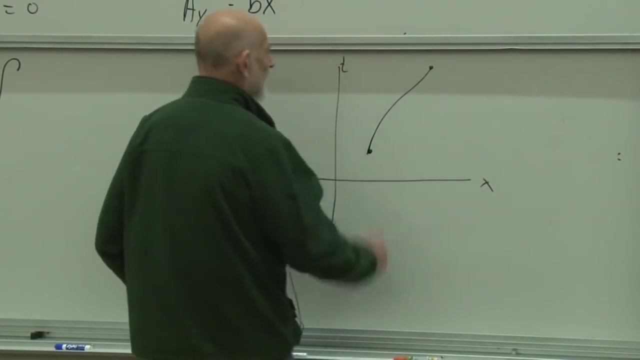 in a short time. it's moving too fast. it's exceeding the speed of light. we don't want to do that. if it was a neutrino it would be okay, but this is a charged particle and so far nobody's right, so let's do it like that. 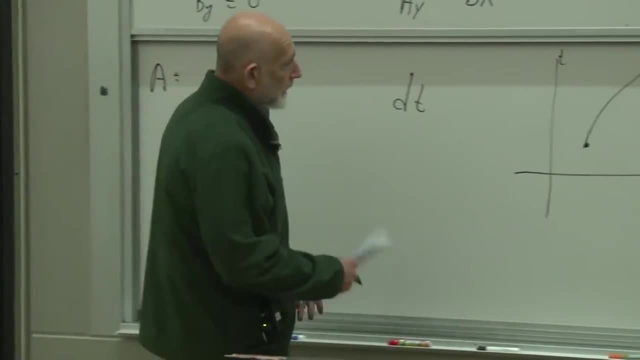 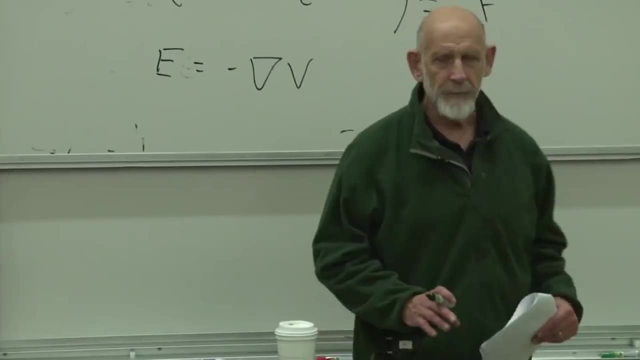 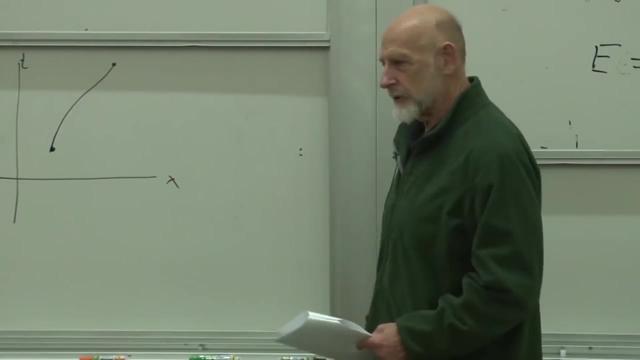 let me just remind you what the action principle says. the action. I'm going to talk about the principle of least action. but it's not really least action, it's stationary action. but nevertheless I'll use the terminology least action just because it rolls off the tongue more easily than stationary action. 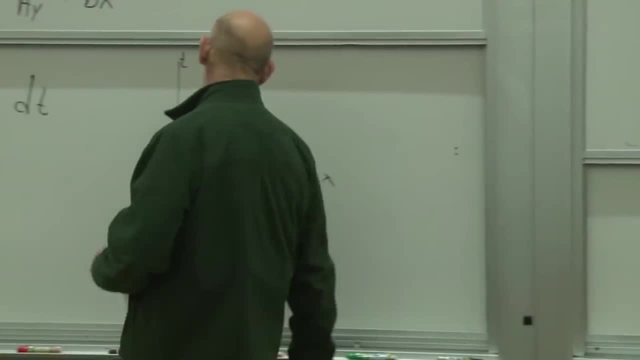 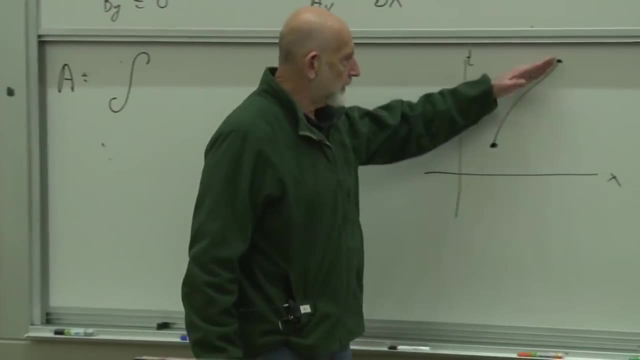 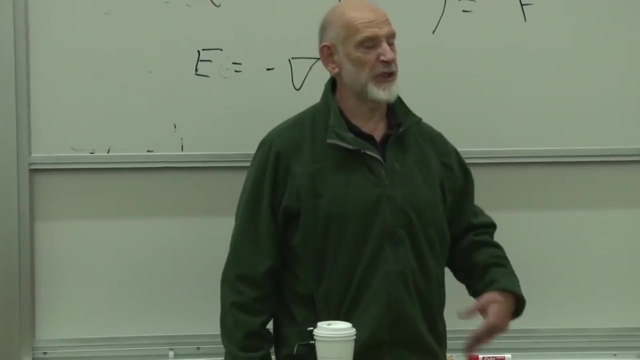 alright. what is the principle? the principle says: first of all, there exists an expression called the action. it's an integral along the trajectory and the rule is: the true trajectory should minimize or stationerize. see, that's the hard one. stationerize, I don't know, it's not a good verb. 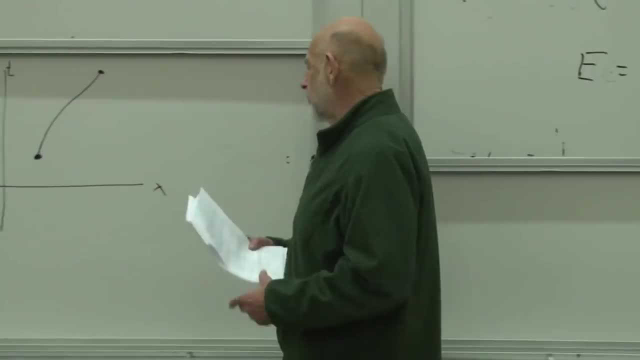 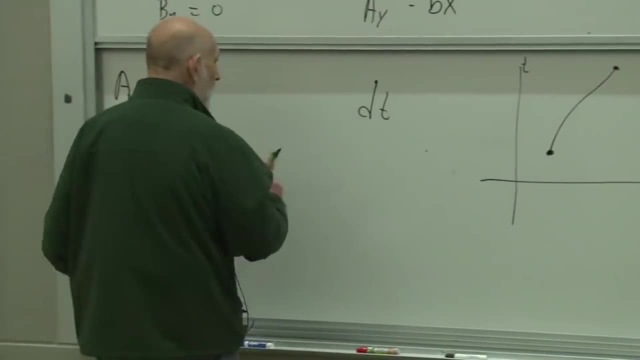 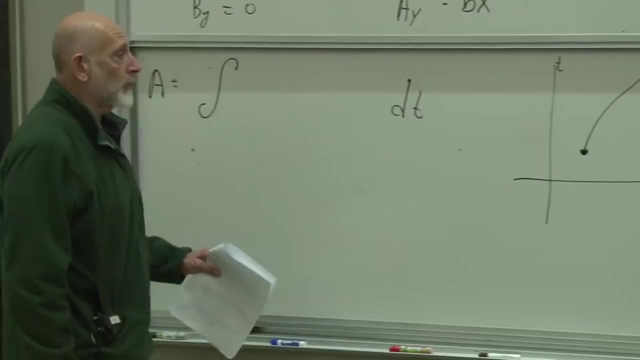 so we'll say minimize, minimize the action along the trajectory. all we need, then, is an expression for action and the expression for the action, oh oh. we hold the two endpoints fixed. this is important. we hold the two endpoints fixed and then vary the trajectory in different ways. 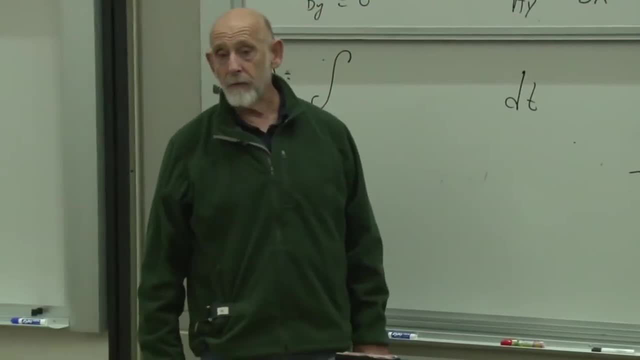 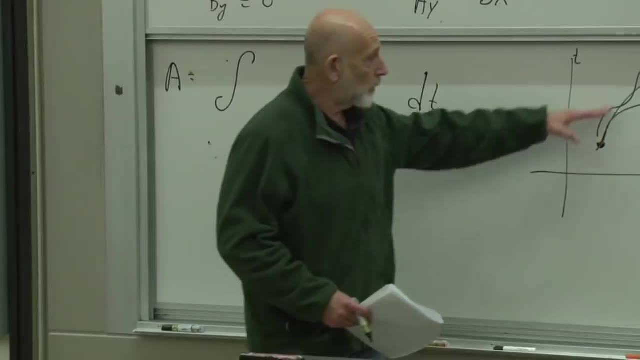 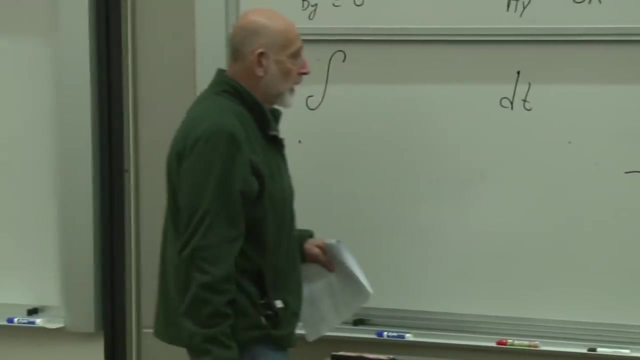 and ask for the trajectory of least action. that defines the true trajectory and using the principle, we work out the Euler-Lagrange equations, which are the equations of motion. just reminding you now. ok, so there's nails in the blackboard which hold these points fixed. 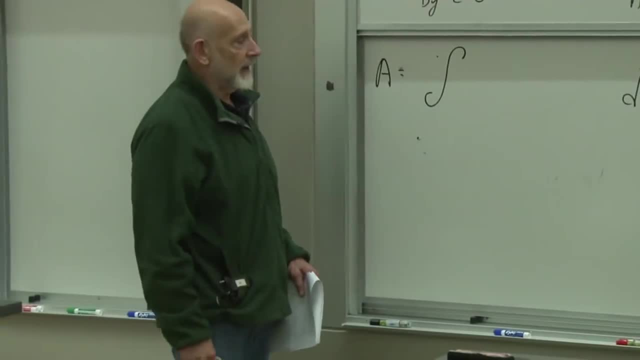 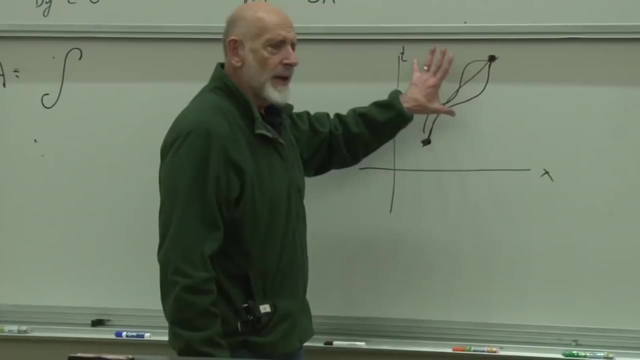 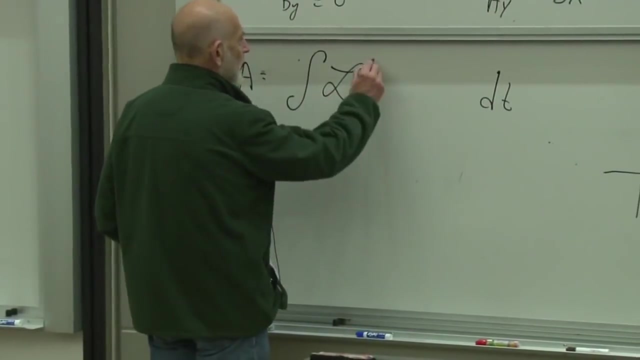 and then we wiggle the string and ask: what configuration? this is not string theory. we wiggle the trajectory and ask what trajectory minimizes the action? ok, what is the action? the action is the integral of a Lagrangian. and what does the Lagrangian 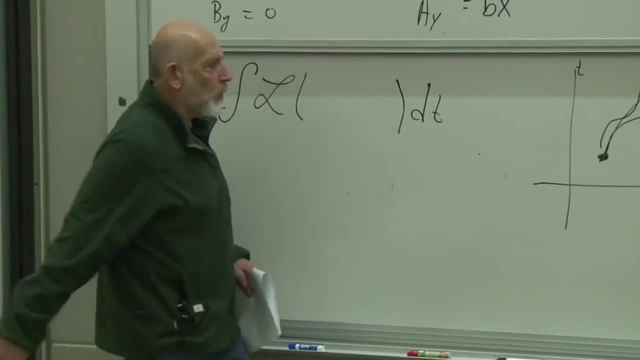 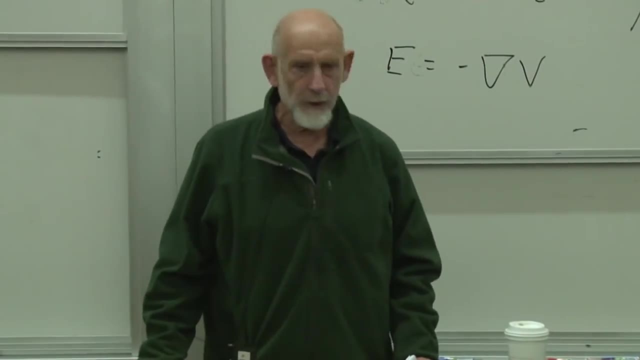 depend on the Lagrangian, depends on the coordinates and the velocities at any given time. we're going to use- I'm not going to use- the notation q for coordinates, because we're really now talking about x, y and z. we'll call them sometimes x1, x2. 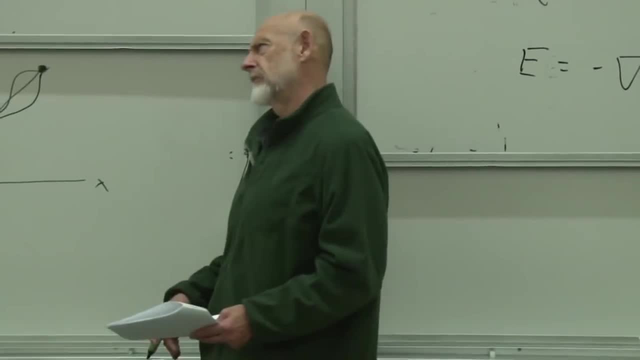 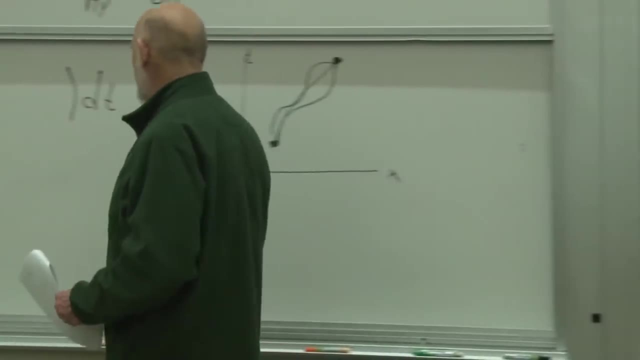 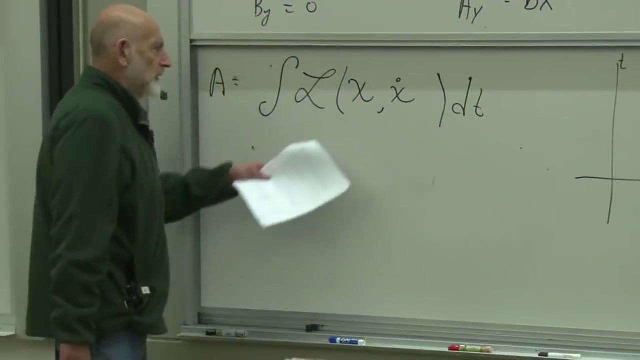 and x3, sometimes xy and xz, sometimes x1, x2, x3, y and z. so, generally speaking, we can call this a function of x's and x dots, without overly labeling things with i's and j's, and things a function of positions. 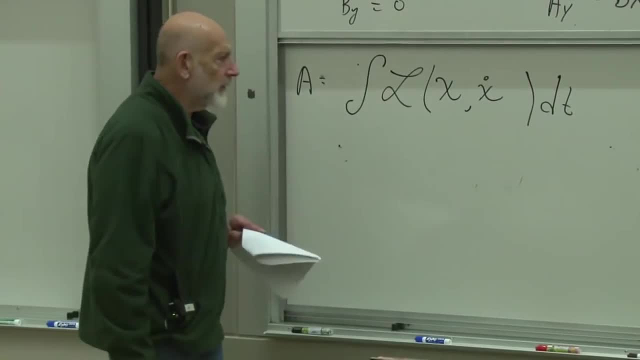 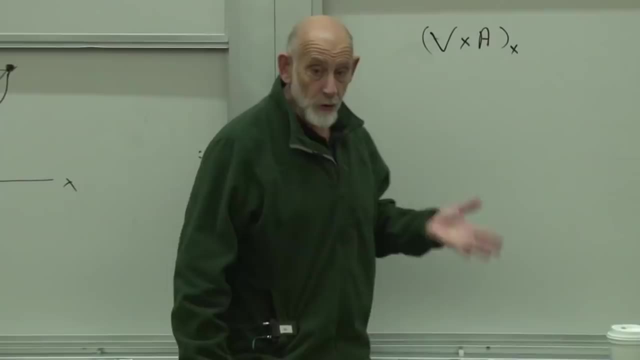 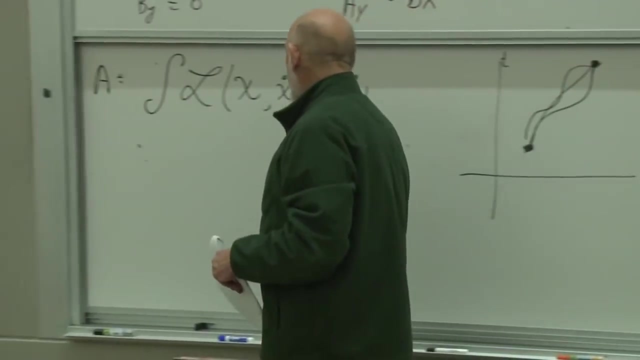 and velocities. if we know L, then through the Euler-Lagrange equations of motion, we figure out, we reproduce Newton's equations or hopefully, the Lorentz force law. ok, what kind of things can we write in the Lagrangian? well, first of all, if we turned off all fields, 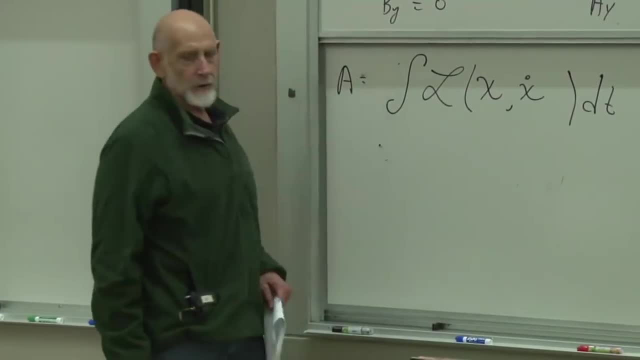 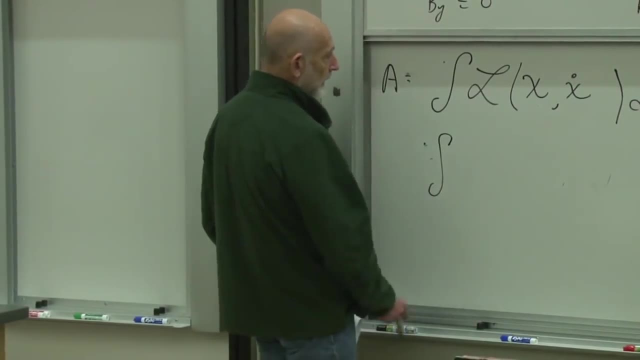 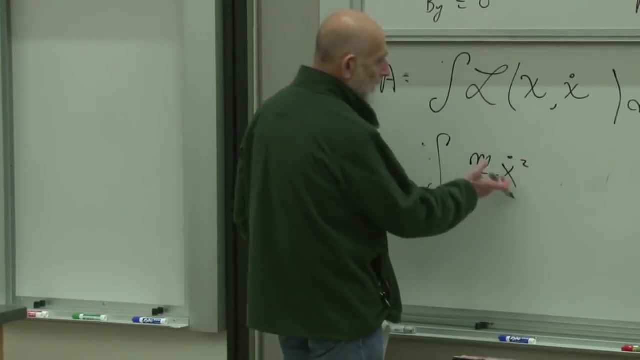 if we turned off all fields, we would expect this Lagrangian just to be the kinetic energy. no forces, just the kinetic energy. and so we begin with the mass of the particle divided by 2 times x dot squared, and this means the sums of the squares. 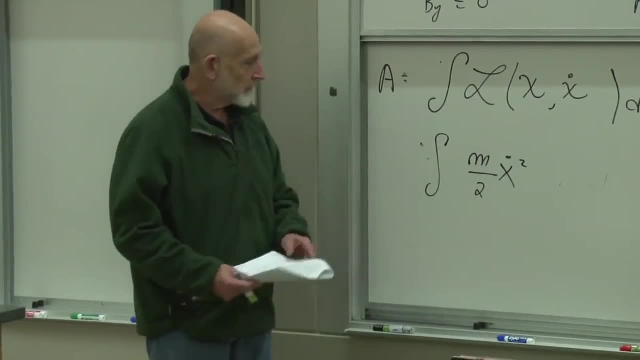 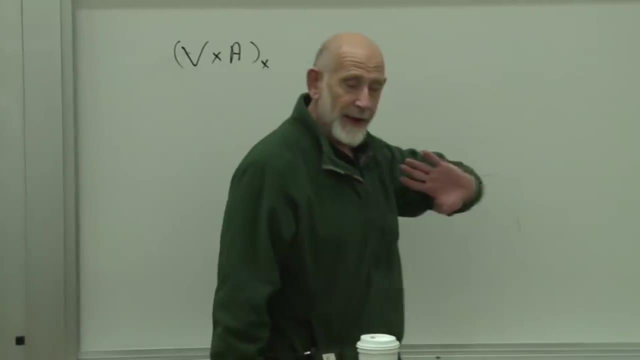 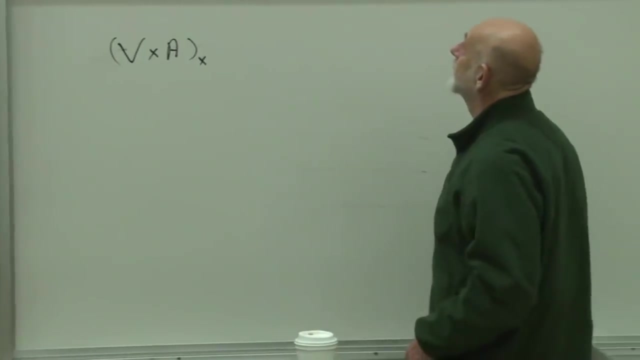 x component, y component and z component of velocities. that's straightforward. now we want to add something that will give rise to a new kind of force. let's forget electric forces. what do you think we do for electric forces? we just subtract the electrostatic. 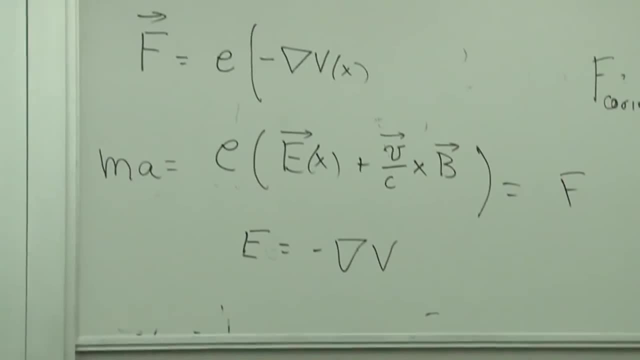 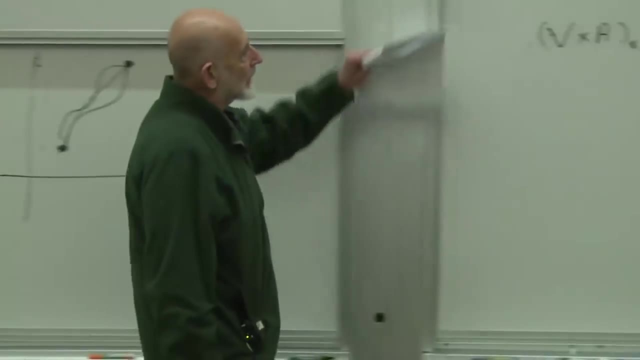 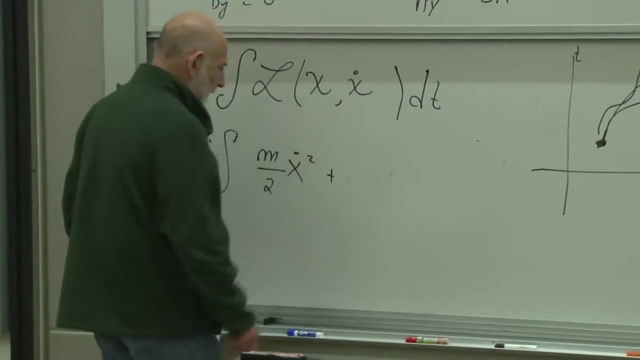 potential energy. I'm not even going to worry about it. we'll worry about it some other time. now we want to reproduce the magnetic term, alright, so what do we expect is going to be here? well, first of all, it's going to be something we're going to add. 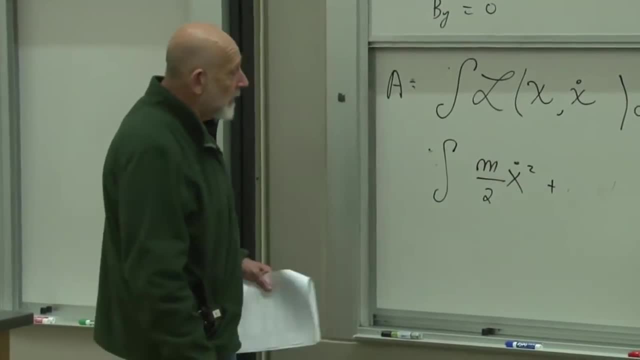 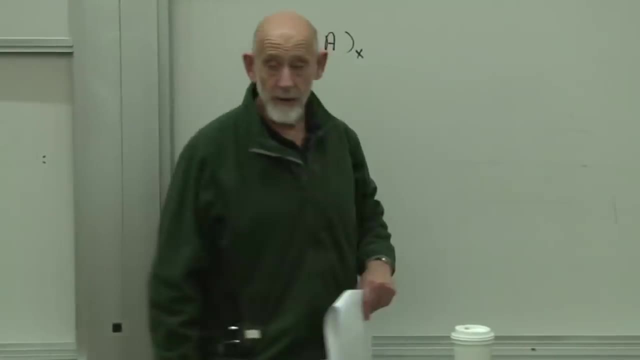 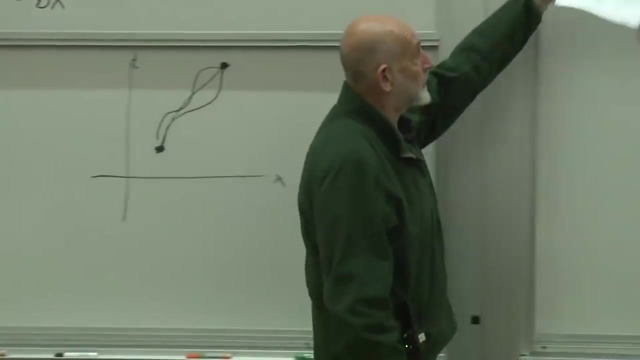 what can it depend on and what should it depend on? first of all, it ought to be proportional to the electric charge. the electric charge occurs in the formula, so it's likely to have an electric charge in it. the electric charge always comes in, at least in the magnetic forces. 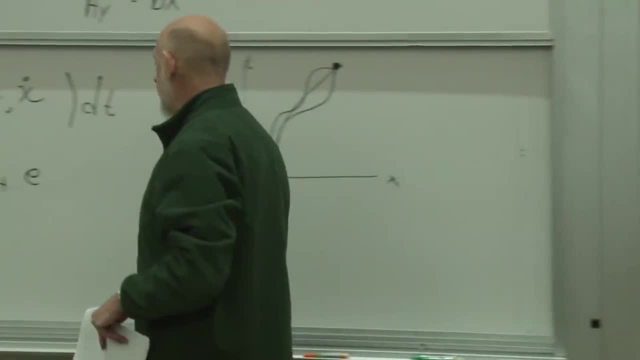 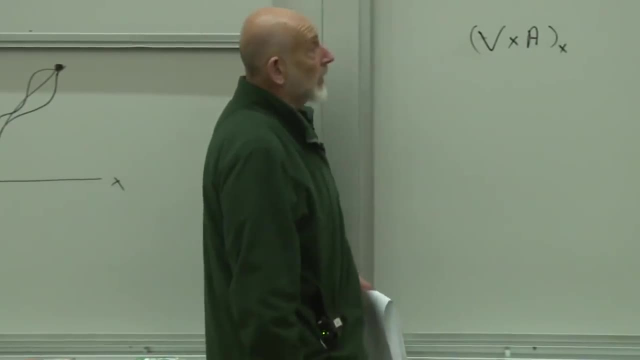 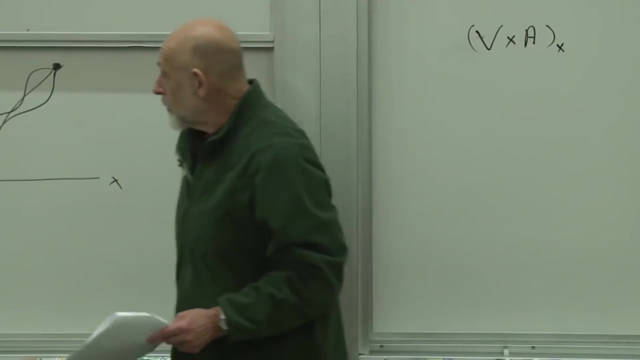 the magnetic side here divided by the speed of light. so we can expect there will be an e over c in there. we expect a velocity, but for sure we expect somehow something proportional to the magnetic field. so we could try putting the magnetic field itself in here. I'm going to leave it to you. 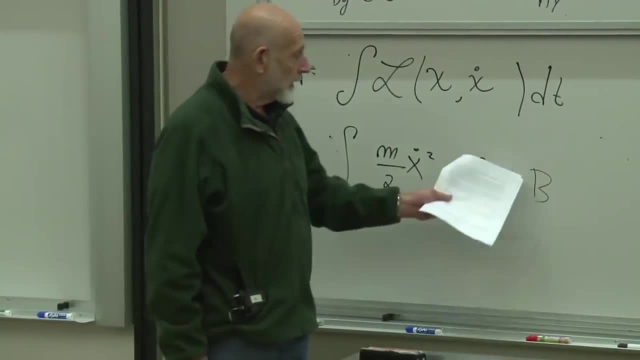 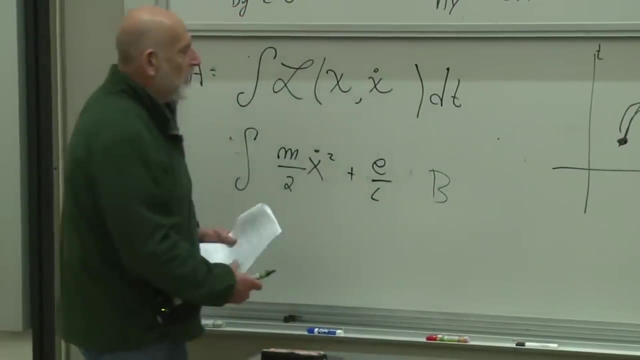 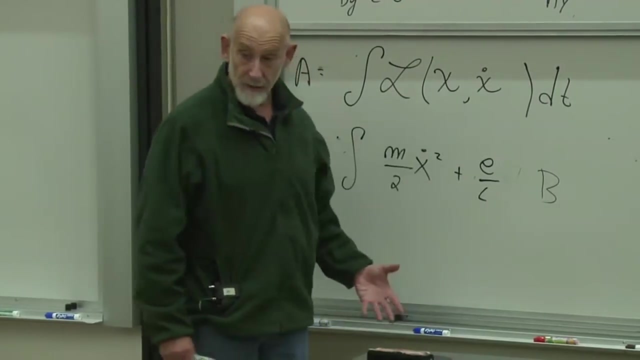 to experiment around and show that you cannot reproduce this formula. incidentally, what would you do with the magnet? alright, let's try it. what would you do if you put the magnetic field here? the magnetic field has components and the Lagrangian is a scalar. the Lagrangian is always a scalar. 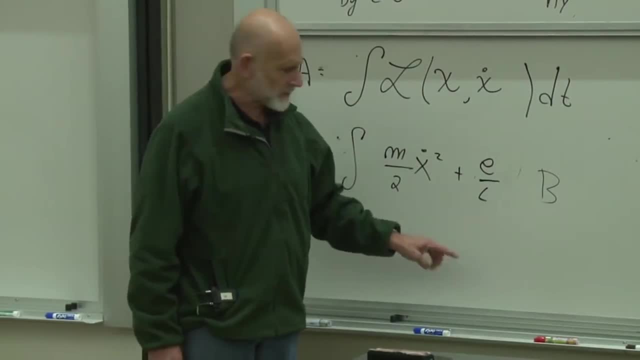 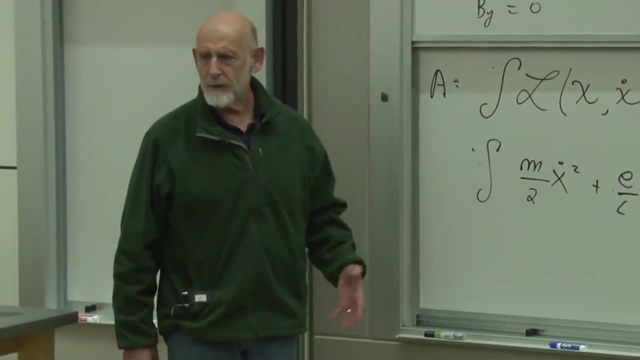 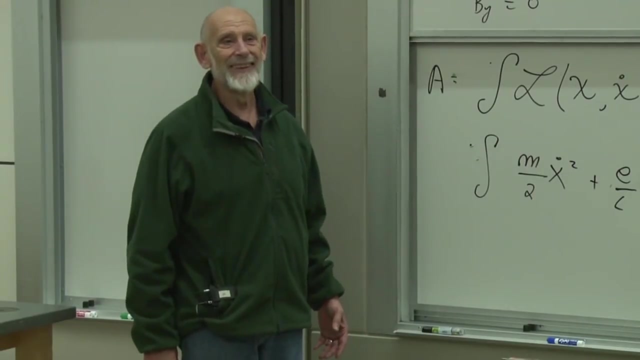 it contains kinetic energy, it contains potential energy, but it doesn't have components. you know Cartesian components. so if we're going to put the magnetic field in here, we have to do something to it to make it into a scalar. what can we do with it? what's that? 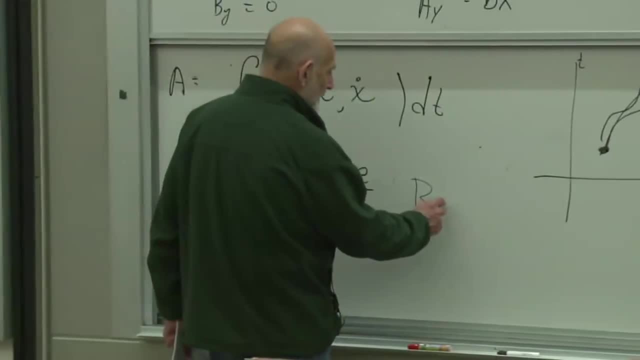 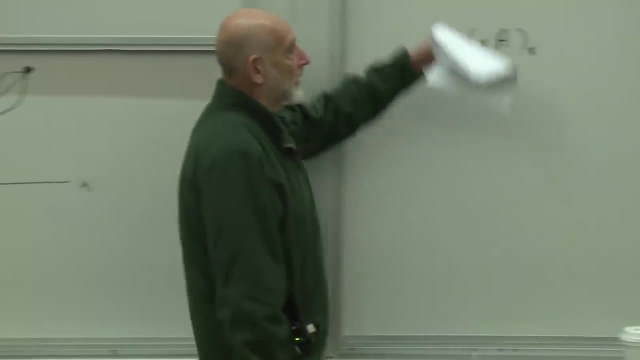 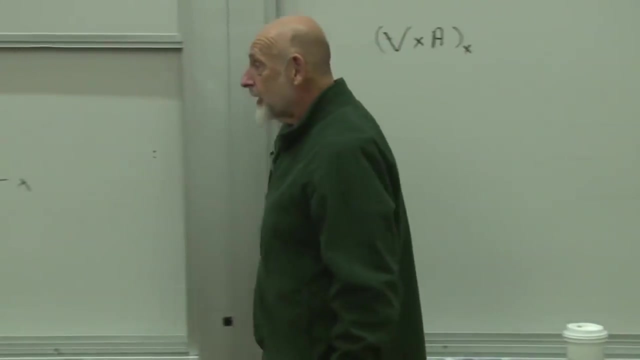 yeah, okay, let's dot it into something what's around to dot it into? the obvious and natural thing is to dot it into the velocity. we're trying to get out a force that's proportional to the velocity. we could try dotting it into the velocity and then working. 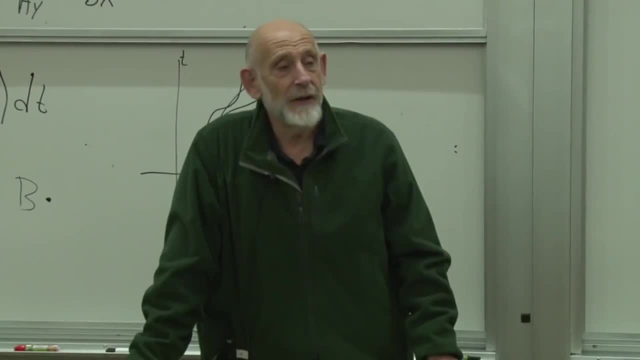 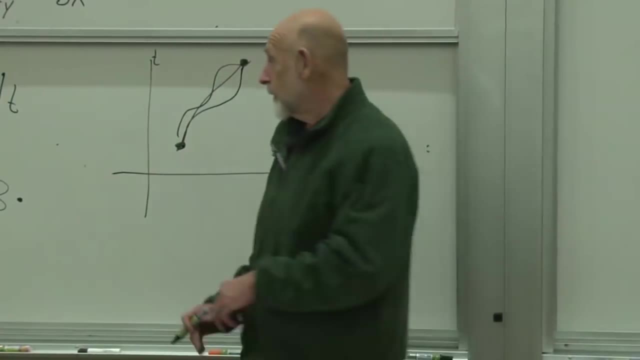 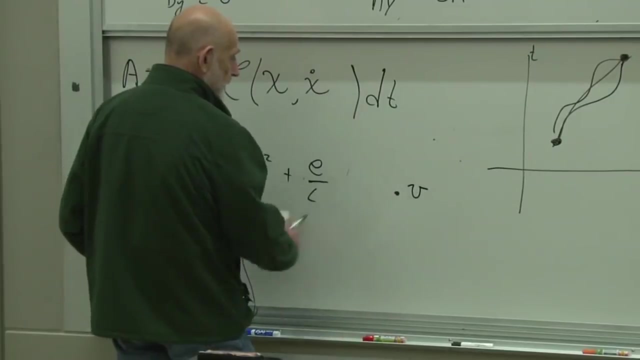 out the Euler Lagrange equations. okay, you can try that. no, no, you can try that. it's worth doing, but I will tell you right now it's the wrong answer. the right answer is to take the velocity and dot it into the vector potential. the vector potential is a function of position. 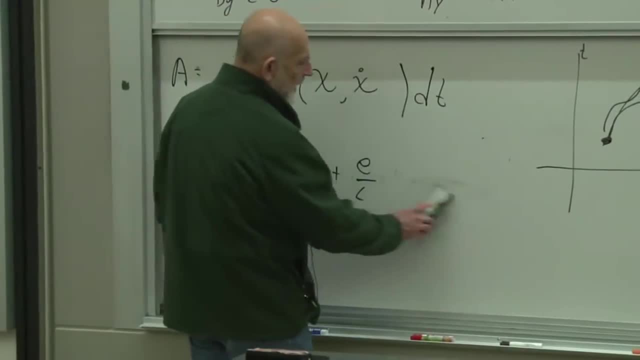 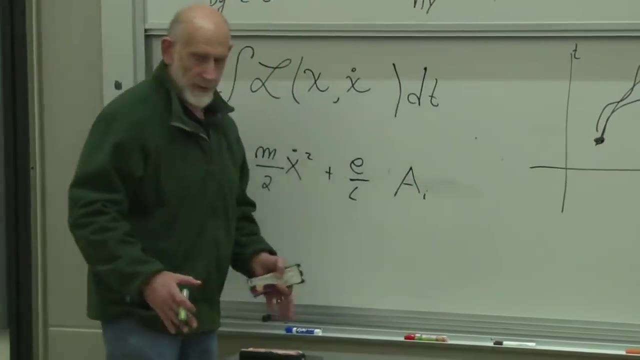 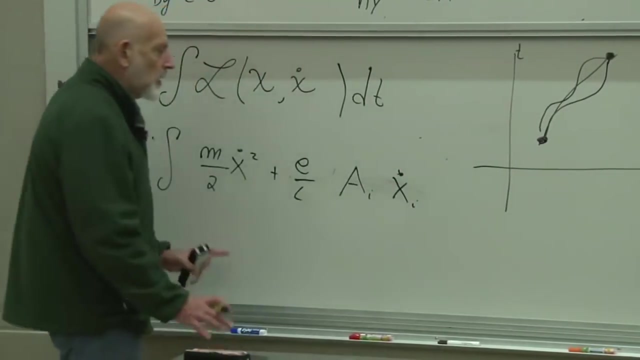 and so we can write this as the component, the ith component of the vector potential as a function of position. I'm not going to write over and over that, it's a function of position times. the ith component of the velocity summed over i, this is vector potential. 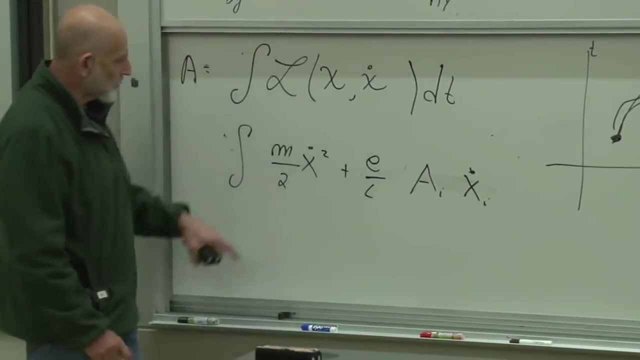 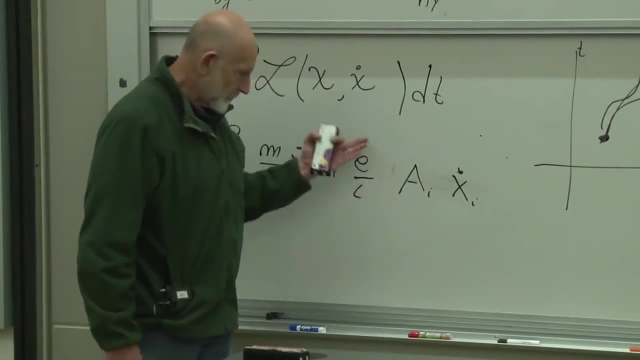 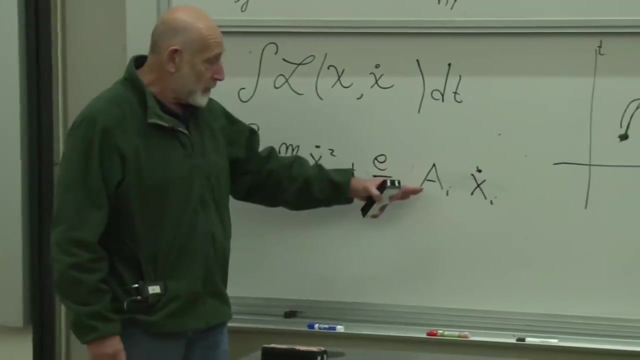 dotted into the velocity summed over i. this is also a sum over i, x sub i dot squared sum over i. this is vector potential dotted velocity. that's what it is. we could try putting b here and work out the equations of motion. we'll get exactly the same answer. 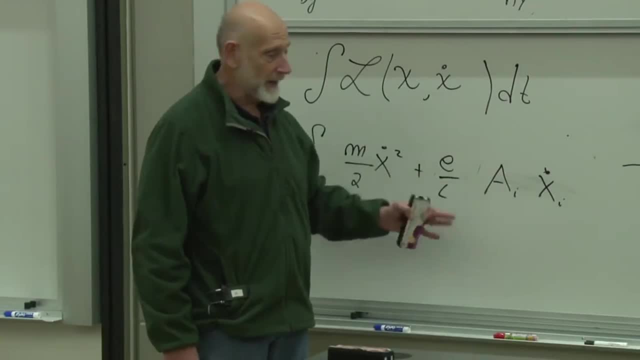 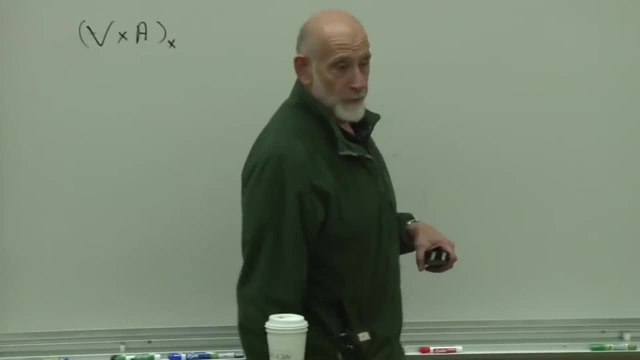 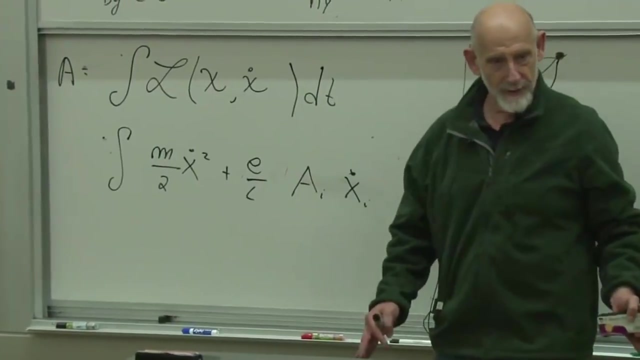 except we replace b by a, the question of which one of them- putting b here or a here- is going to reproduce the Lorentz force law. so whatever we put here, let's just call it a for the time being and see what we get out of this. 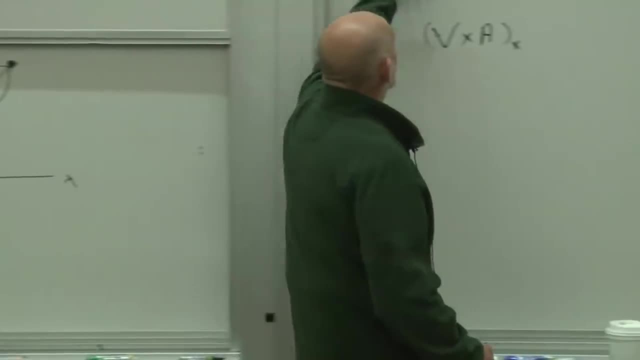 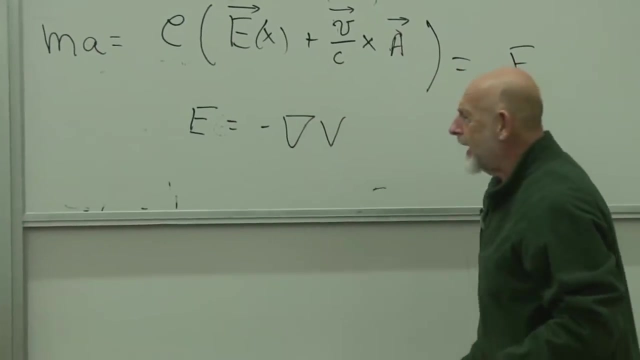 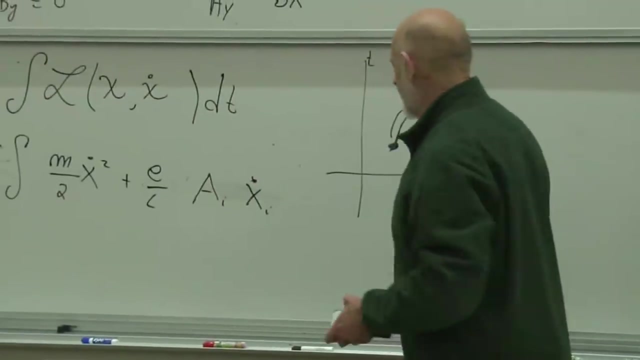 if we wind up getting that the force involves v over c, cross the vector potential, then we'll say, no, that wasn't right. hey, i got a good idea: instead of putting vector potential, let's put magnetic field. but that's not what's going to happen. what's going to happen is if we put a here, 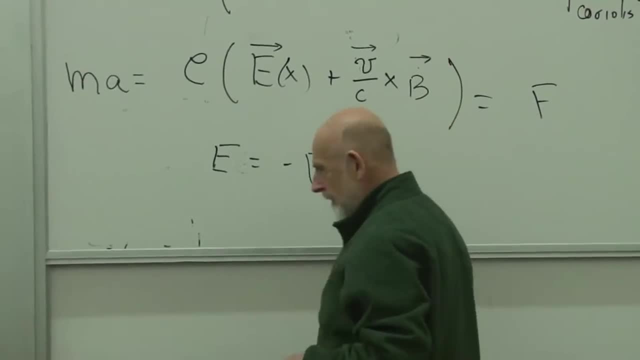 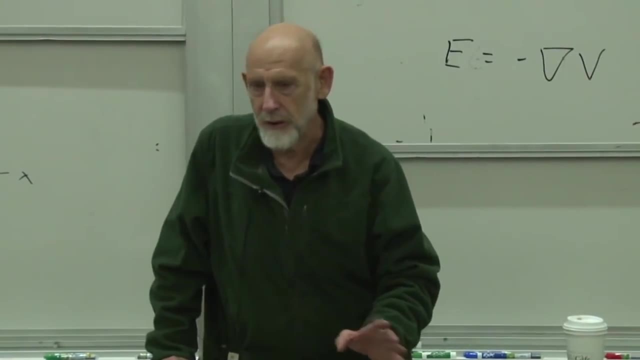 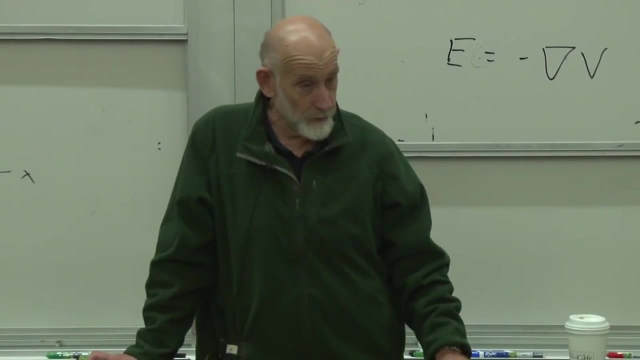 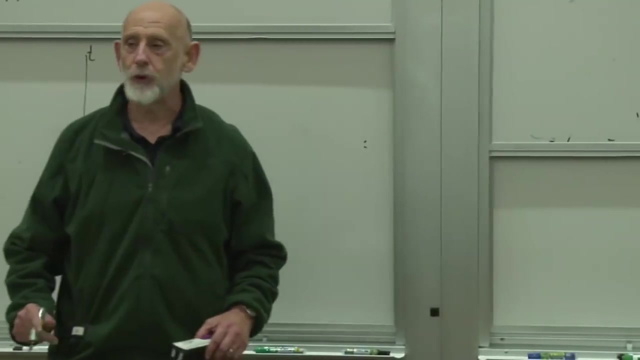 then we'll get b here. now there's an immediate question that should occur to you right now. a is not unique. a is subject to 1 gauge transformations. what's going to happen if i change a from one gauge to another? that's the language from one. 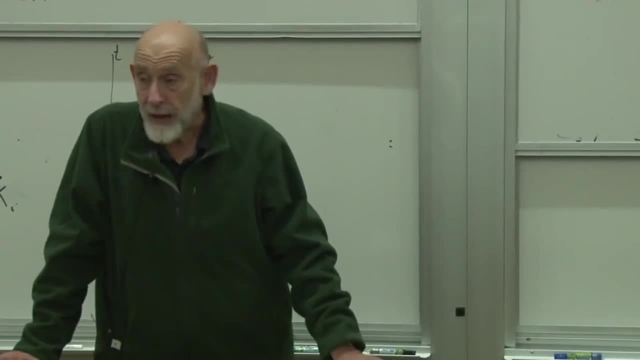 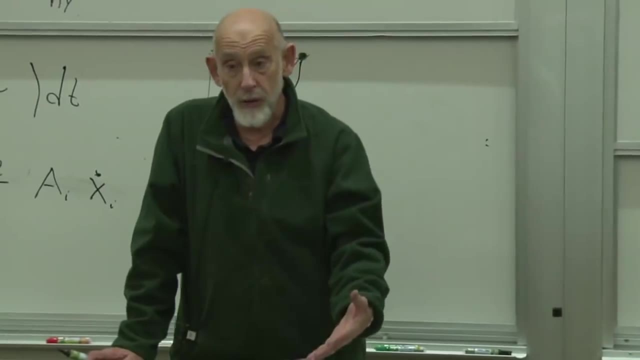 gauge to another, is the answer gonna come out to be the same? is the action going to change? and if it does change, is the change going to be of a form which will change the equations of motion? so what i'm going to do with the rest of the 10 minutes? 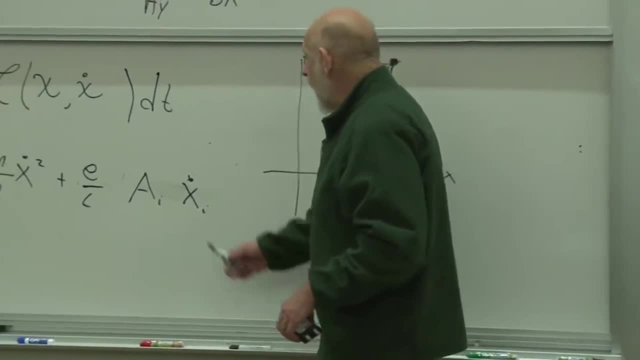 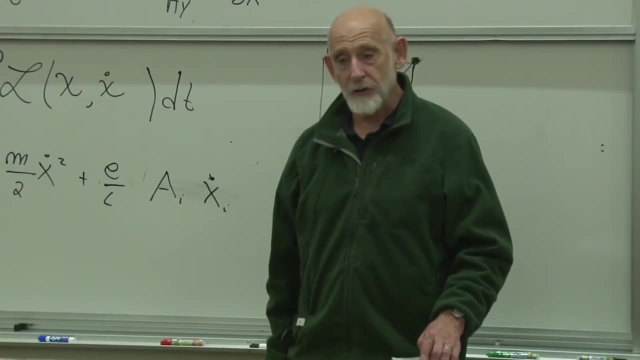 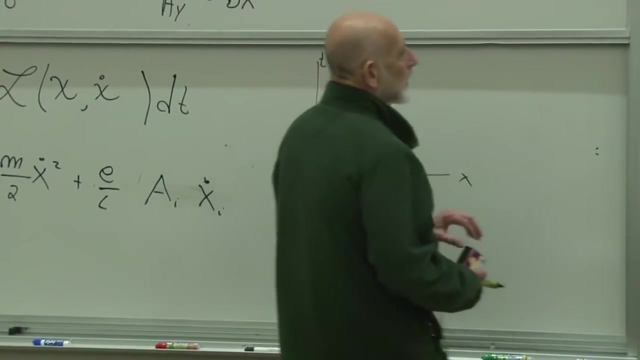 is, we may run out of time. show you why making a gauge transformation doesn't affect the equations of motion. it has a small effect on the action, but it's an effect that doesn't change the equations of motion. so let's go through that. here we are. 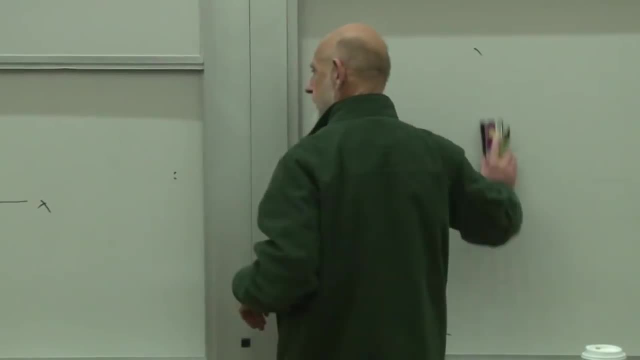 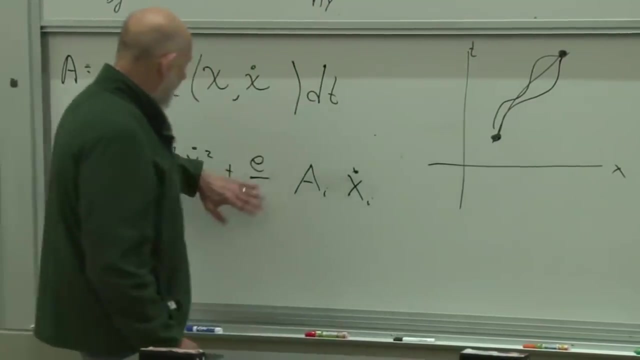 let's go over to this blackboard the new term that i advocate, that i'm advocating now to put into the lagrangian. let's write it over here. and let's forget e over c. not interested in that. what i'm interested in is the integral of a, dot, x, dot. 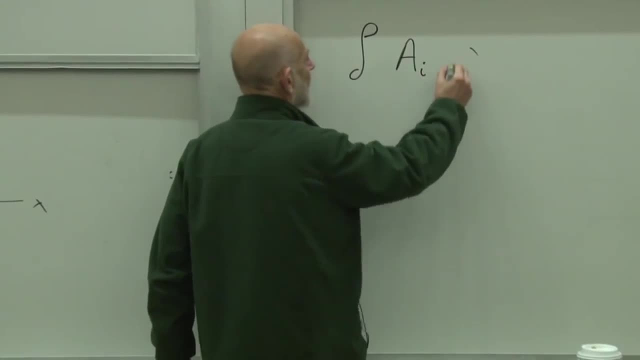 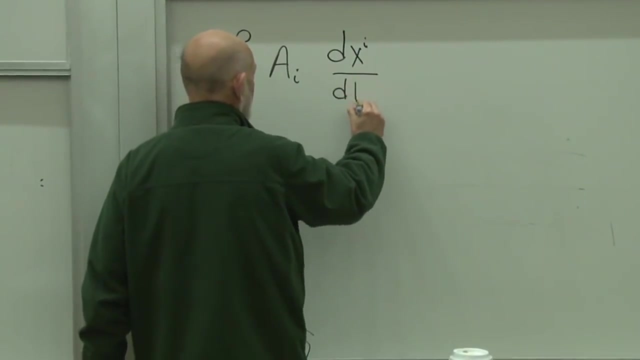 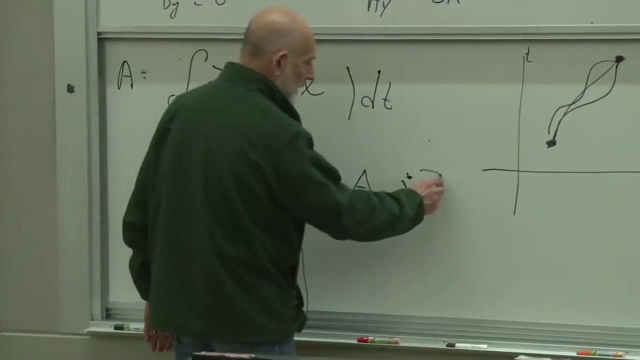 integral of a sub i, x dot. but what is x dot, x dot is the x i by dt, right that is. and now the thing that i left out of this integral here. this is not a decent looking integral. it has to have d something and dt. 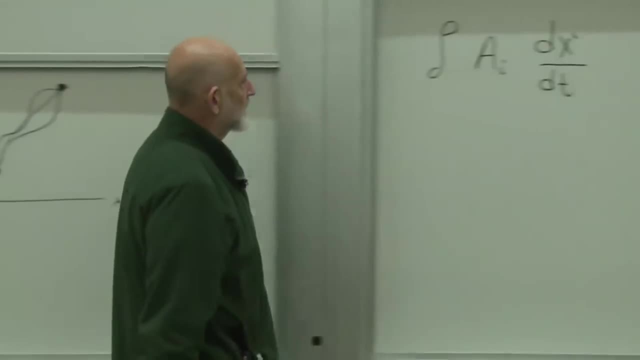 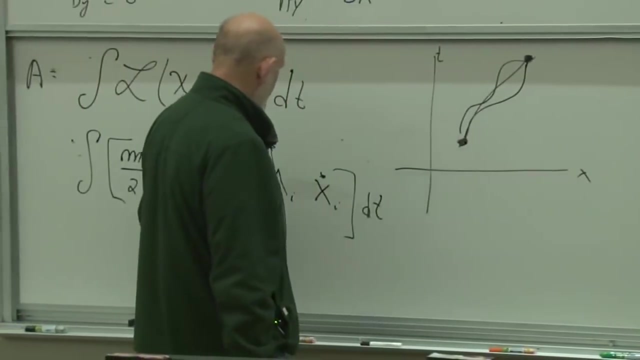 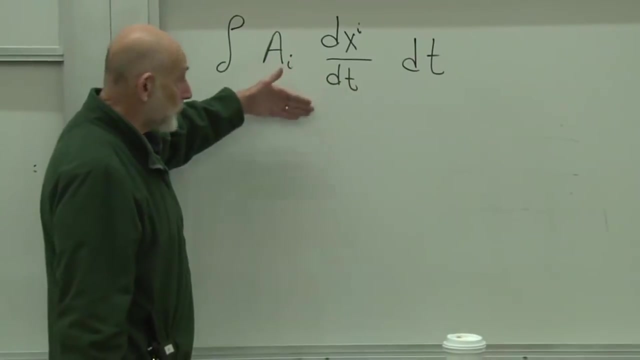 we have to put dt there, so we'll want to put dt here. that's the contribution to the action apart from the factor of e over c. this is the contribution to the action coming from the new term. okay, how does it change if we do a gauge transformation? 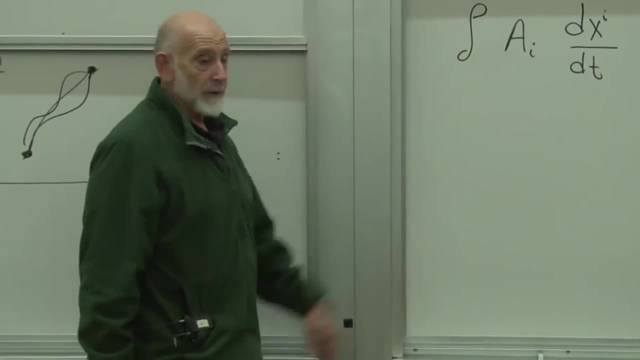 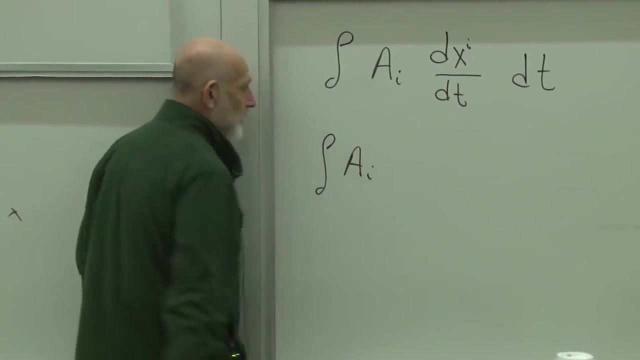 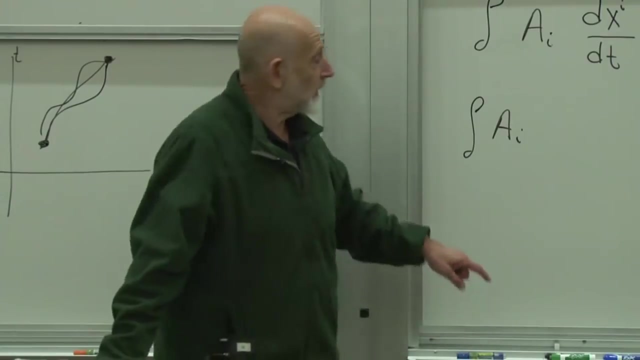 well, let's do a gauge transformation and compare the answer with this. if we do a gauge transformation, We will be writing a sub i. Now What's what's the gauge transformation? You add what to a Gradient? what is the component of a gradient? the ith component of a gradient. 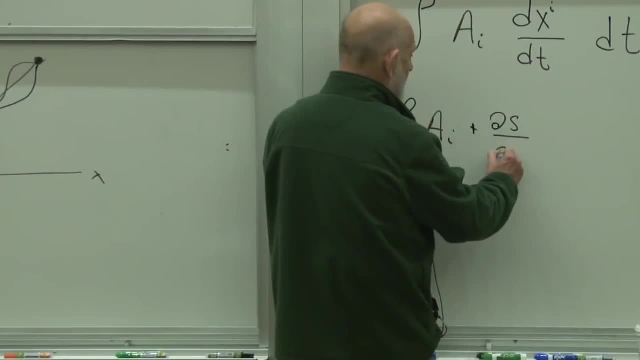 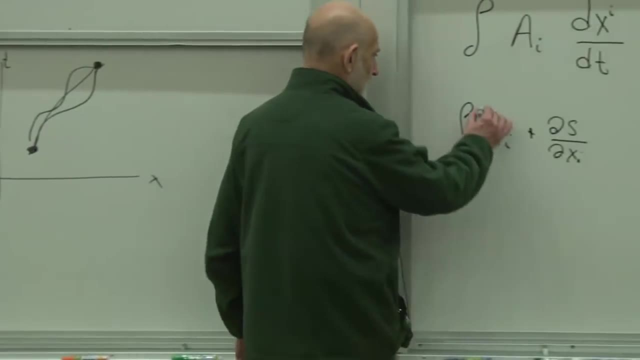 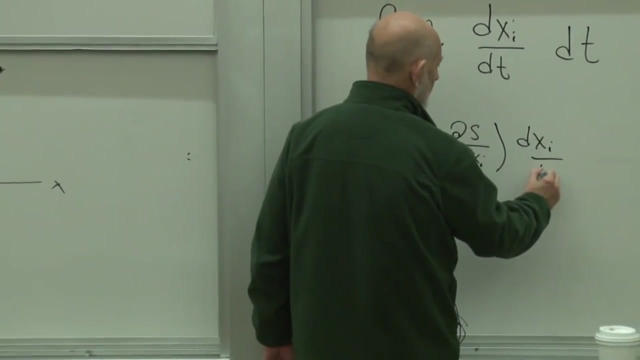 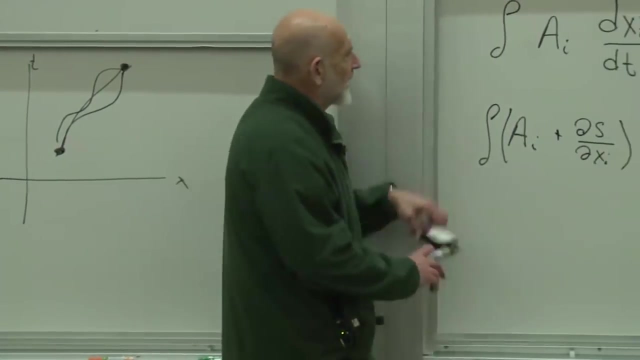 Plus partial of some scalar with respect to x sub i. You can choose that scalar in many ways, every way. where you choose it is another gauge times the x i By Dt, Dt. well, the first thing is, even before, Before making the gauge transformation, even before doing that, let's just notice that the Dt's cancel. 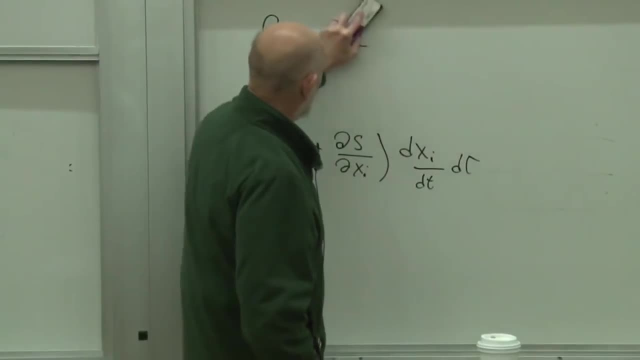 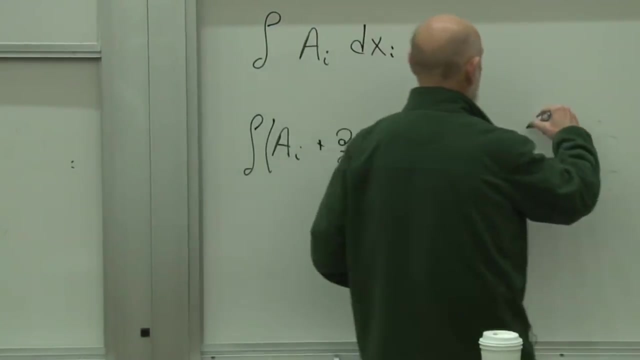 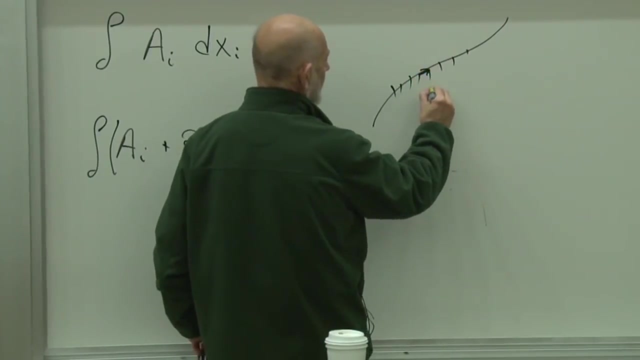 All right. so this is. this can also be written as integral: the a, i, the x, i. What does this mean? it means you have a trajectory. You break up the trajectory into little pieces. each piece, each little interval. here can be written: Dx, I. 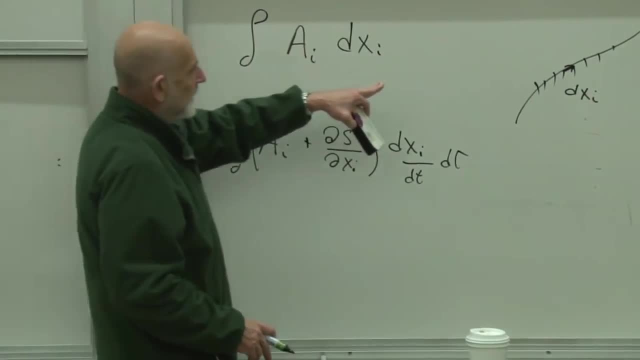 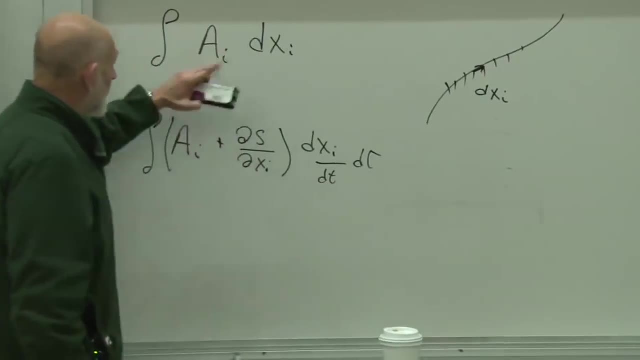 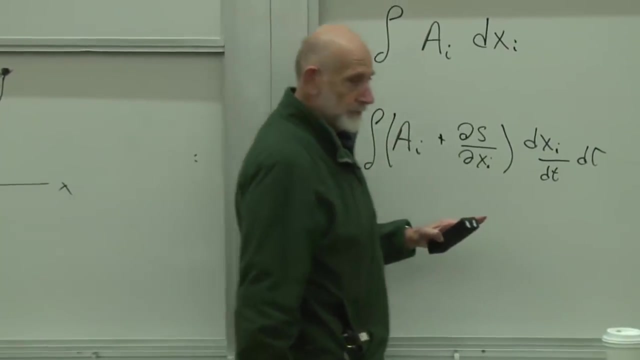 You take each little interval and you dot it into the vector potential And you add them all up. It's called a line integral. in other words, the additional term in the action is the line integral of the vector potential. another way to think about it is: it's the integral of the. 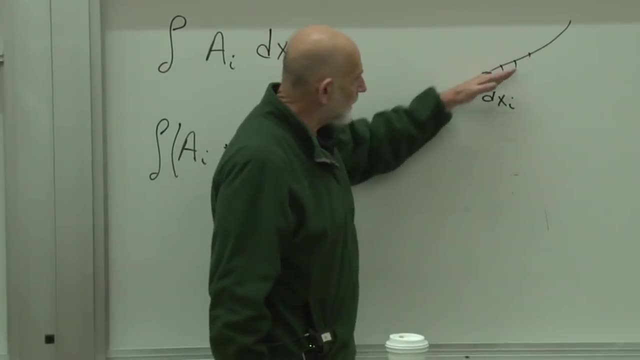 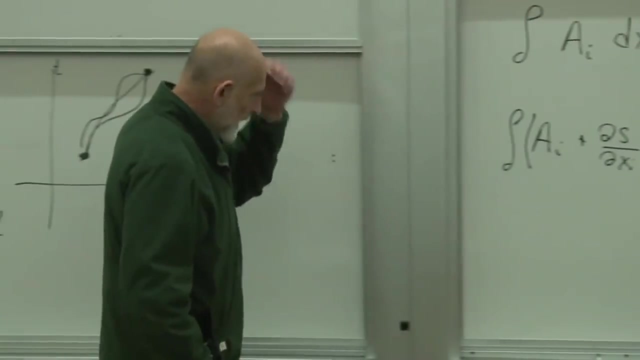 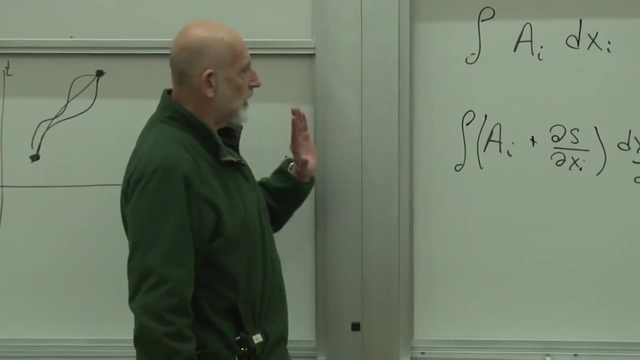 Component of the vector potential along the trajectory, Integrated from the beginning of the trajectory to the end of the trajectory. That's the new piece that we're putting in. But if we now change a by a gauge transformation, We've changed the action by this much. Here's the change in the action. 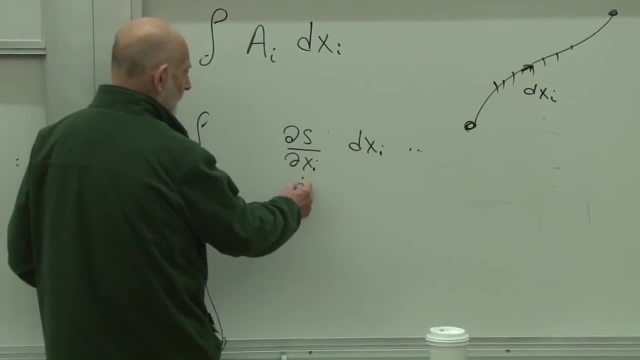 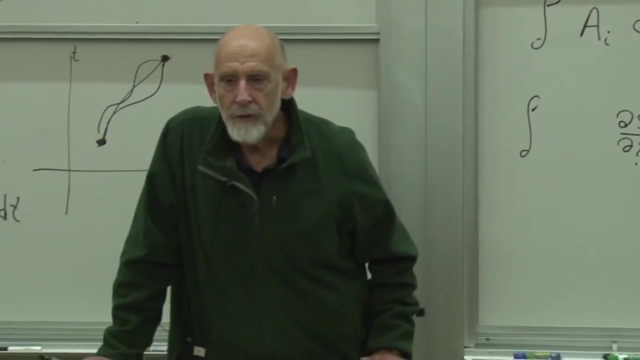 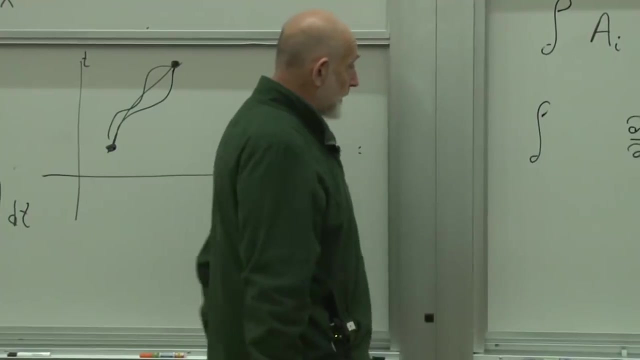 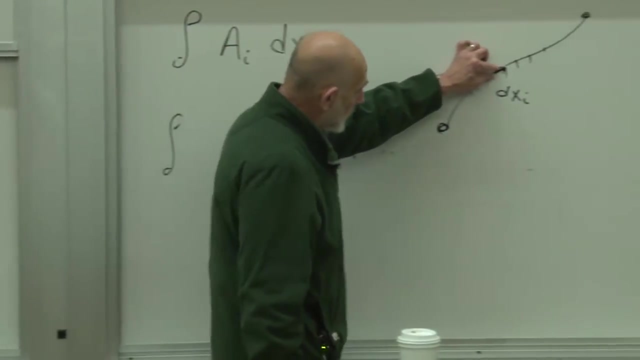 Let's write it out: the s by the x i, the x i and the. that's the: the change in the action under a gauge transformation. How about this? What is this? this Is the change in s when you change x i a little bit. in other words, when you move along the trajectory times, the x i. 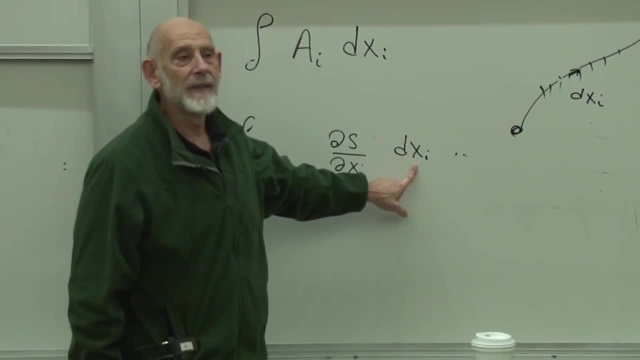 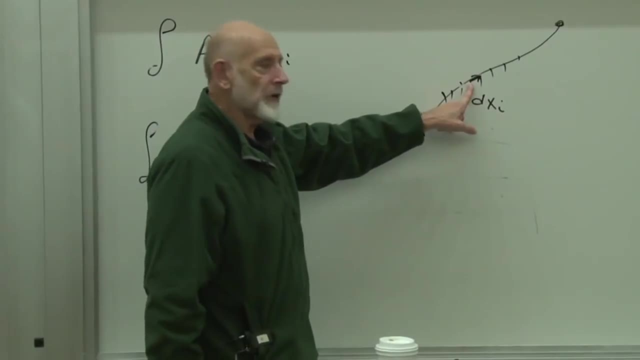 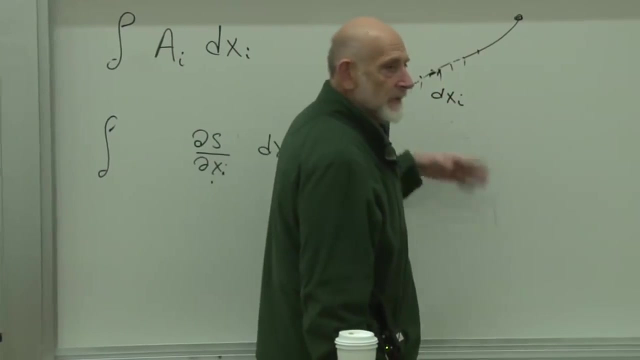 What does that give? Yeah, it just gives you. well, each little interval gives you the value of S at the one end of the interval, minus the value of S at the other end of the interval. If you add them all together, they'll all cancel out, except the ones on the endpoints. 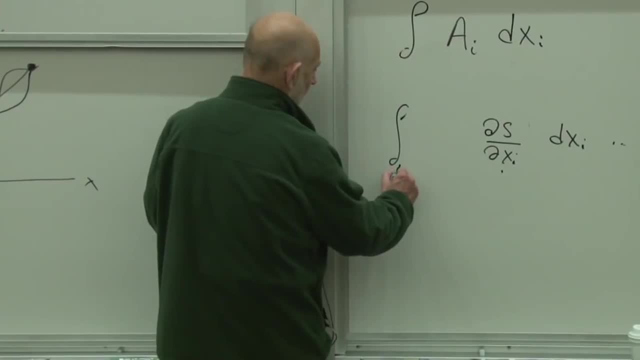 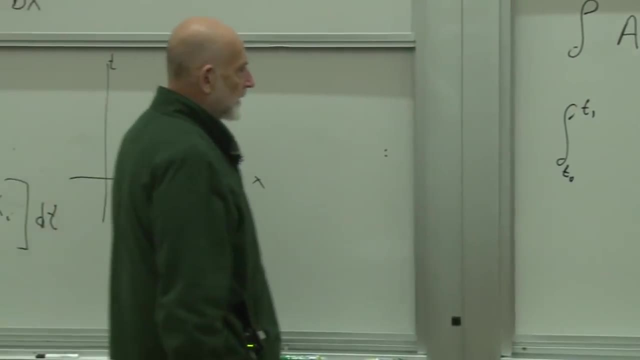 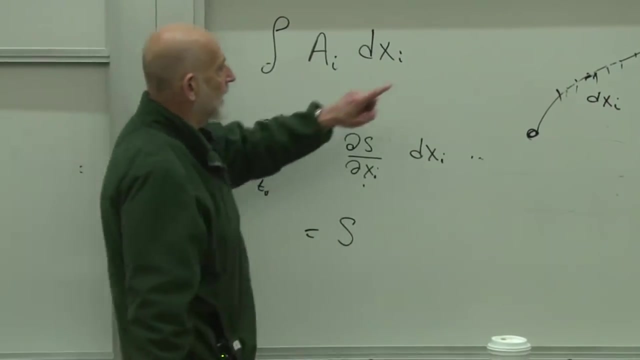 So all together. let's see this goes from T initial to T final. let's say Zero to one. This will give you the value of S at the end of the trajectory. Let's call that. tell you what I'm going to call this initial and final. 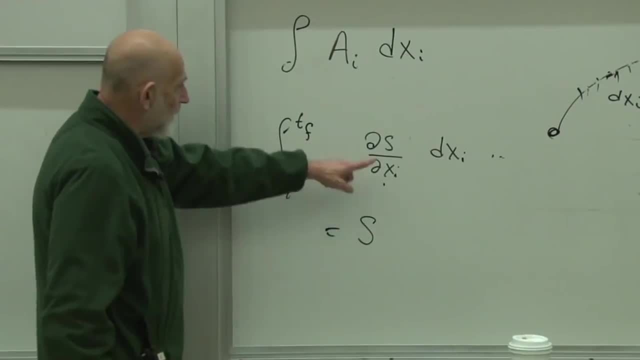 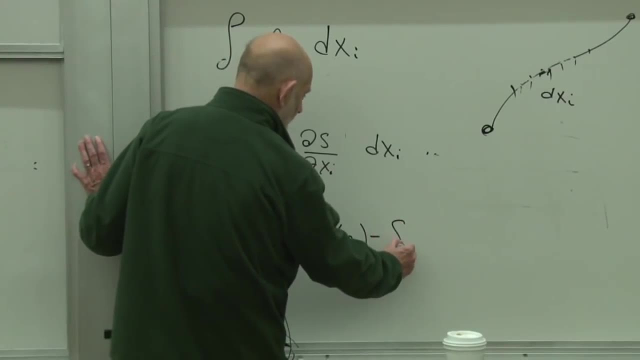 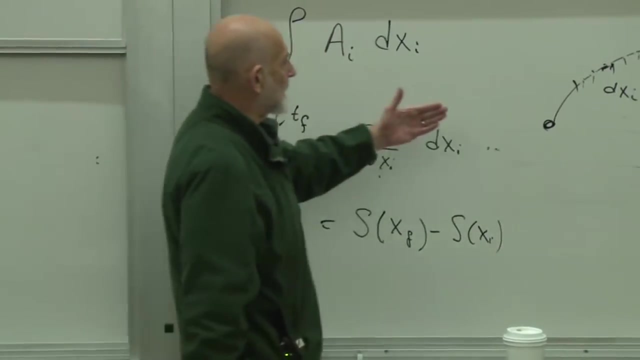 Initial and final. It gives you the value of S at the final position minus the value of S at the initial position. In other words, the whole thing only depends on the trajectory and the value of S at the end of the interval, At the ends of the trajectory. 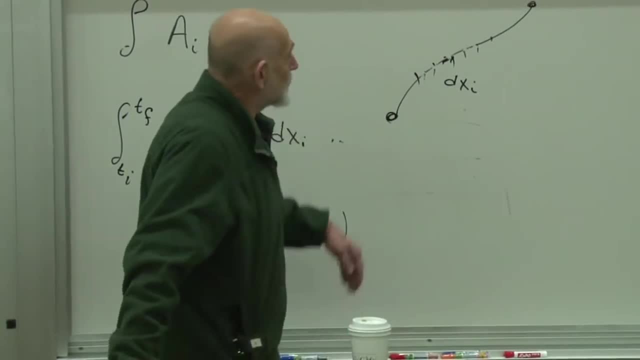 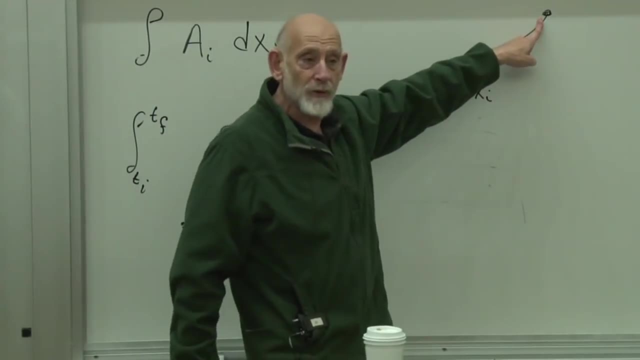 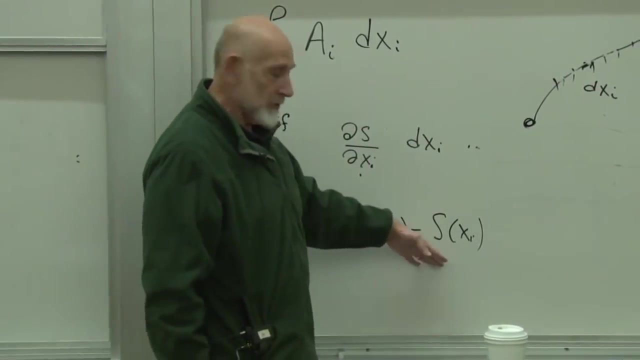 Now, what is the action principle? The action principle says the true trajectory between here and here is gotten by exploring different trajectories, keeping the endpoints fixed. If you keep the endpoints fixed and you do this exploration, then the S's will only be evaluated at the endpoints. 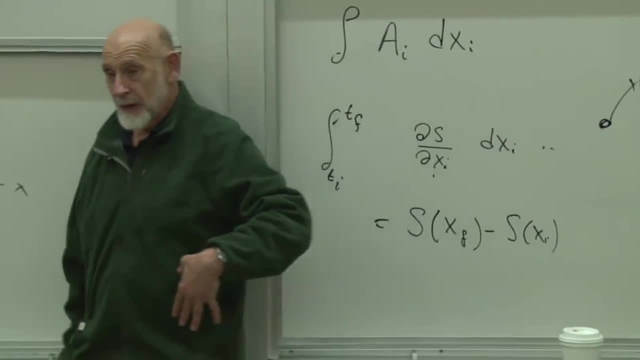 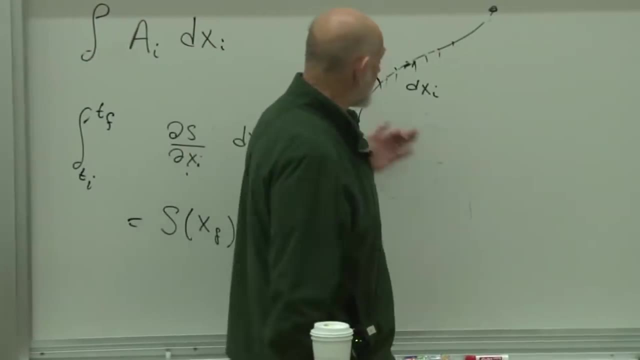 and they won't change as you wiggle the trajectory. So this is a contribution to the action, Which really doesn't depend on the trajectory at all. It depends on the endpoints of the trajectory, but in using the action principle we keep the endpoints fixed. 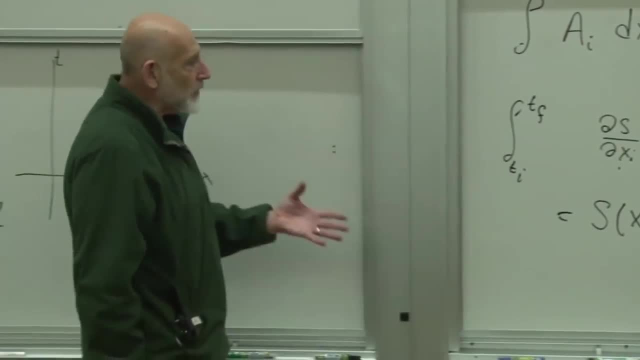 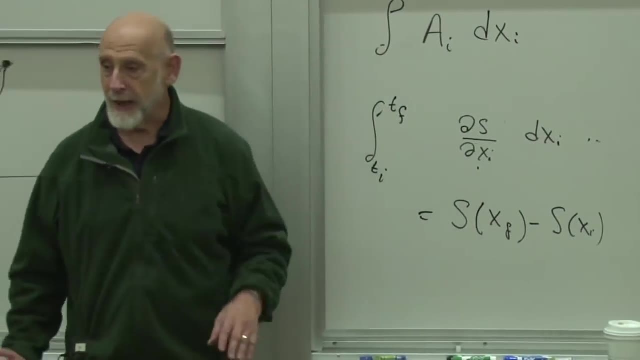 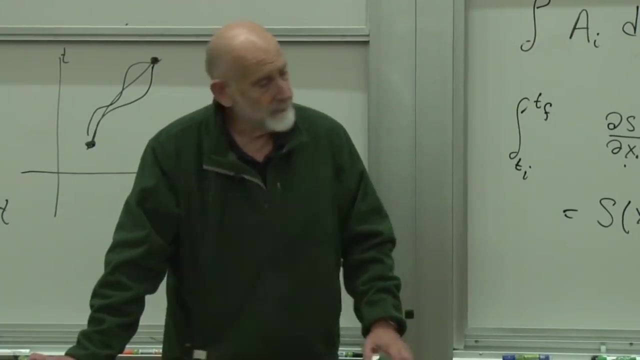 The result is that the equations of motion and the choice of correct trajectory will not change when you do a gauge transformation. So it's not quite true that the action is gauge invariant. It gets a new contribution, But the equations of motion that follow from it.